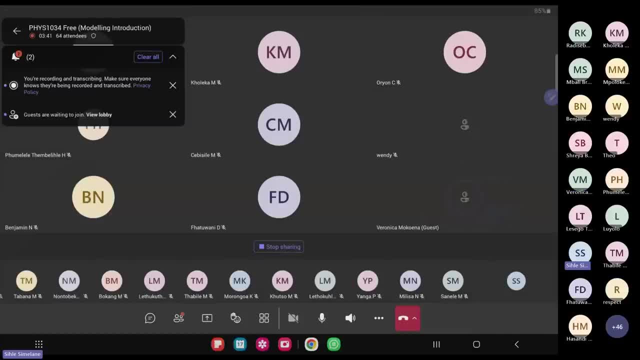 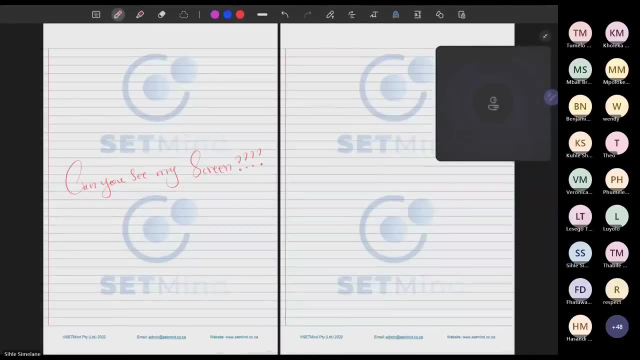 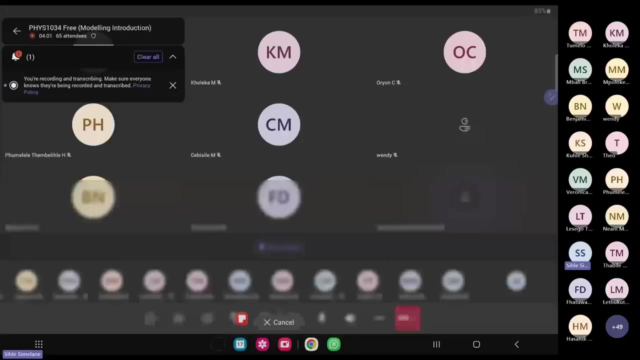 Keep the mute in and then you will unmute when you have a question. Okay, so good morning to all and thank you for coming. I think you should be thanking yourself more for coming than I am thanking you, because means you are taking the very first step towards making sure that you do well in your academics. 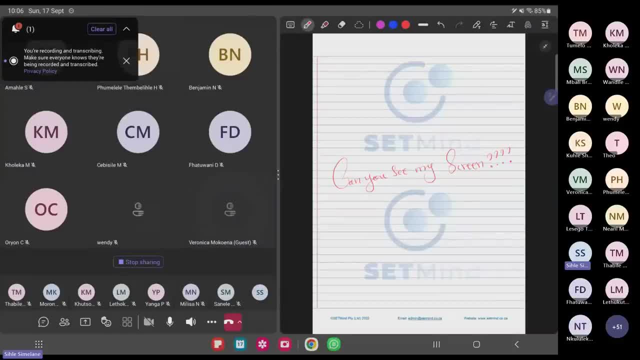 So I think you should applaud yourself and give yourself a round of applause, because other people are doing things which will not really help towards making their academic journey and attaining their engineering degree to be easy. So I want to see yourself clapping for yourself there, because 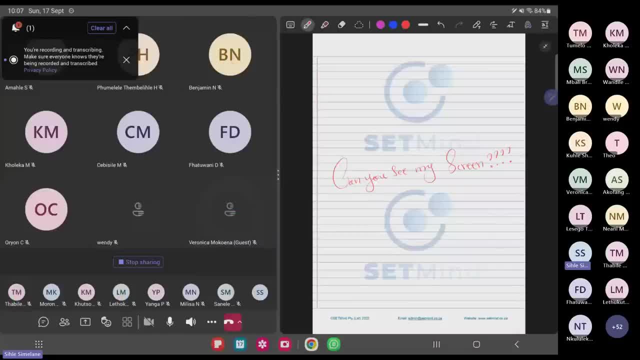 this Sunday, I think we could all be doing with watching some movies or going outside. So discipline starts today and if you carry on the same attitude, believe me, you'll be out of the institution in three years time, or four years time for those who have really not done okay for first semester. 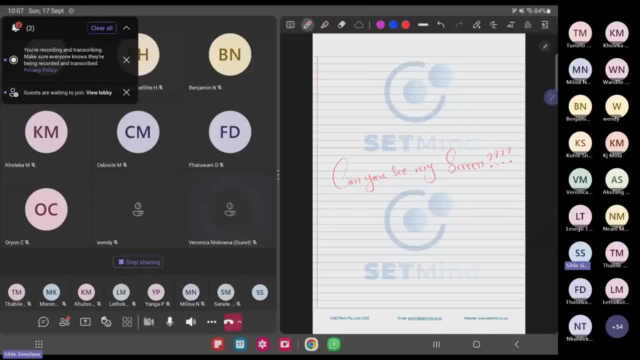 So I need two things from all of you, those who are in the meeting. so if you can see my screen, there's people on the on the lobby, so I cannot admit them once I start writing. So when you see someone trying to enter the meeting, please afford them the right and admit them to the. 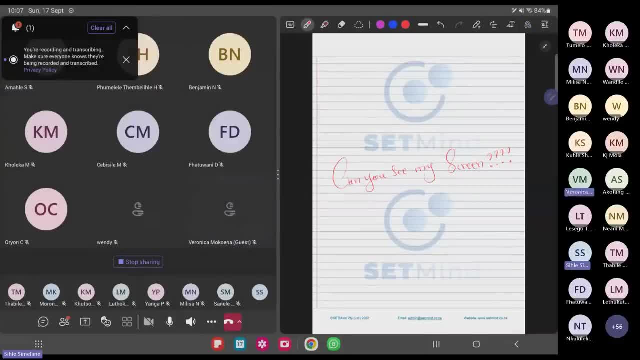 meeting so that they can gain as much as you are going to gain. So when a pop-up shows up on your screen and say admit, Admit everyone as soon as you can. And then number two, I should be the only one that win. So I'm aίy be the only one win. So number two, I should be. 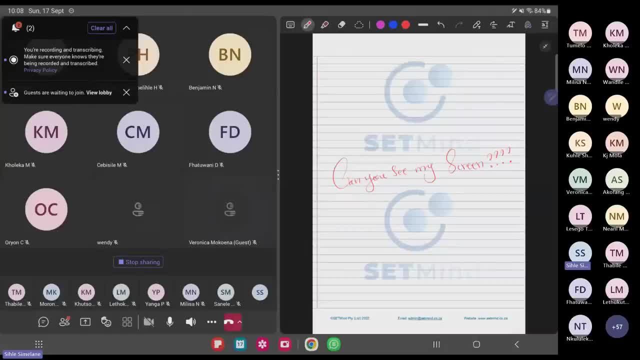 who's recording the meeting. for a simple reason: if any of you start trying to record the meeting, i will not be able to access it later, because later, when i access it, i'm gonna download it, upload it even on youtube or send it through for everyone who was not able to attend the meeting. 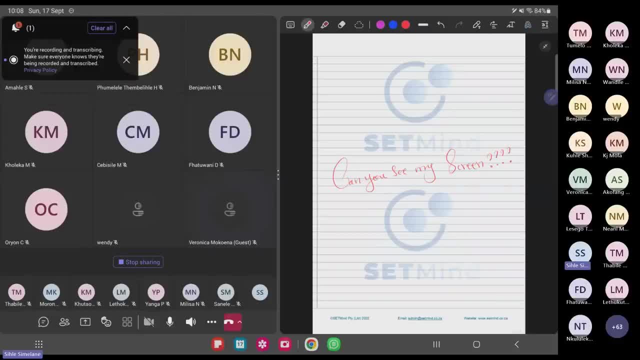 but if you record it, you are the one who's going to be able to see it and no one else will be able to see the meeting and you might not be able to share. so please, if you are recording, stop the recording. if you did not start the recording yourself, then do not worry, it's all okay. 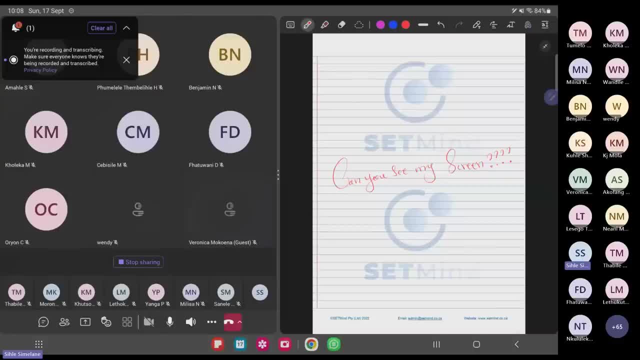 and then the second thing which i need from you is, once i go to the screen where i'm writing, i cannot see the chat section. so since i cannot see the chat section, please, when you see a question which is typed if you, if you can unmute, read the question outline. 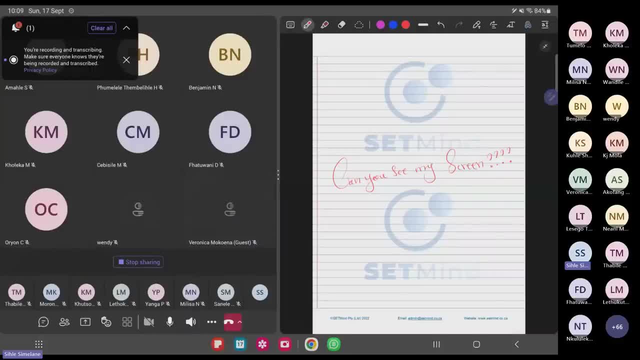 it out loud, because i cannot see the chat section once i start writing. so those are the things which i need from you. if you see a question on the chat section, be reminded. i'm not going to be able to see the question. so if you can afford to unmute and say: 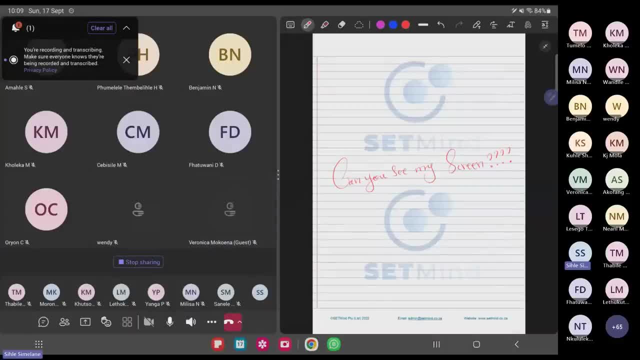 there's a question in the chat section, because in abc is saying: why did you multiply that part by this? then i'm going to be able to respond because i cannot see the chat section. so do we have any questions in advance? so if you are all ready, please give me a hands up, give me some thumbs up, so i want to see them. 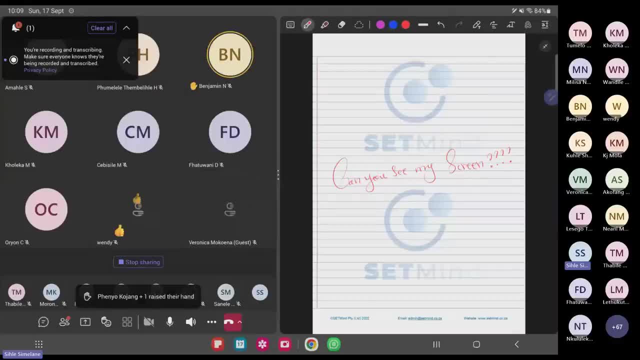 on the screen. it's still early. we should not be numb. we should approach this block with a different attitude. what happened last block has passed, so i'm expecting many thumbs up here. it's still early in the morning for us to be not light spirited. i need more. 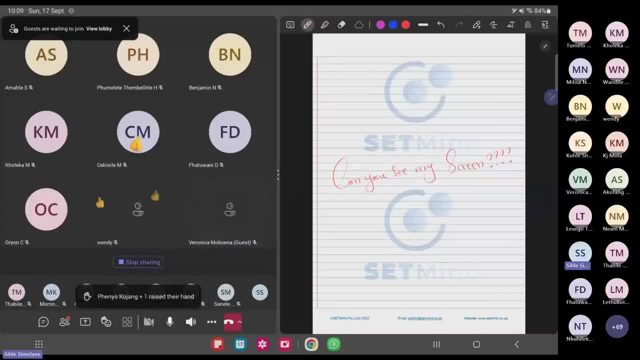 make sure you check your mic should not be muted. and for us the question: let's be cooperative, it's too early for us to not be happy. the block just again. some people just say we just arrived. so let me confirm the last time if i am recording and then we can kick start so that the recording 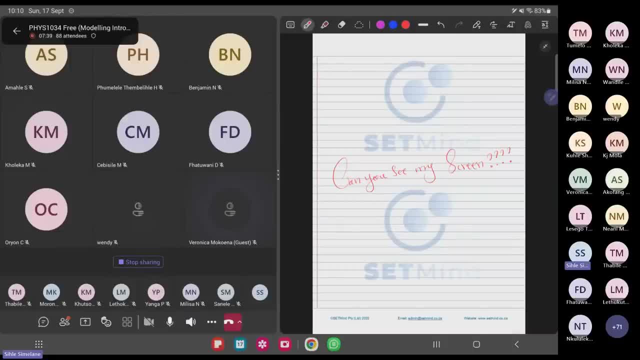 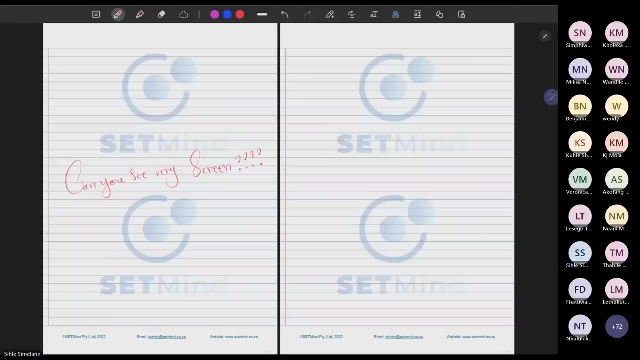 is up, so i'll move from the screen and then remember. when you see someone trying to enter a meeting and guess a question, let them answer. style to end: update, so you can do it. so i just forget to give you my screen. okay, sweet, if everyone wants to hear me and they can see my screen, then that's business of the day. and the people who are muted: please look at your mic. you should all be muted unless you are asking a question. let's make a session to be waited. 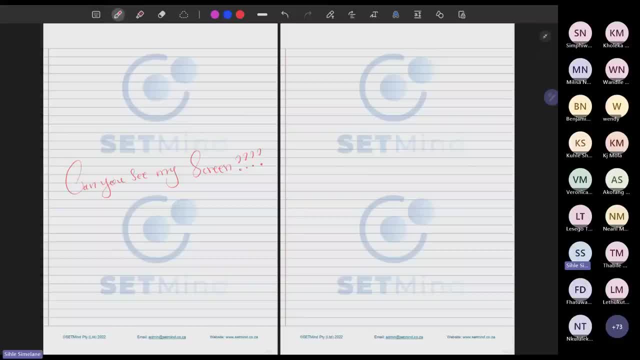 really push it quickly if i see people. so let us now move on. so let's all take a break and focus on um learning about dance, because we all decided to set our time apart to come here and learn. So let's not be destructive by having our mics not muted. 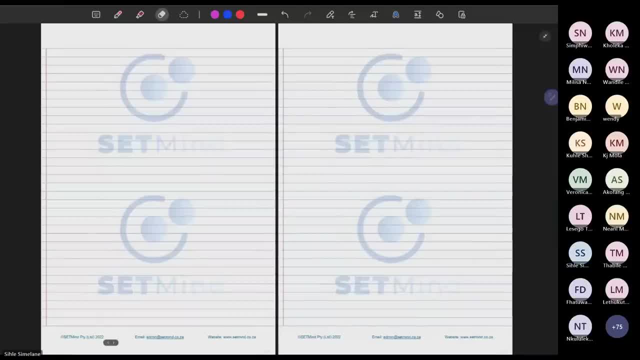 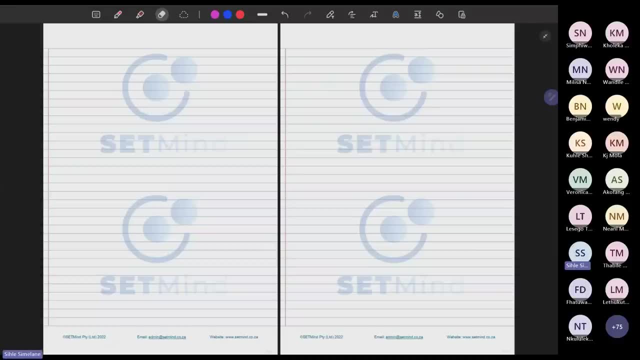 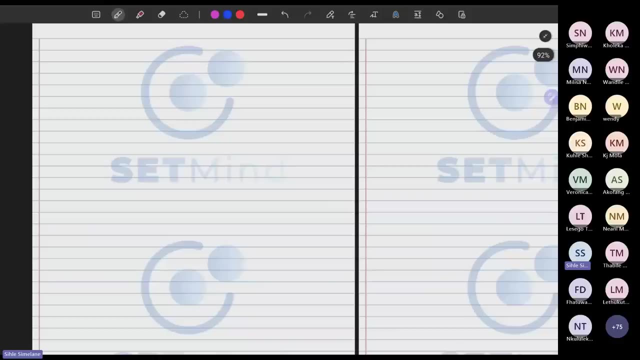 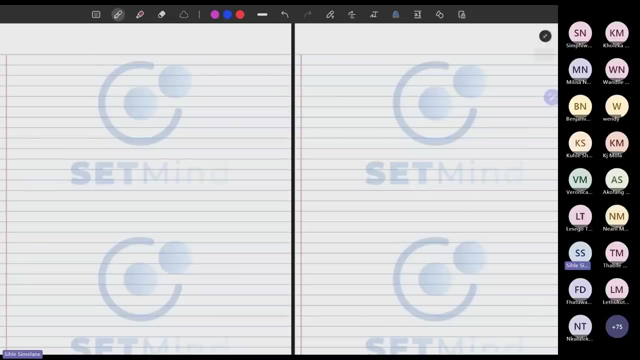 especially when we are not asking questions. So if you saw the poster which was shared- I believe it should be yesterday- One of the key points which was written there, essentially, was that we are going to do an introduction to modeling and then we are going to focus on dimensional analysis. 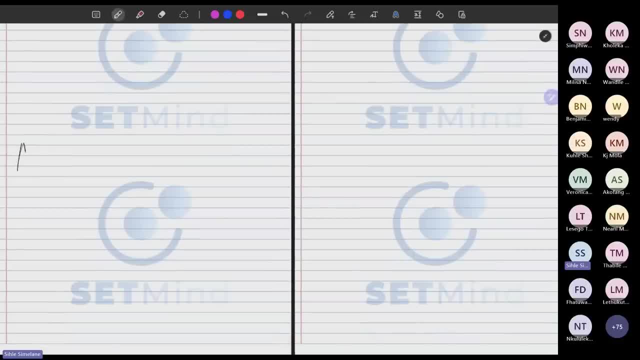 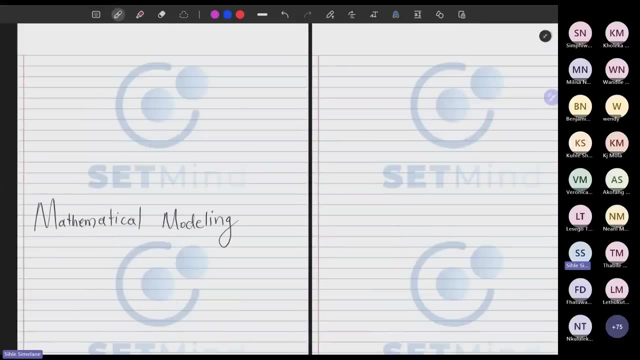 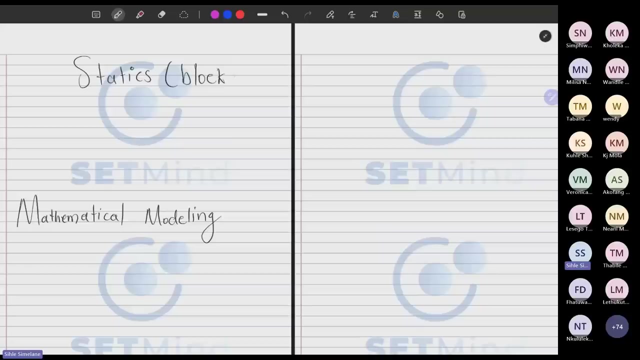 So if you look at applied physics- this block- you will be doing what they refer to as mathematical modeling. That's the focus, this block. So last block you were dealing with statics. this was your block three, and this you will do for the entire block four. 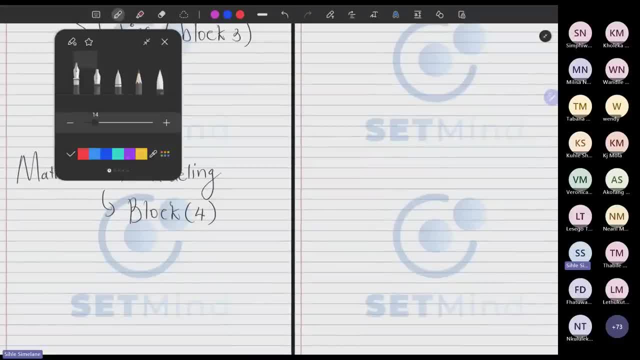 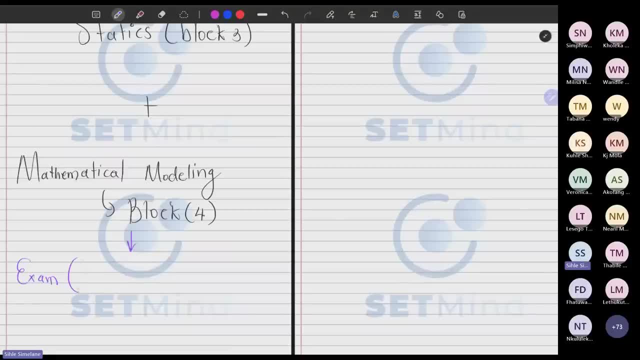 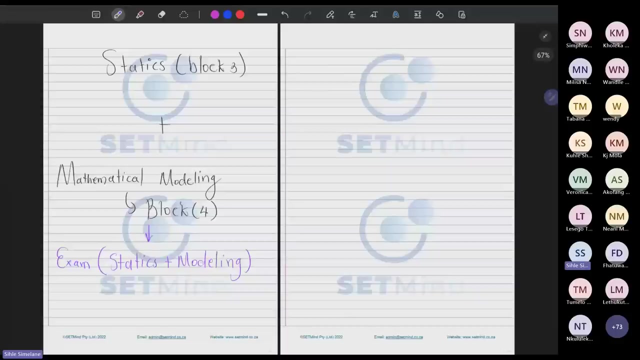 And what you should be aware of is that your exam, your final exam, will assess both statics plus what you are doing now, which is modeling. So, which means, come December, you should be proficient in statics and you should be proficient in modeling. 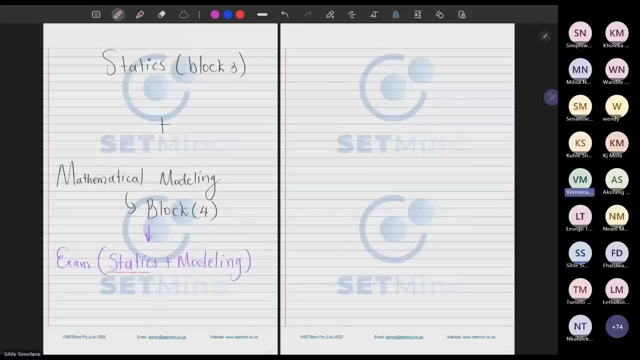 because your final exam will compromise of statics and you will also have modeling. So, to those who think we're done with statics, just be aware that you will need to do some revision before you write your exam, because it's going to be statics and modeling. 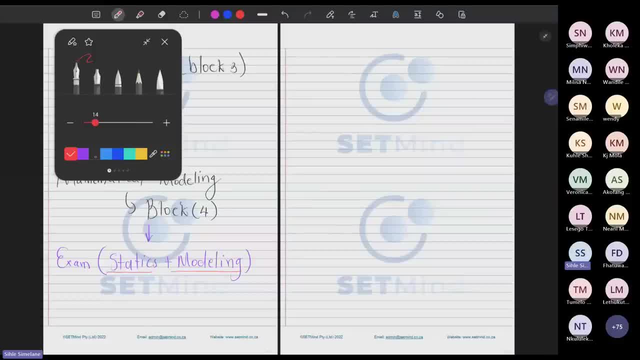 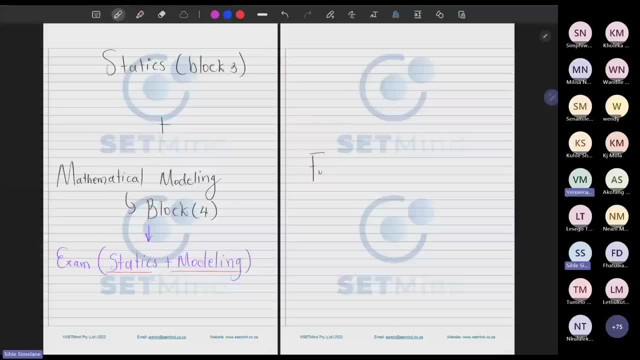 So our focus today, obviously, will be modeling, because we have passed statics, So let's quickly dive into what do they mean when they say modeling? Do we dress up a certain way, Do we walk a certain way? And the answer is no. 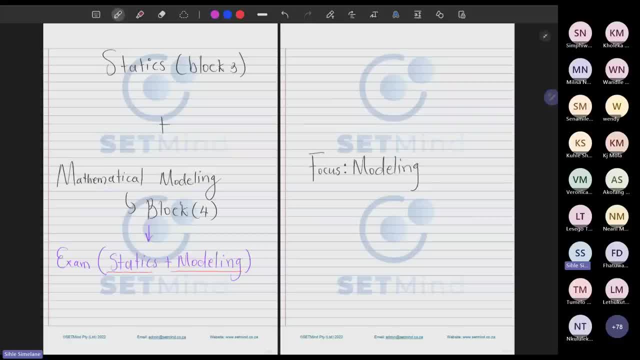 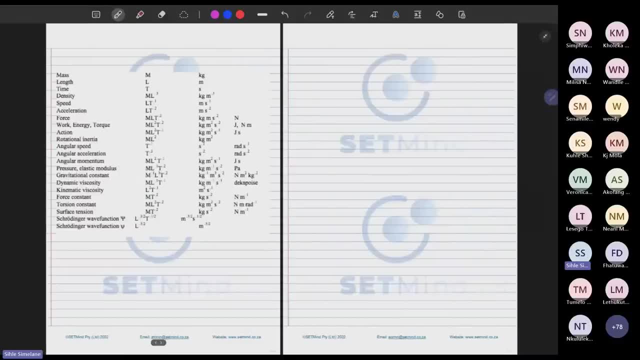 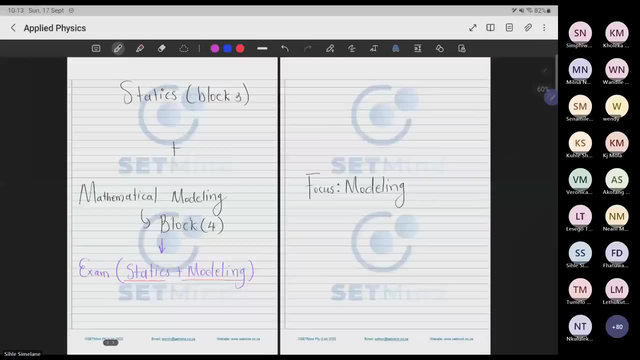 But we certainly need to think a certain way for us to be able to do modeling. So when they refer to, when they talk about modeling, let me add a page. We'll come back to what is there, So let's add. 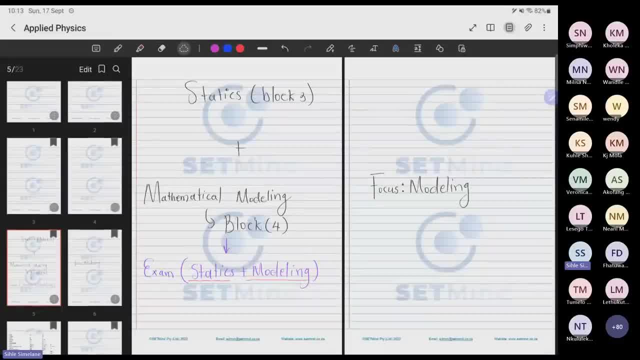 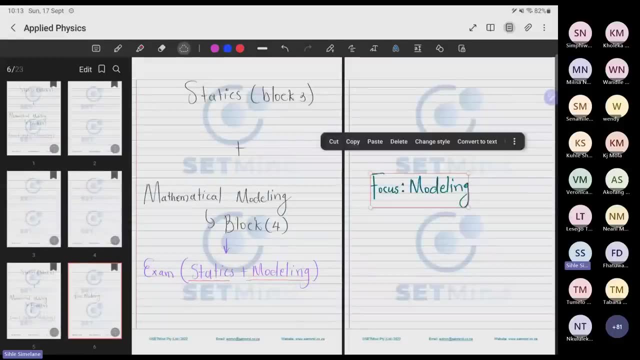 Here. I made a dire mistake here. Let's quickly rectify that. It's really easy. We always make mistakes and we should rectify them. Copy, And I need this one. Copy it and then paste it here. There you go. 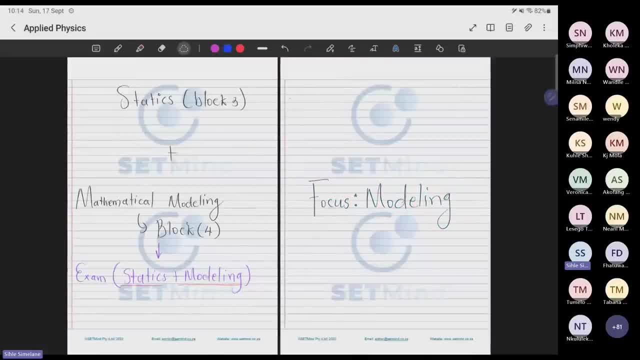 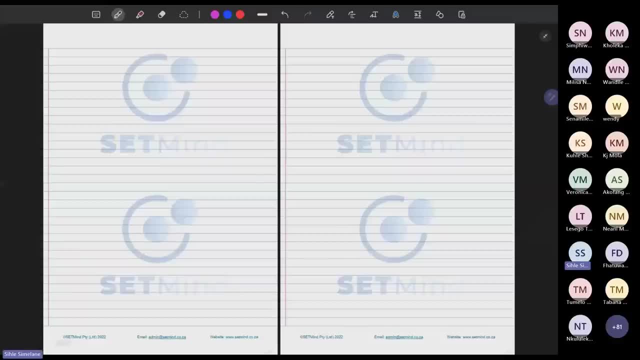 Easy. So when you make a mistake on the exam, you should be as fast Spot the mistake when it's very early. So when we speak of modeling, I'm just going to give you a number of examples which you should think of. 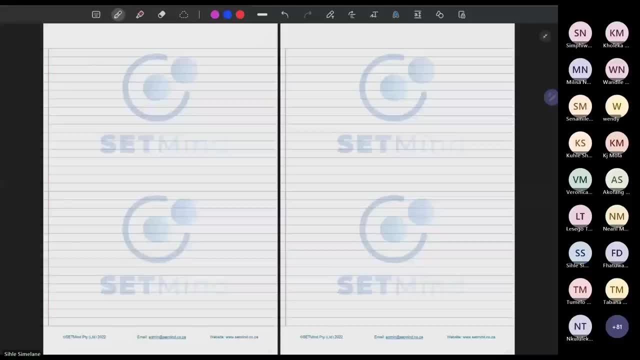 So think of yourself as this engineer. You are faced with a problem and you need to do mathematical modeling. So one of the examples where we will use mathematical modeling is when we are trying to estimate the population. So say, in South Africa now we have 5 million people. 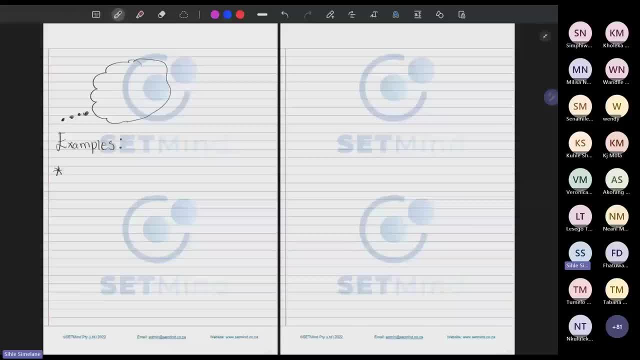 or 70. And then they give you how many people we had, let's say, 10 years back, And they're saying: please estimate 20,, 30. How many people are we going to have? Essentially, when you work around the formulas and then you create a model, 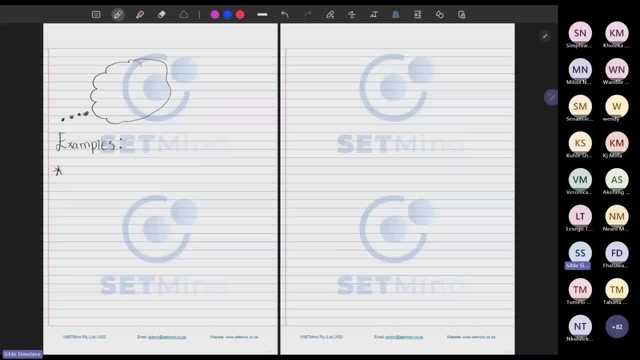 which will be able to estimate the population come 2030, that's what we refer to also as modeling. So one of the examples is population growth. So that's where you are going to use modeling. I will tell you that 2010,. 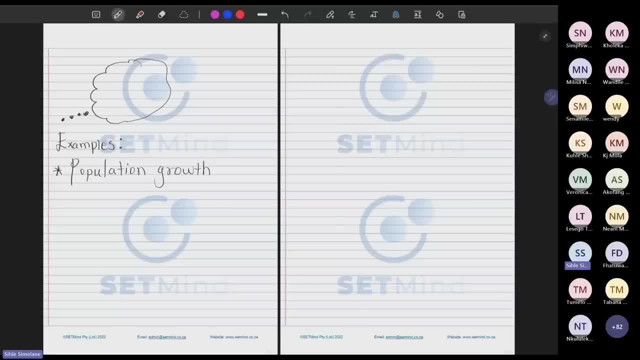 we had 2 million people in SA. Now it is 2022.. Maybe we have 7 million. Please try to determine or estimate how many number of people we are going to have come 2050. And what you will be applying there. 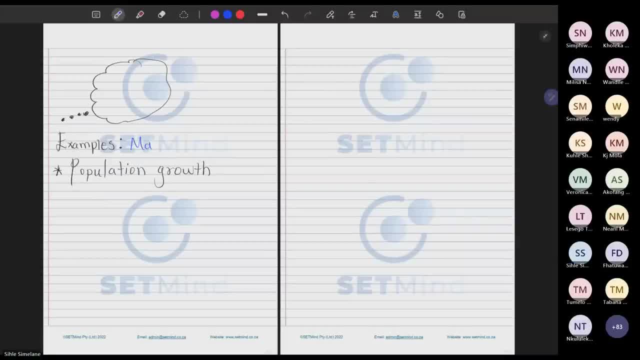 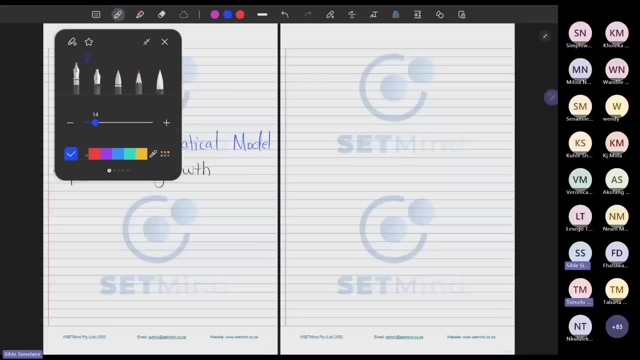 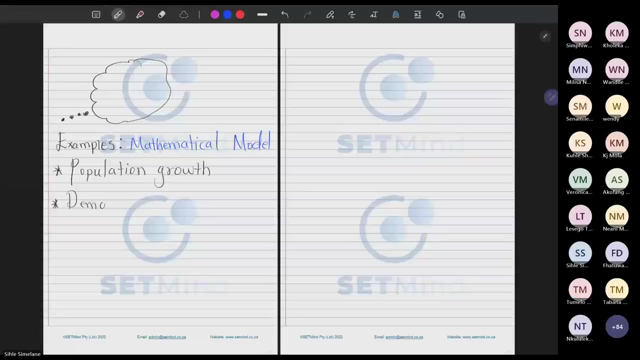 is mathematical modeling- Mathematical, let me call model- And one of its application is: we'll use it in population growth. And then another area where you will apply mathematical modeling is what we refer to as demand and supply. Demand and supply is straightforward. 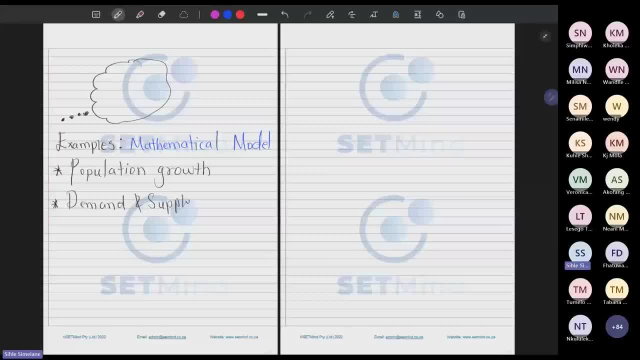 You have a demand which you have currently, And then you have a supply which you have. So if we have a certain demand, let's say in a few years time how much should the supply be? So you need to develop a mathematical model. 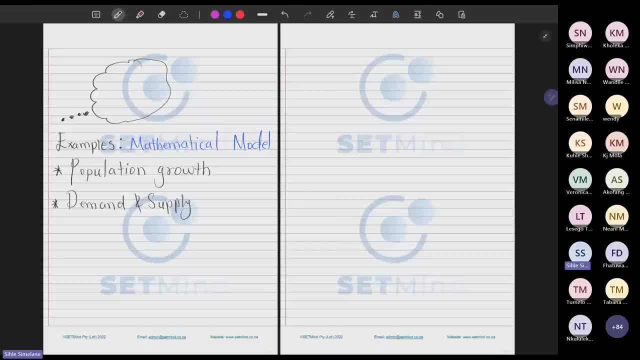 to be able to predict what the demand will be, given the supply and all other parameters which you will be having. Another application, mathematical modeling, is what we refer to as Newton cooling, And this is the one which is more exciting, Because I remember. 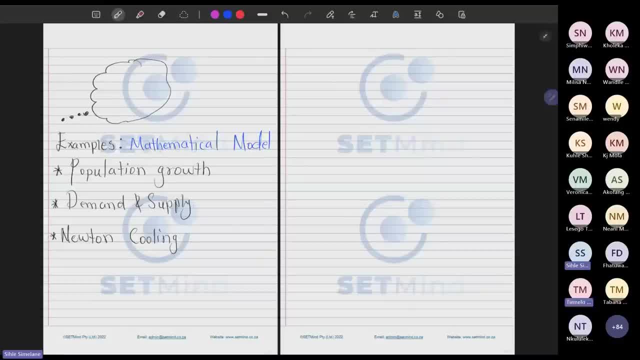 in 2019, the equation paper, when you look at Newton cooling. there was a question which was: I need you to think of this carefully: Does a person or is a crime scene? I want you to imagine this. how you can then use mathematical modeling. 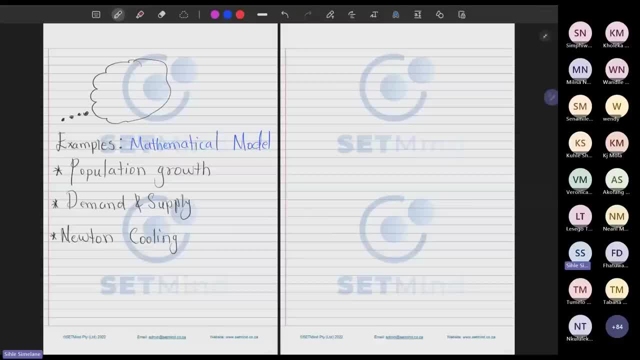 Is a crime scene of a person who has passed on The forensic people. they get to the crime scene at, let's say, 4 am And the body temperature of the person, let's say it is now 2 degrees, And then at 5 am. 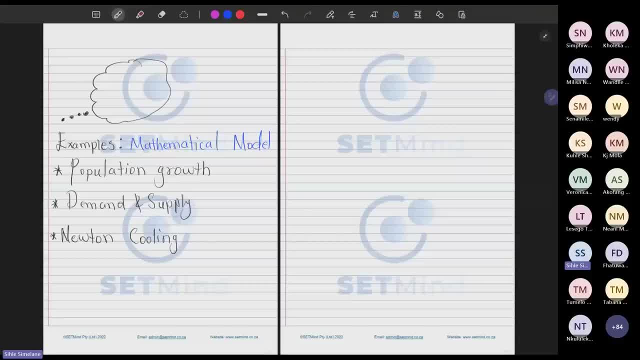 let's say, the body temperature drops to 1 degrees And they are being told that the body temperature of a person, let's say who has passed on, decreases by this amount per unit time. And then now the question to the engineers of 2019 was: 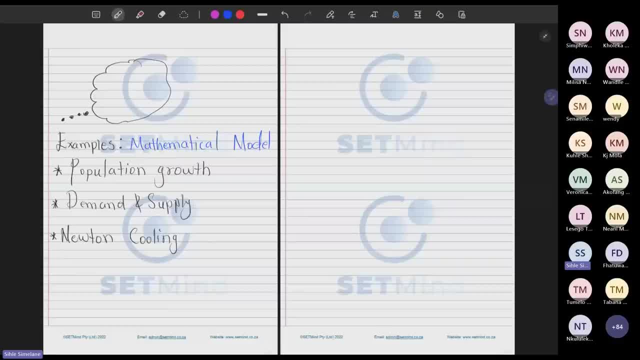 determine when did this person pass on, And all that is mathematical modeling, Which means you get there, you don't know anything, you just know a number of parameters. You need to determine when was this person executed, And it all forms part of mathematical modeling. 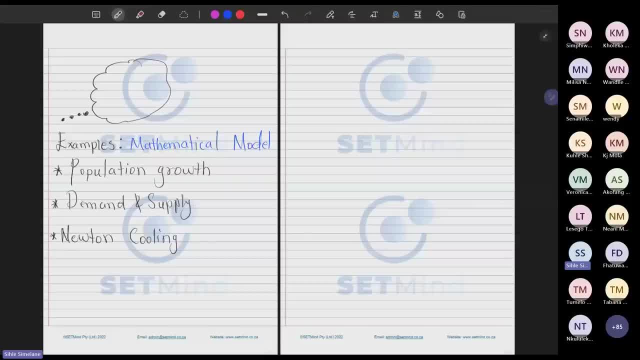 which you might do under Newton cooling That question, it will be there. Or you can think of a glass which is cooling down for your tea. You boil your water, you make your tea and then you measure the temperature of your tea at time zero. 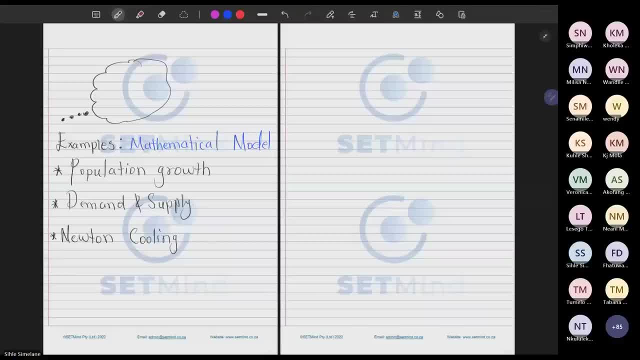 And then you measure again after 10 minutes And maybe you measure again after 20 minutes And then you try to determine how. what temperature would my tea be after an hour? You can easily calculate that using methamphetamine, Using mathematical modeling. 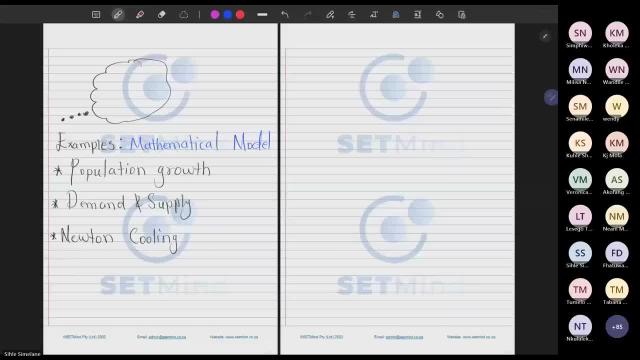 which is exactly what they are trying to equip you with. So there's a whole number of applications which you will do, but mostly you will focus on these, on these three for your course, And then the last application, which is what you will start with this coming week. 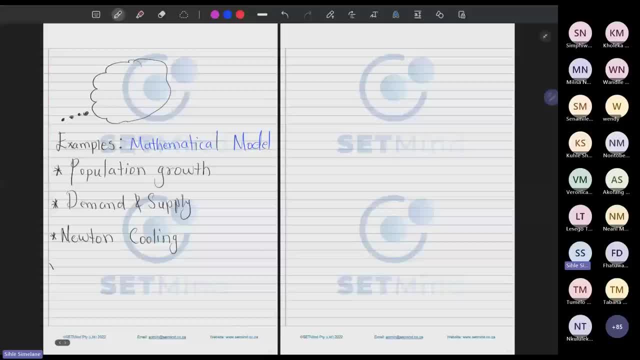 is what we refer to as dimensional analysis, which is what we will be doing. Dimensional analysis- This will be our focus for today, And what we mean when we say dimensional analysis is really straightforward. You should have intuitive understanding of this and then believe me. 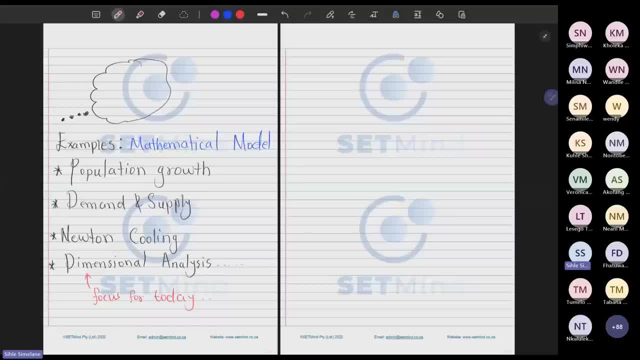 it will make total sense. The person with their mic unmuted: please mute. unless you are asking a question, Please check your mic. Let's all be cooperative. So our focus will be dimensional analysis. So it is story time. So everyone who's in this meeting, 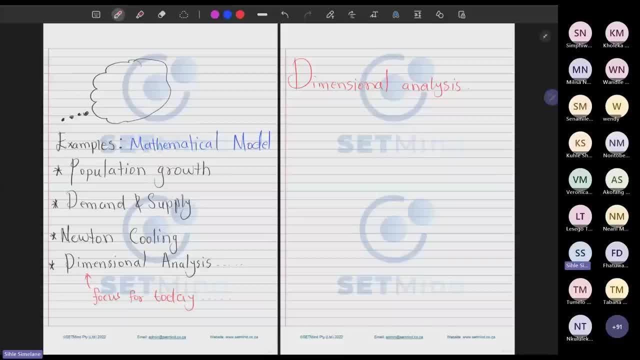 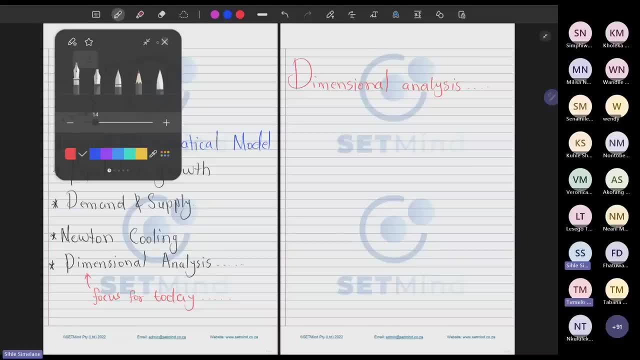 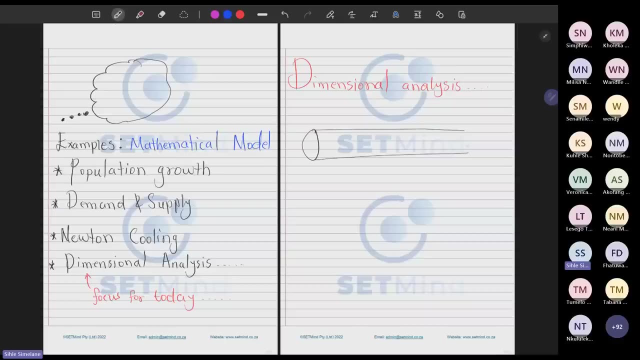 is working towards attaining their engineering degree. But with engineering comes complexity. So let's say, you come across a problem where they're saying: let's just consider a pipe as an example. This is the pipe and we're transporting fluid. There's something which is flowing inside this pipe here. 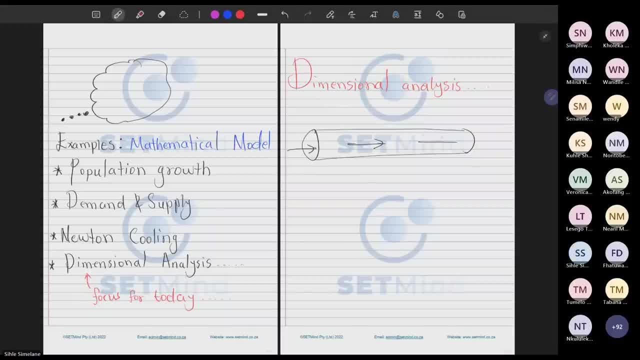 And they say to you: you are the engineer, we will give you the velocity, Velocity At which the fluid is moving inside, And then we will also give you the pressure in the pipe, And then we will also give you D, the diameter of the pipe. 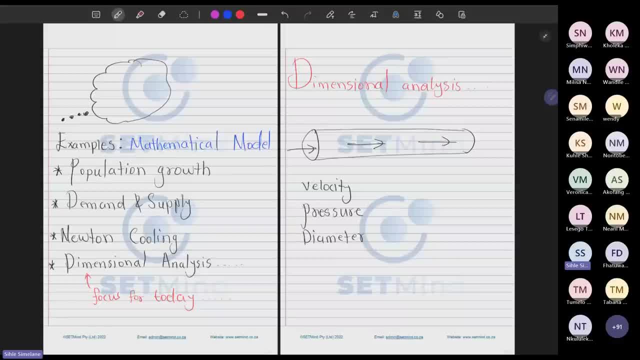 And we will also give you, let me see the length of the pipe. And then they ask you: how is let's phrase the question here? and then we'll try to start thinking. And then they say: how is V? 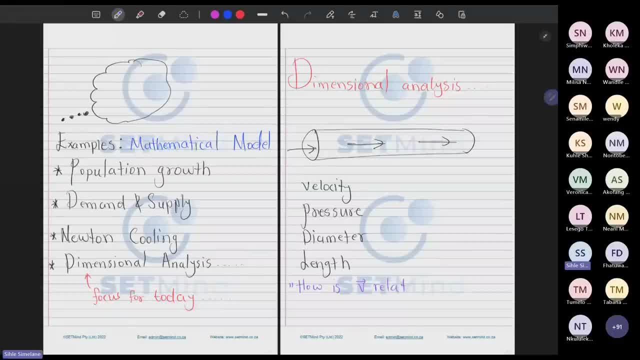 which is the velocity. how is it related to the pressure? It's a question which we are presented with. You have a pipe and then we have something, some fluid flowing inside the pipe. Maybe we are transporting oil. They give you the velocity at which the oil is moving. 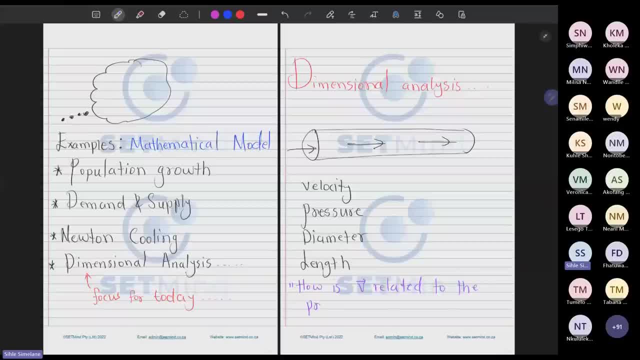 They give you the pressure, they give you the diameter of the pipe and then they give you the length of the pipe. Then the question they ask you is: how is V, the velocity, related to the pressure? The question which you need to think of. 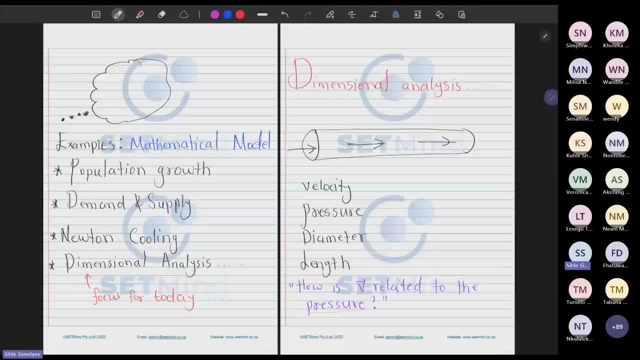 and, if you think carefully, you can always look things up on the internet, but there's certain things which are not there. So you, as an engineer who did dimensional analysis, should be able to unpack and give them the answer that maybe the velocity is directly proportional. 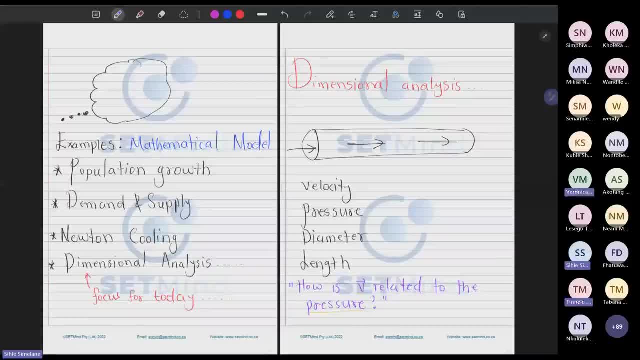 to the square of the pressure. So it is questions like this, among many, which dimensional analysis will enable you to be able to answer. So you should be able to relate variables to each other using dimensional analysis. So let's pause this question for now, and we'll come back to it later. 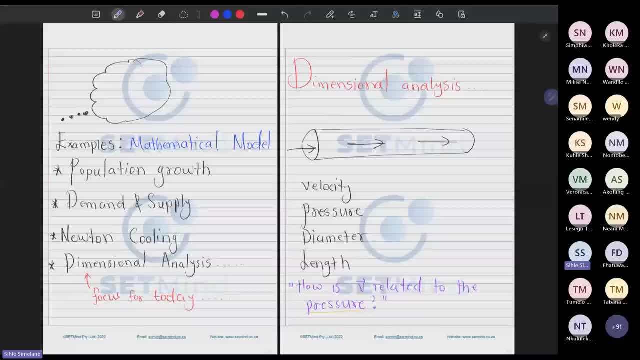 Let's look at what we refer to in dimensional analysis as the fundamental dimensions. We are building up towards being able to answer such questions, And if you can be able to grasp what I'm about to say, the next two or three weeks will be easy for you. 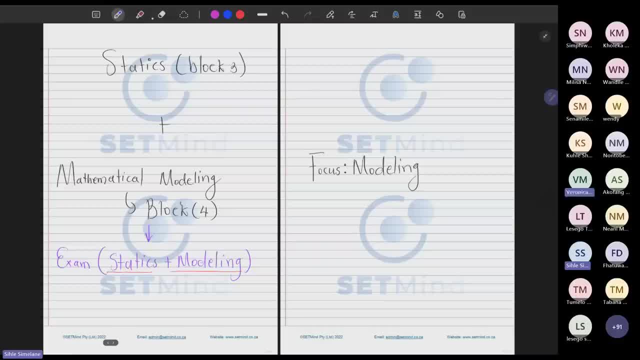 So we are still on dimensional analysis. There's something which we need to look at, which we refer to as the fundamental dimension. Let me erase this and then we get to that. So, just like we have fundamental building blocks, even in dimensional analysis, 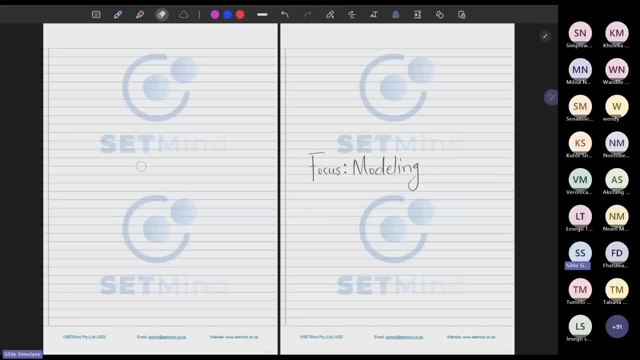 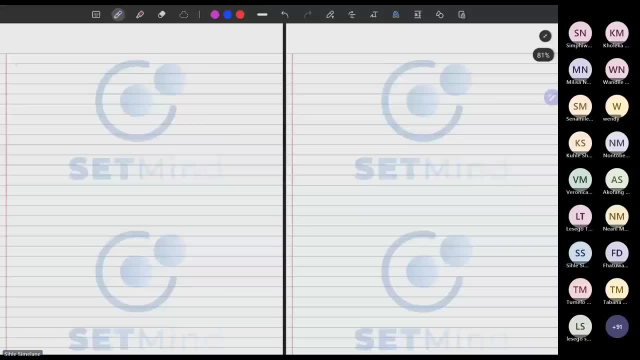 we have fundamental dimensions, So we have what we refer to. I'll say note, because this is what you need not to forget: So we have what we refer to as fundamental dimensions And our fundamental dimensions one. the first one is time. 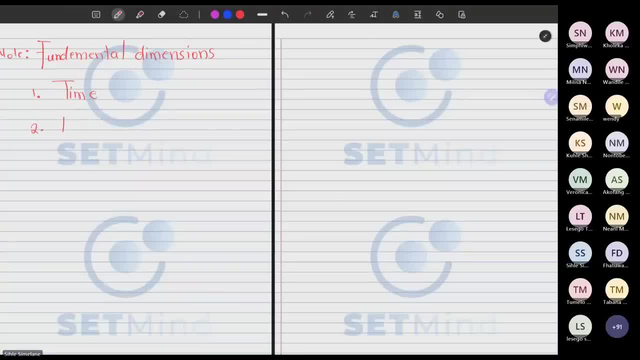 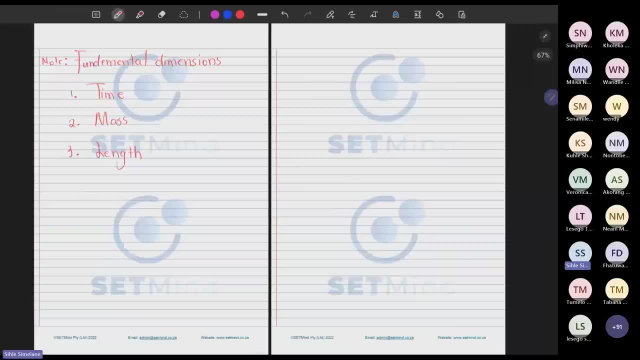 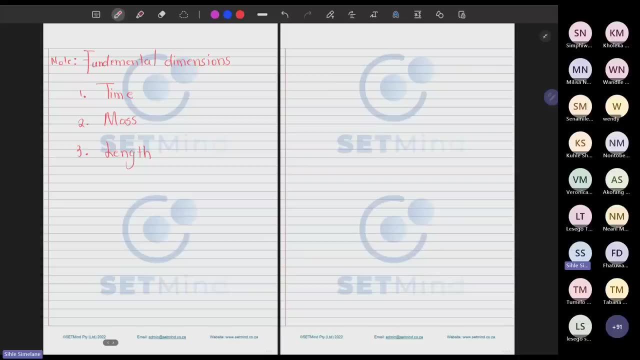 The second one is mass And the third one is length. These are what we refer to as fundamental dimensions- time, mass and length- And using these fundamental dimensions we can then create different variables or different properties which have different fundamental variables. 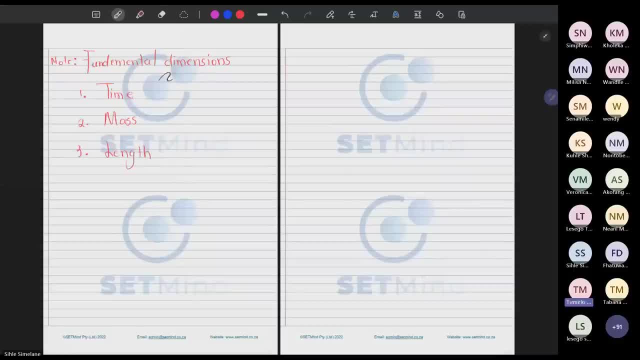 So time we'll denote it with T: Fundamental dimension is T, And then mass, its fundamental dimension will denote it as M, And then length, its fundamental dimension will represent it as L. Okay, So remember, we're looking at dimensions. 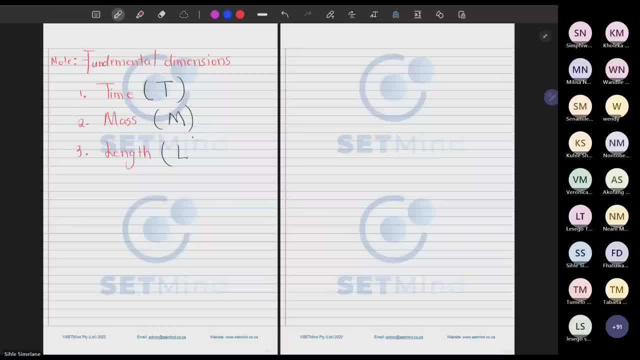 not units. So dimensions make units. So that's one thing you should be noting. Let me just say here I will say: dimensions make units. So someone else: where they were looking, where there was mass, they were tempted to say: 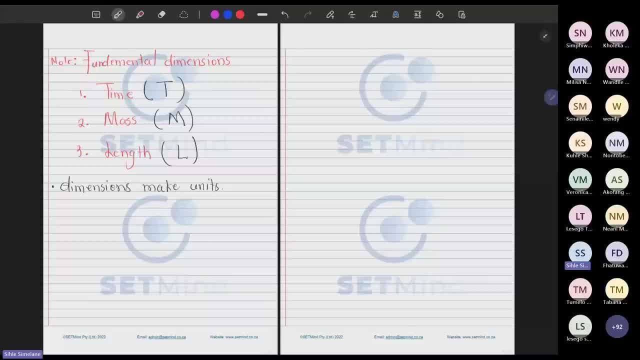 he's going to put in kg there, But where there's time, they were tempted to say he's going to put in seconds. Well, it's not the case. We are looking at dimensions, not units. S for second is a unit. 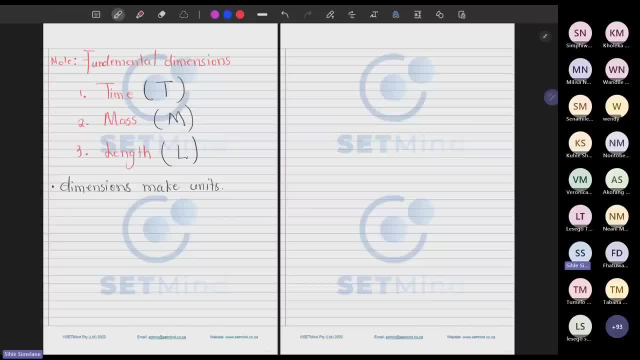 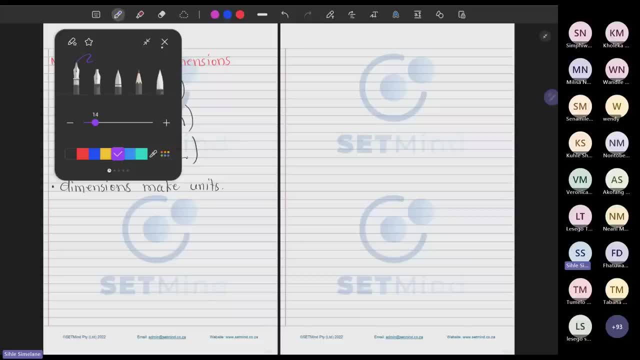 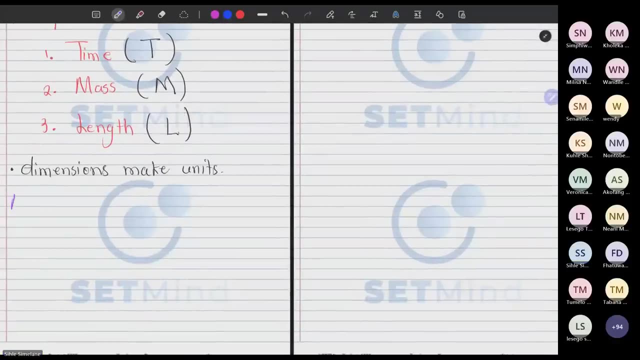 It is not a dimension. So let's consider a number of cases where we are trying to express the quantity using its fundamental dimension. So let me say here I will need some of you to cooperate, those who can unmute themselves. 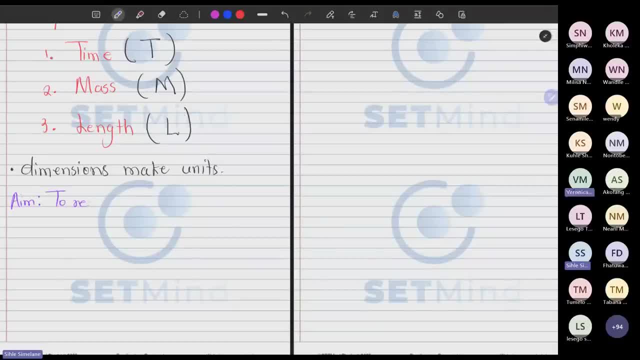 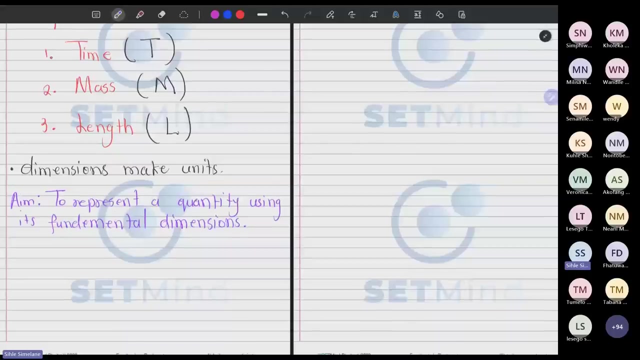 I'll say: the aim here is to represent, represent a quantity using its fundamental- sorry, fundamental- dimensions. So that's what we are going to do. We are going, we are going to represent a quantity using its fundamental. 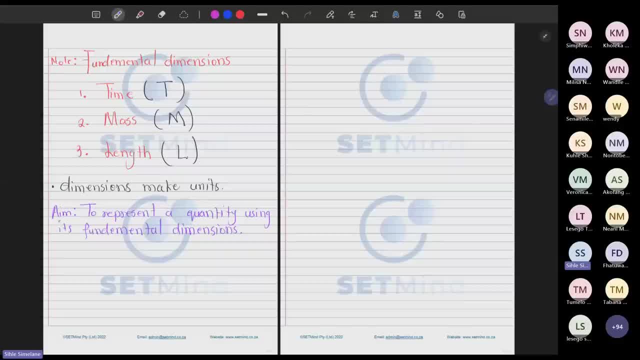 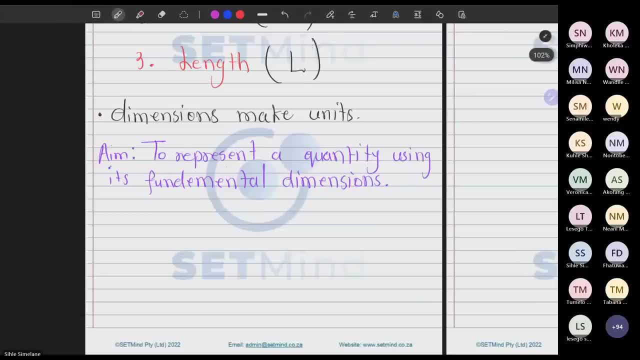 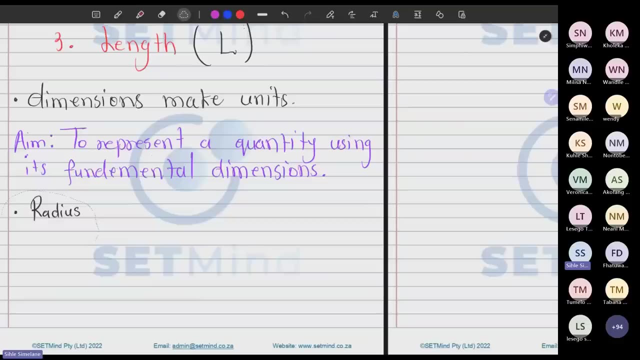 dimensions. So let's consider the easiest one, which is force, But let's consider radius. So when we look at radius, so I will say: here it's the quantity, And then here I will say dimensions. So when you look at radius, 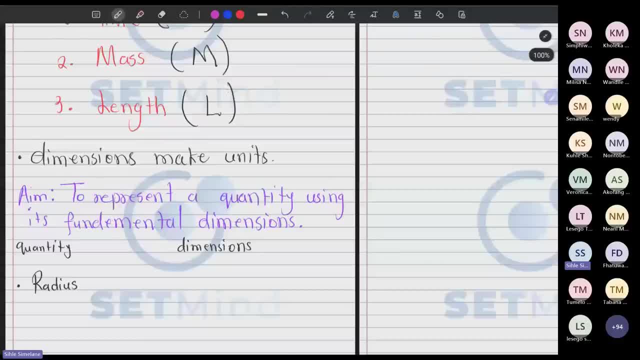 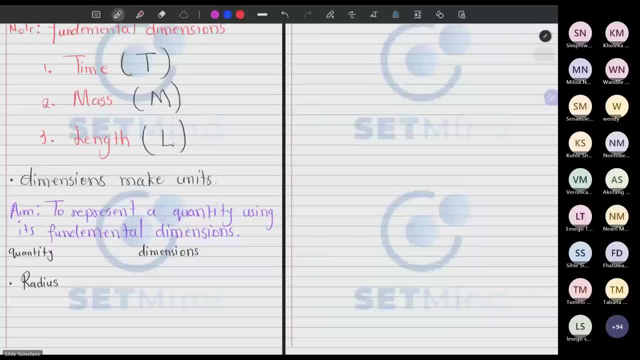 when you look at radius, what is it made of? when we look at the fundamental dimension, Length, Length. So radius, we will say length. Okay, because radius is just length. You are moving from one point to another one. 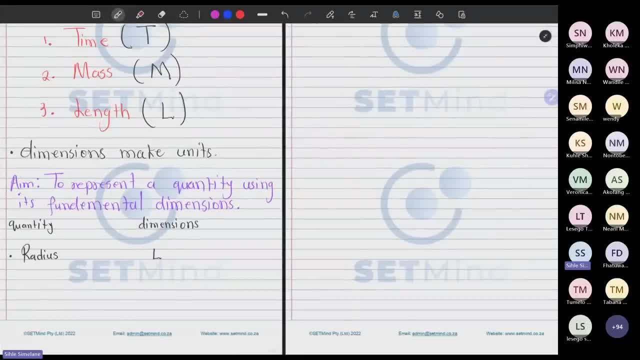 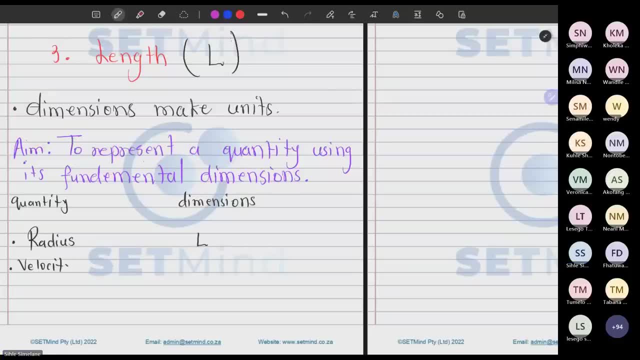 this is L, And then let's look at velocity. So I need you to think carefully here: Velocity. So velocity, we know that it is. we are looking at the units. So let me make dimension and then let me make units. 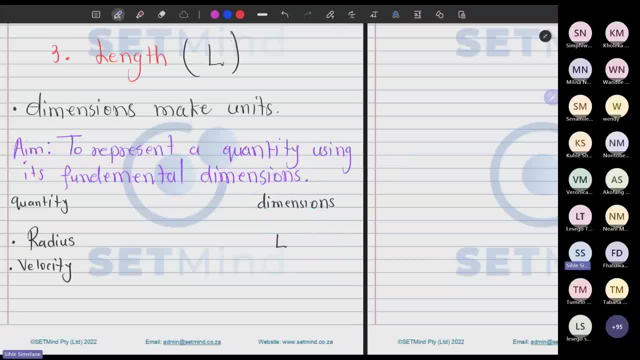 It will be easy to move from one to the other. So let's come here and say unit Or units, So radius obviously in units. it is usually in meters, It's considered a standard unit, So radius is denoted in meters. 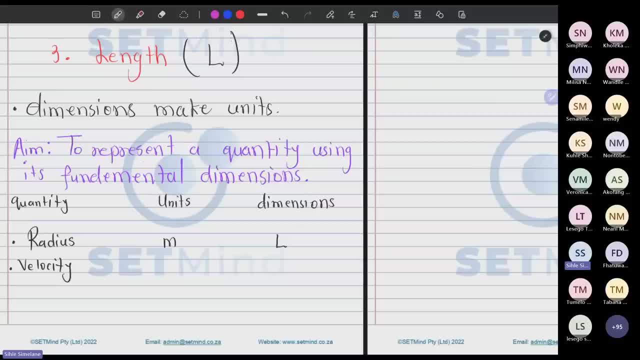 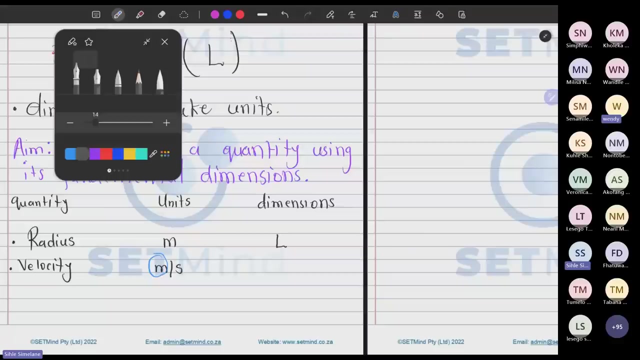 So velocity, what is? what are the units for velocity? Anyone? The unit for velocity, The second, The second, And we know that meters is length. We'll go to dimensions and say L over second. I know. 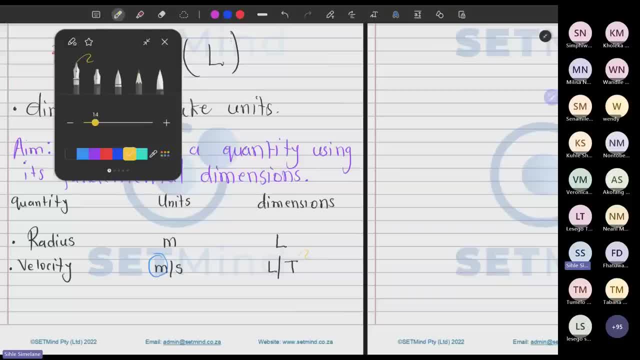 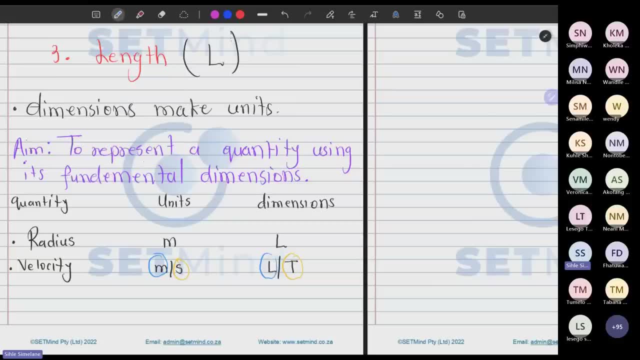 it is time. So look at what we did here. There's seconds, which is time, There's meters, which is length. So our dimension of velocity will be L over T, But we prefer to write it as L. 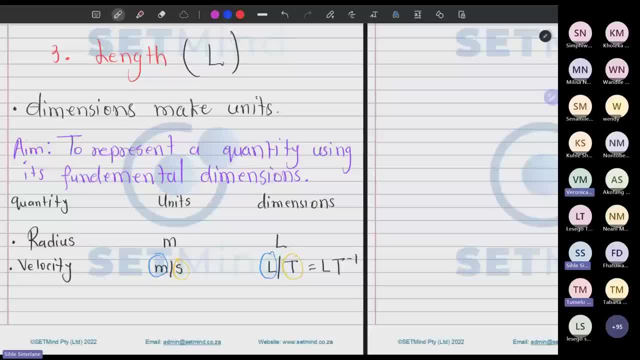 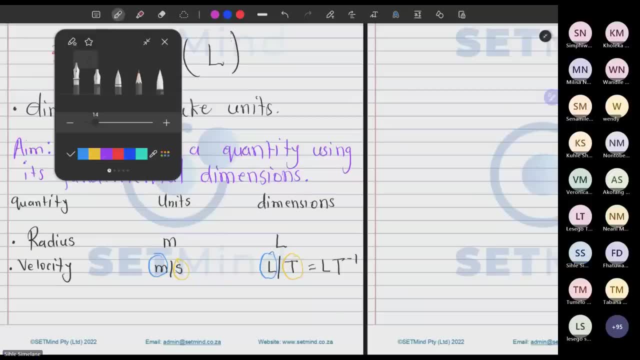 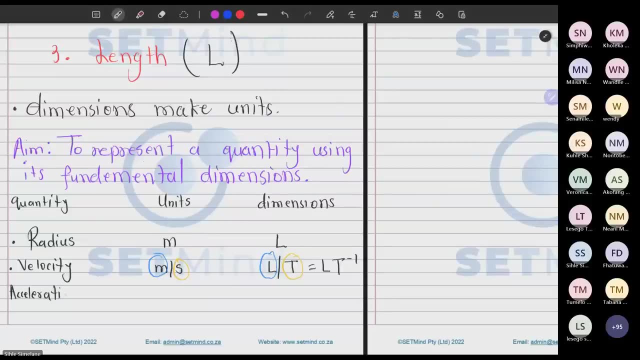 T to the minus one. T to the minus one is the same as dividing by T. Okay, Let's look at acceleration. What are the units for acceleration Meters per second squared? Anyone, This is not a tricky question. 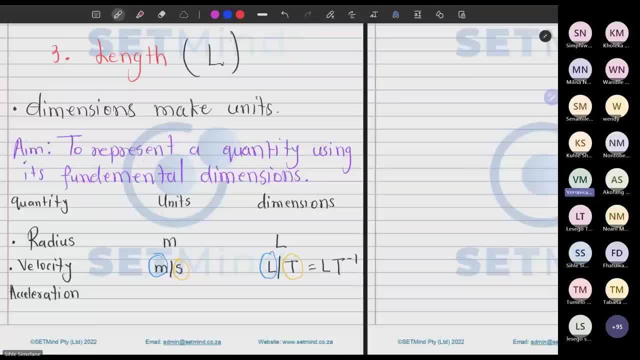 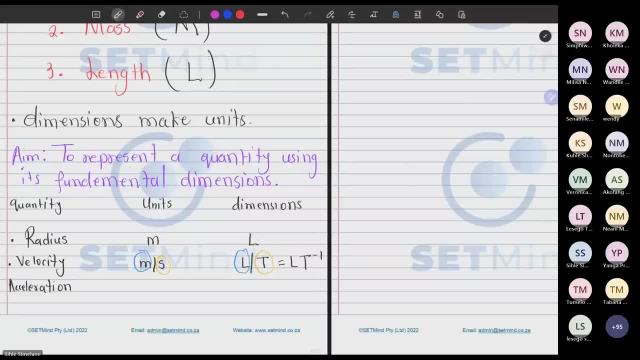 What are the units for acceleration? Give it a short. Meters per second squared. Give it a short. We will wait until someone answers. What are the units for acceleration? We should all be active. It's still in the morning. What are the units for acceleration? 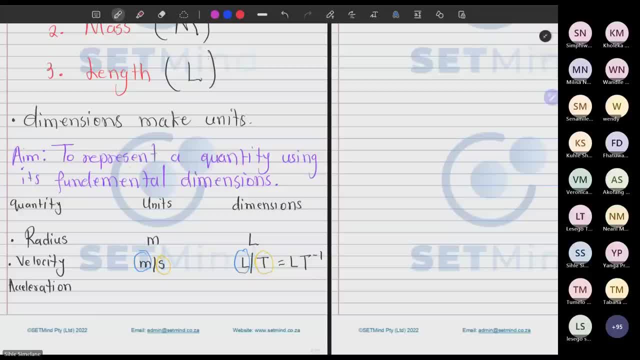 Meters per second squared. Thank you, The units for acceleration. it is meters per second squared. So when we go to our dimensions, we look here Meters. Well, it sounds like we are speaking of length, So I'm going to have L divided by. 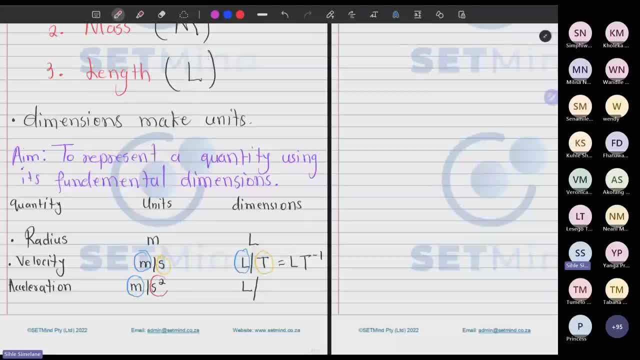 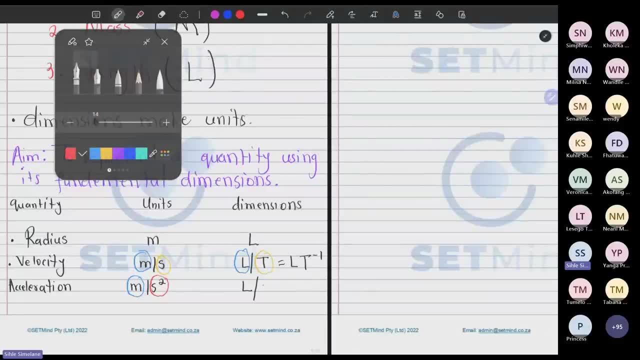 we have seconds. Seconds sounds like we're speaking of time, but we are squaring the time. So I'm going to go there and say: divided by T, squared. There you go. That's the second part. And then we dislike having things dividing. 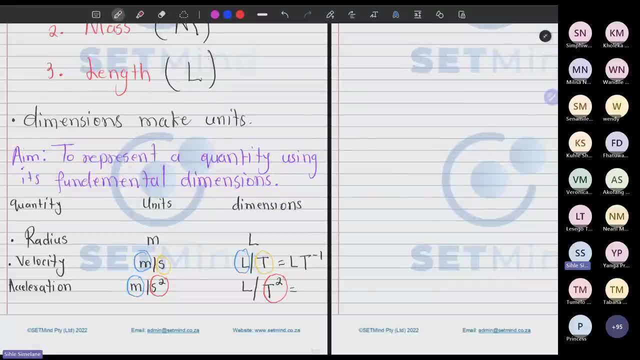 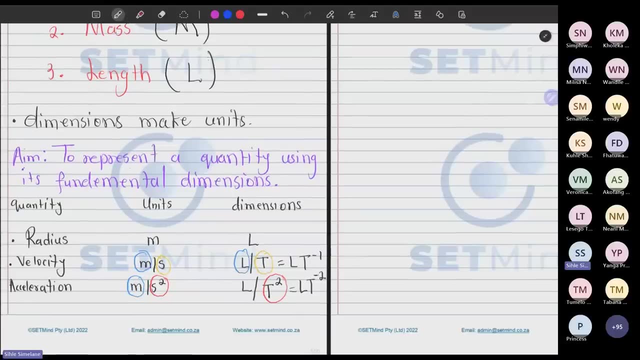 So we resort to using exponents, So we'll have L T minus two. This is still the same, Just that I took the T. raise it to the power of negative two to have a product instead of things dividing one another. Okay. 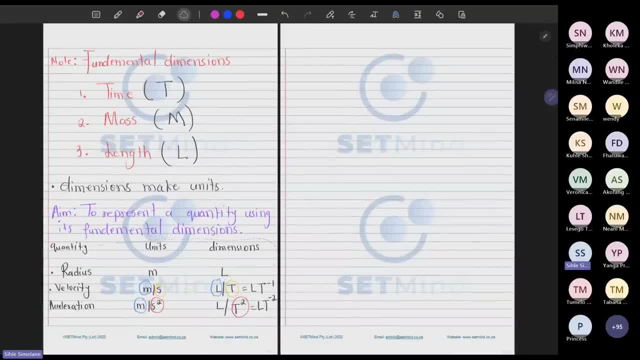 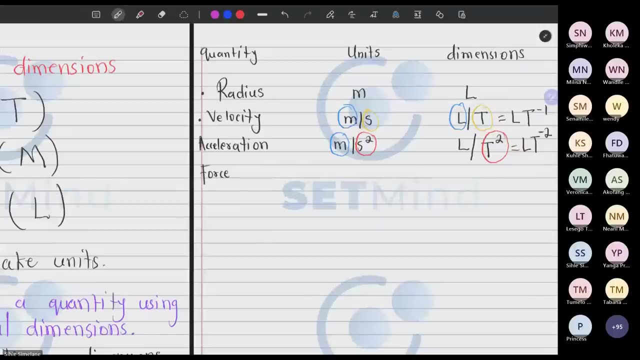 Let's take our table to the next page and continue To expand in these fundamental dimensions. So let's take force Force. What are the units for force? Anyone? Kilograms times, meter per second squared. Okay, So force is Newtons. 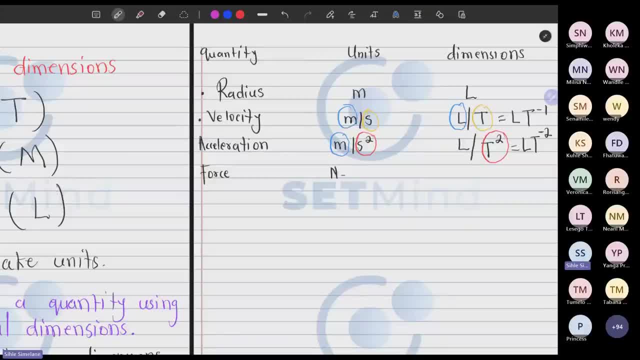 And Newtons. we know force is MA, So which means we have kilograms, We have kilograms. Let me write the kg Because what I need you to remember here, let me come here and say: remember that force for F net, the force acting on a body, is just MA. 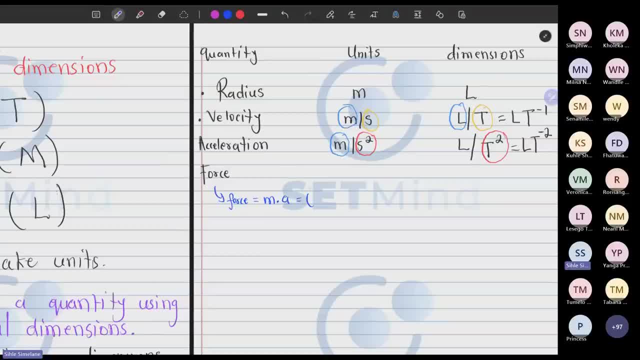 And M. we know that it is given by kgs. That's the M, which is mass, And then the acceleration. we know it is given by meters per second squared. Okay, So the units for force are: is kg? meters per second squared. 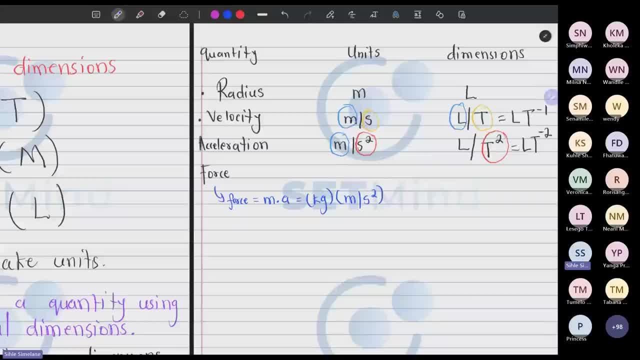 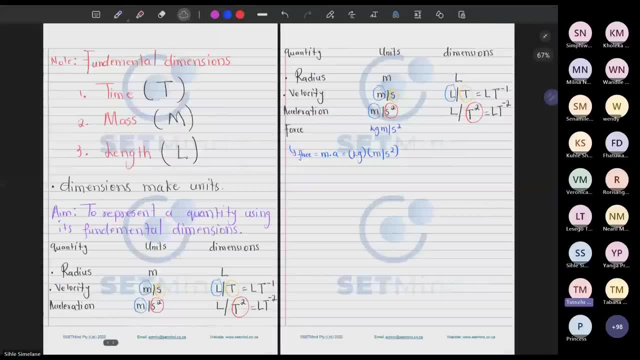 Okay, And then let's see how then do we take those to the fundamental dimensions? So let's go. I can see kg here. kg, it is not confusing, It is mass. So I go there and say I have. 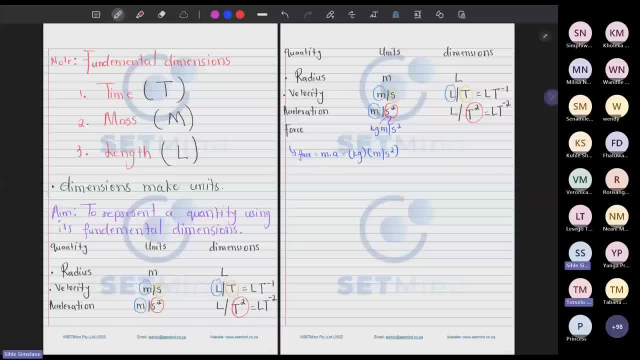 let's pull it down. I go there and I say I am going to have mass. It's highlighted in purple but deals with the kg part, Because mass, we said, we are always going to denote as M When we do dimensional analysis. 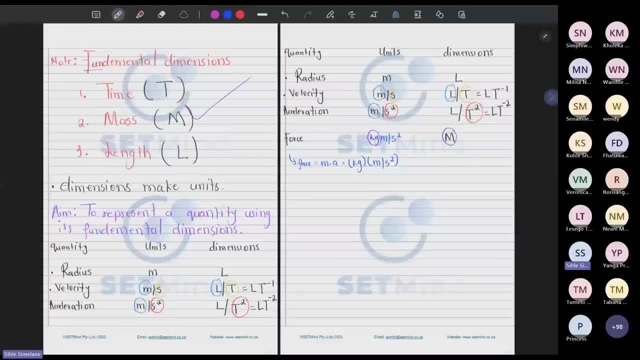 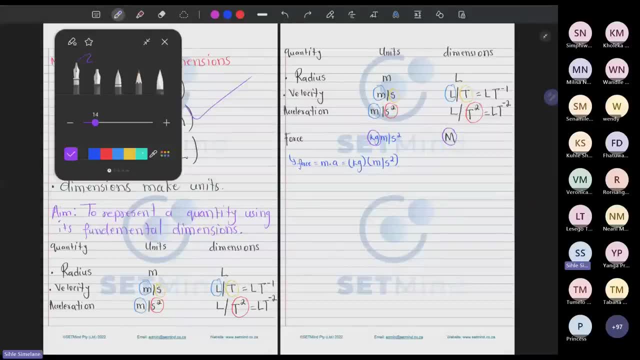 we are not going to have kgs. We are trying to go to fundamental dimensions for us to be able to solve a problem. And then let's go and look at M. There's our M, there M is meters. And what is meters? 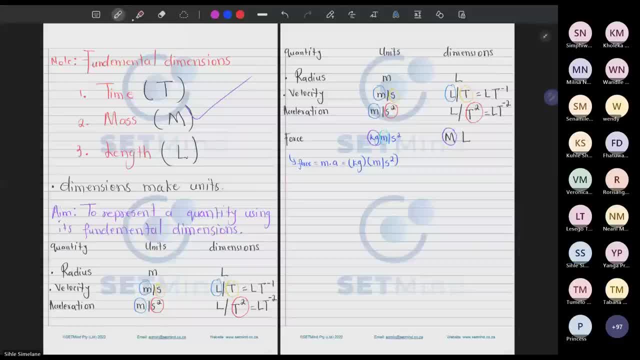 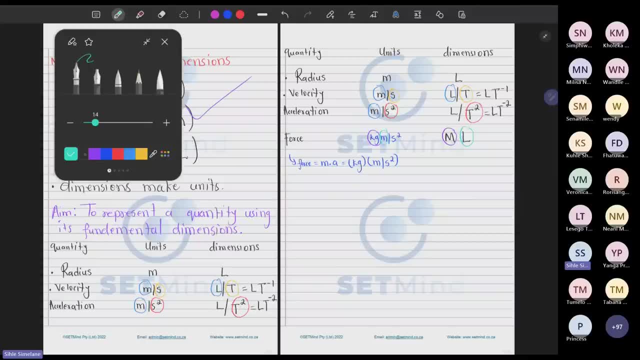 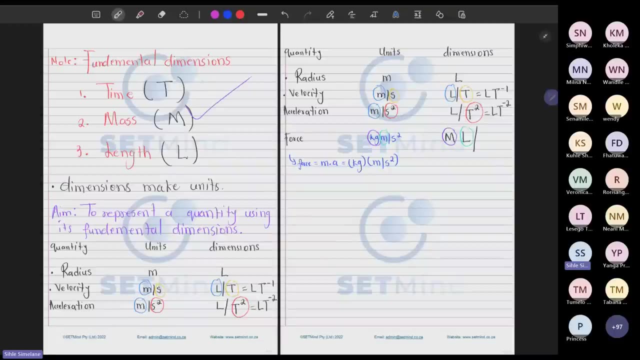 Meters sounds like length to me, So let's highlight that also. Then we have divided by S. squared S is for second. That sounds like time to me, So I'm going to have time squared, Okay, And then remember I said we really do not like having divisions. 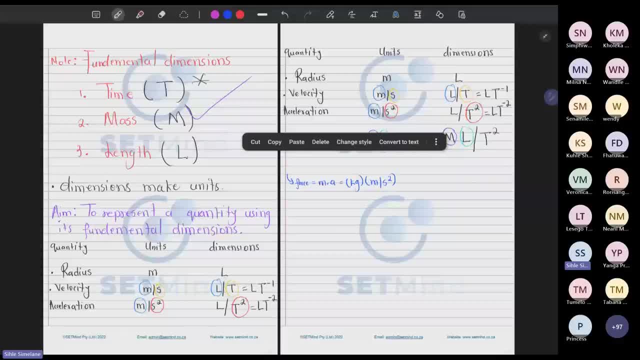 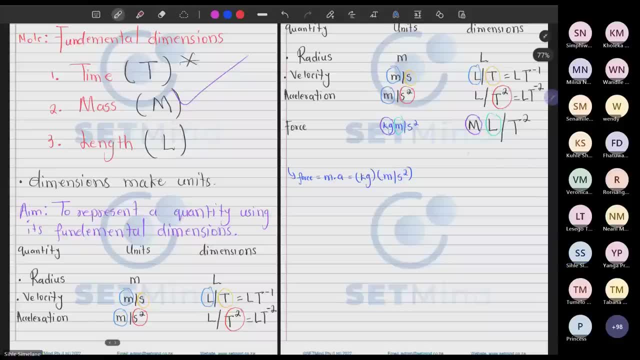 So we'll resort to having a product. If it means we should have negative exponents, that is total. So it means my force will simply have M, Force will simply have M L, T minus two. That's my fundamental dimension of force. 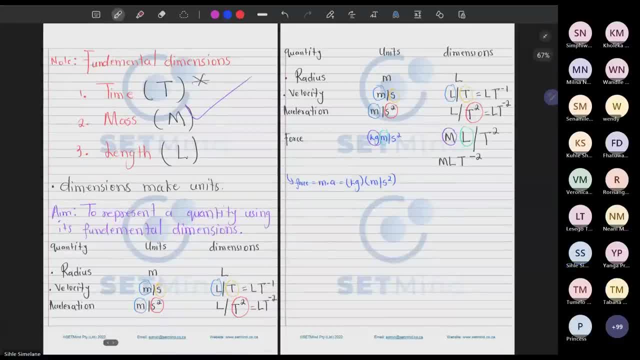 Okay, Let's look at torque Torque. Anyone who remembers the units for torque Torque is force, times, distance or displacement. So if you think of it, it is just force which is the Newton times displacement. But already force was. 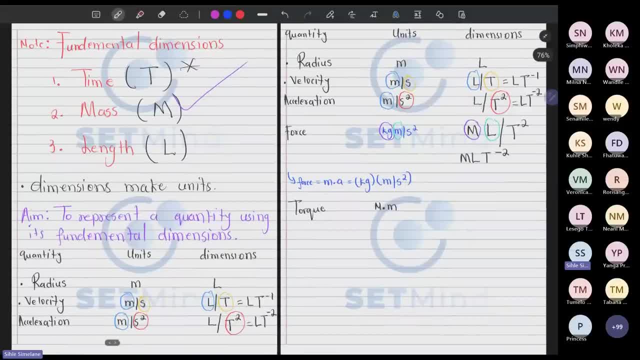 let's come here and let me write it down just below and say: remember that your torque is just force and then multiplied by displacement. And remember that if you look at above, our force is mass times acceleration, So it is kg times acceleration. 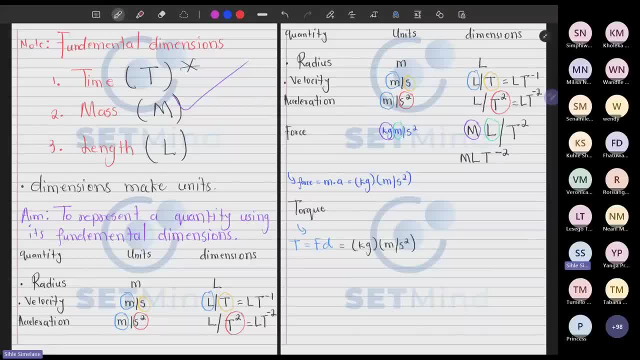 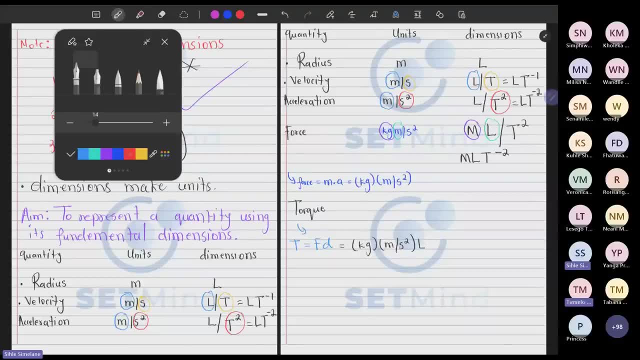 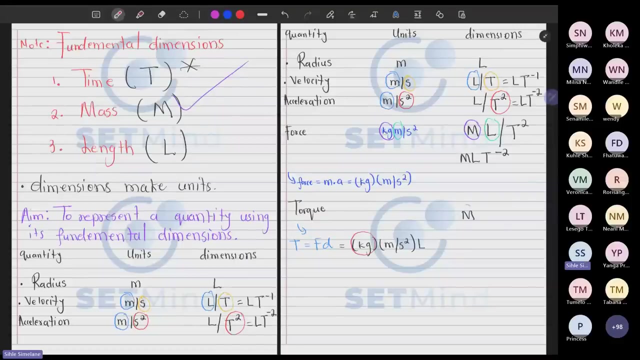 which is meters per second squared times D. D sounds like me length. Okay, So this means my fundamental dimensions for torque will be: I have mass from that. kg is mass. And then let me go further. I have M And the M there is for meters. 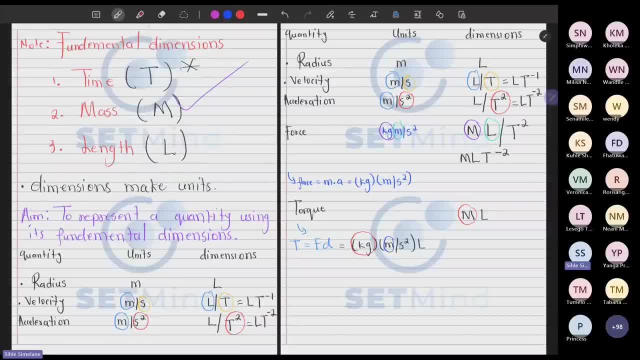 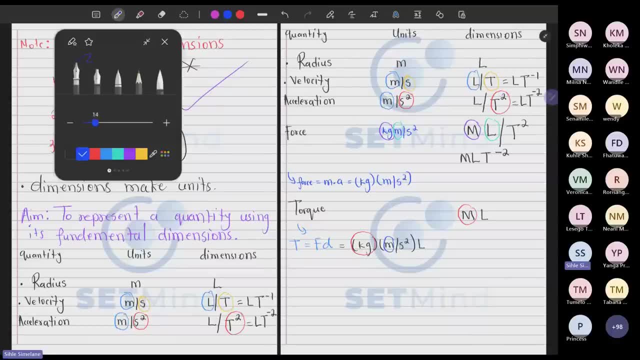 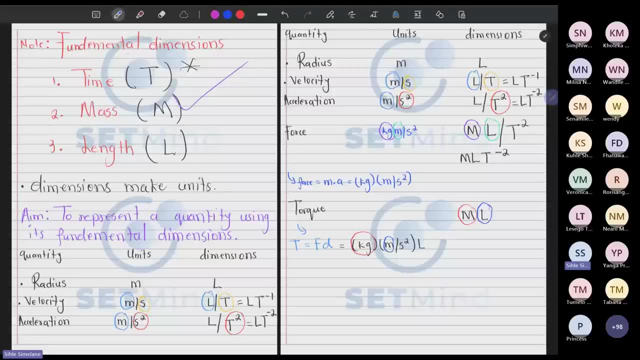 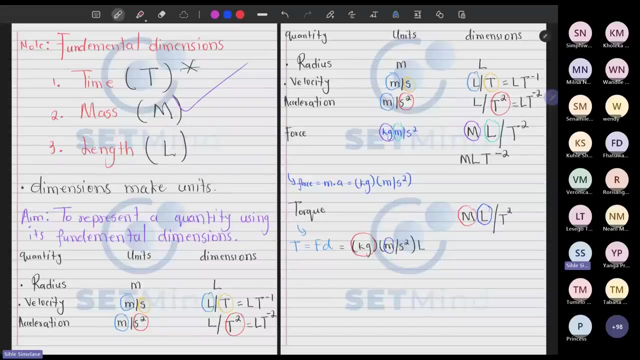 Meters sounds like length to me. Okay, Highlight that also. Meters is length. And then we have divided by S squared. We know that S is time, So let's divide by T squared. And then we are multiplying by the displacement. 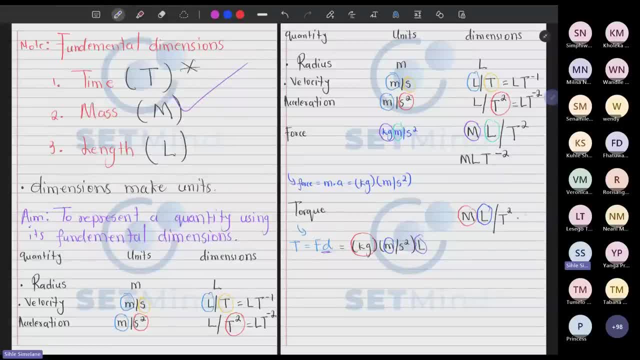 which is just length. So I'm just going to multiply by length also. So when you look at our final answer, it is going to be: we are going to have M, And then the L's will multiply, giving us L squared. 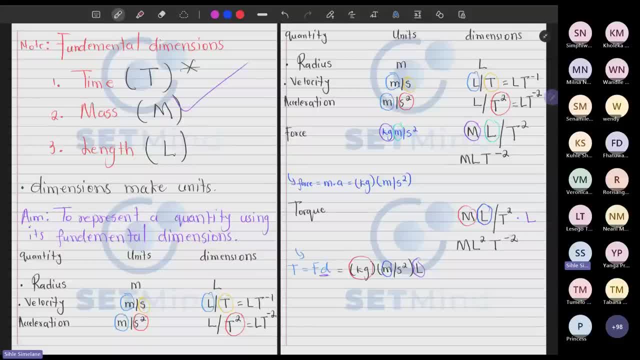 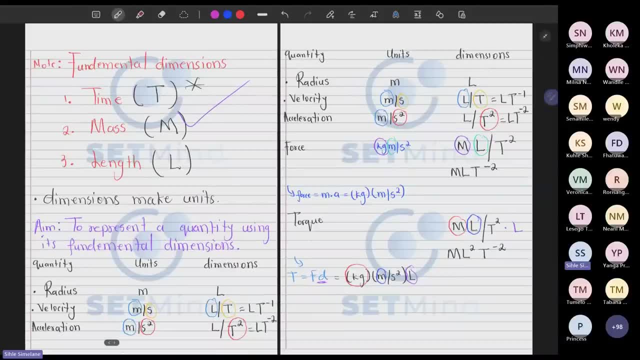 And then the T will be, will push it up, give us minus two. So these would be the fundamental dimensions for dimension four, torque. Okay, Let's do pressure and then torque and think about where are we headed exactly, because we need to have direction. 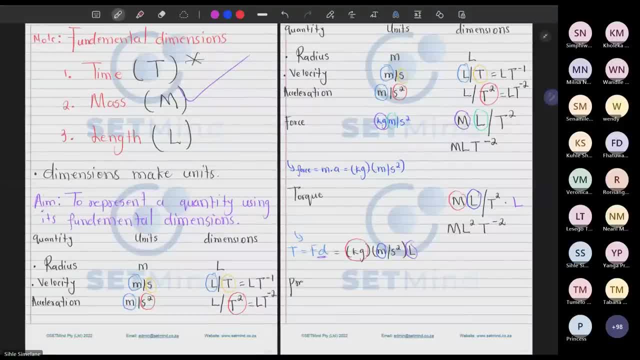 So let's look at pressure. Okay, So anyone who knows the fundamental or the units for pressure, or maybe you just know the formula, how of pressure, how it relates to force and something Someone else, please tell us how we can then find the dimensions. 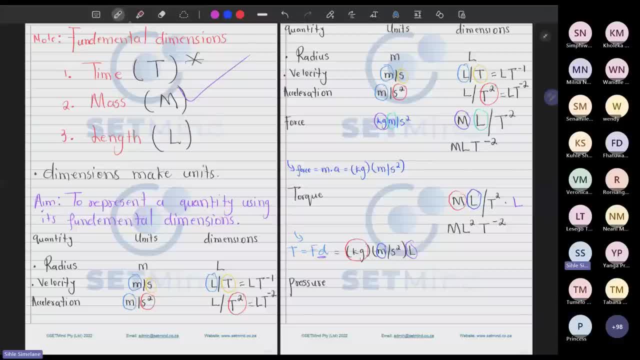 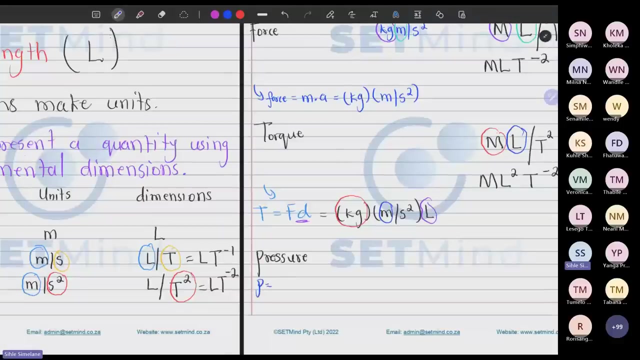 for pressure. What is pressure equal to? Pressure equals to four: force over area. Force over The area. Okay, No problem. So let's write your formula down so that we can be able to derive the dimensions. So pressure equals force over area. 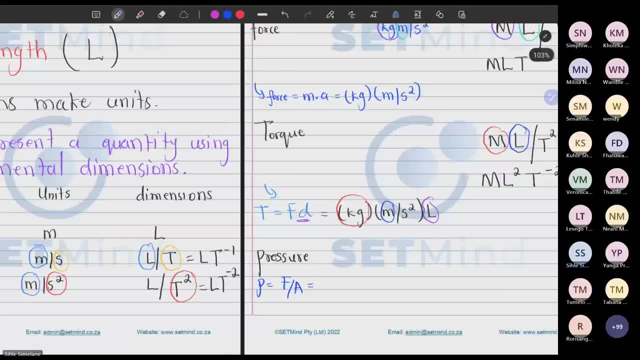 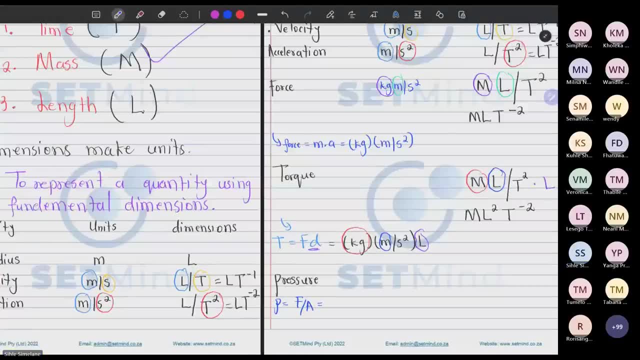 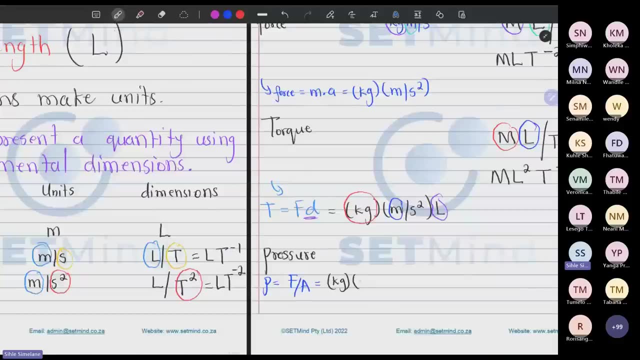 So of course, we have already to choose that the fundamental dimensions are: or let me just write force. Force is just kg, which is mass times. acceleration Acceleration will be meters per second squared Area. if you remember, it is just meters squared. 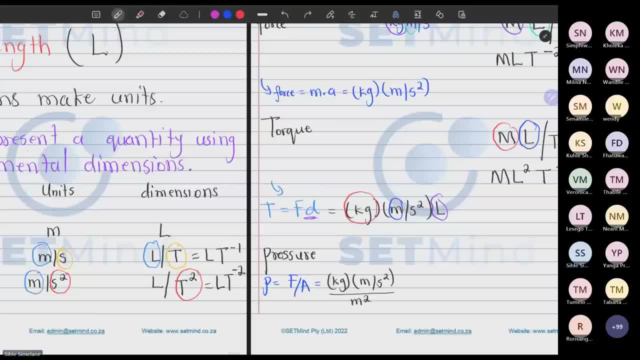 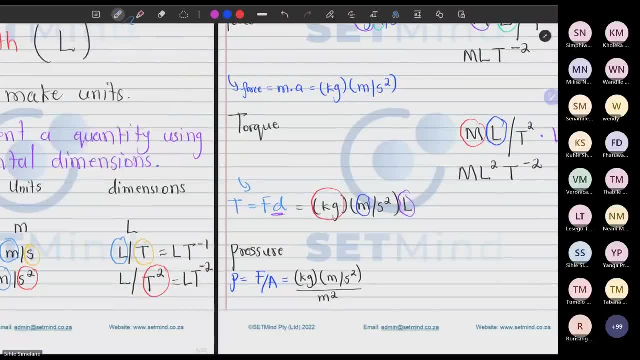 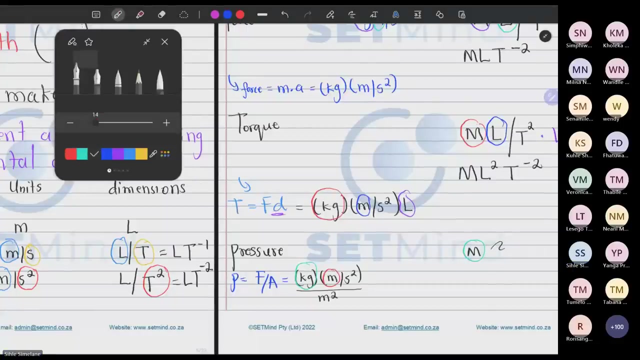 Area. the fundamental units are meters squared. So when you look carefully, when we now go to the dimension, we will have the kg, which is mass, Okay, And then the m, which is here is length, Nothing confusing- And then the s. 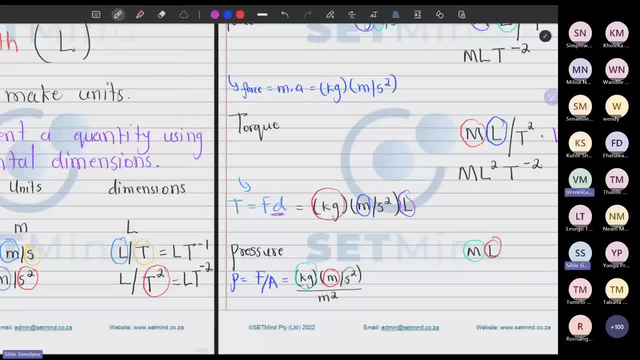 which is here is a second, So that means it's time. So I'm going to divide by time. but it is squared, So I'm going to square it, Then divide it by below. I have area which is meters squared. 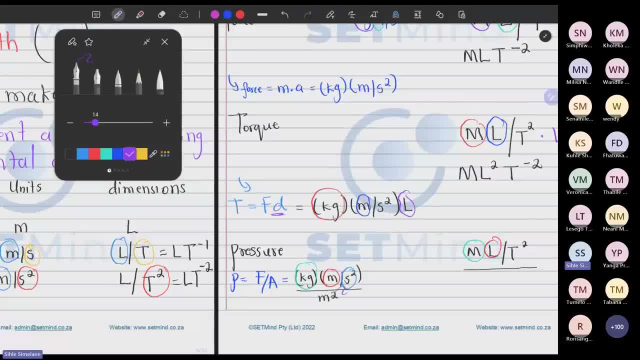 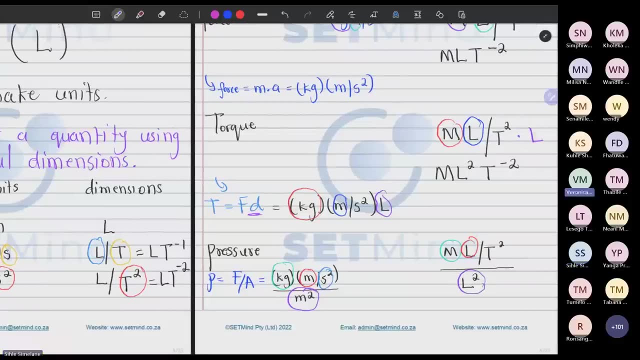 And meters squared. I know it is just length, So that means what I have is simply length squared, Okay, So we just highlight that And there you go, We have length squared. So this, obviously, we can try to write in a more simplified form. 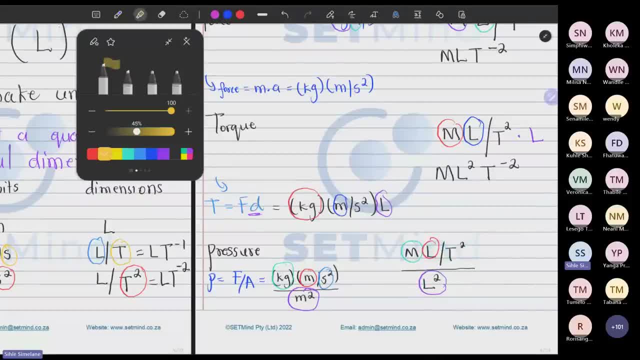 by simply canceling the l's, one of the l's and the other one there, and then putting the t up there. So when we simplify this, the answer which we obtain is simply m. Then one l will be left in the denominator. 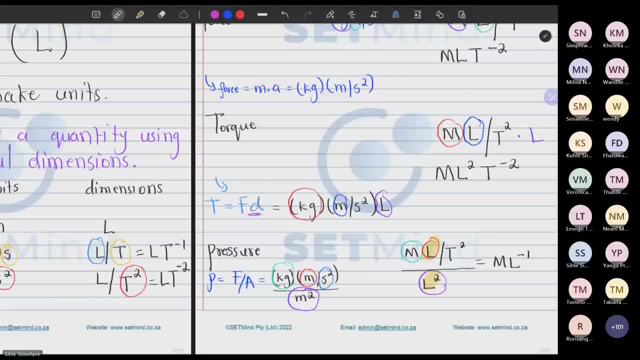 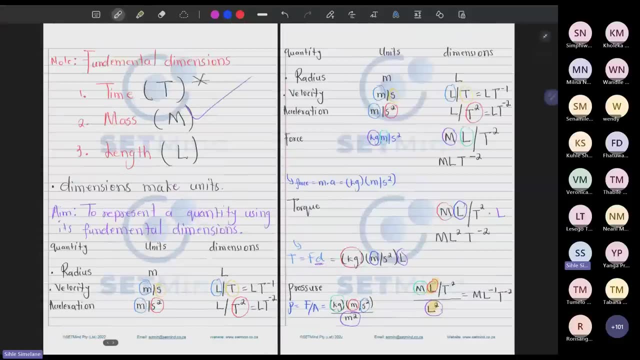 but we'll put it up and say minus one And then the t squared in the denominator. we push it up and then we put minus t. This would be the fundamental dimension, Dimension or present. So your focus on the course is on these. 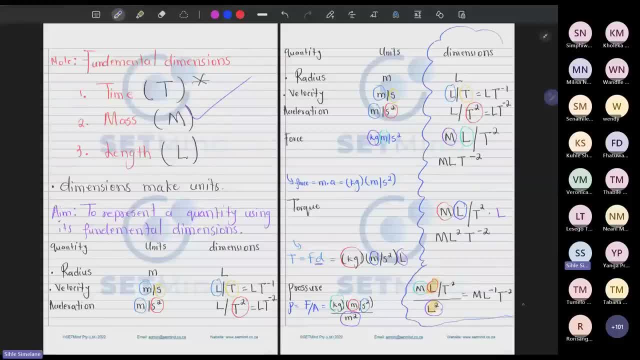 these ones here, What is going on this side? So, meaning, when you do dimensional analysis, the first thing you should do, they tell you your force, your area and whatnot. Take what you are given, write it in terms of its fundamental dimension. 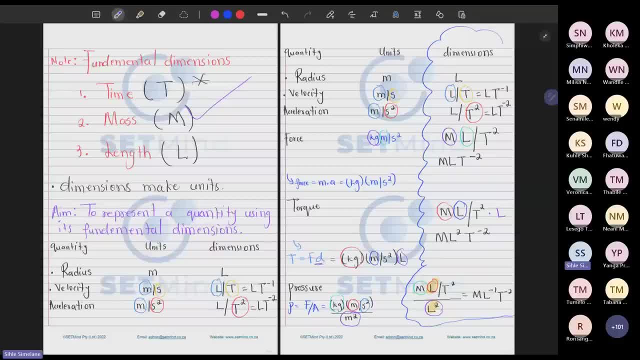 Okay, That should be what you do. Let's erase this for need purposes. Go to the next page and see exactly where are we headed with what we are doing here. So, as much as we have quantities which have dimension, we have what we call dimensionless quantities. 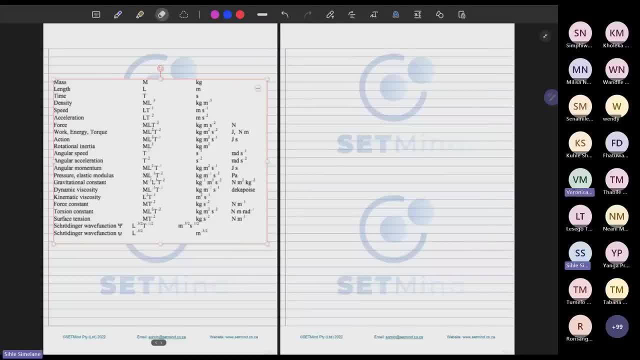 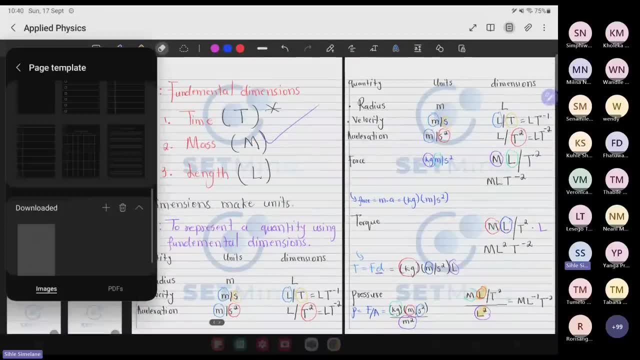 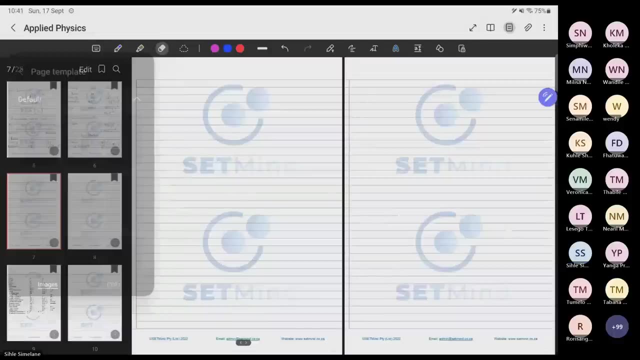 Okay, Let's go to the next page. This page here you will see later. That's just what we need to know on top of your head. If you do not, you will need to do the deriving yourself, but you should not worry. 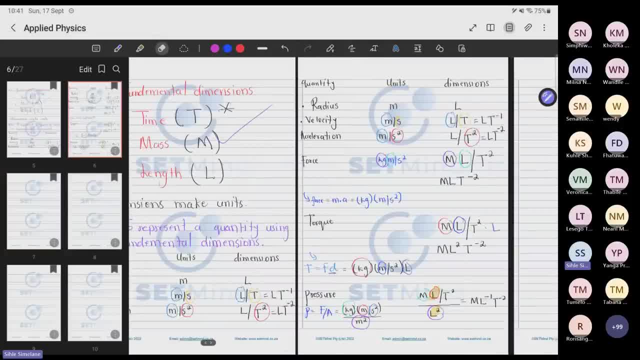 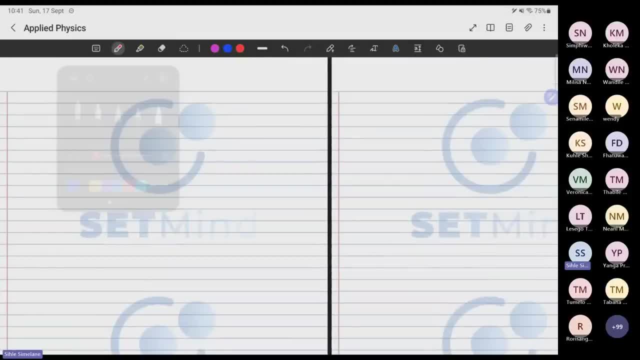 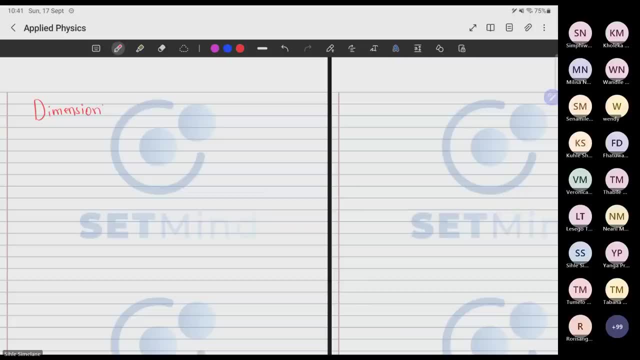 It is really easy. Okay, Let's come here and say to you: I'm saying we have what we refer to as a dimensionless quantity, And the question you might start asking yourself is: what does this mean, really, Dimensionless quantity? What it means is that we have a quantity. 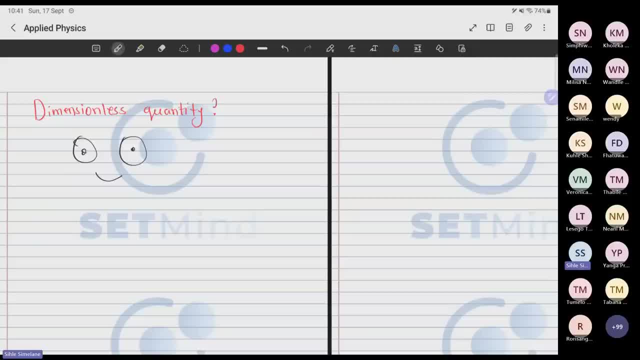 which doesn't have length, it doesn't have mass and it does not have time. Okay, So what it means in human language is quantity that does not have, does not have time, it does not have mass and it does not have length. 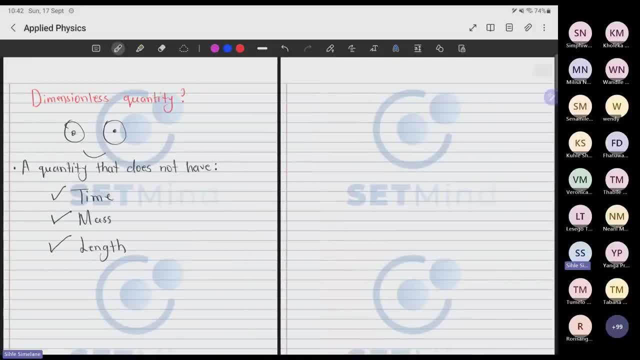 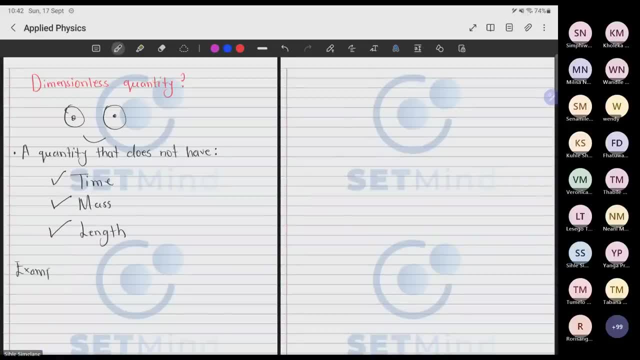 Okay, That's what we mean. So an example would be: if I come to you and I say pi I'm not saying pi radian, I'm not saying pi anything. I just say to you pi Your brain should fire up and say: okay. 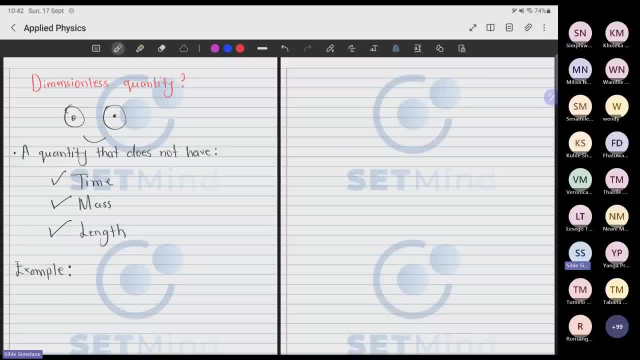 Well, he's saying just pi, So it's dimensionless, Unless he says radians, then you can easily lead or link radians to time. It's easy. So if I come to someone and say just pi, the question is, what are the dimensions? 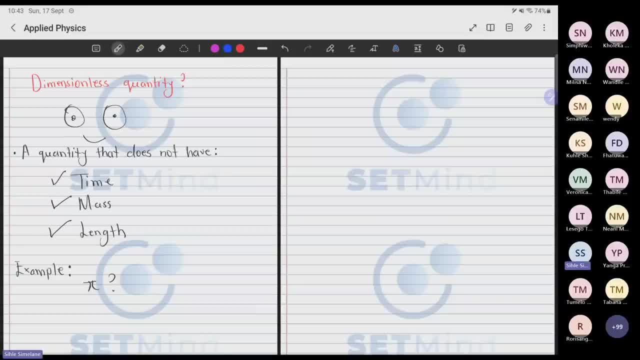 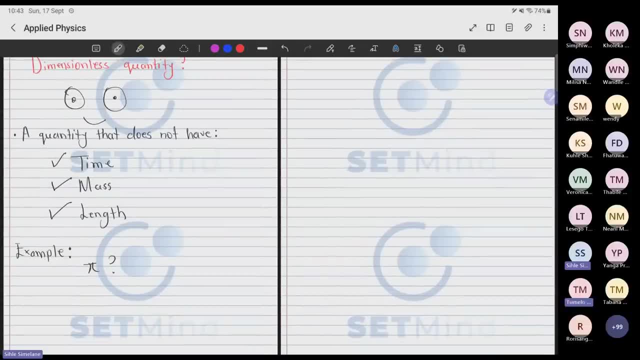 What are you speaking about when you say pi? So think of the importance of having dimensions and units. If we live in a world where units do not matter and dimensions do not matter, it would be really interesting. So imagine someone coming to you and they are saying: 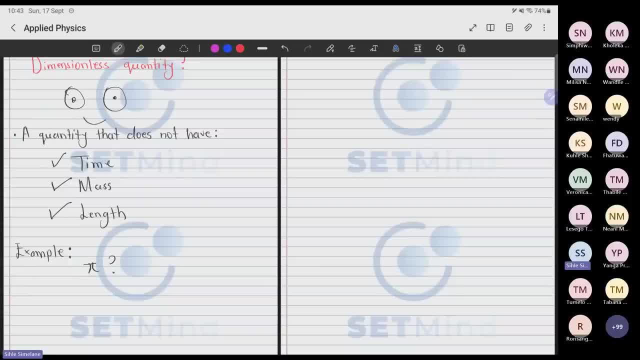 I want to give you a million And when you think of them, obviously I think many of you are wired to think that it's probably money, But the units, they matter, because you are giving me a million. what Are you giving me a million? one rands. 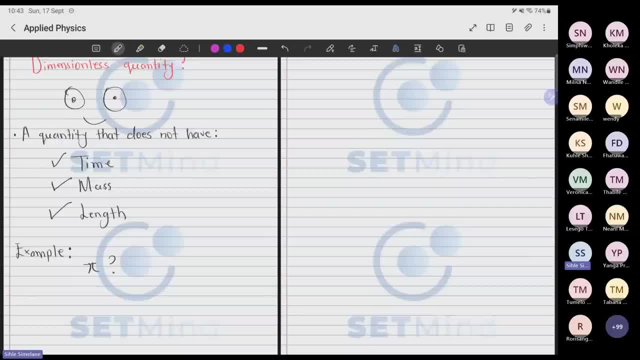 Are you giving me a million two rands? Are you giving me a million dollars? Are you giving me a million square meters of land? Are you giving me a million Zim dollar? Are you giving me a million Bula? It really matters. 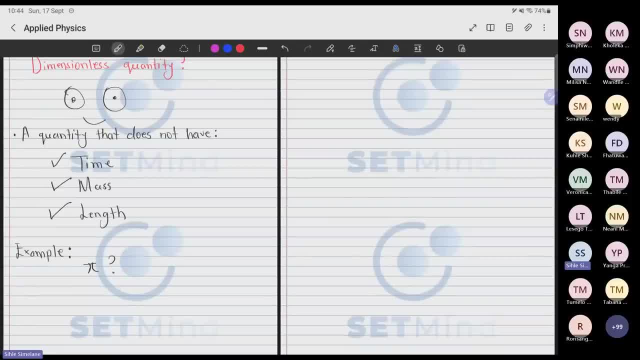 what the units are. So it is for this reason that you need to also understand that, as much as units matter, there are quantities which are dimensionless, And when a quantity is dimensionless, what that means is that it does not have time. 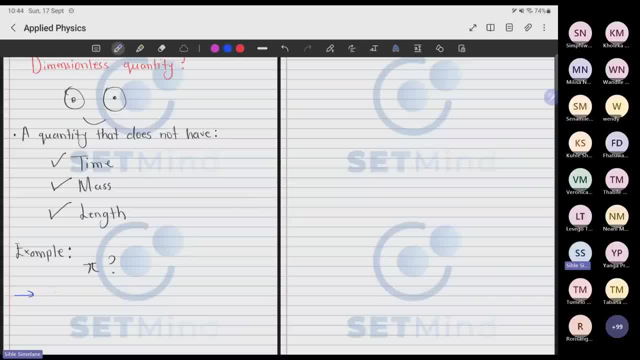 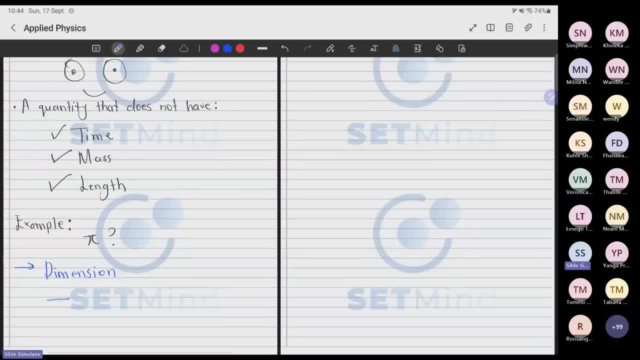 it does not have mass, it does not have length. It means, when we look at its dimension, the T is to the zero, the L is to the zero and the M is to the zero, Because when these are to the zero, 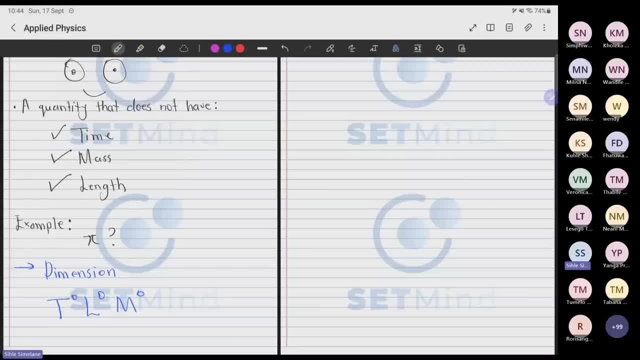 then it means we have no time, we have no length, we have no mass. This is what would be called dimensionless. When something is dimensionless, it means the T is to the zero, the L is to the zero and the M is to the zero. 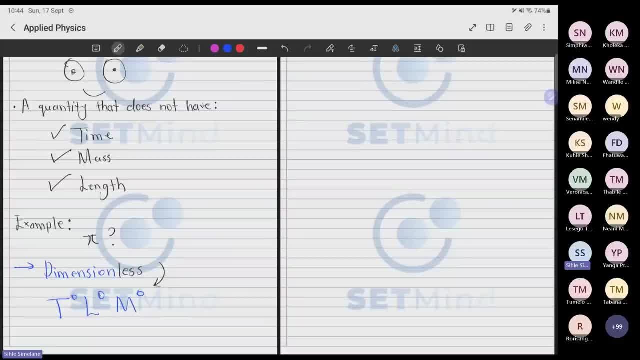 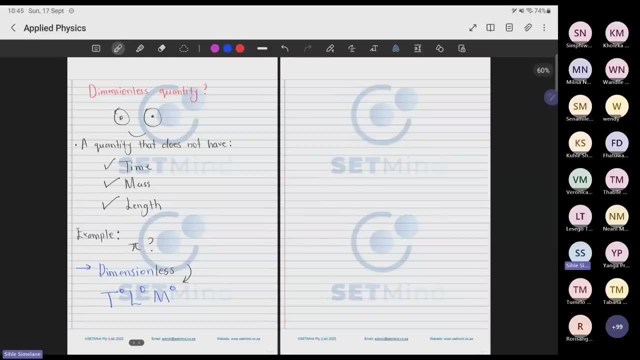 Once one of them is not to the power of zero, meaning it is present- the quantity will not be dimensionless. Okay, So that's what you need to note. And why is all of this useful, Why does it even matter? And the reason it matters. 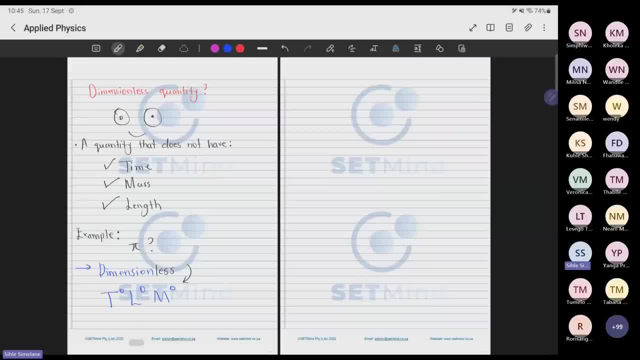 is because we are going to relate quantities such that they are dimensionless, And after we've related them, then we can be able to find relationships between two quantities. Okay, Let's think of an example. Give me a second. So let's say we have 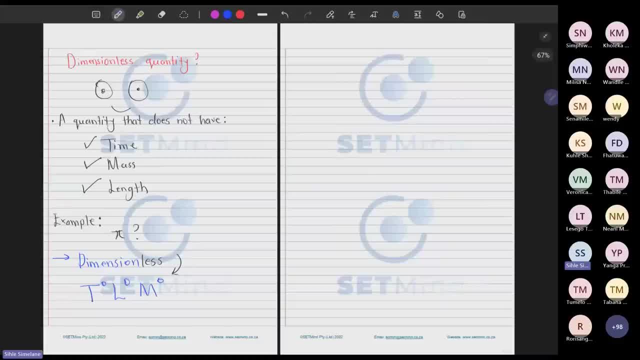 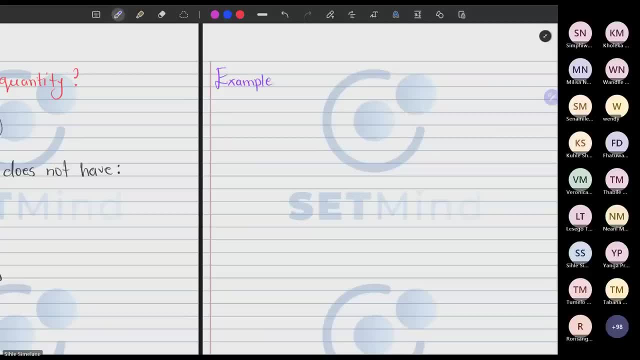 I'll call it example one. I need you to hold on tight for me here, So let's call this example one. Okay, For example one I'm going to consider, let me see radius, the length. Okay, Let's consider example one. 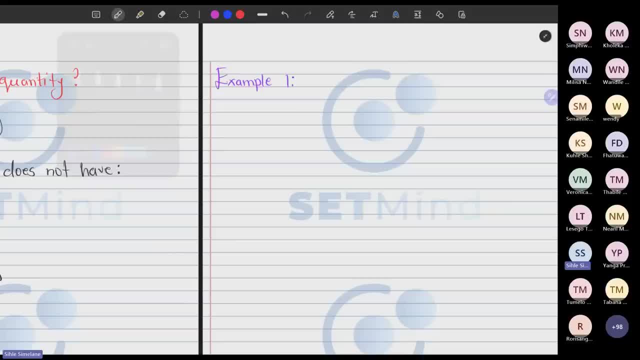 I'll give you a scenario And then we'll go to the example which is more likely to be the first part. Okay, So let's say we consider, let me take my pipe. I'll make a hypothetical example so that we get the point across. 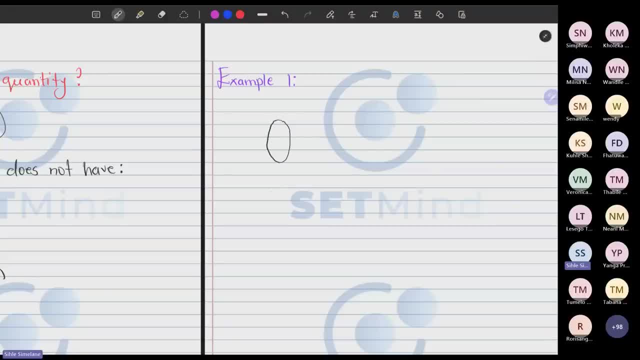 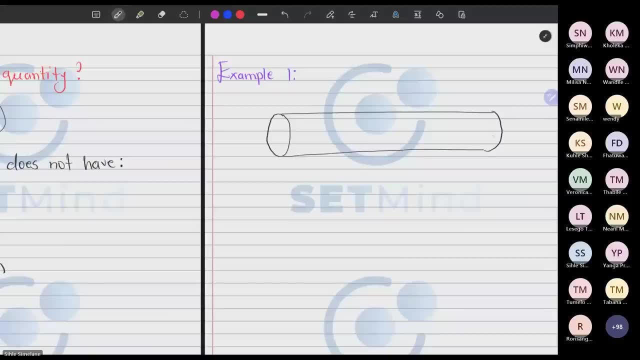 So let's take my pipe I drew earlier, And then in this pipe of mine we are transporting, maybe, fuel. The fuel is moving from Chobik south to the north. This pipe is, if you've seen them, there are pipes which transport fuel. 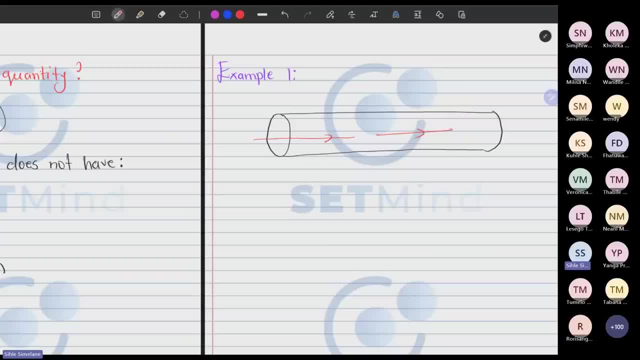 Some of them. they transport oil. You see a big pipe near the road. Well, it serves that purpose. So let's say the pipe is transporting whatever it is transporting And what it is transporting. the fuel is obviously moving at a certain velocity. 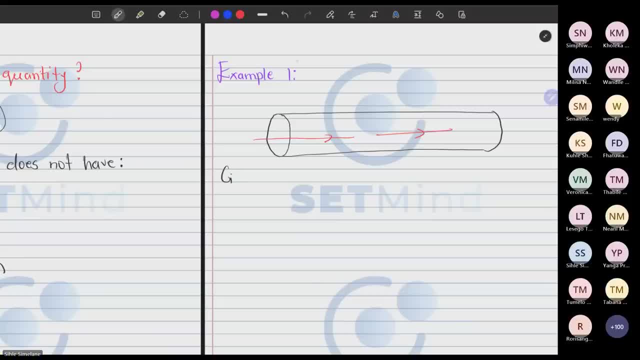 So let's say we are given. we are given the parameters of interest. And they say: one of the parameters of interest when you look at this pipe is the velocity, The velocity at which the fuel is moving. So velocity is obviously V. 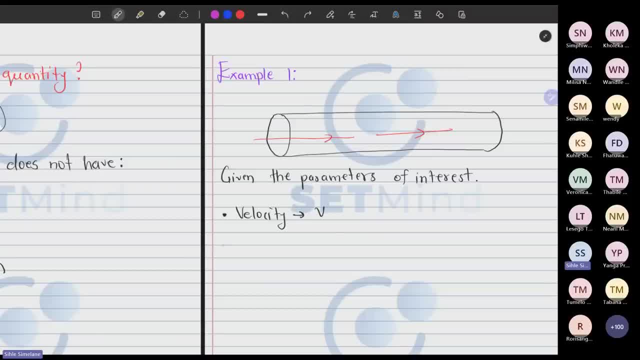 Okay. And then they say we are also interested in the pressure, And pressure will just be noted as that. And then they also say we are interested in the radius. Let's use the diameter, The pipe, which is just V for diameter. 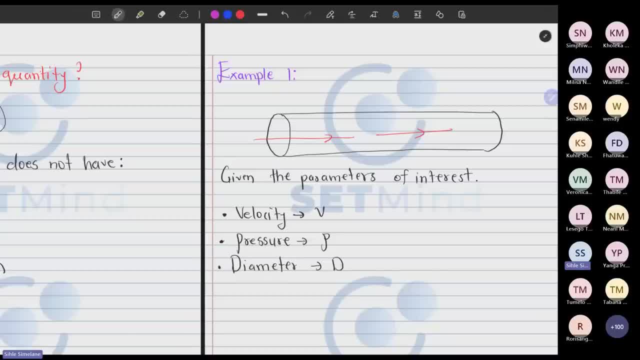 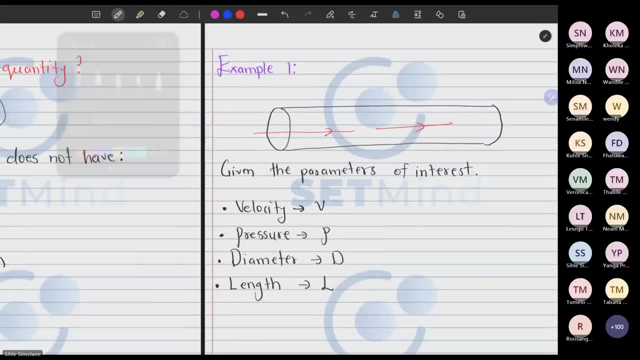 And then let's look at one last quantity, which is going to be, let's say, the length, The length of the pipe which I'm just going to denote as L. So these are the parameters of interest. And then they say here: 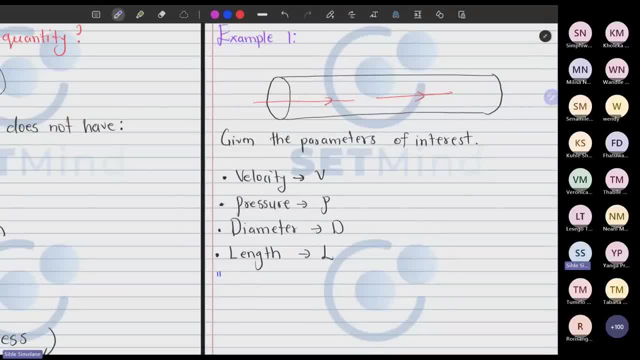 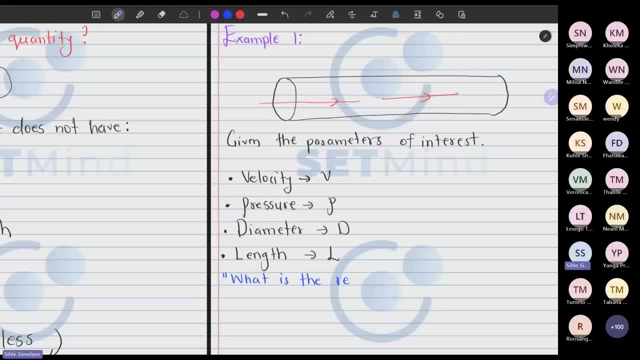 let's pose the question I posed earlier. Then they say: what is the relationship? Or let's say: how is- let's put it that way- How is velocity related to pressure? That's the question they're asking. We want to design this pipe. 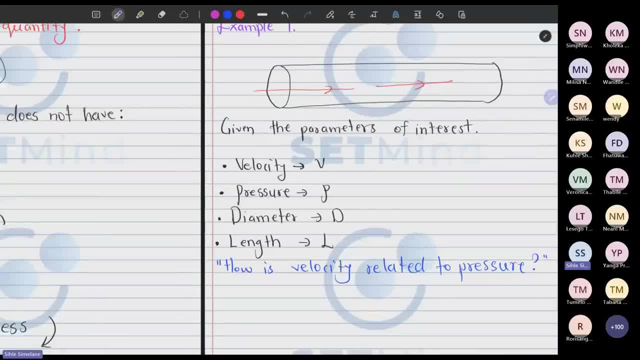 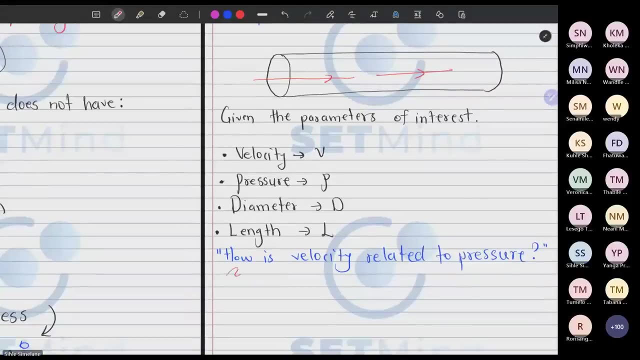 and we want to modify. we increase the velocity. What should we decrease or what should we increase for us to achieve that? So there's what we call a dimensionless product, which is where you should start. Okay, Step one, Step one. 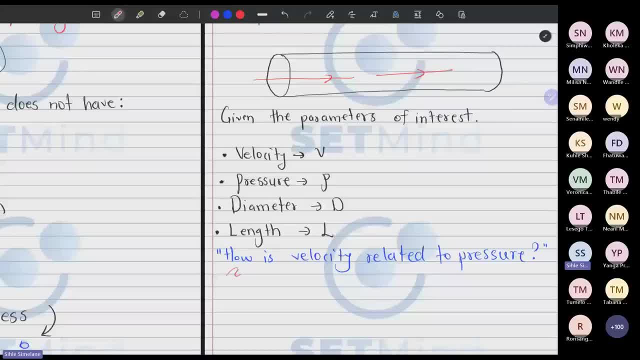 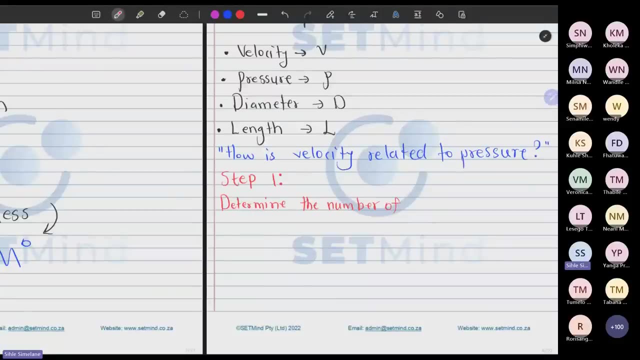 Or let me, for. step one says you need to determine the number of groups which you can make. So step one, let me say: determine- this will make sense shortly- The number of groups you should make. And this leads us to what they call. 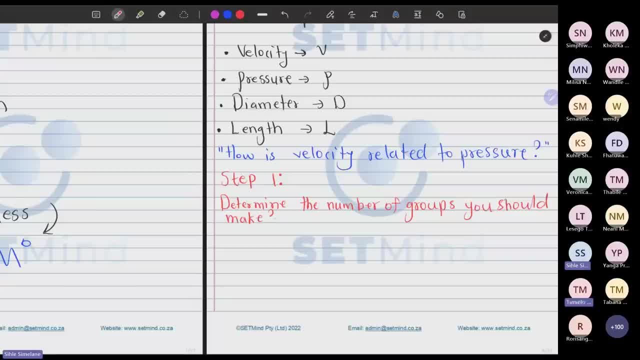 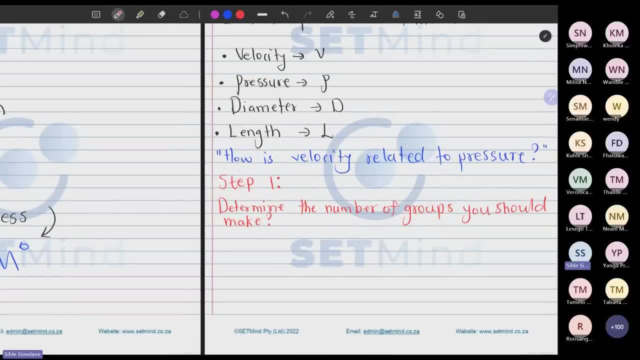 the Beckingham theorem, But when I was looking at last year's material, they didn't do it as much. So what we mean by the number of groups is that you can do various combinations and get different groups, So meaning you can have a combination. 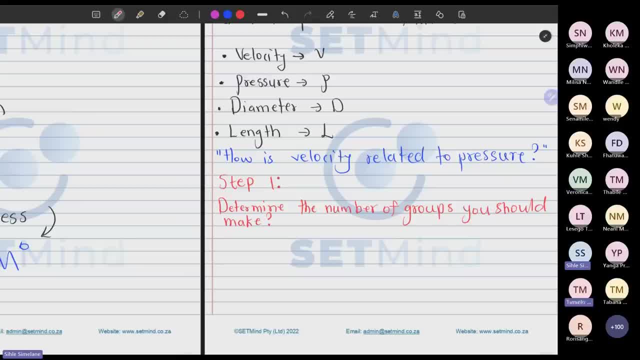 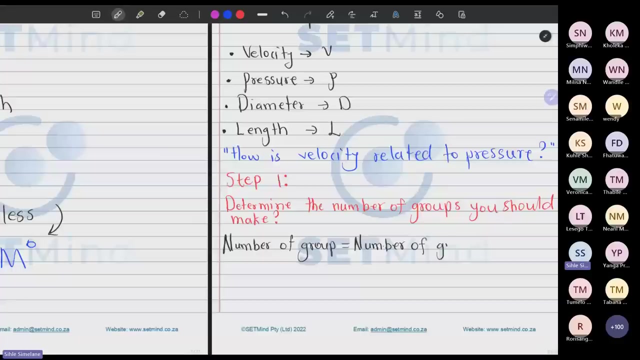 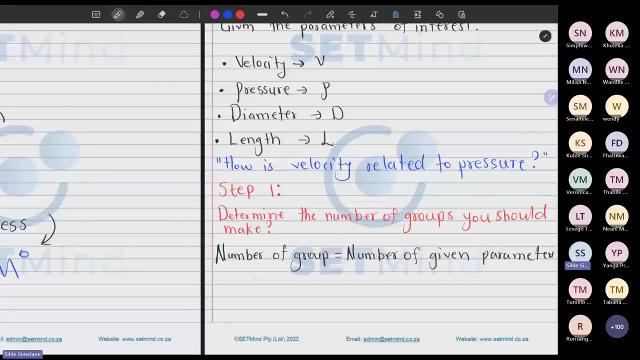 which has this group combination, which has another group, And how do you find the number of groups? The number of groups will be: it will be equal to the number of parameters we're given Number of given parameters And we will minus. 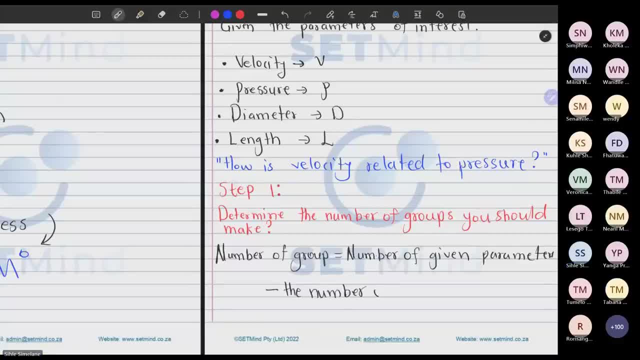 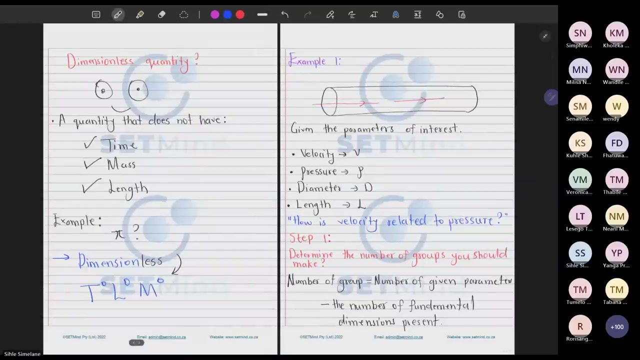 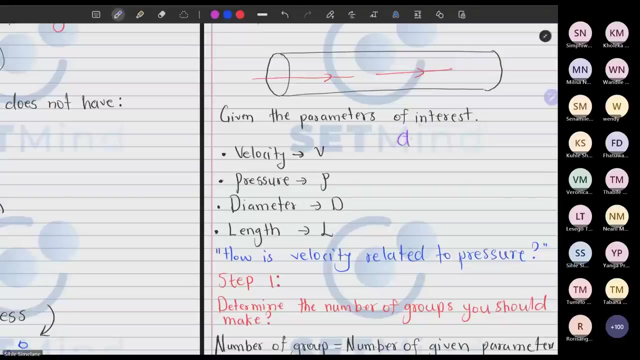 the number of fundamental dimensions present. Fundamental dimensions present. Okay, So what this means in human language is: let's quickly write the dimension for these ones. I'll just come here and say dimensions. So that's one of the things you should always do. 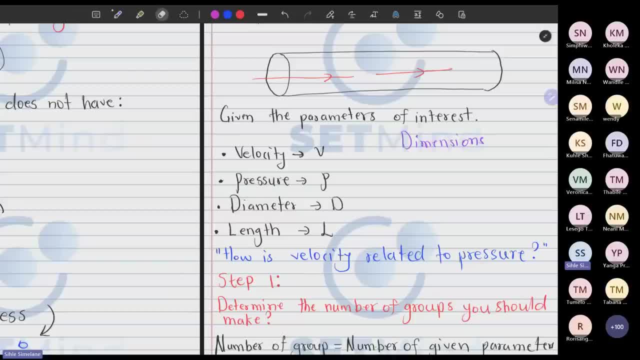 when you start a problem, Your dimensions are. we have velocity Velocity- if you can look at the previous problem, it is meters per second. In meters per second it is length, t to the minus one, And then pressure. where is pressure? 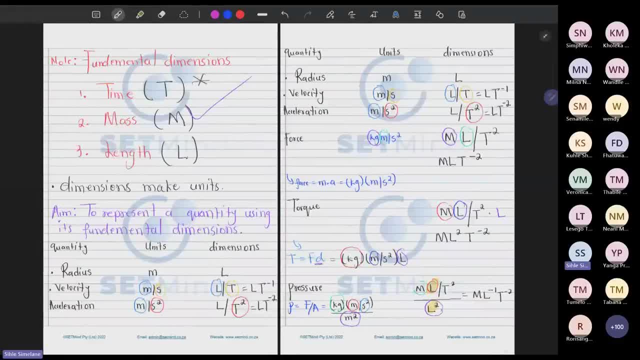 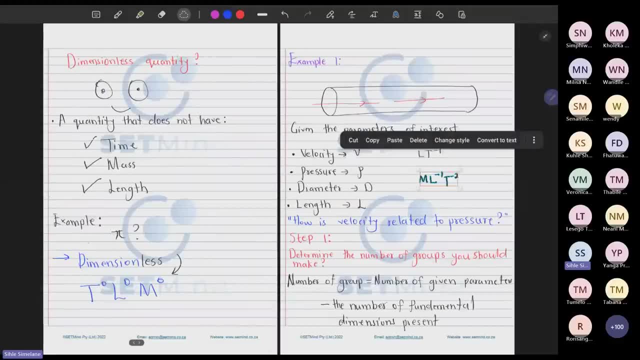 We found it: Pressure, pressure, pressure. there you go, Let me copy pressure and then go and paste it there. So there's our unit for pressure, And then diameter is length, So I'm just going to put L. 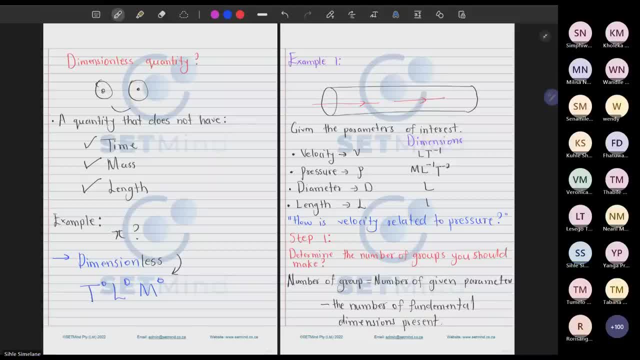 and length is length. I'm going to put L. So what we mean when we say subtract the number of given parameters, we are given one, two, three, four parameters. Okay, So that means the number of given parameters is four. 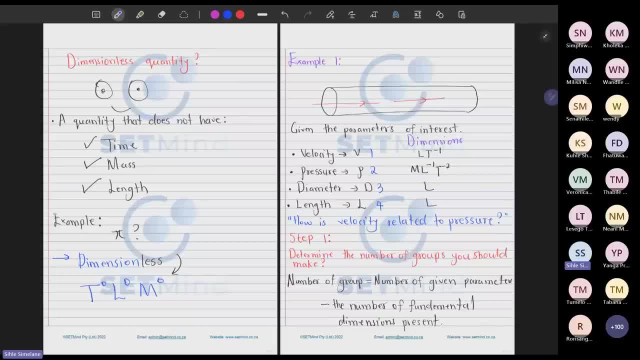 Then minus the number of fundamental dimensions present. The fundamental dimensions, remember, it is time, it is length and then it is mass. The question we need to ask ourselves: in the given parameters, do we somewhere see a T? do we see an L? 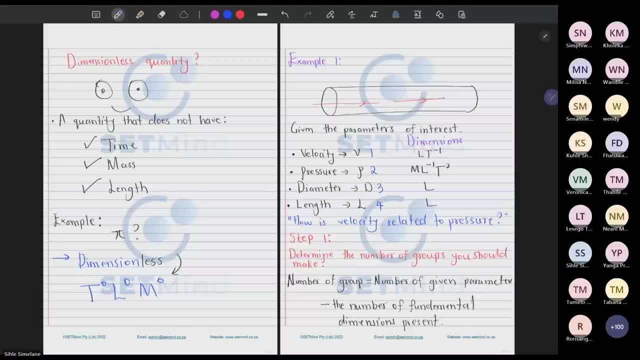 do we see an M when all of them are combined? If yes, then it means the number of fundamental dimensions present is three of them. Okay, So if you look carefully, when we look at our variables, there's our mass. 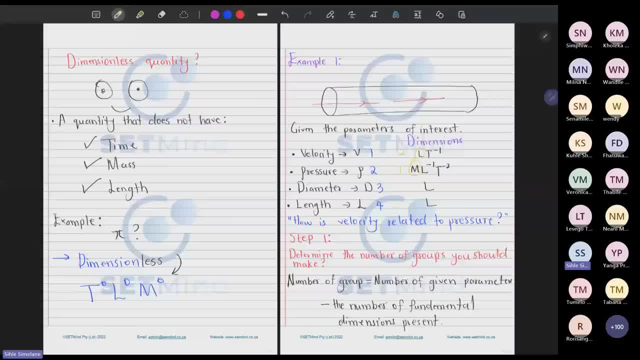 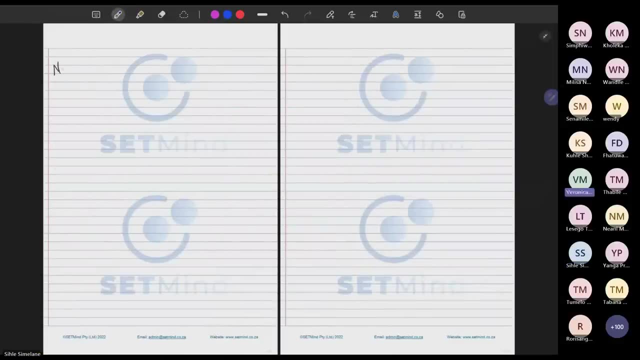 that's one, there's our L, that's two, there's our T, that's three, which means we have three fundamental dimensions. So our number of groups will be four of groups, it will be four minus three. 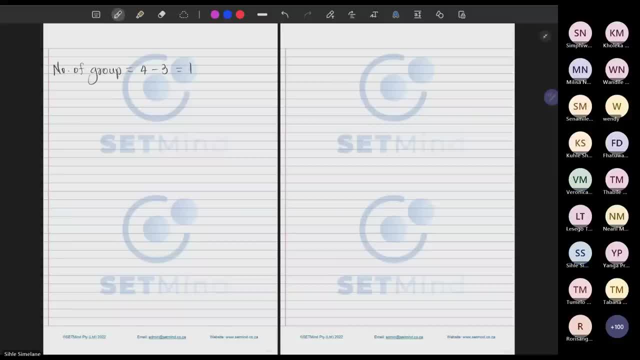 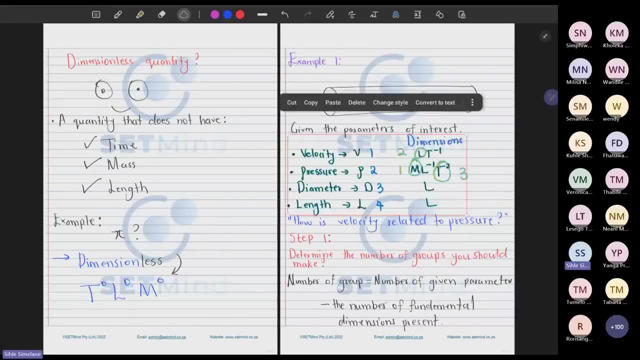 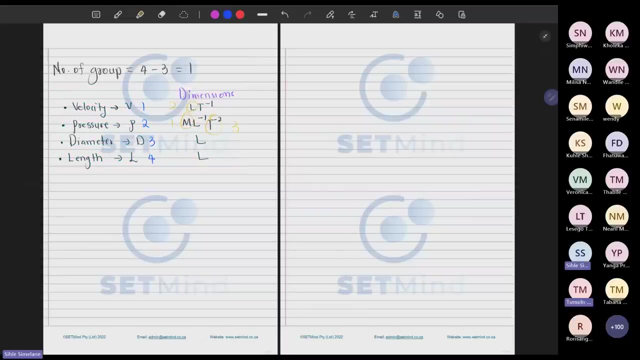 so, which means we can only make one group. What does this one group mean? You will see it shortly. So let's say hypothetically, let me copy the situation here and show you something. So let's say: when you look at the 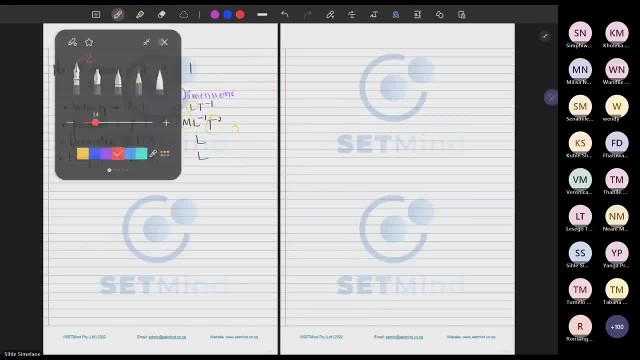 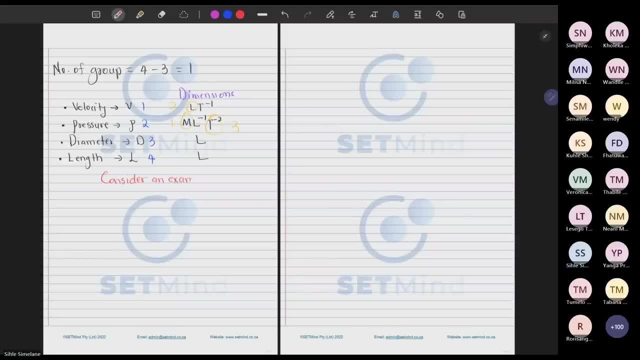 fundamental dimensions. let me deviate a bit An example. let's say: whatever, whatever parameters we have, we end up finding. one of them has dimension length, one of them has time, one of them has length, time, like that. 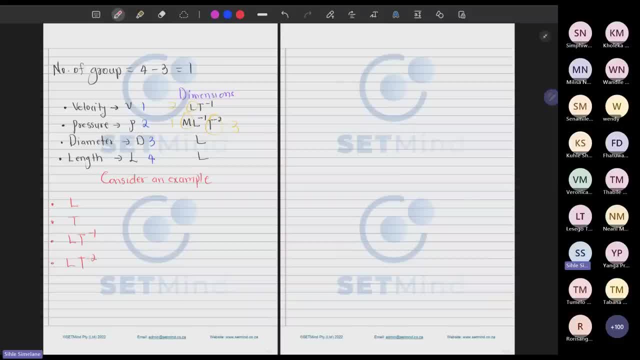 then one of them has length times minus two squared. So what we are going to be doing here is: we can see we have four parameters. That is straightforward. But then we look at the number of fundamental dimensions present. We see our L. 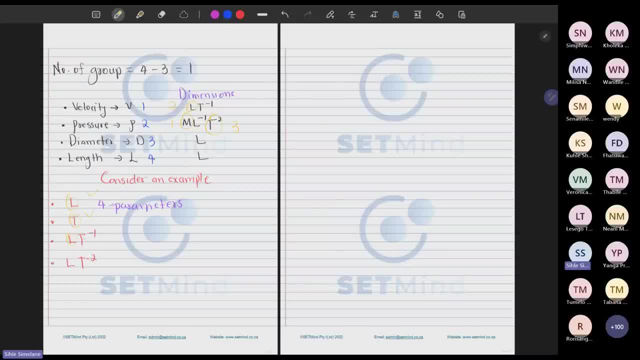 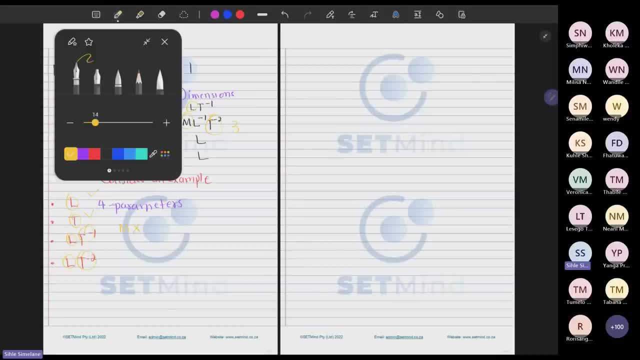 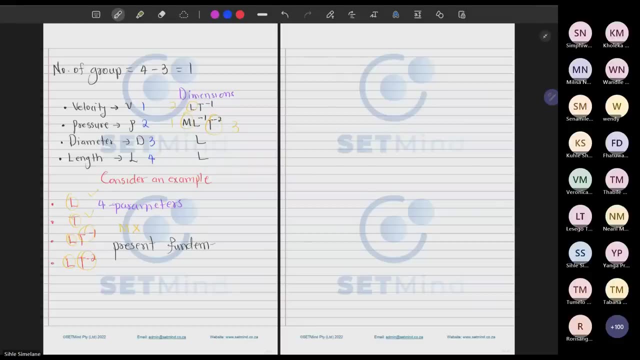 that's okay. We see our T, that's okay. A L again, T again, L again, T again. but mass is not there. So this means our present fundamental dimension. they equal two, Because one of them is missing. 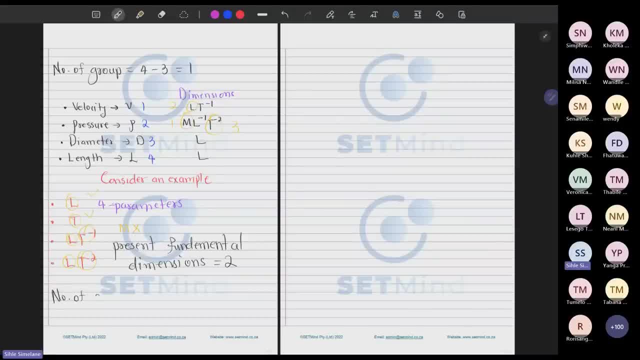 So in this case, it means the number of groups, which you should not stress about now, which has need to be four minus two, which means you need to make two groups, Okay. So this is an example to show you that. 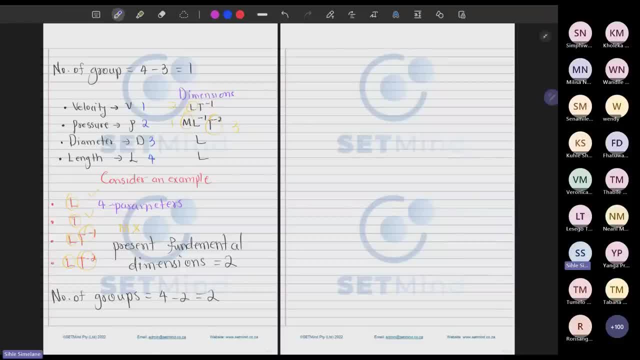 what do we mean when we say the number of present dimensions or fundamental dimensions? Okay, So let's come back to our problem. We are happy that we need to find one group. We are really happy because this means there's not a lot of work. 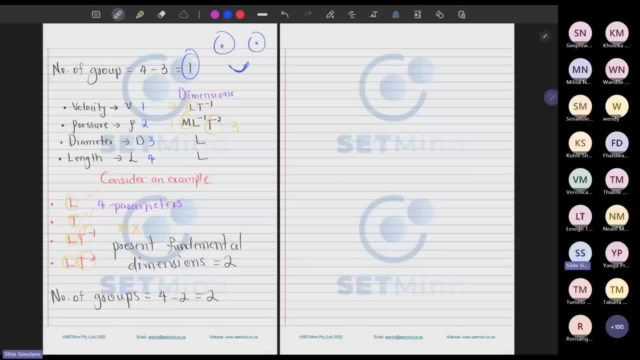 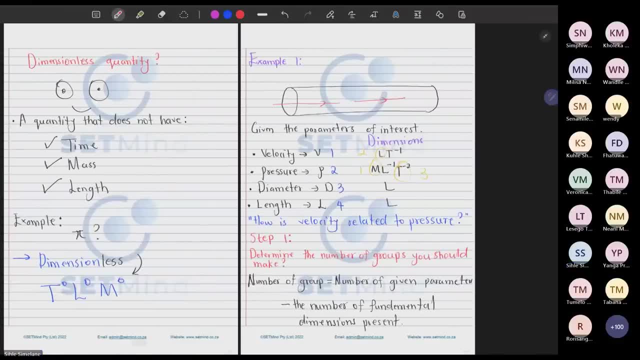 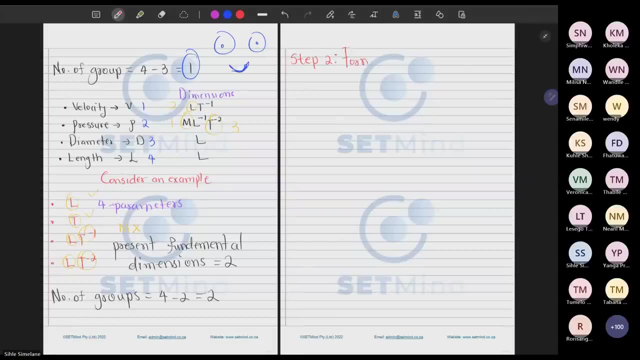 Life, life is easy. Okay, So we will form step number two. But step number one, I said you need to determine the number. Then, step number two, you need to form a dimensionless, dimensionless product of the parameters. 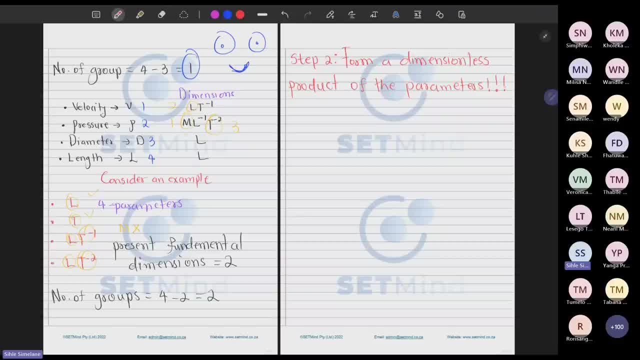 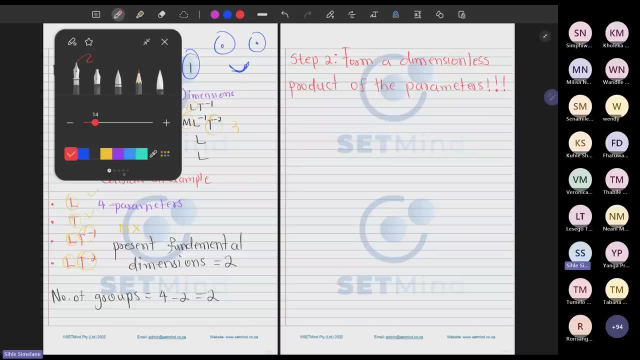 This sounds cool. The statement is straightforward: You need to form a dimensionless product of the parameters, meaning we multiply them. Then the answer we get should be dimensionless. Okay, So we have velocity. Look at what we are going to do. 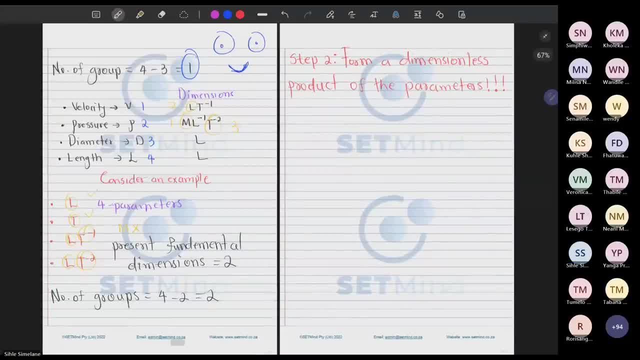 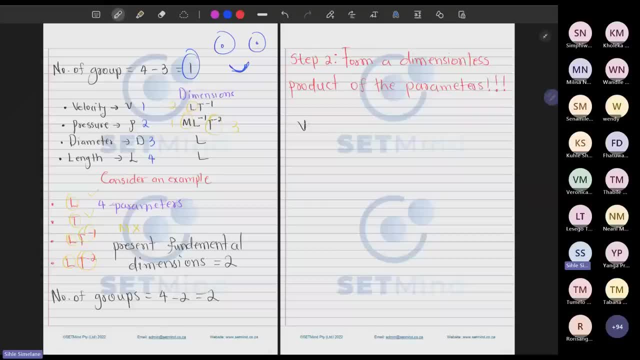 Step number two says: form a product, The parameters such that they are dimensionless. So we have velocity, which is V. Product means multiply: We'll multiply with pressure, Then we'll multiply with diameter, Then we'll multiply with length. 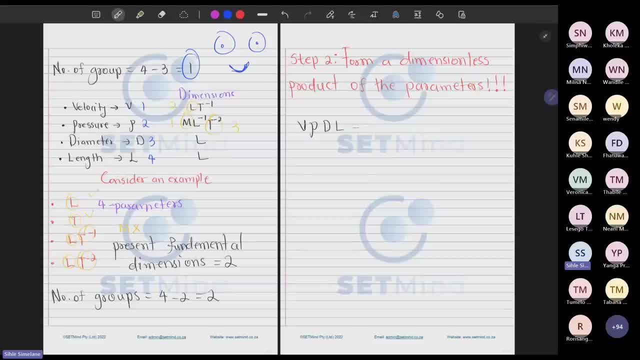 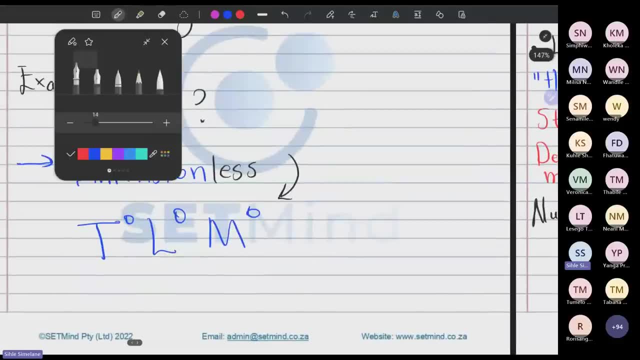 And this should give us a dimensionless product. Remember what I said about dimensionless. Come here. Where is it There? you go Dimensionless Here. When something is dimensionless, it means the T is to the zero. 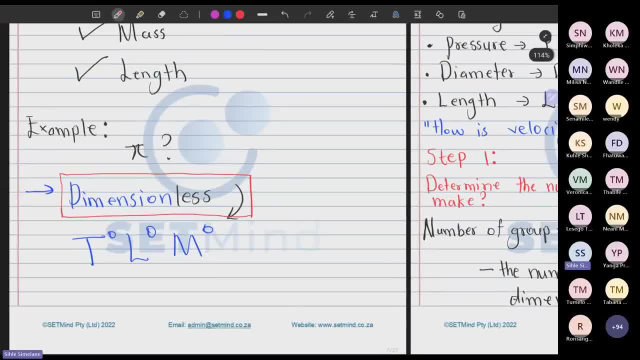 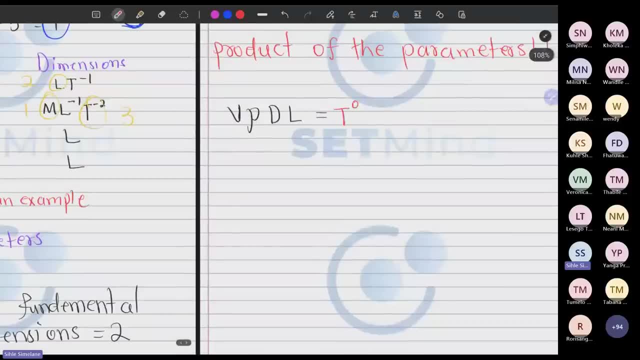 The L is to the zero And the M is to the zero also. So it means my answer here is equal T to the zero, L to the zero And M to the zero. This is dimensionless. 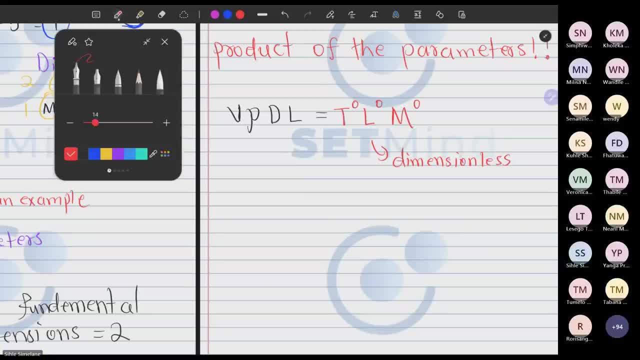 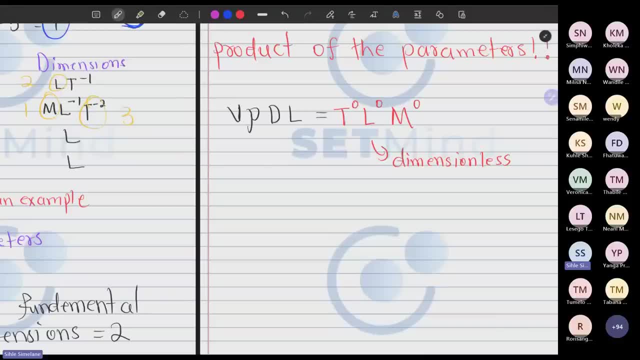 Then there's only one thing which we need to fix here: When you multiply these, without doing any multiplication, without doing any manipulation, you are not going to get a dimensionless quantity. So we'll put exponents, We'll put A. 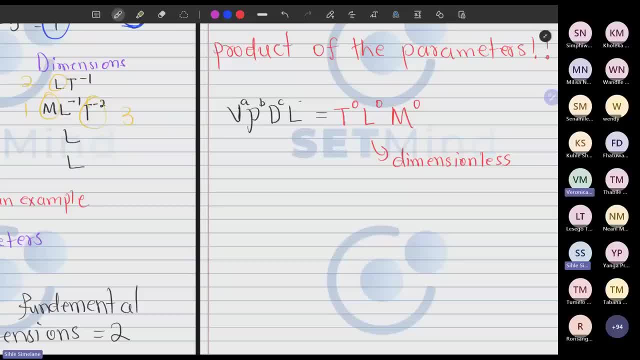 We'll put B, We'll put C, Then we'll put D. Okay, So V is to the power of A, P is to the power of B, And then D is to the power of C, And then L is to the power of D. 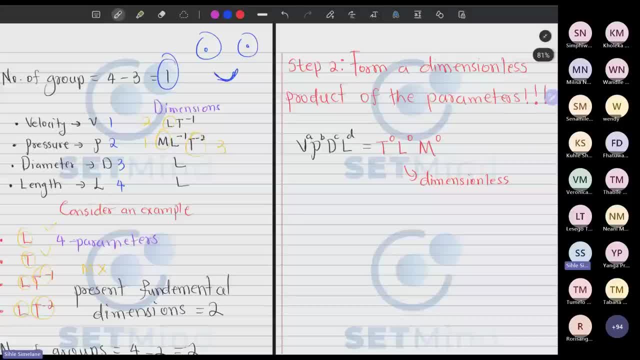 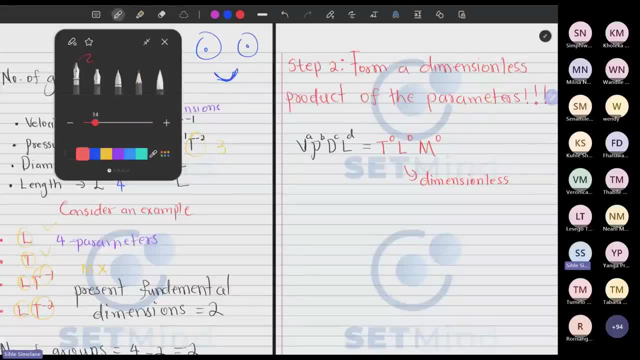 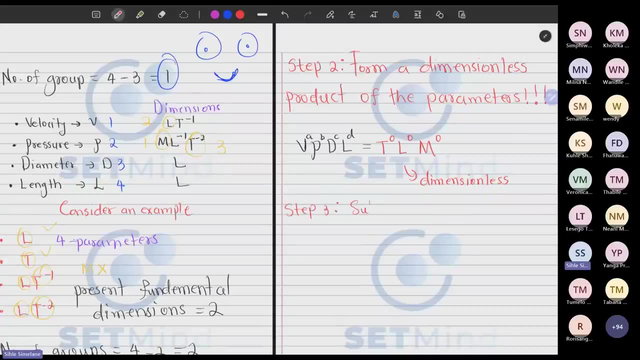 And then now, after doing this, we need to write our parameters in their fundamental dimensions. You'll see how we are going to be able to answer that question, because we started not knowing. So step three, Let me say substitute. 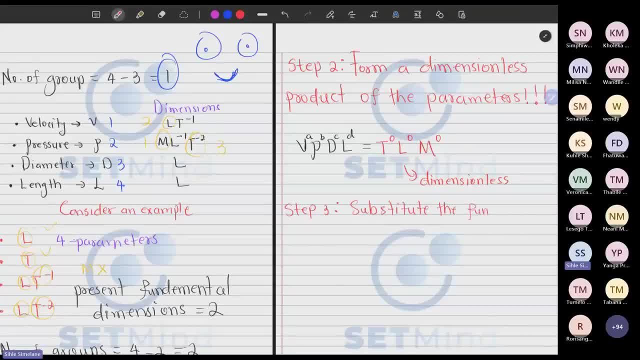 the fundamental dimensions in step two, So meaning the answer we have from step two. that's where we start putting in our fundamental dimensions. Okay, Look at what we do: Velocity, which is V Velocity: we know there are fundamental dimensions. 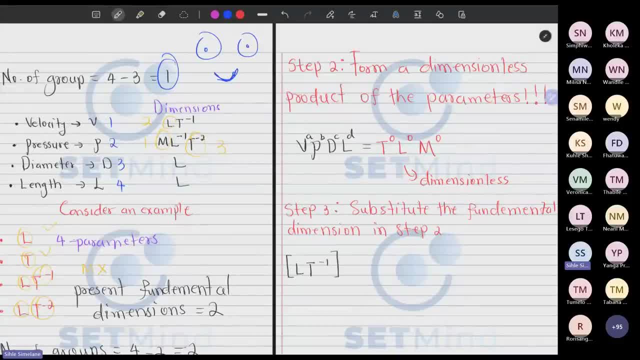 It is L Velocity to the minus one, And this is to the power of A Pressure. So the fundamental dimensions. you should know them, the same way you know WSS. So do not worry With time, you will be able to recall them. 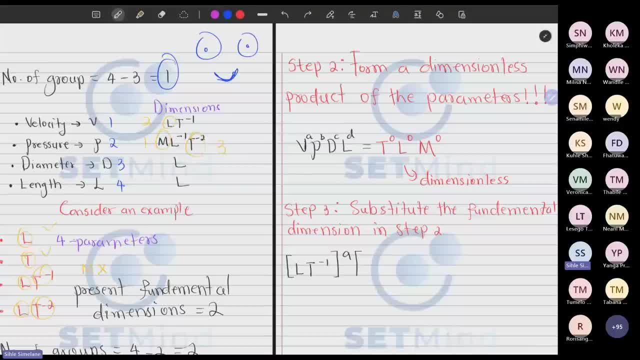 If you do not mistaken Chamber of Minds for WSS, when you look at fundamental dimensions, the more you do them, you will not mistaken both for pressure, Okay, So it's really nothing hectic. Hang in there And believe me, with time. 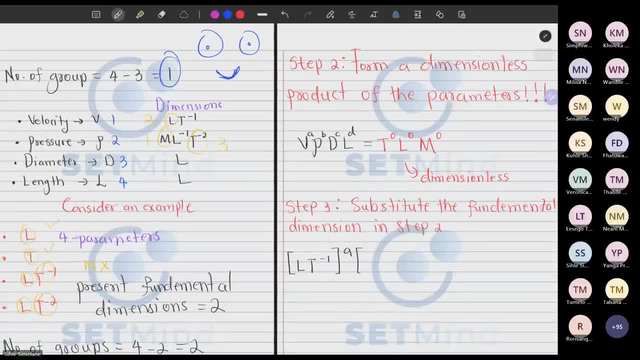 you'll be able to recall this, Because you should print a table this week which should stay on the wall of your room or your study room where, when you wake up, you look at the fundamental dimensions And say, pressure, I know it on top of my head. 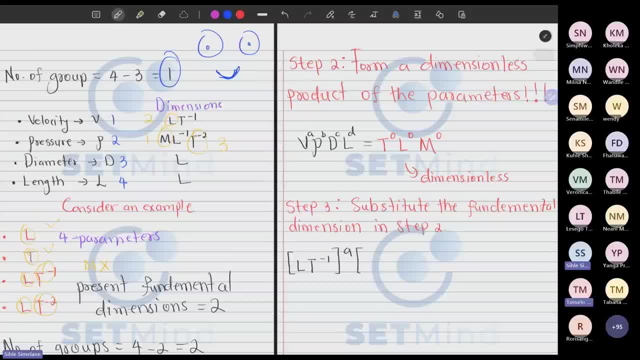 Force. I know it on top of my head Because it's going to save you time when you write your exam. If you know what force is already, you are many steps ahead. You know what velocity is. If you know what pressure is. 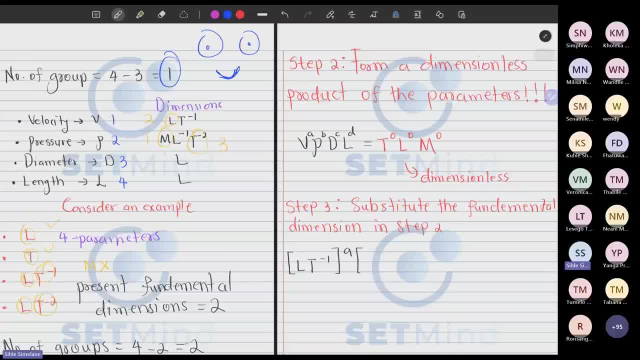 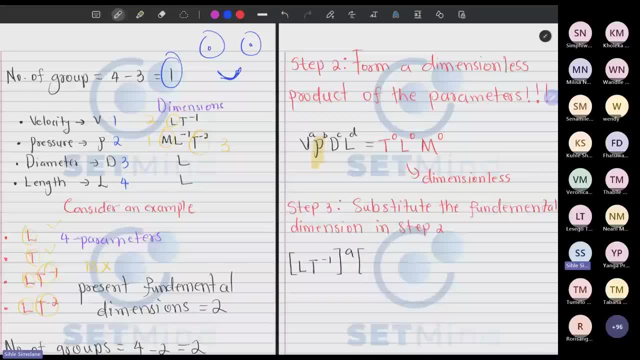 you will jump. You will jump many steps and give them the answer. So back to what we are saying. Let's go and substitute the dimensions for pressure. We look them up on the left. We have to choose them to be m l minus one. 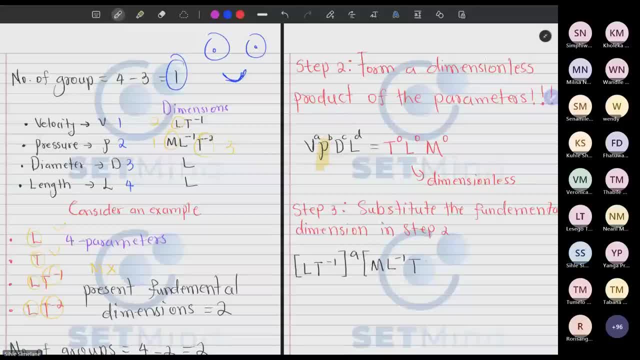 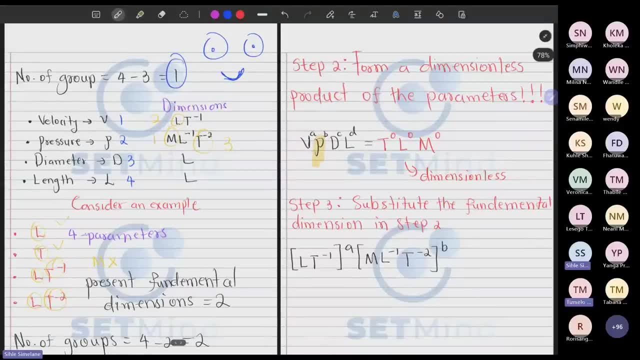 t minus two, And then this is to the power of b. Okay, And then we go to diameter: Diameter. well, it sounds like length to me. Well, we'll put in l to the power of c, And then we have the length of the pipe. 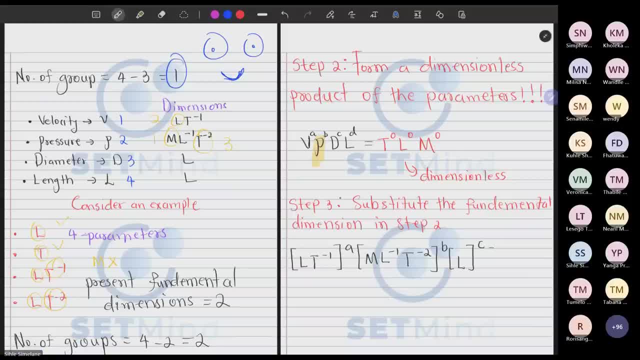 Well, according to fundamental dimension, length is length. So I put l to the d, And then let's make this smaller to write our dimensionless quantity on the right hand side. All this should equal to m to the zero, t to the zero. 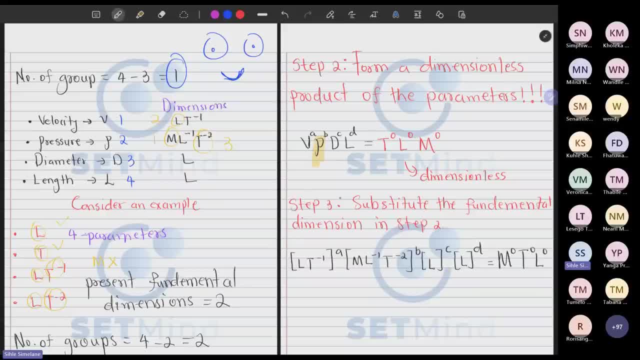 and l to the zero, Because we said step two form a dimensionless product of the parameters. Okay, And then now, what we are going to do is we will distribute the exponents. Okay, Let's get to this grade nine maths. 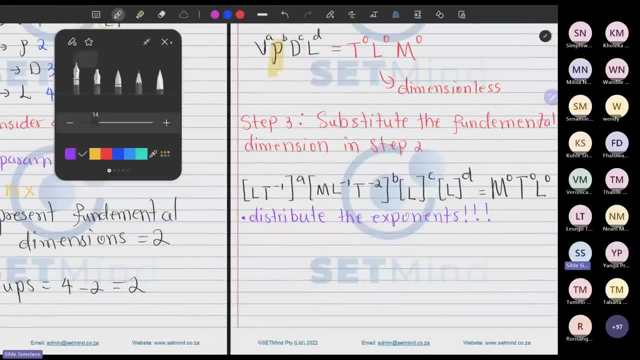 which your sibling should be able to do, or your cousin or your friend. So if we distribute the exponents, let's focus on the a part, Let's focus on this one first. Others will follow. So if you look at what is going on here, 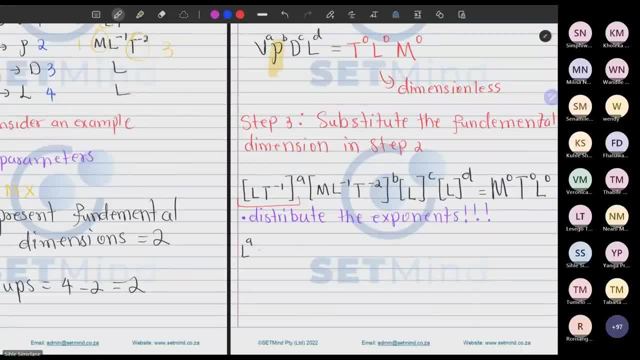 the a will go to the l, So we'll have l to the a, We'll have l, We'll have t to the minus a. Remember exponential laws with people. When you have a to the m to the n, the answer is simply a m? n. 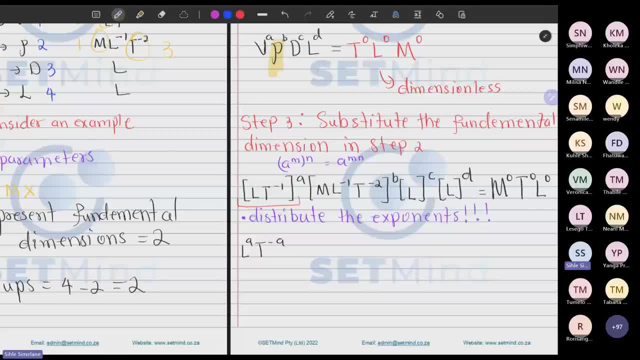 This is grade nine. Okay, So let's quickly look at the other one. So when we look at the b part, the part which is raised to the exponent of b, it will be m to the b, l to the minus b. 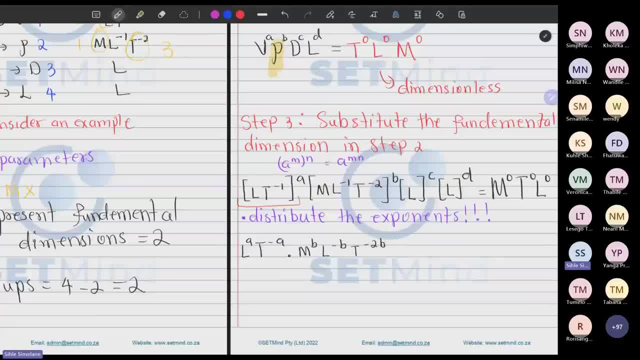 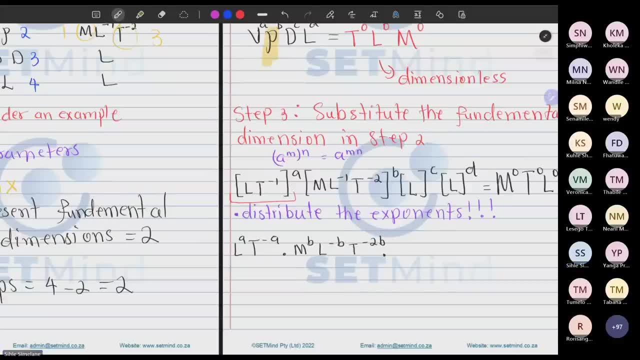 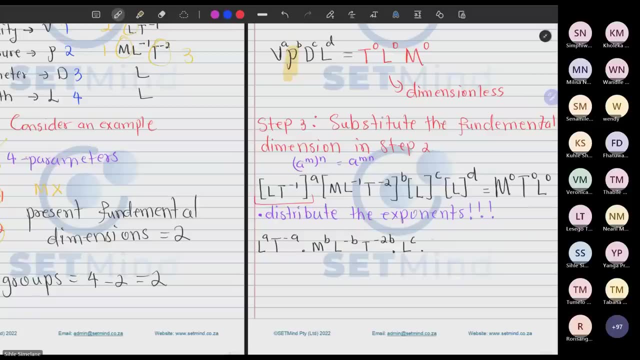 t to the minus two b. Okay, So then, when you look at the part which is raised to the power of c, it is l to the c. Well, that's done. Then, when you look at the part which is raised to the power of d, 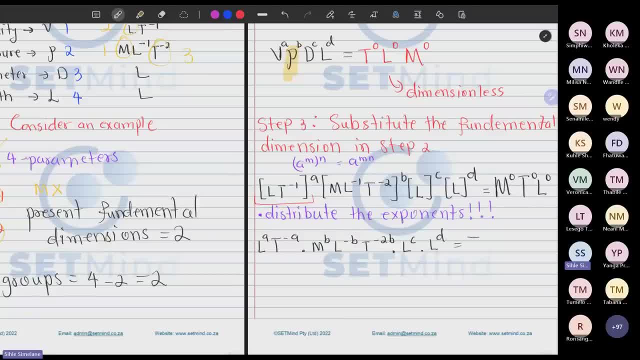 it is d, it is l to the d, And this should equal to m to the zero, t to the zero and l to the zero. And then now, what we need to do is to combine like terms. We may combine like terms. 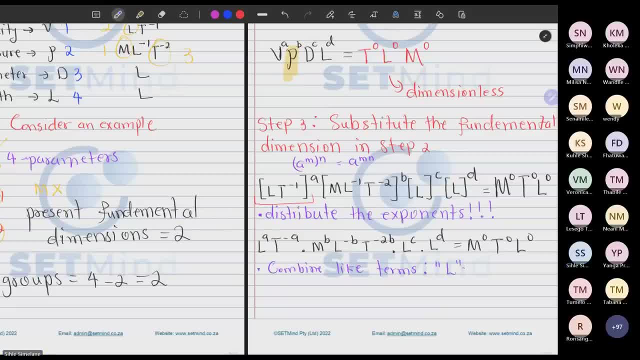 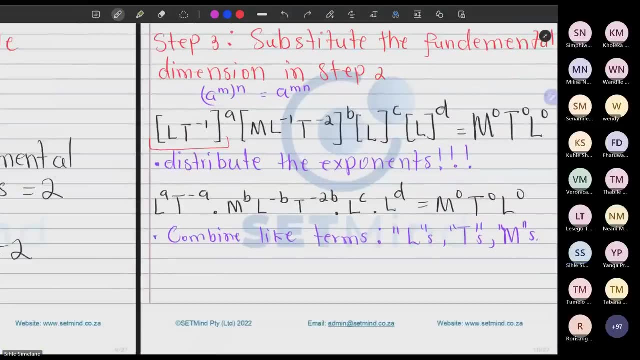 What we mean by that is combine the l's, the t's and the m's. Okay, Let's quickly see how we can do that. So let's put the l, So we are multiplying. So for the l, it means I'll have a. 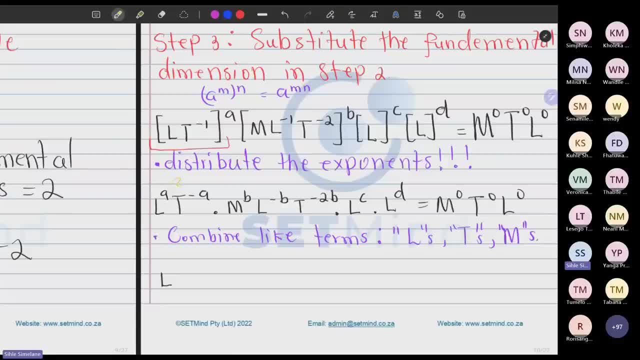 When you multiply, remember the same way as you add the exponents. So I have to the power of a and then it will multiply by that, which means I'll have a minus b. It will multiply with that, Then plus c. 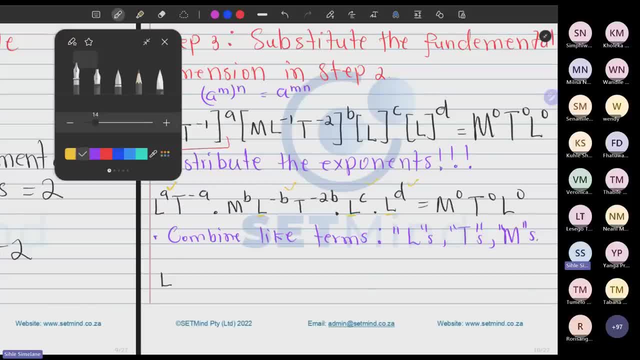 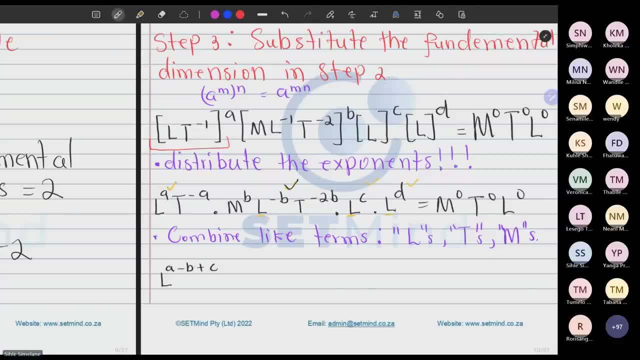 it will multiply with that plus d. So what that means is that I have a minus b because of that exponent, plus c because of this one and then plus d Because of that one. Okay, Done with the l, Let's go and focus on the m. 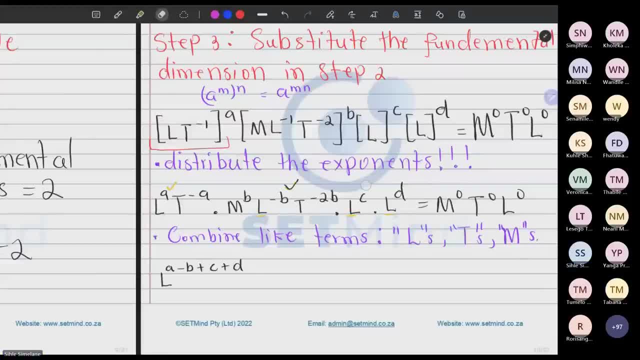 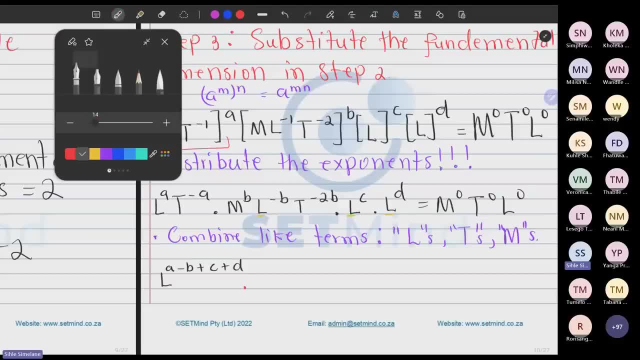 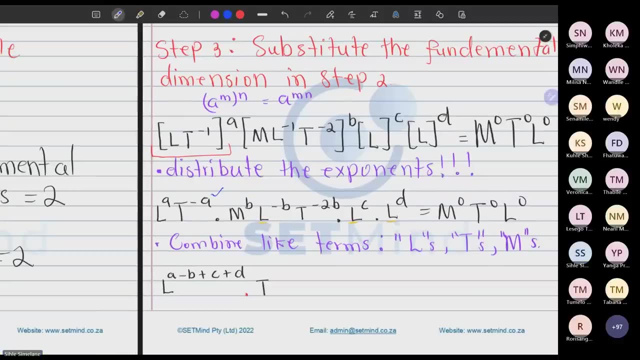 And then eventually focus on the t. Okay, Let's put it out here And then take our t. So when you look at our t, you multiply the same way as you add the exponents, So we'll have minus a, minus 2b. 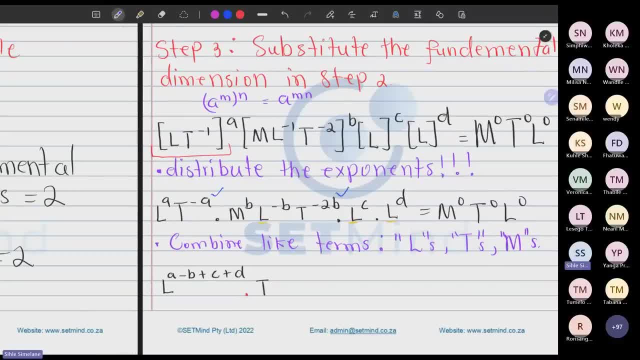 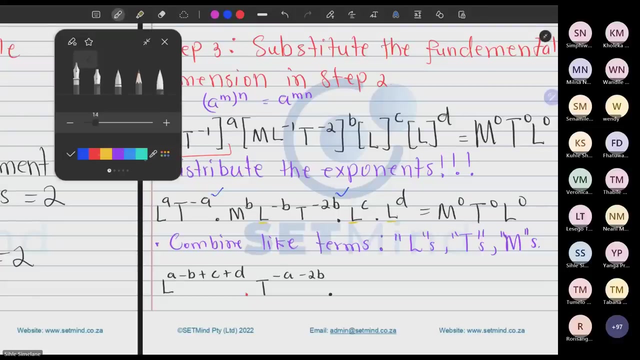 well, that's done. So we have minus a, minus 2b, and then we are done. I can't see any other t. Okay, No problem. But now we are left with the m, So let's see, Yeah. 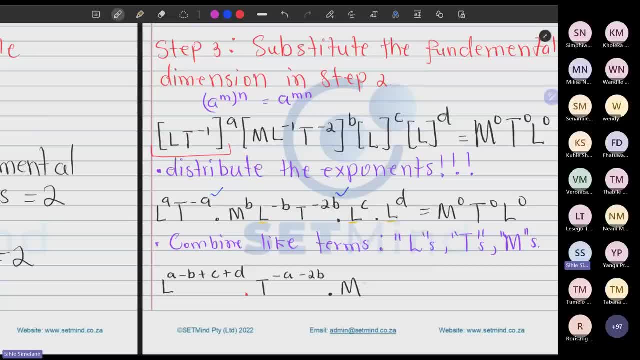 So let's put the m here. Then when I look at the m, I have m and that's the end. So I'm going to have m to the b and then this will equal m 0, and then l 0,. 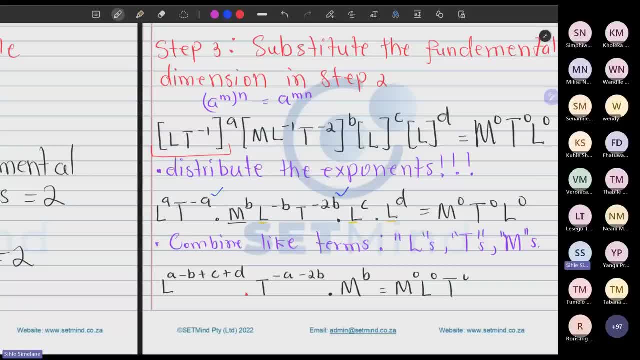 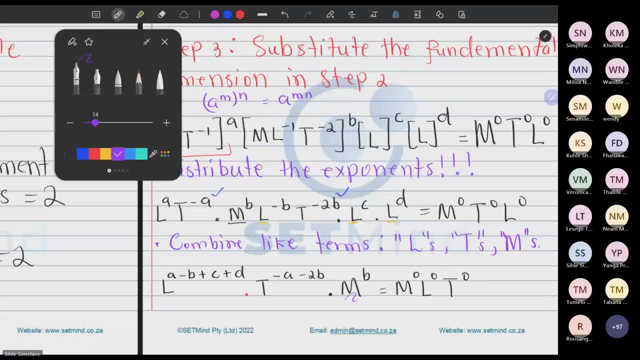 and then t 0.. Okay, And then this is where we start comparing the right-hand side and the left-hand side. Okay, So when you compare the right-hand side and the left-hand side, we can see that this here should be equal to that. 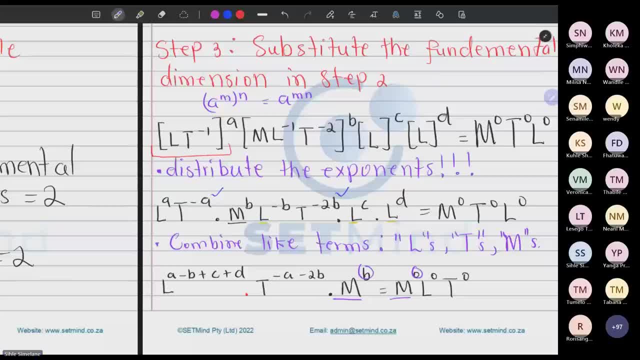 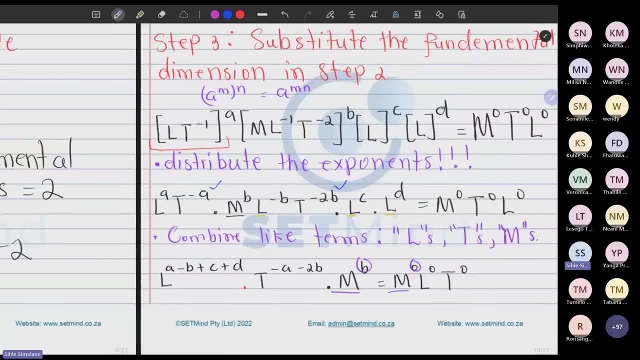 And then we compare the others again so that we can form a dimensionless quantity. So if you look carefully, our m should be 0,, our b should be 0. And then you'll be able to solve all the others. So before I carry on here, 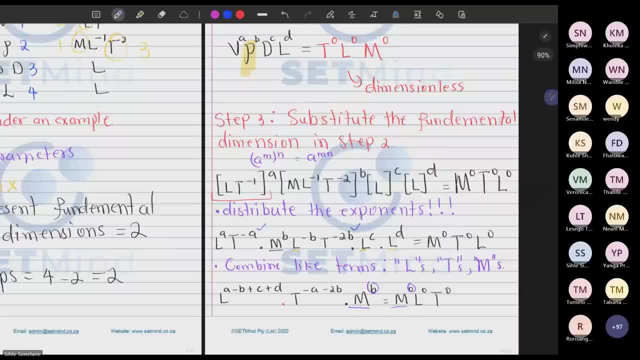 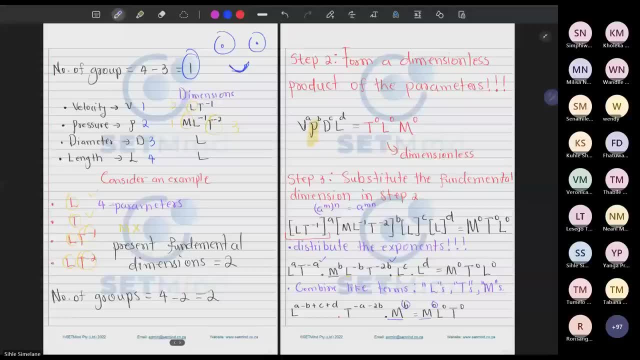 do we have anyone who has a question? Okay, Let's quickly compare this and then I'll comment on one mistake which you should not do. Okay, Which is why I was talking about the number of groups here. So our hypothetical example is problematic. 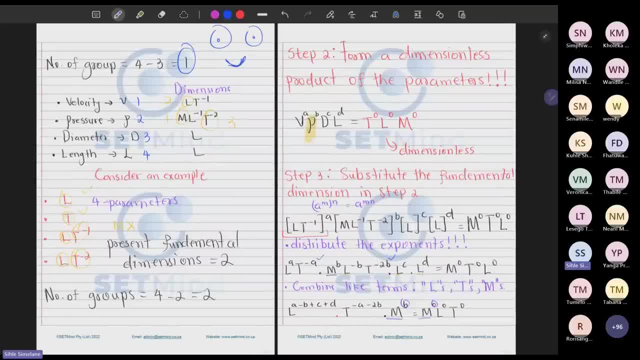 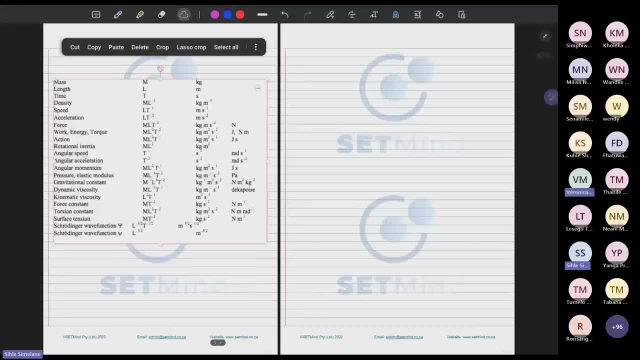 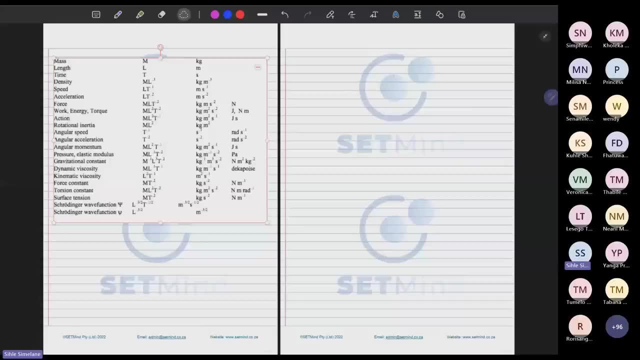 but why not? So if we look at the m's, let's copy this. go to the next page. Okay, Let me just show you this before we carry on. So this is one of the tables which you should know. I believe it is there at the back of your study guide. 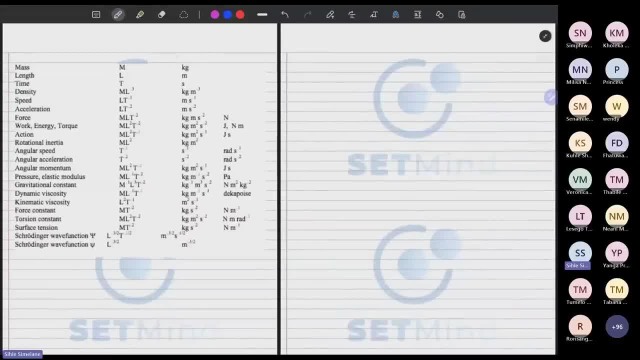 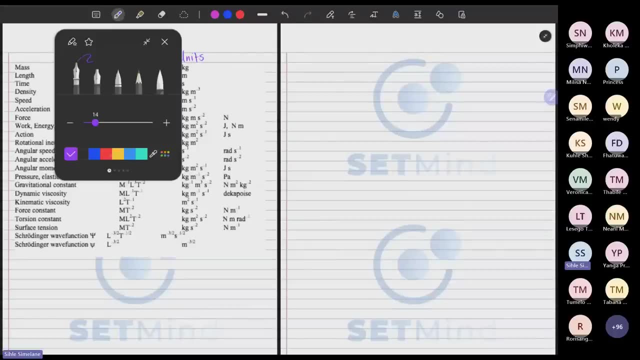 So if you look here, what we have here is simply units And what we have here is the dimensions. So this here. you need to know all of this, because that's where you are just going to be working. You should know mass. 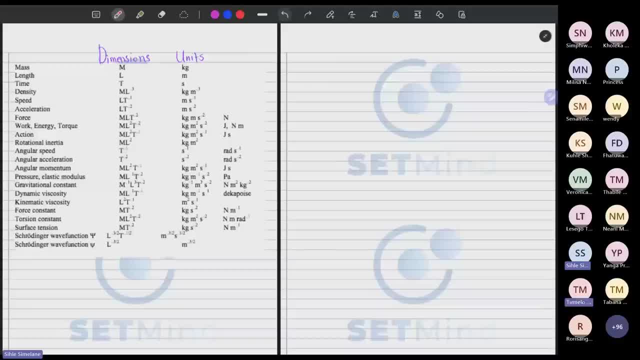 You should know length, time, density, speed, acceleration, force work, action, rotational inertia and the rest. You should make sure that you know them. So, if you can know this, let me exclude these ones here, Let me cancel these ones. 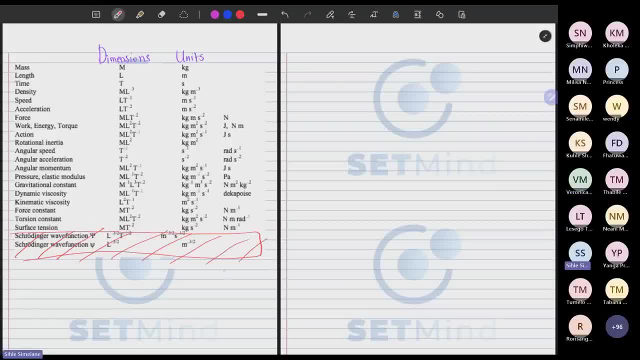 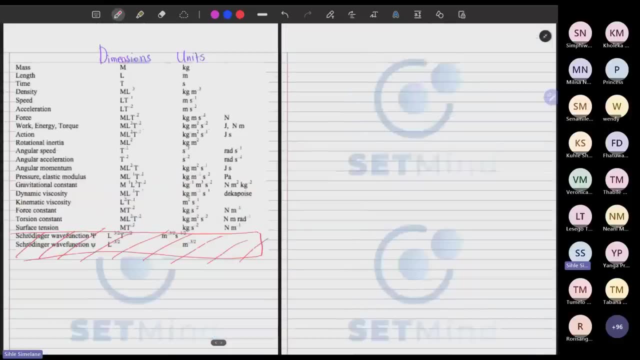 Otherwise, everything else which is here is make sure that you know it. One way or another, when you do your TAT questions, it is going to pop up, Okay? So if you look at the problem, so this table is a mass node. 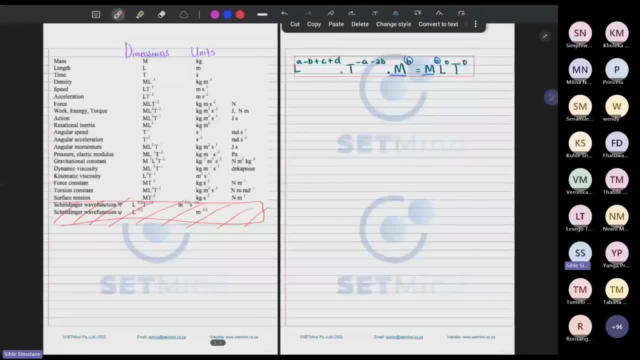 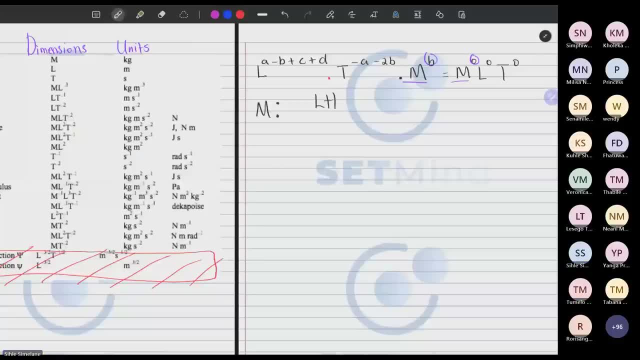 Let me paste here. So let's look at what is going on. So let's focus on the M. So if you look at the left-hand side and the right-hand side, So for the M on the left-hand side, we have M to the B. 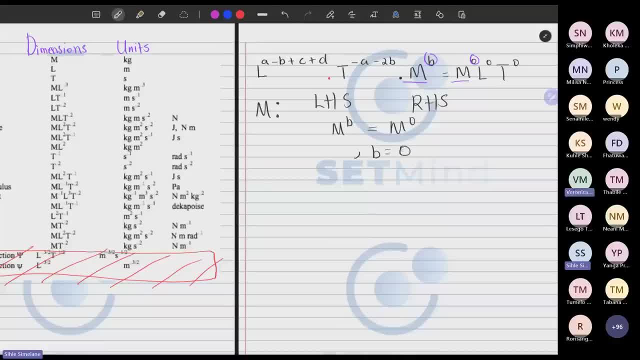 On the right-hand side we have M to the zero, So this means B is zero. And then let's look at the T. The T on the left-hand side is T minus A minus 2B The T on the right-hand side. 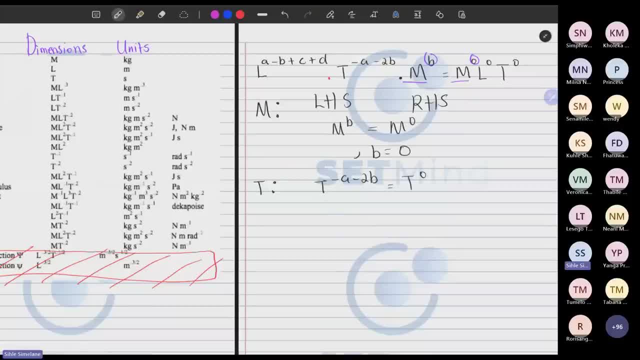 is T to the zero. So if you look carefully when you solve here, you'll have negative A minus 2B, Equaling zero, But however, B is zero, So you find A as zero. Okay, Let's go to L. 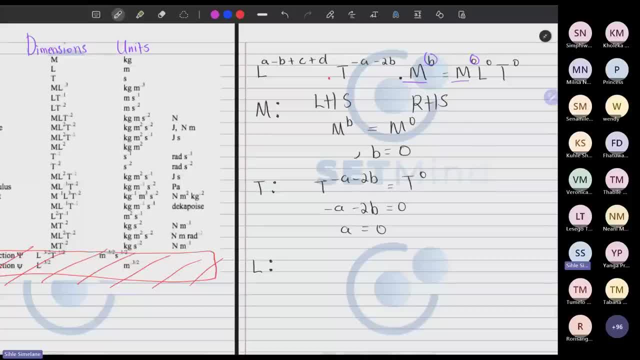 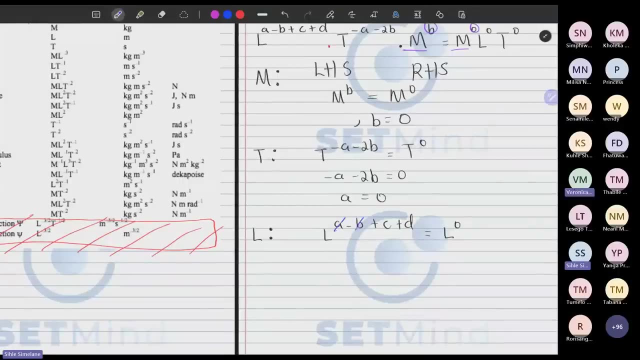 So when we go to L, if you look carefully, we have L to the A minus B, plus C plus D equals. on the right-hand side we have L to the zero. So A and B are zero already. So A and B are zero. 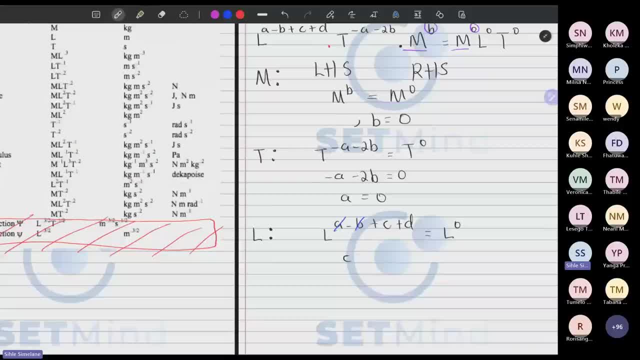 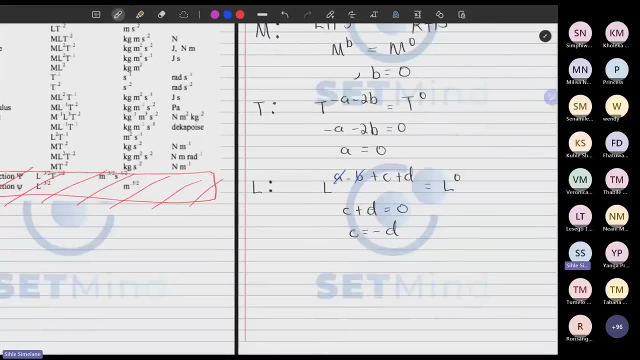 So, if you look carefully, what we are going to have is simply: C plus D equals zero, So our C will be negative D. Okay, So C is negative D. We can choose them to be anything, But let's go to our original combination. 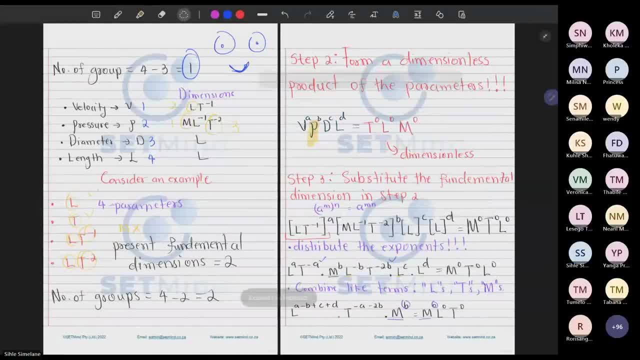 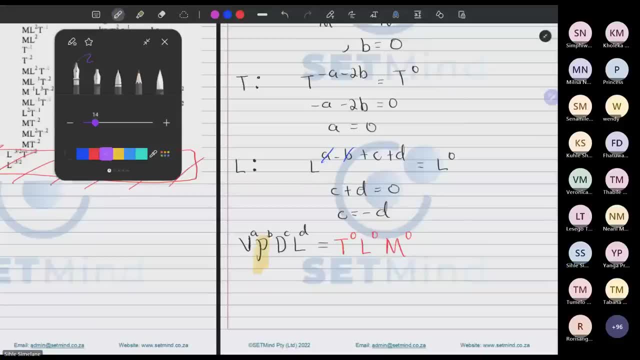 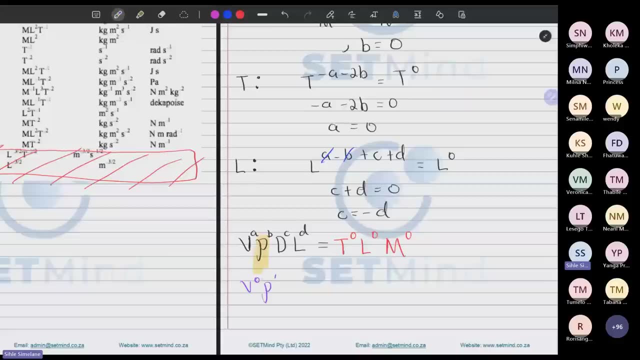 of these terms and see what this means. So, if you look carefully, our A we obtained as zero, So meaning we have velocity to the zero, We have present to the zero, because the B was zero And then C, they are saying D to the C. 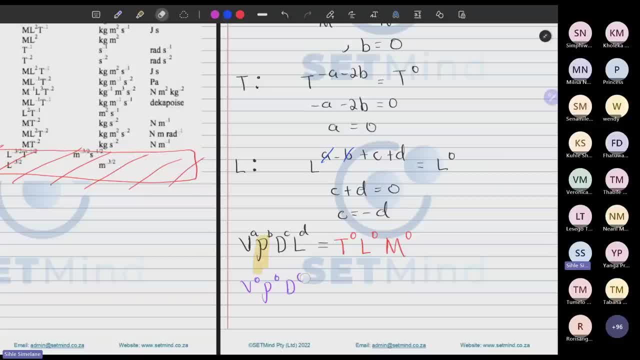 C is equal to negative D. So I can choose to put negative D here And then the L I can put D. So these ones, if you look carefully, they just die out. And then this I can equate to a dimensionless property. 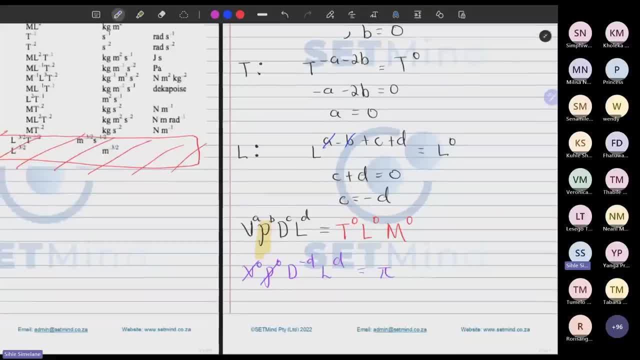 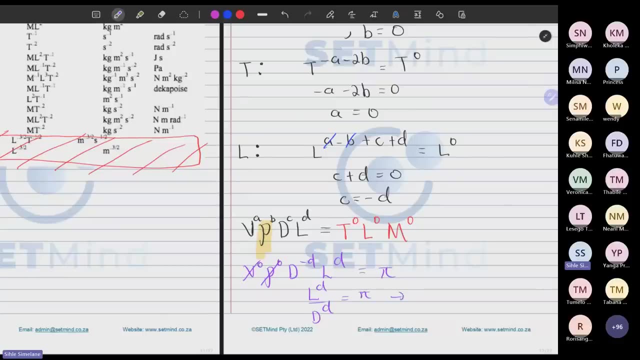 Let me call it pi. So if you look carefully what is going on, we have L to the D over D to the D, equaling pi, And indeed this is dimensionless. So if you look carefully, what we end up having is we can decide on D and A. 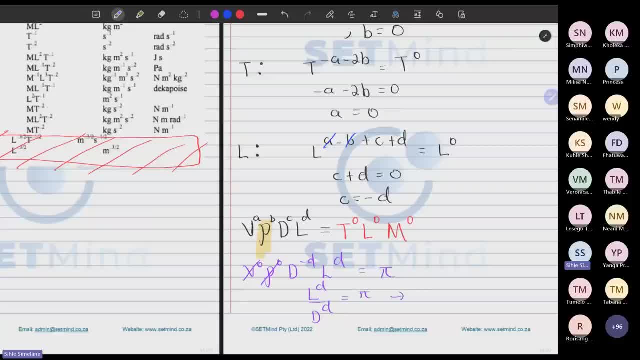 You can make them to be one. Whatever you make them, the relationship between the two is the same: That L over D will always give us a dimensionless property, which I will call pi two. Okay, And then a question we start asking ourselves is: 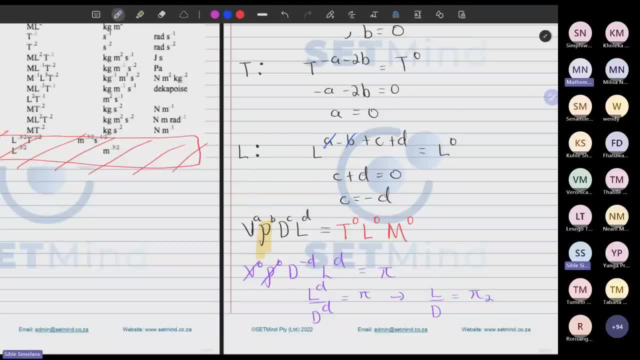 why is present, not popping up here? But before we go there, do we have anyone who has a question? Anyone? Okay, you can. the first question I captured. if you are still, can I please re-explain. There was someone else. 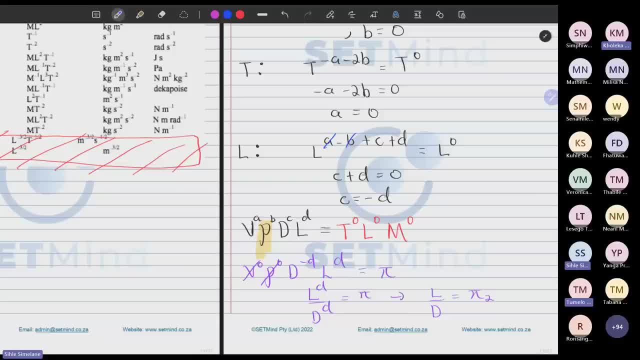 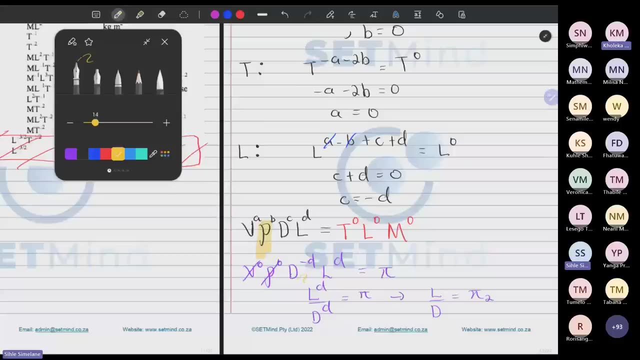 wanted to ask a question. I wanted to ask: why did we say L to the power D divided by D to the power D? Okay, so do you understand why we have D to that power minus D? Yes, Okay, do you understand. 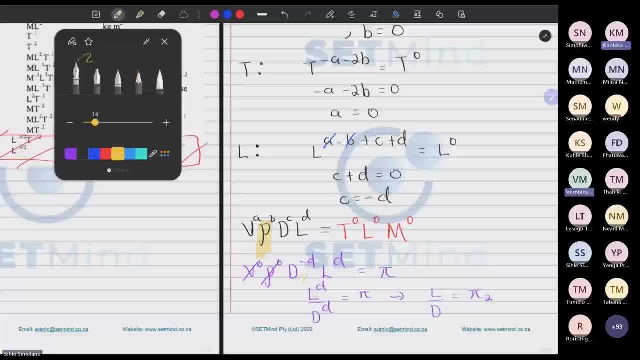 why we have L to the power of D. Yes, Okay, so when you have a negative exponent, for example, two to the minus one or two to the minus three, is the same as one over two to the three. Yes, 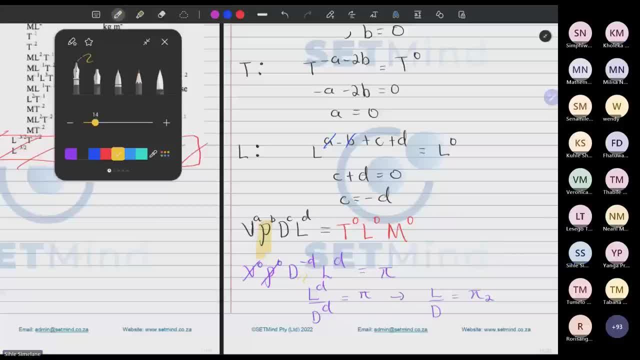 We know that. So that is why. And then you just push it to the denominator, you change the power you make to be positive. Does it make sense? Yes, So if it was a positive D in both, what was going to be the case? 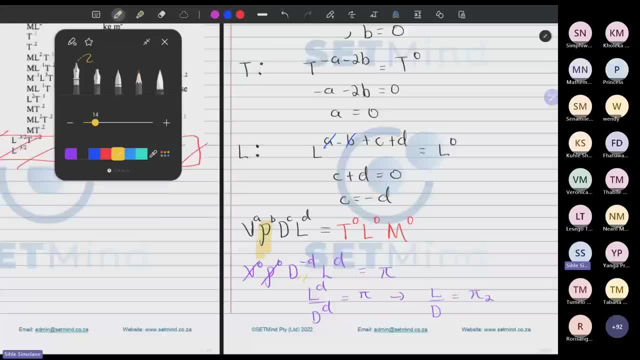 It was going to be D to the D times L to the D, So there's nothing which we are doing here which is something special. It is just three multiplications, Okay, Okay, And there was the gentleman who posed a question. Please go ahead. 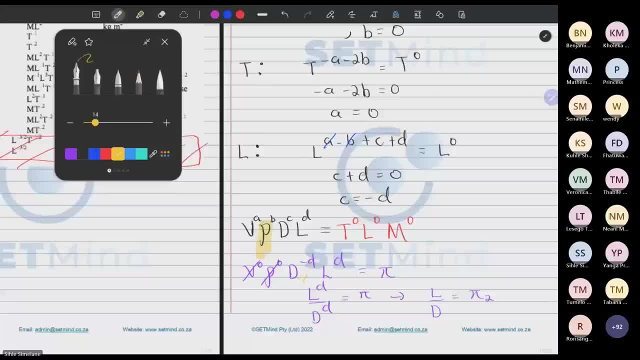 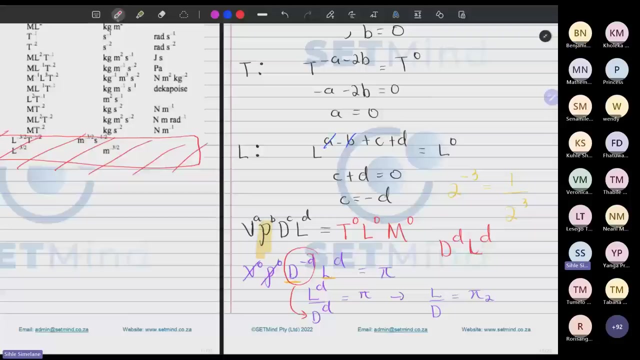 Okay. So I don't understand the part where you equated D to the power minus D and L to the power, D to pi. Okay? You mean here? Yeah, Okay. So pi is the dimensionless quantity. So this here: 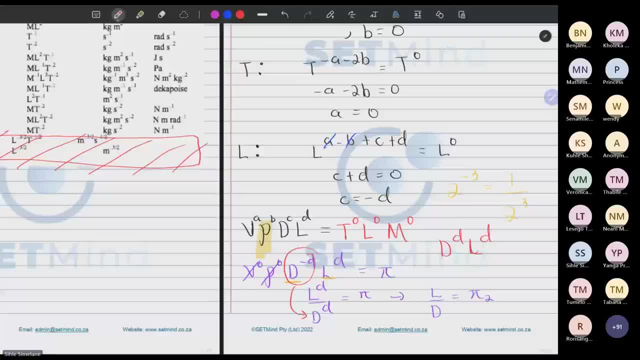 this side is dimensionless. So what I'm doing is, even after obtaining the values which would make this to be dimensionless, it is still dimensionless. So I chose pi. So I'm going to equate to pi, which is dimensionless. 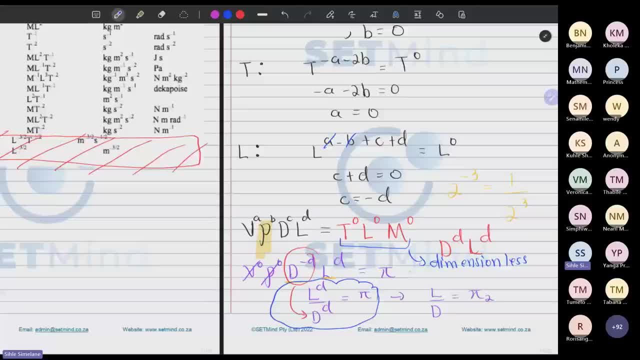 Or maybe just the quantity can go with that way, Not just pi pi as in like pi 3.14,, but I'm just representing a dimensionless quantity using pi Oh, So the product is still dimensionless. You understand? Yes, sir. 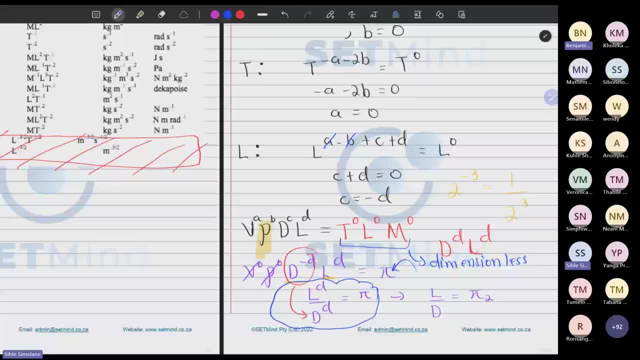 So, sir, on the second question, you dropped out this D on the part of L over D. This D disappeared here. It's because we do not know what D is. So you can choose D to be 1.. And then, by choosing D, 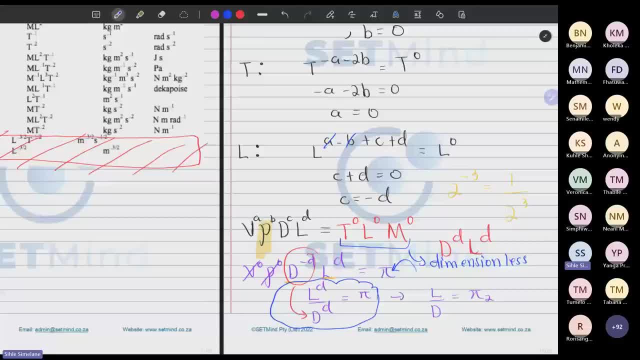 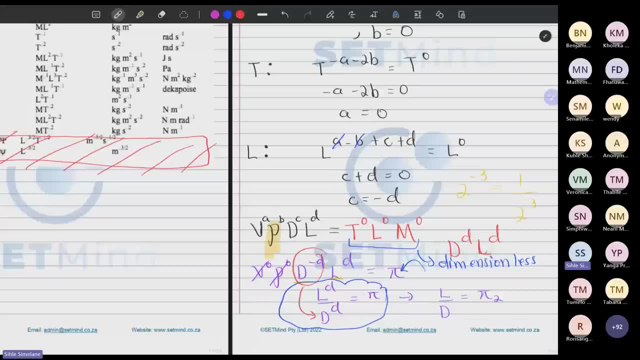 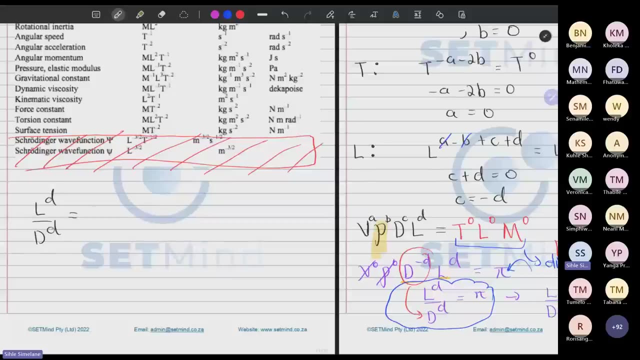 you are choosing C indirectly, But the logic is, just think of it this way: If L to the power of D over D to the power of D, they give me something which is dimensionless. You can also take the square root or the D root. 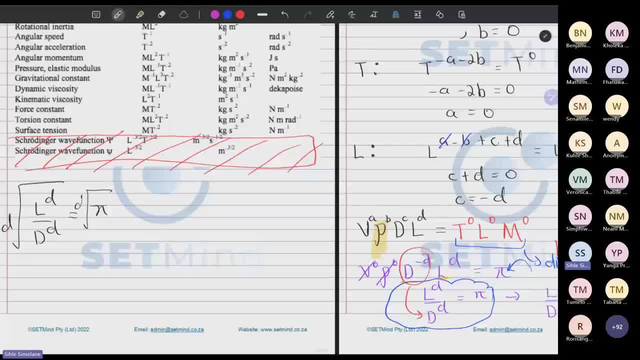 such that you cancel both sides the D and then you have L over D. It would still be dimensionless, because on the right hand side, if you take the square root of a dimensionless thing, you still do not get any dimensions. So instead of now leaving it at pi, 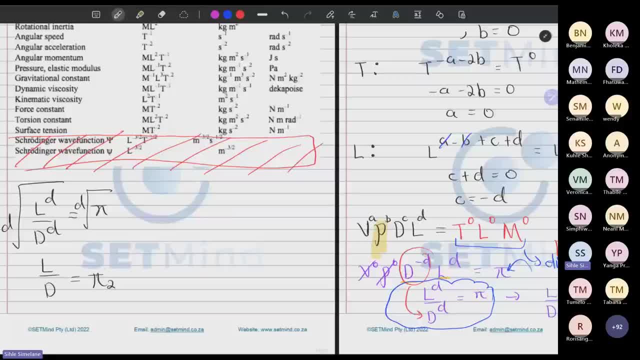 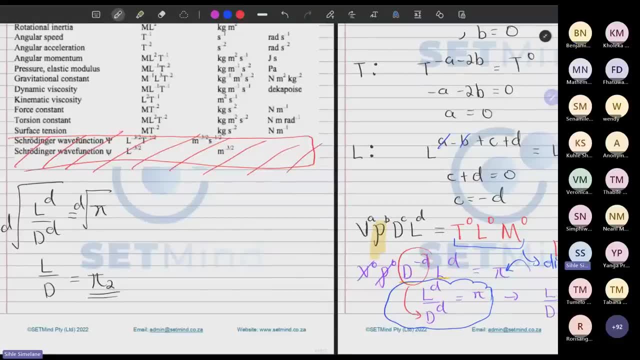 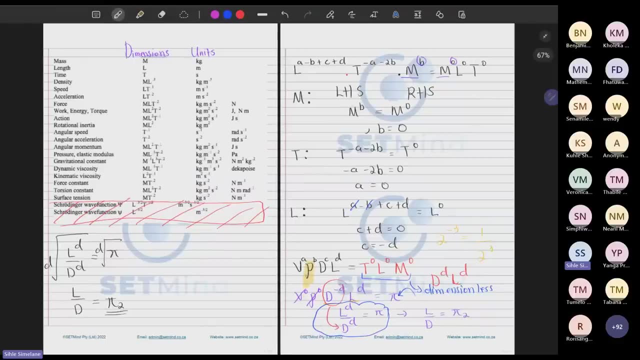 I'm just going to say it's pi 2, but it's still dimensionless. Do you understand? Yes, sir, Okay, No problem. So here's what I need you to think of carefully. The original question was saying: how is pressure related to? 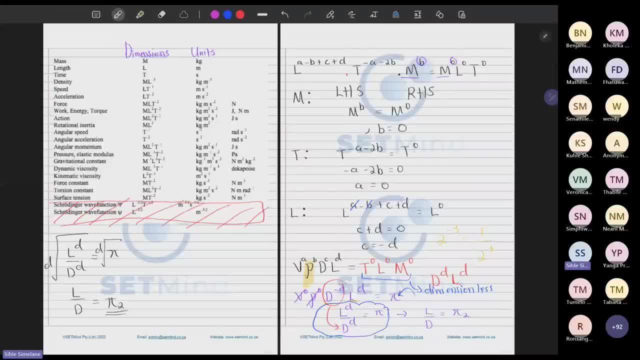 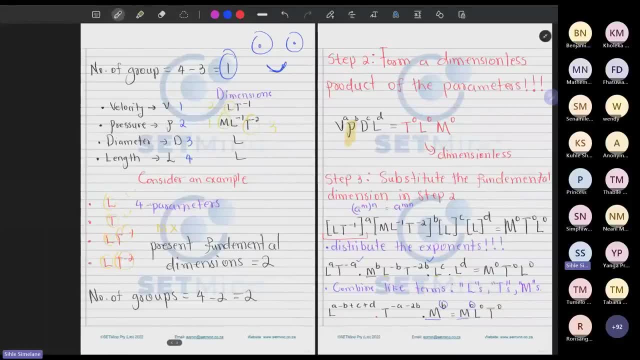 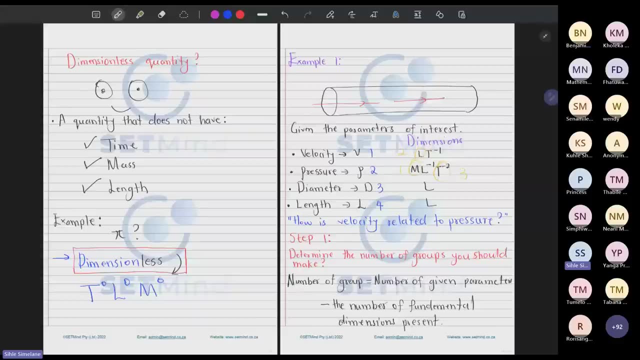 what you call. how is it related to? let me quickly look at the question. How is it related to? how is velocity related to pressure? That was the question. So the problem we are presented with here was that we had two dimensions which were geometric. 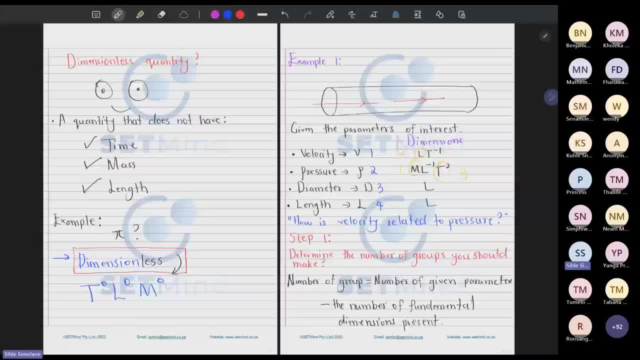 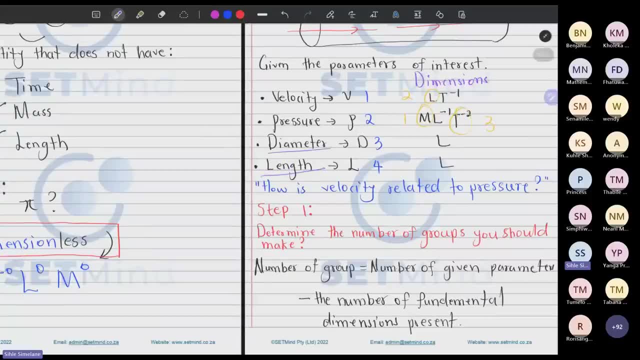 This is where you will learn about your Birkin M theorem. So, if you think carefully, length and diameter are not too different. They are not far from each other. This is the problem of this problem which we face here With these two geometric parameters. 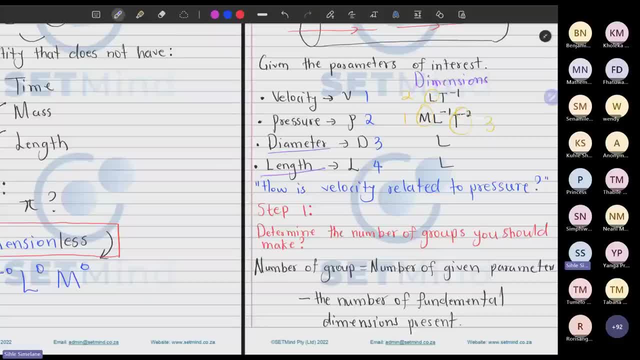 which were not too different from each other. That's where problems started. Okay, So one thing I know is they will not prevent you with the problem where you will come across two geometric parameters, especially when they want a relationship between two of them. 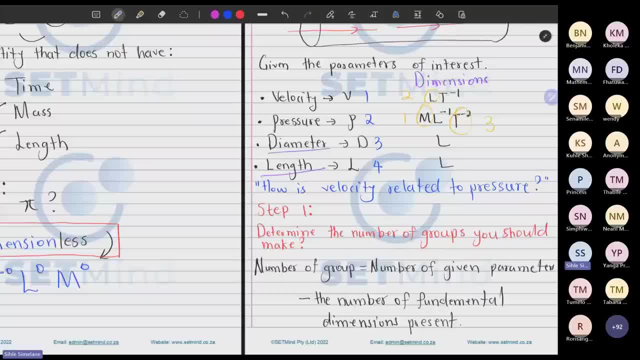 because how we deal with them is using the Birkin M theorem. So if, for example, we take the same problem and remove, let's say, length, and put in force- which I think was last year's tutorial too- you then 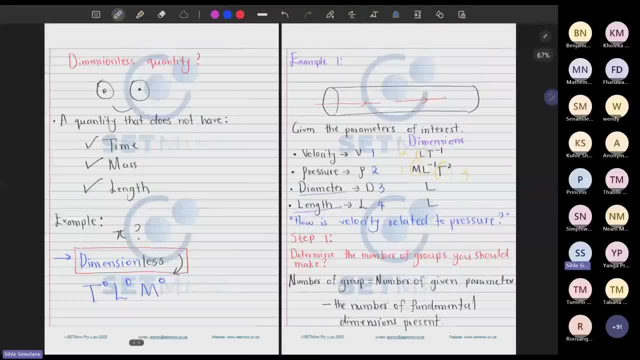 the problem then becomes easy, really easy. Let me show you what I mean. So let's copy this example and make it to be example two, And after this example, I am tempted to believe, if you understand it, sorry- you will be able to go easy. 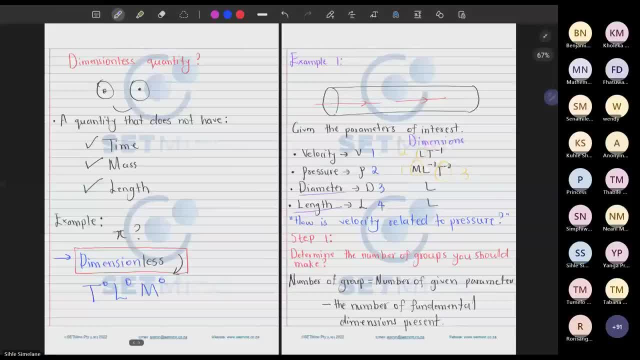 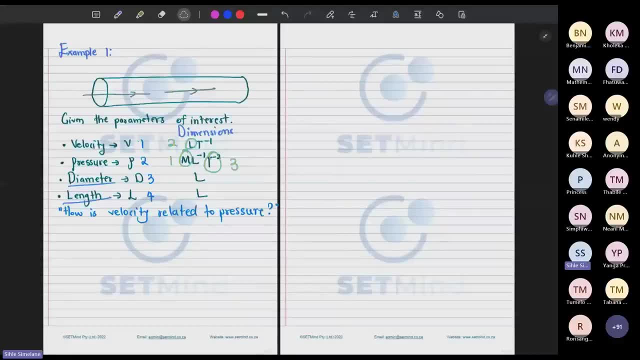 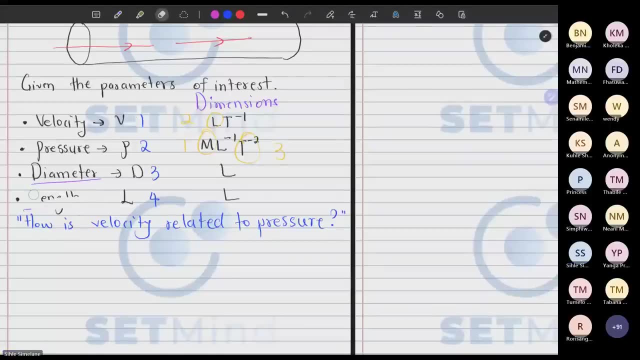 for the next two weeks or so. So let's come here and then paste. The question does not change. The only thing we are doing is we are introducing force and remove length, because there's the force which this must be pushed. So let's put in force here. 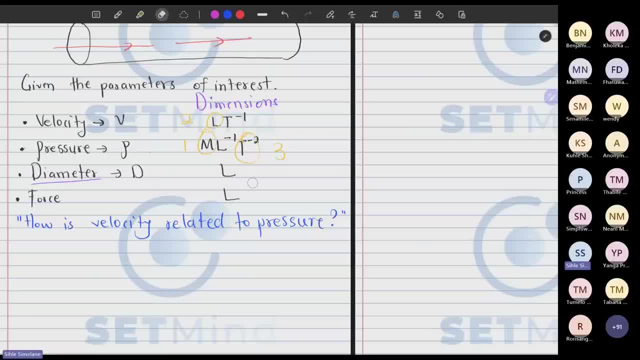 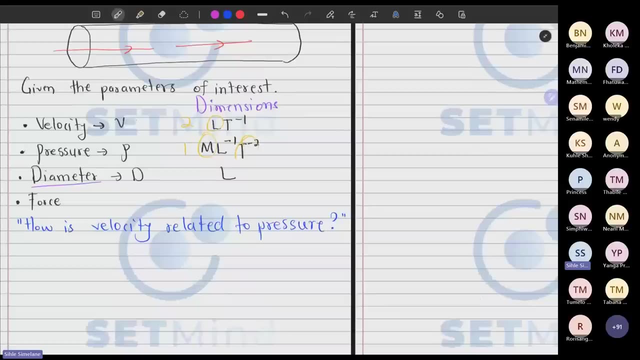 And then you'll see how this works. So someone please give me the dimensions for force, And then let's speed up the process. for this one, Let me call it example two: Someone give me the dimension for force, Let's go. good people. 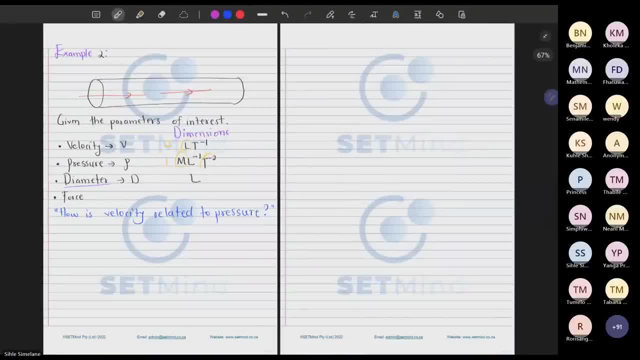 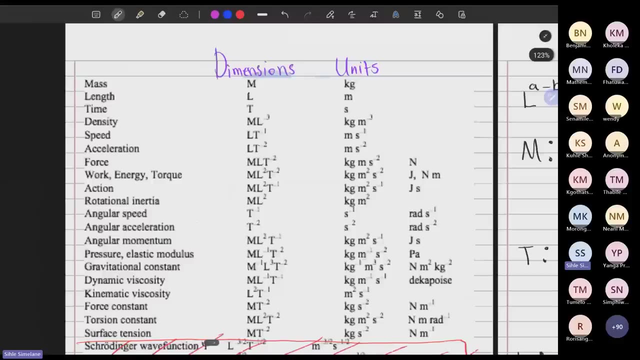 What are the dimensions for force: MLT to the power, negative two: MLT to the power of negative two. Let's quickly confirm with our table. Where is it? Force, force, force. There it is. MLT to the negative two. 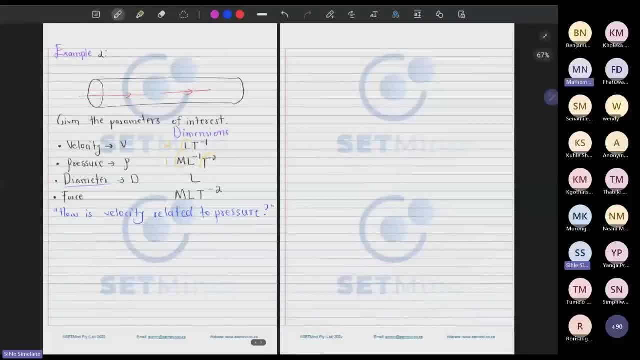 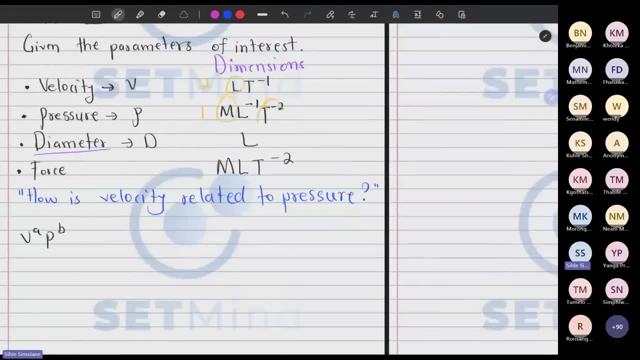 You should know this by heart. And then we do exactly the same thing. We need to form a dimensionless product, which means we need to have V to the A, pressure to the B, diameter to the C, force to the D. 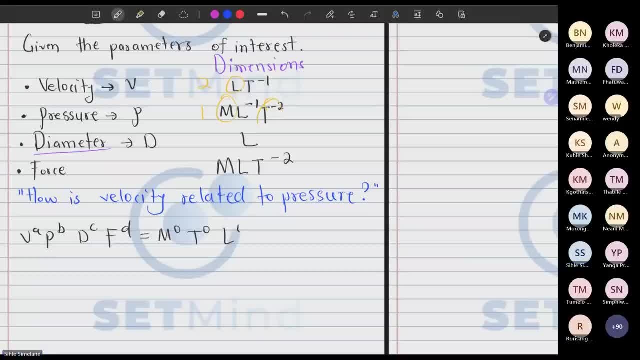 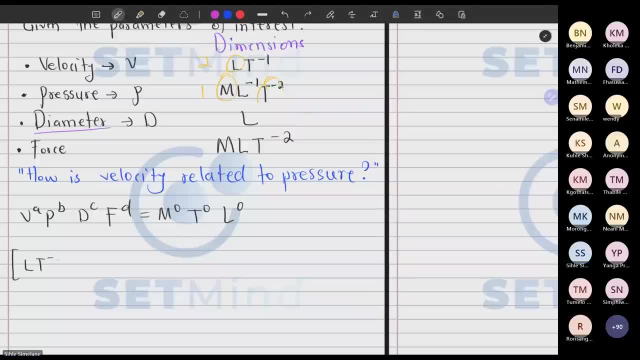 And this should give us T zero, T zero, L zero. Okay, This we have done before, Let's quickly do it. LT minus one, That's four velocity to the A Pressure. we have M, L minus one, T minus two. 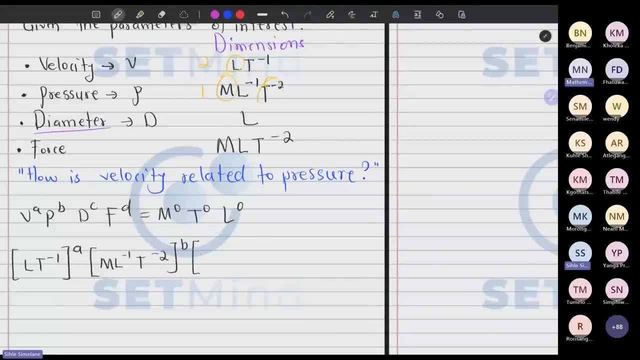 to the power of B, Diameter is L to the C, Then force MT minus two T MT. 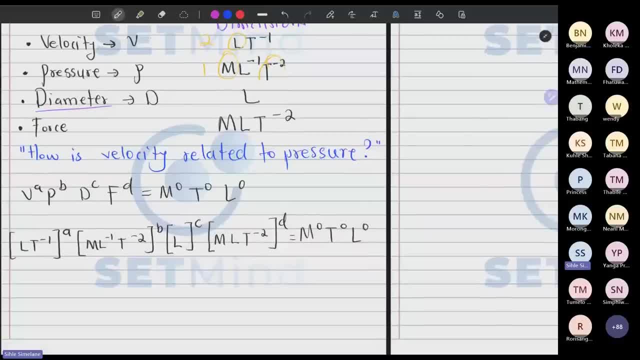 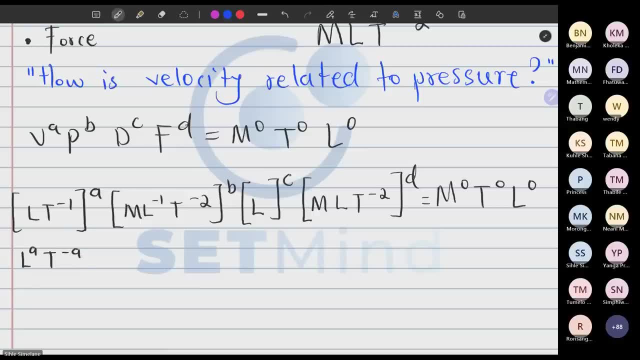 m to the d l to the d t to the minus 2 d, and this will be m 0, t 0 and l 0. okay, this is what we have. 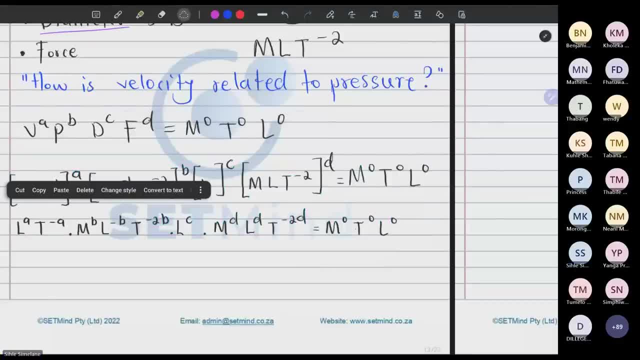 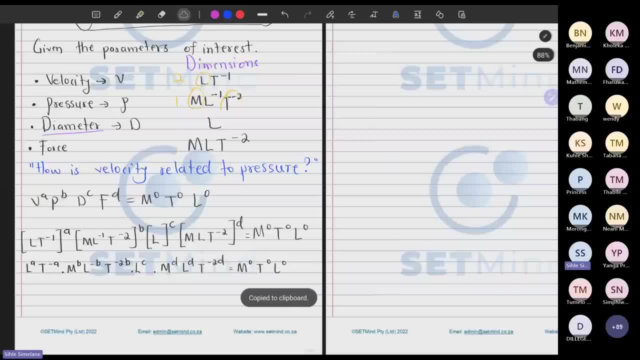 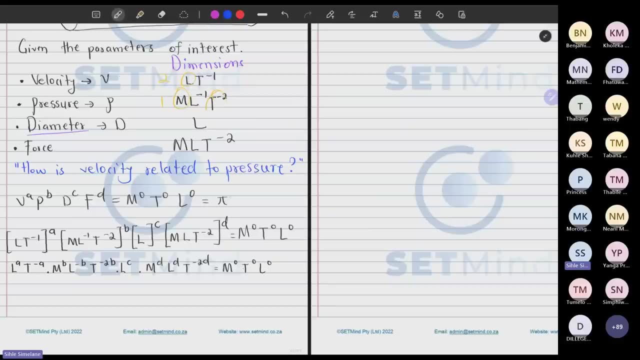 and then let's go to the next page and try to figure out and solve for the l, for the a, b, c and d, because that's the whole aim here. we are trying to solve for the a, b, c and d, because this here is a dimensionless product. we'll just equate it to pi, where pi is just constant, which is: 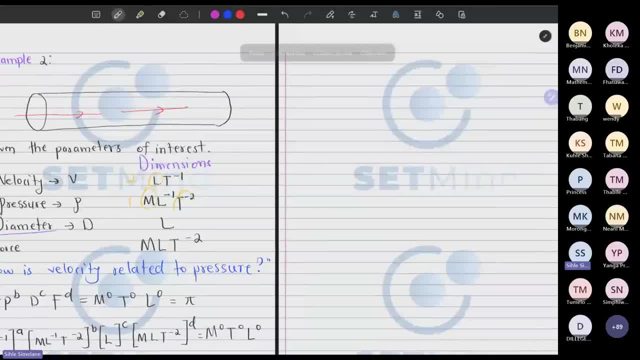 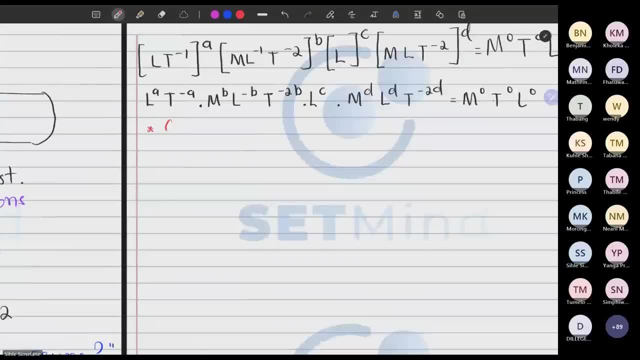 dimensionless, come here and paste and then start collecting the terms. so let's call it collect like terms. so if you look at when we collect like terms, we look at the l first. l will be to the power of a minus b, plus c and then plus d. okay, we are done with l, so let's erase it and then let's go to. 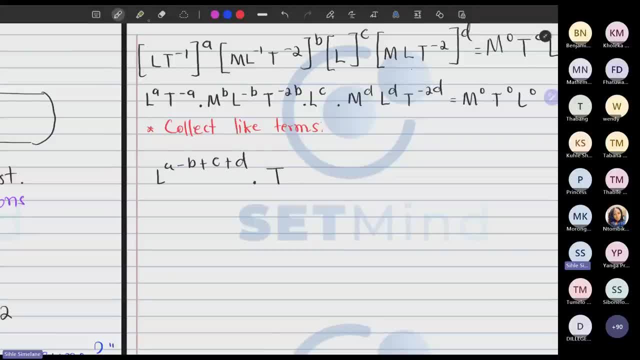 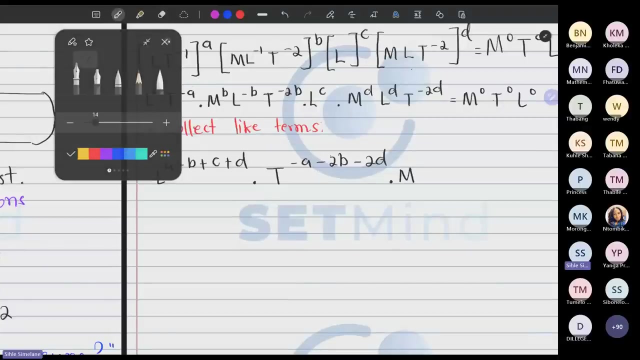 t dot t. and if you look at our t, we have minus a. it is minus a, and then it is minus 2b and then it is minus 2d. we are done. then let's look at m. erase these ones. where is our m? our m has a b. 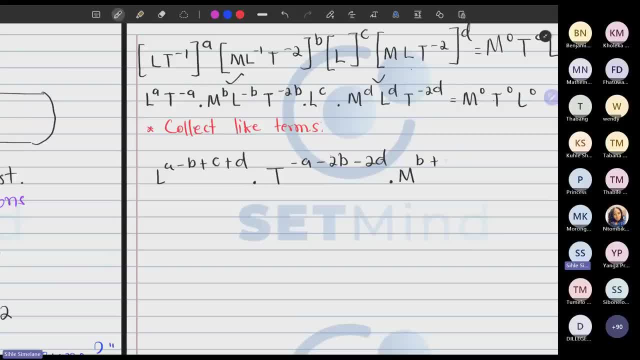 and the next m we see has a plus d, it's a positive d, then this should be equal to m0, l0, d, t0. okay, and then now what we do is we simply compare the m's, compare the l's and compare the t's. 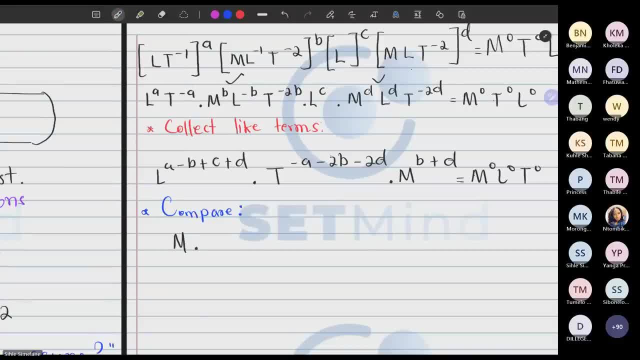 so let's see, let's start with the m's. so if you look at the left hand side and you look at the right hand side, the left hand side, we have m to the b plus d, then the right hand side, we have m to the zero. it will always be m to the zero. 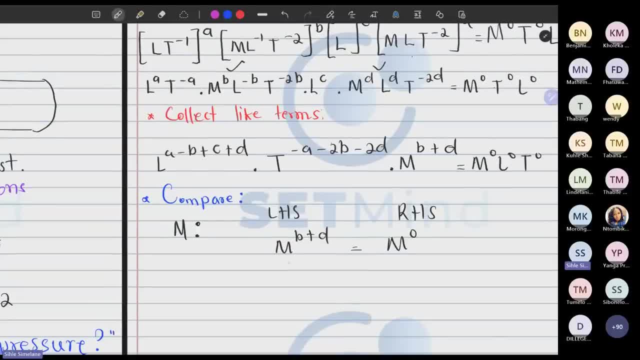 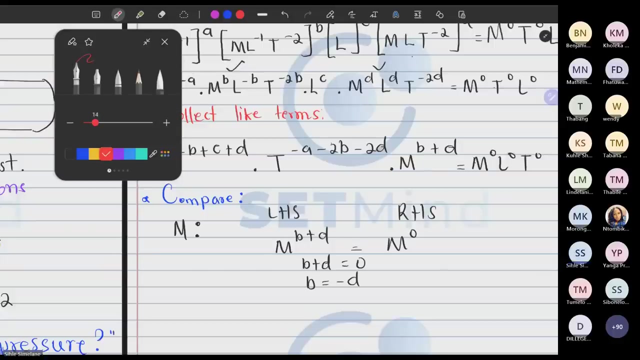 okay, and then now what you should be looking at is high school, same base. we equate the exponent, so that means b plus b is zero. that means b is equal to negative d. okay, and then the easiest thing you can do is to choose one. you see, for example, here the relationship is saying b is negative d. 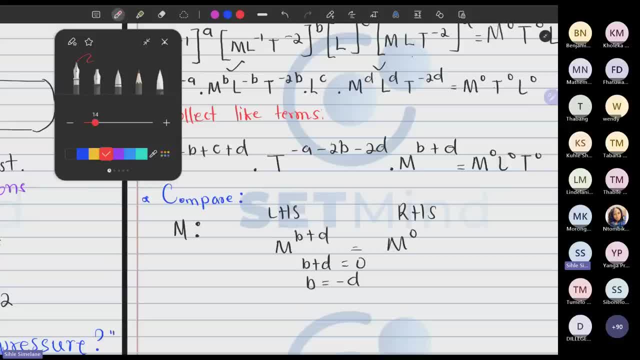 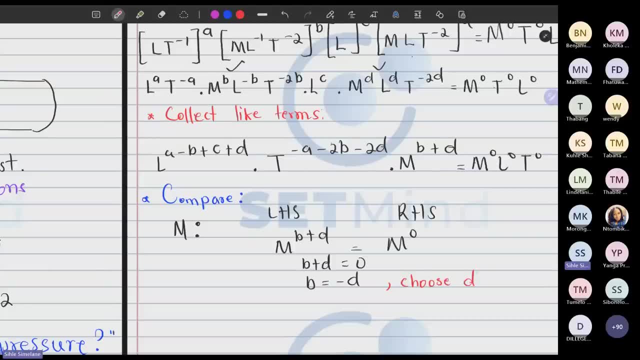 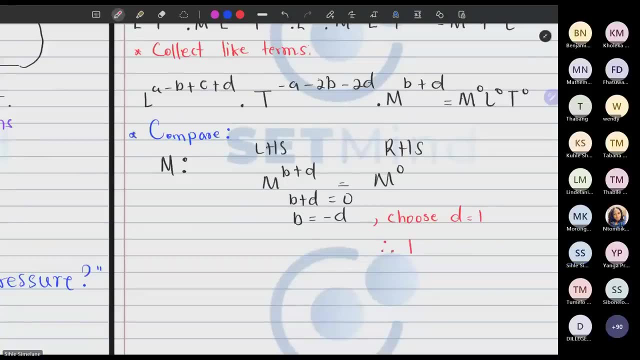 so what you can do, the easiest thing is to just choose one. okay, so you can choose. let's say your d to be one. then, when you choose your d to be one, therefore, your b becomes negative two times minus one. okay, let's leave them like this. let's carry on and look at the t, or let's look at: 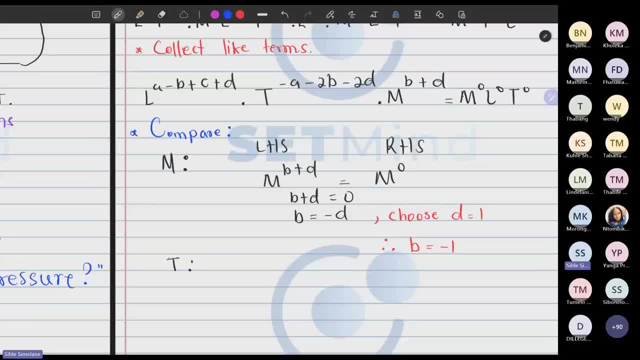 t. yes, let's look at the t one. so for t on the right hand side. on the left hand side we have negative a, negative two b, negative two d. on the right hand side we have t to the zero, same base. we equate the exponents. so that means 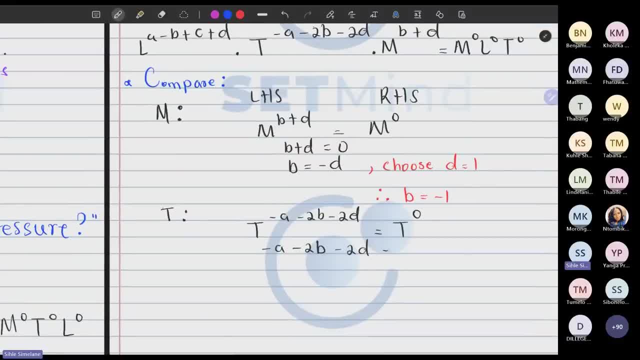 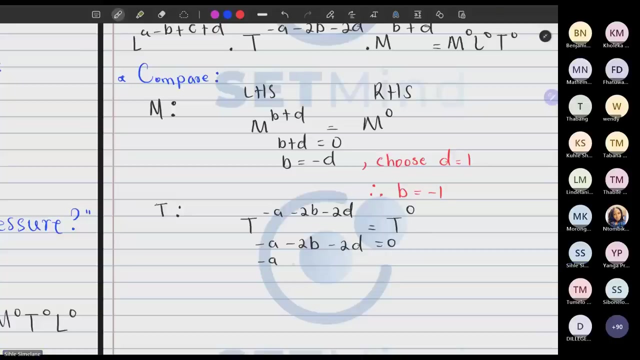 negative a minus two b minus two d is zero. okay, but already we have our a and we also have our. we have our d and we have our b. so if you look carefully, what we do not have is a here. so if we have negative, a will be equal to two b. 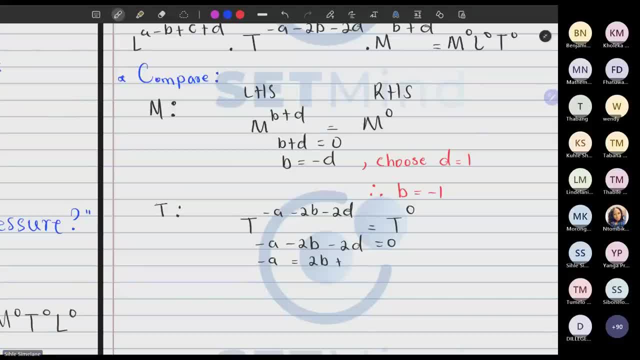 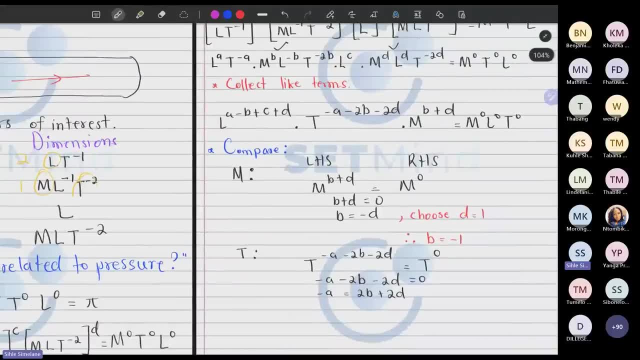 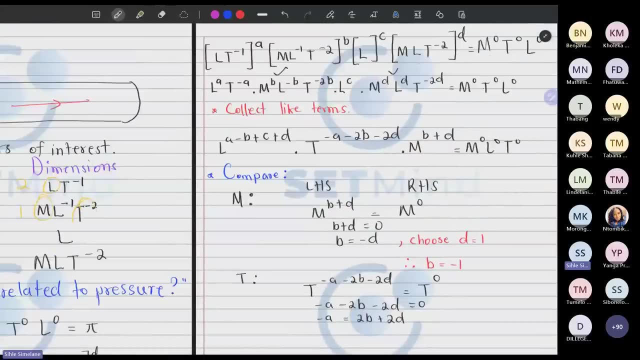 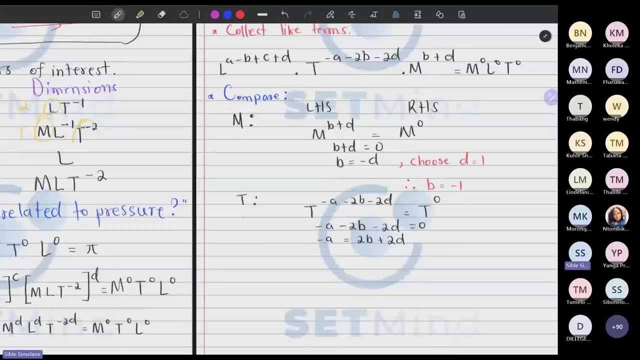 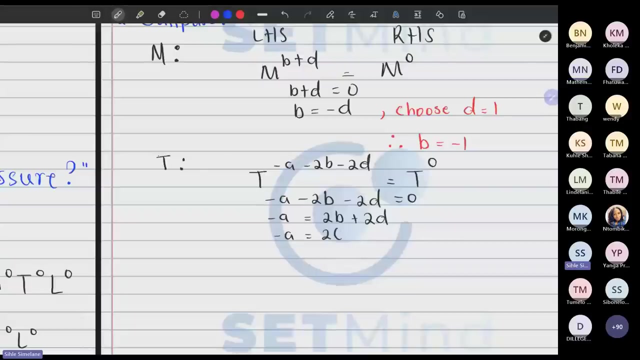 and then plus- let's see this- plus two t. let me quickly check if we are making no mistake here: minus that two t, minus that. okay, that's what we we have. so, if you look carefully, our a will be negative 2b. we chose our b and d there, so our negative a will be two times. our b is negative one plus two times. 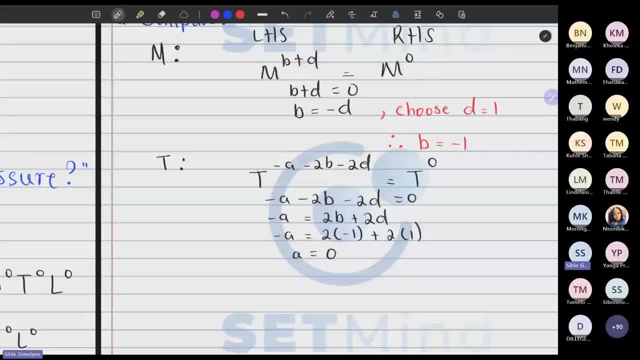 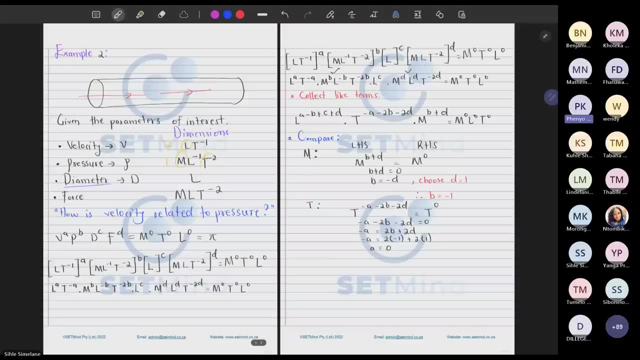 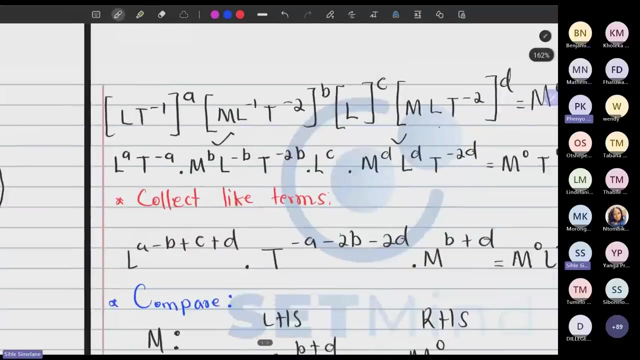 our d is one, so our e will be zero. do you have any questions? yes, sir, um, for m do we have like m plus d, or i mean m to the power of b plus d or m to the power of b minus d. let's quickly see for m, yes, for m, at the m here. so for m we have the power b. 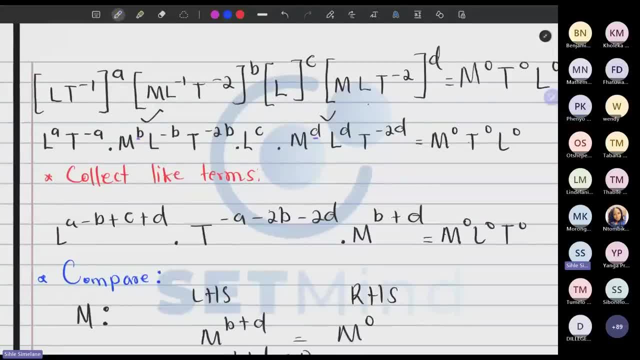 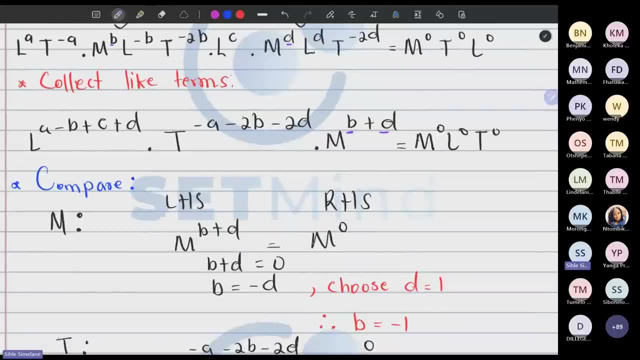 then we have. so that means we have b plus d, b plus d. and then the right hand side, it is m to the zero. so you equate the exponents because the bases are the same. so you have b plus d equals zero. so your b, when you transpose it, will be negative d. 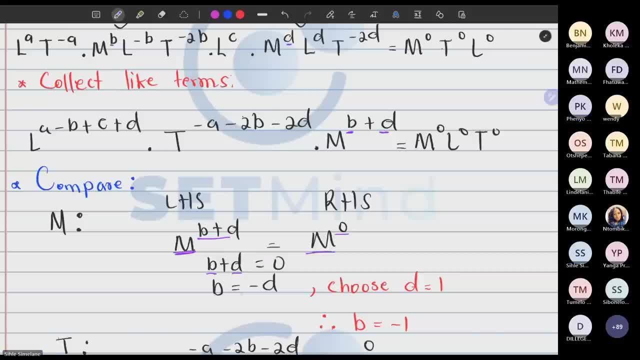 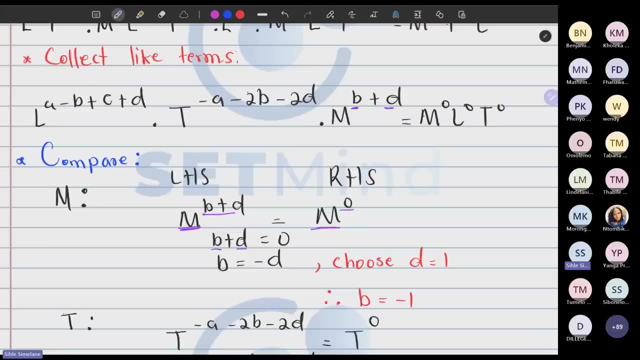 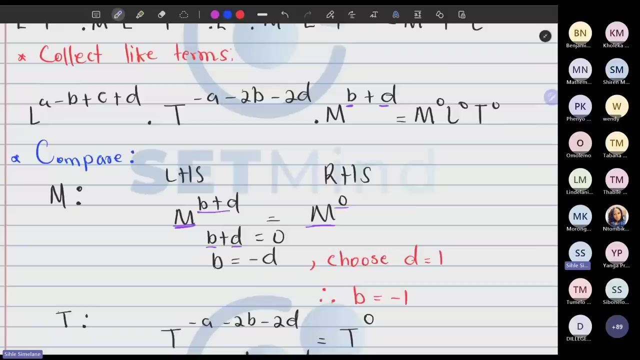 did it do? did i answer your question? um, isn't it like d minus 2d, um negative d? let me see: d minus 2d, negative d? um what we are saying? um for, for the power of m, for the power of m, so for m. 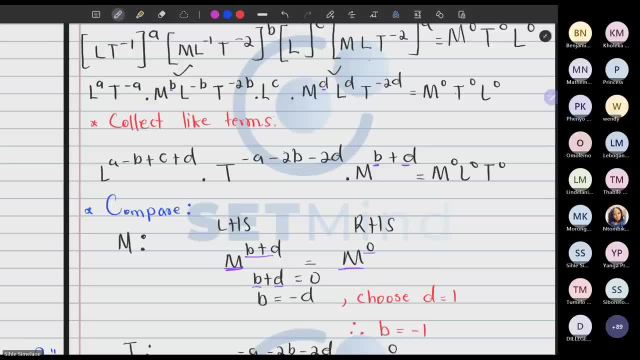 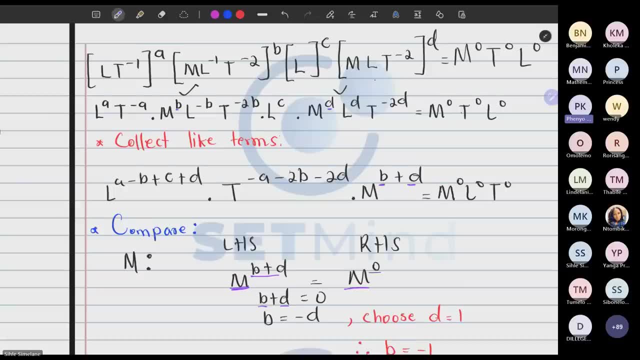 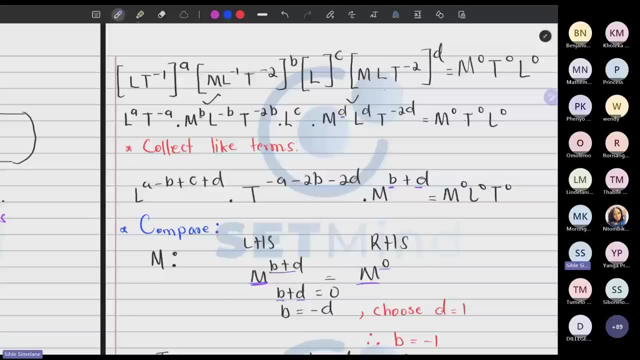 yeah, yeah, so we have m to the b right, and then another m is m to the d. oh no, i understand now. so you can just add the. so, if you look carefully, our a becomes our zero and then we can now go to the t. we have the t, we have the l, we need to go to l now. so if you look at l for l, we have l to the a minus b, plus c plus d, and this will be l to the z. 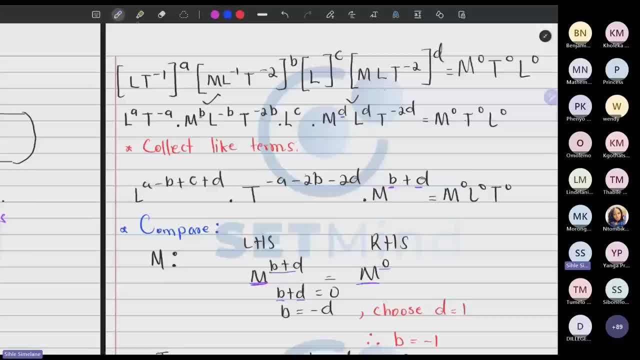 so if you look carefully, our a becomes our zero and then we can now go to the t. we have the t, we have the l, we need to go to l now. so if you look at l for l, we have l to the a minus b plus c plus d, and this will be l to the z. 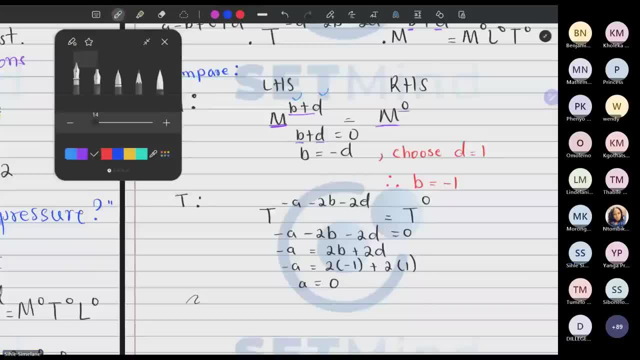 so, if you look carefully, our a becomes our a becomes our zero, and then we can now go to the t. we have the t, we have the l, we need to go to l now. so if you look at l for l, we have l to the a, minus b, plus c, plus d, and this will be l to the z. 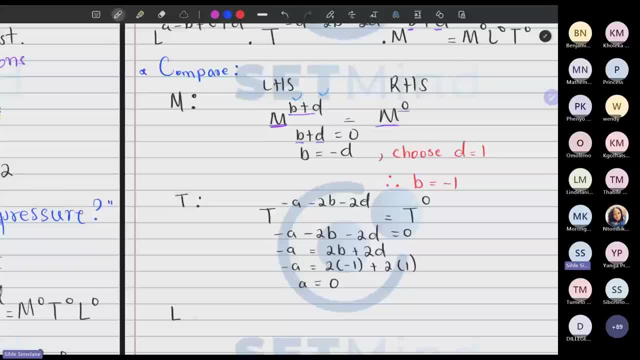 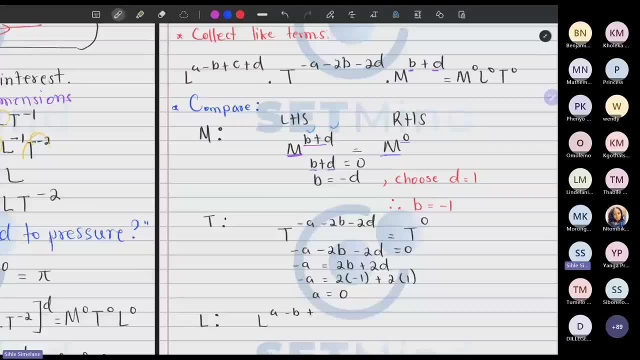 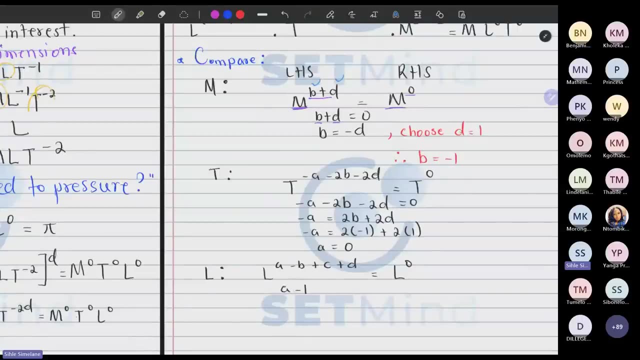 so if you look carefully, our a becomes our zero and then we can now go to the t. we have the t, we have the l, we need to go to l now. so if you look at l for l, we have l to the a, minus b, plus c, plus d, and this will be l to the zero on the right hand side. so our a we already have as zero. so we have our a minus b, plus c, plus d, equaling zero. same base. you equate the exponent. so our a is zero, so we have negative. our b is minus one. and then we have our a minus b, plus c, plus d, equaling zero, same base. you equate the exponent. so our a is zero, so we have negative. our b is minus one. and then we have our a minus b, plus c, plus d, equaling zero. same base. you equate the exponent. so our a is zero, so we have negative. our b is minus one. and then we have our a minus b, plus c, plus d, equaling zero. same base. you equate the exponent. so our a is zero. so we have negative. our b is minus one. and then we 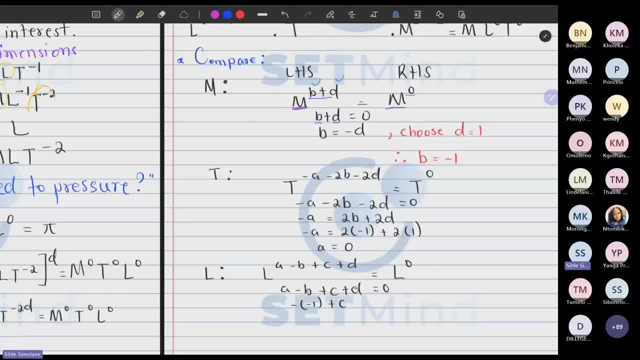 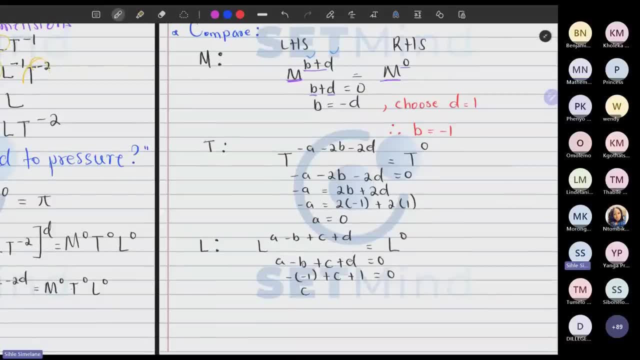 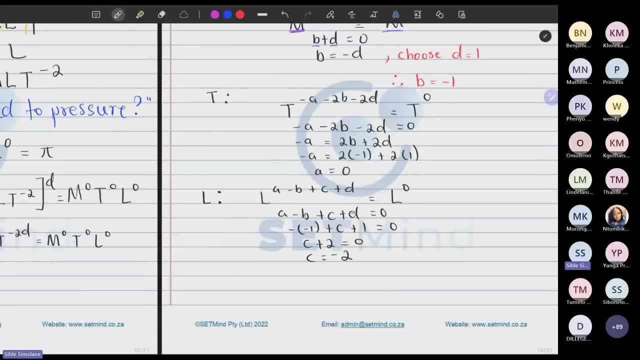 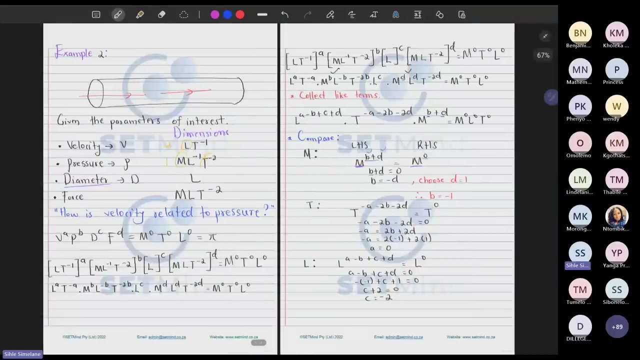 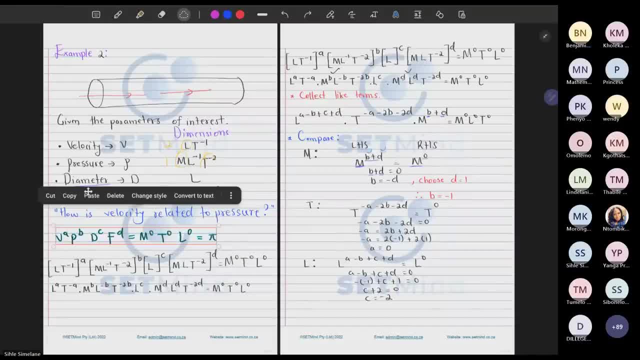 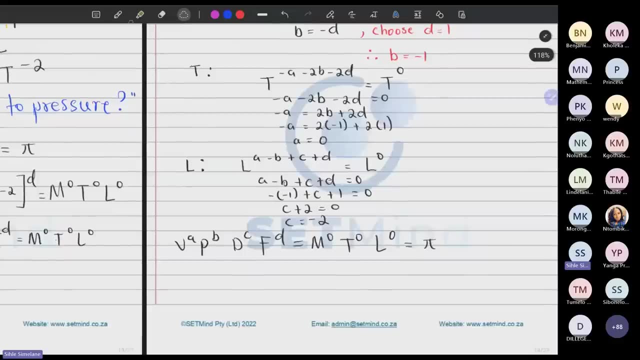 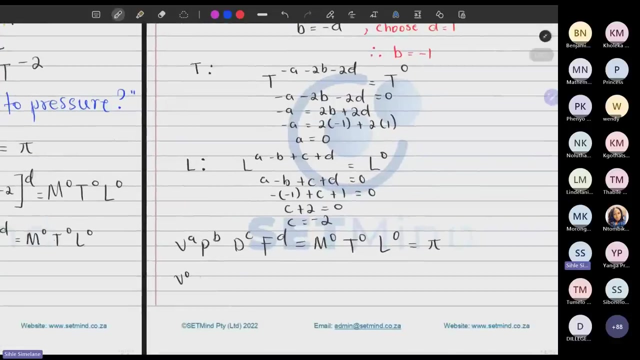 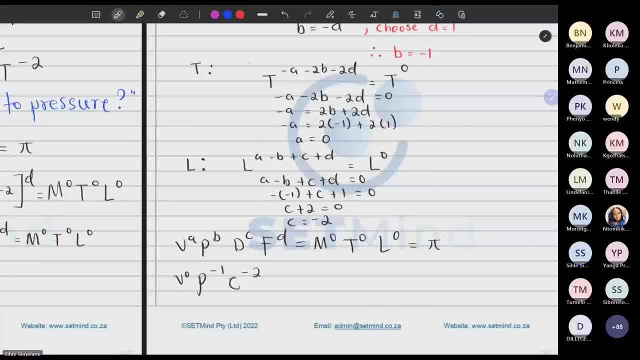 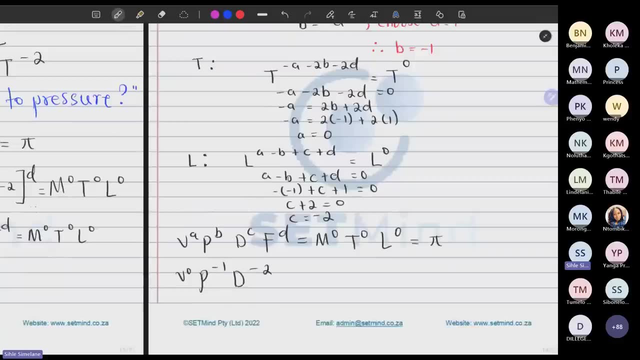 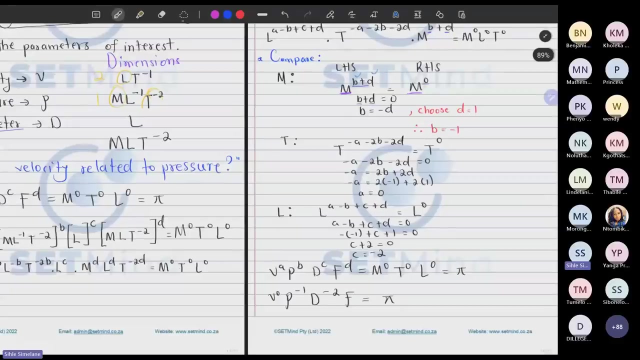 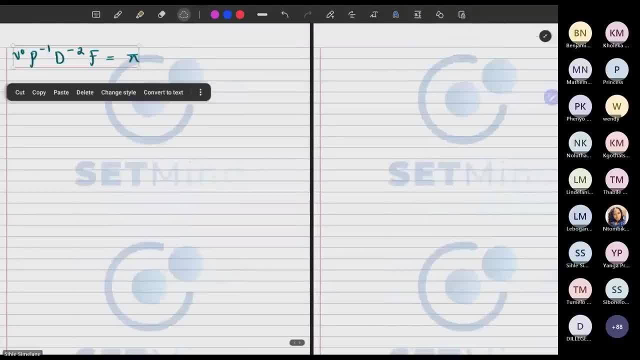 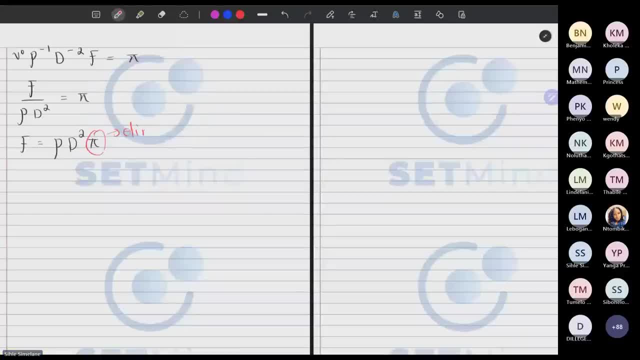 is a dimensionless quantity, Mentionless quantity. So in other ways you can think of pi as a proportionality constant. So if you look carefully, what we are able to find is the relationship between force and pressure. So our force is just given by the pi. I can just 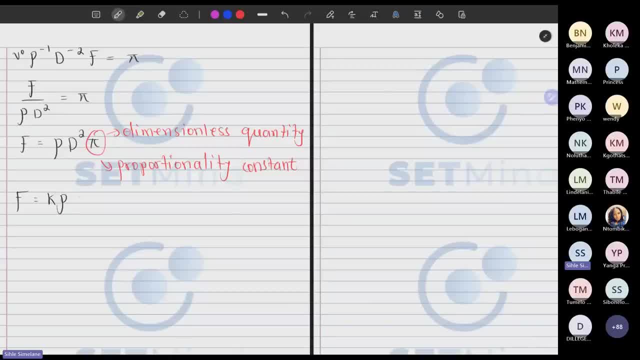 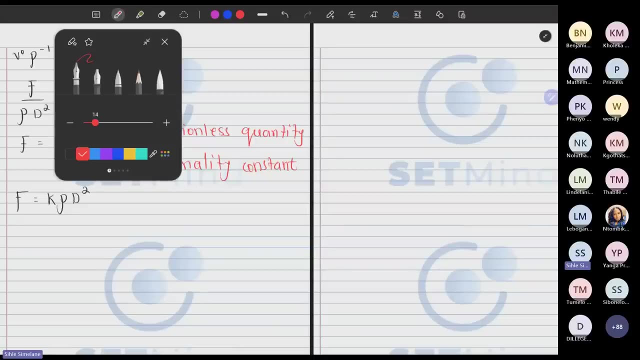 call it k, which is just the proportionality constant times the pressure, then the diameter squared. So which means this is the relationship we could afford to give them to say: look, I do not know much, but I know that the force is directly proportional to the pressure. 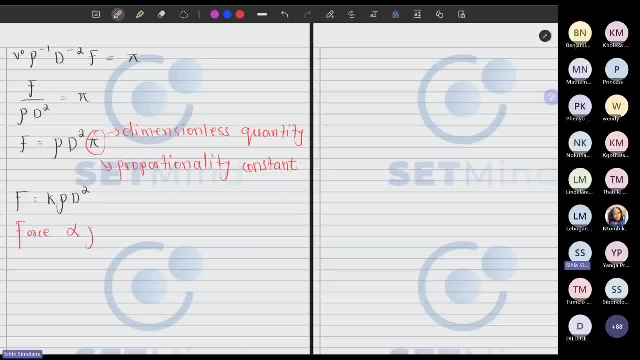 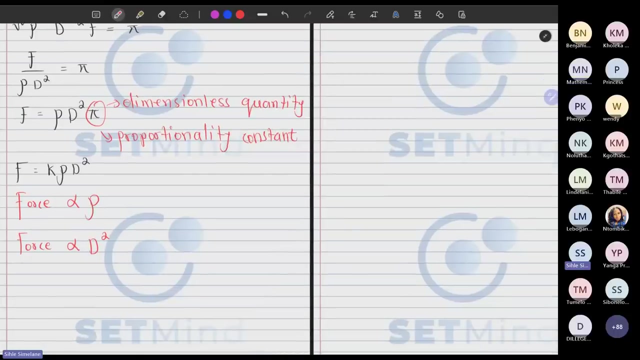 So meaning an increase in force means we are increasing the pressure. And also you can tell them that the force is directly proportional to the diameter squared And then, equally so if they are looking for a different relationship, the pressure, when you divide, you can see. 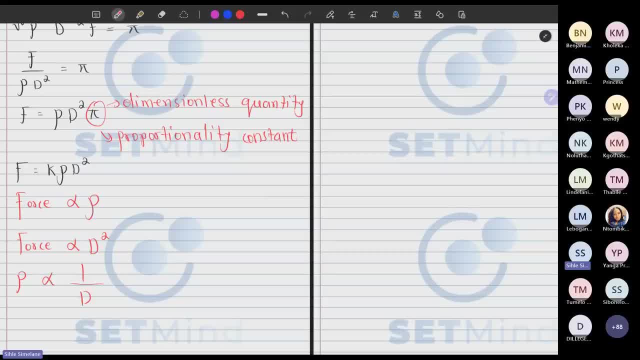 that it is inversely proportional to the diameter squared. So if you look at this, you can see that this is a very important dimension for the temperature in the experiment. So I am going to try to solve it with this question. So if the force is directly proportional, 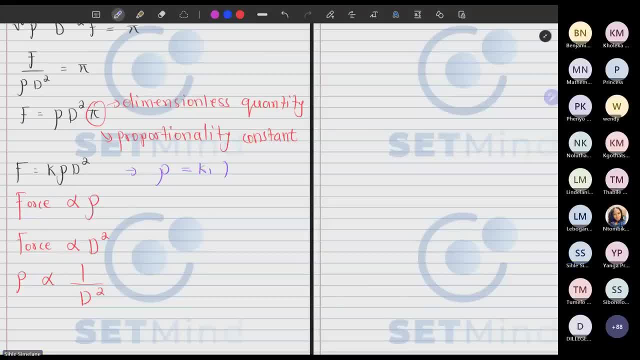 to one over the diameter squared. So meaning when you increase the diameter you are decreasing the pressure, But when you decrease the diameter you are increasing the pressure. Because when you try to solve for diameter here or for pressure, sorry, you will see that pressure. 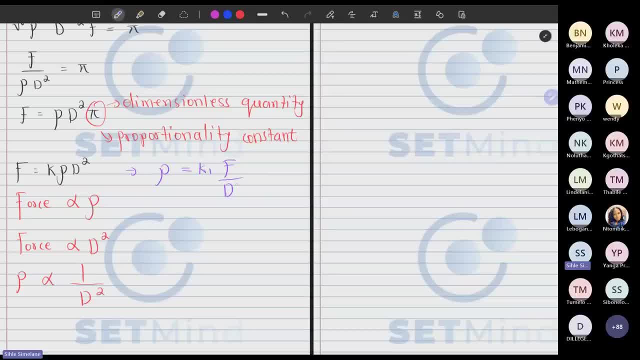 will just be another proportionality constant than force over diameter squared. So you can see that pressure is a better thing than force over diameter squared. So if you give inversely proportional to the diameter squared, and this makes intuitive sense, if you have a pipe and you are trying to push something inside, 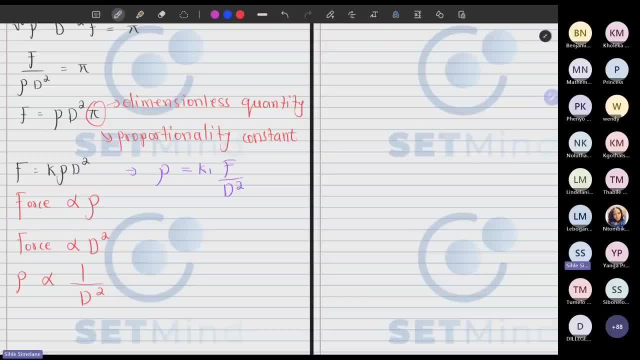 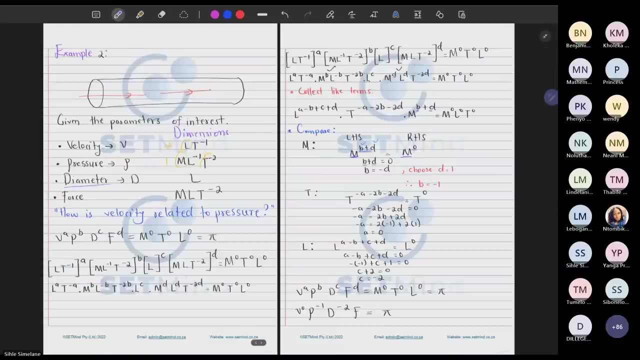 if you, let's see if you decrease the diameter, you are increasing the pressure. okay, do we have any questions? I want to ask on the previous example. we did: yeah, so there, when they wanted to, they said: compare, let me check. they said: how is velocity related to pressure? did we answer? 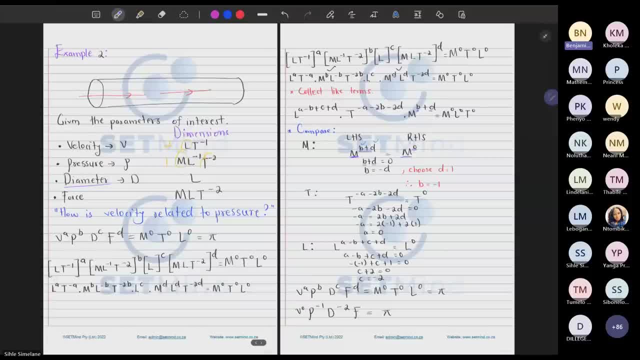 the question. did we answer the question or was there anything? so here's what's going on there. so I formulated the question myself. there's one mistake I made then, which was there were two geometric quantities, so, but it's not something you should. you should stress about in the question. they 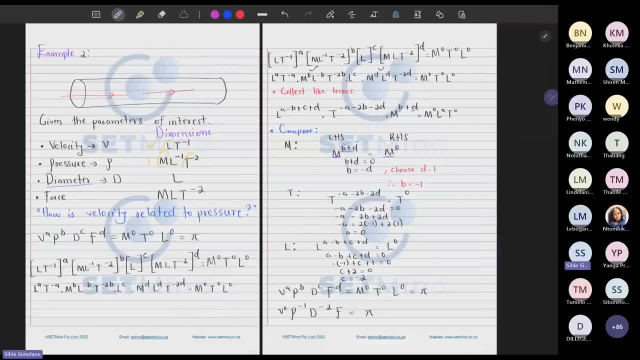 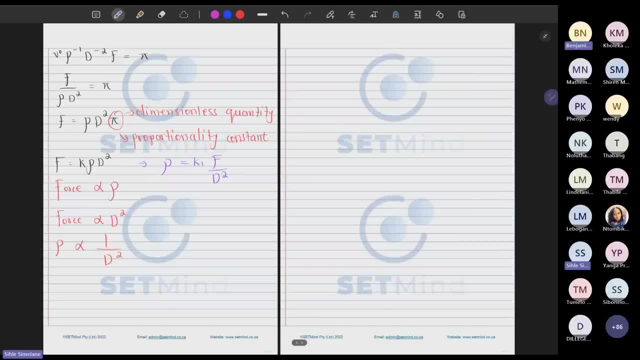 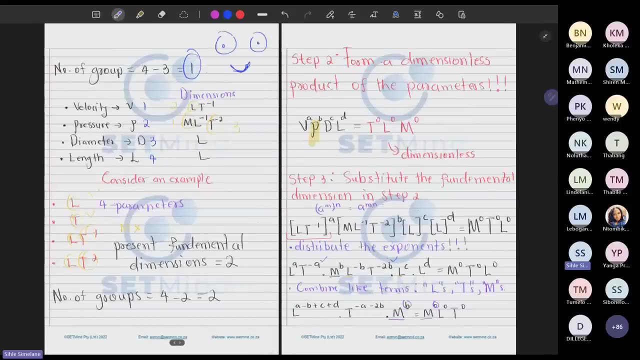 will never give you a question, which you should not do, but to give you understanding, there's a quantity which you call geometry, and then there's flow, and then there is, I think, there's, there's geometry, there's flow. I forgot the last one, so I had two geometric quantities here: geometric. 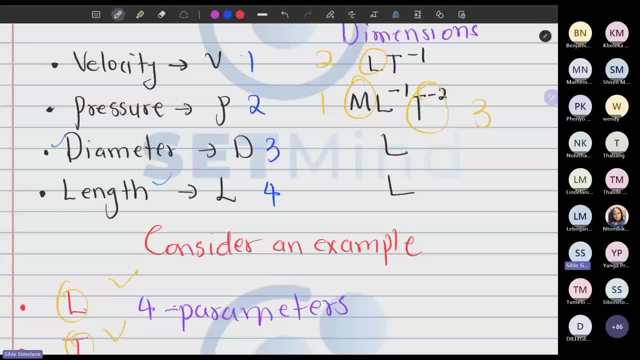 diameter is geometric and length is geometry in phasor. I forgot what they call it, but velocity is related to flow, so I had two dimensions which fall on the same glass. that's where the problem became, because they need to eliminate one another, so they made the others to be. 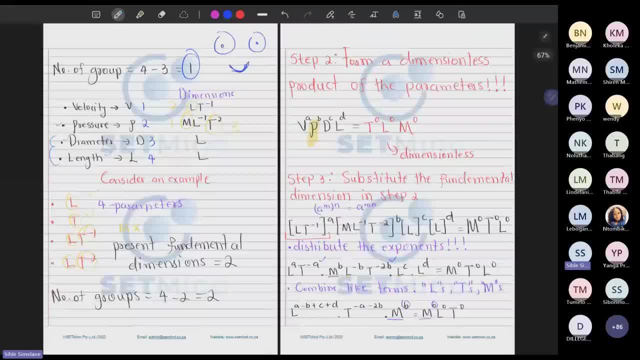 zero. so what I'm saying to you is: do not stress about encountering such a problem, because when they phrase their question, they will not give you dimensions which fall on the same glass, which will present you with the problem which we we had. so I thought of it in advance. 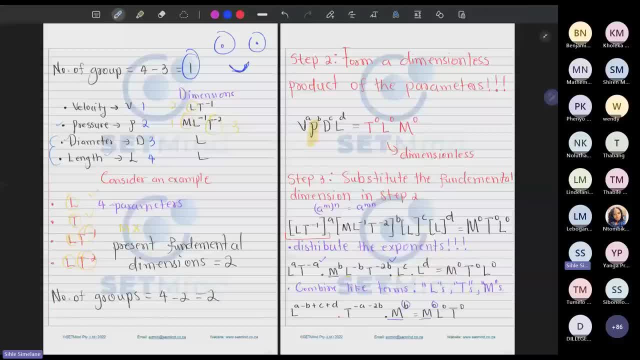 two geometric parameters or a class of parameters which fall on the same class. okay, so then we're going to go to the next slide. okay, so then we're going to go to the next slide there when you uh, yeah, yeah, yeah, yeah. so if you can check, say when on the last. 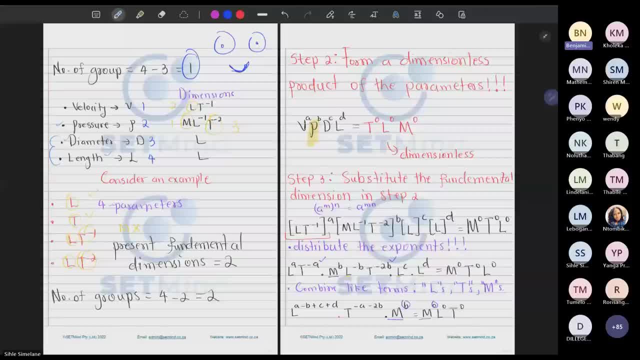 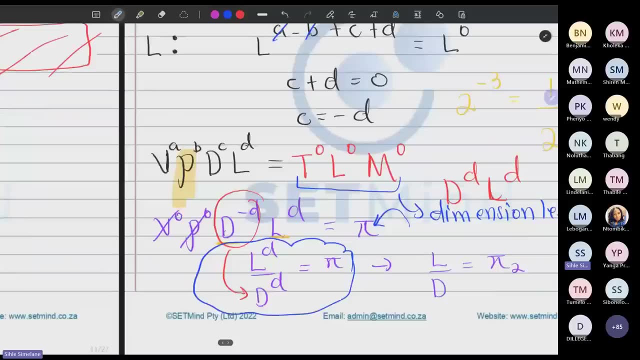 part on that problem. when you say l to the d over d to the d, yes, yeah, yeah, these geometric parameters, they wanted to eliminate one another. so when you have length over diameter, it becomes a dimensionless quantity. so in essence, we have achieved that, but the only problem is: 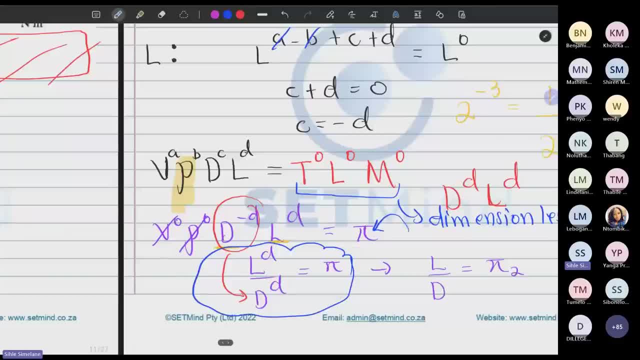 that we have not made a good combination. these quantities combined with the ones we've given, they didn't make a good combination. so for for the current one that we were on, can I like conclude that the ones that we want to compare, we must assign them to, maybe, a value. 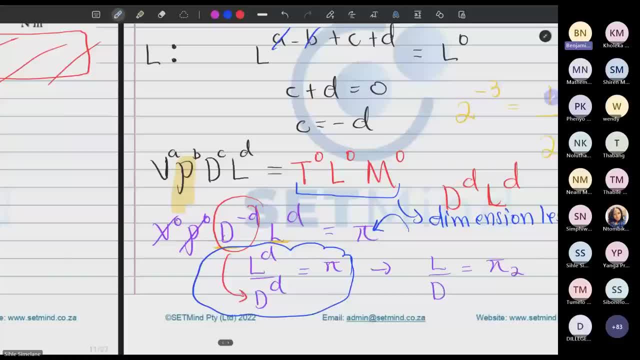 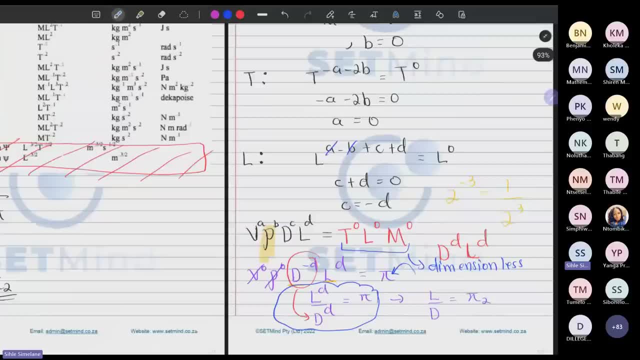 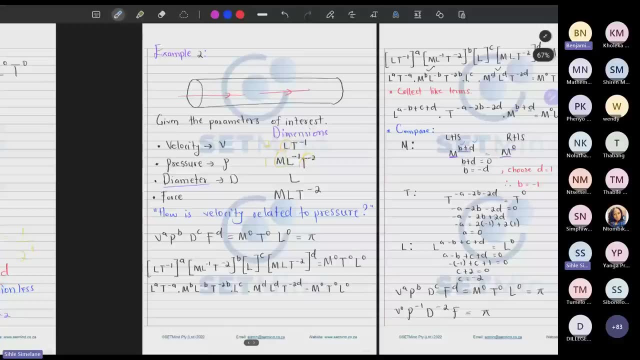 such that you say, choose d equal to 1, so that at the end we can sort of like compare, uh, force and pressure. anyway should do um, in fact, you, you are very smart. let me say that first. let me copy this, let me copy this. so look at what he's. he's saying um, the question here we are trying to look at, 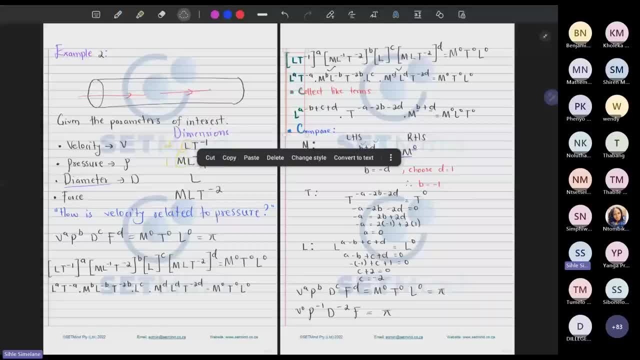 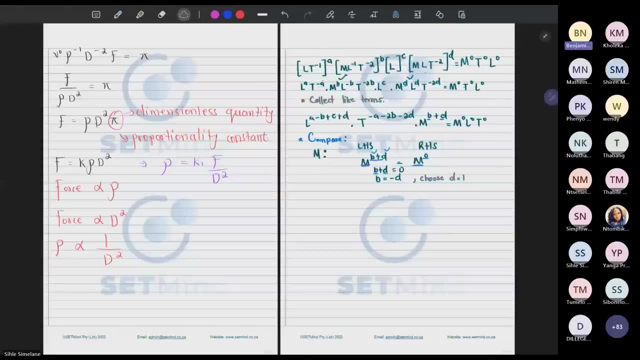 pressure and velocity. let's, let's copy this and let me show you something from what he's saying. what he's saying, so let's copy that, go to the next page and paste so here. i'll need you to really bear with me. so here's what we are trying to do here. 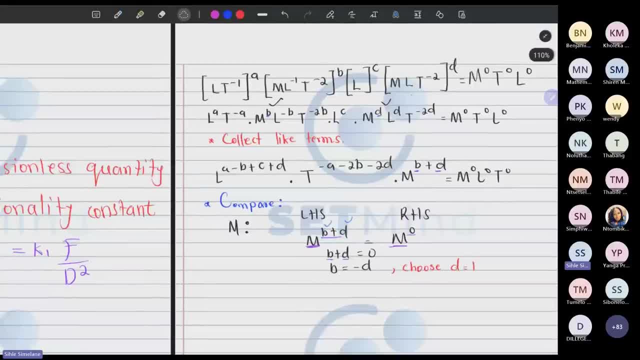 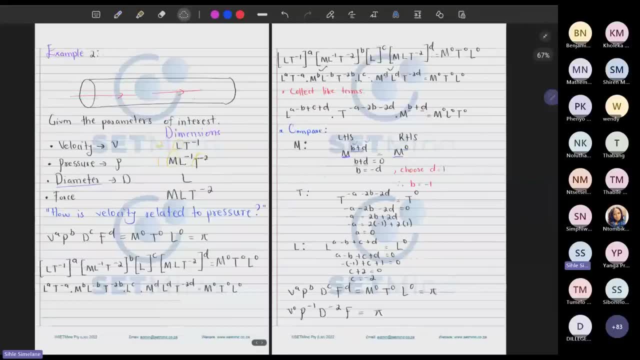 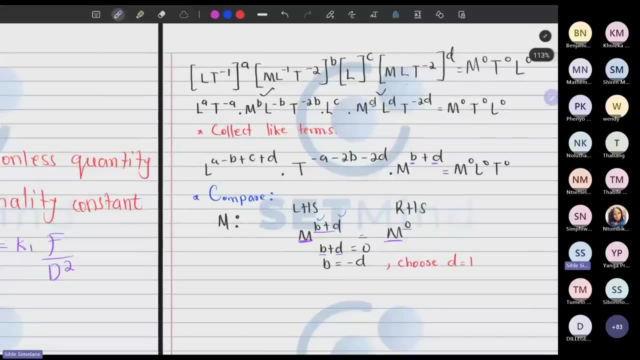 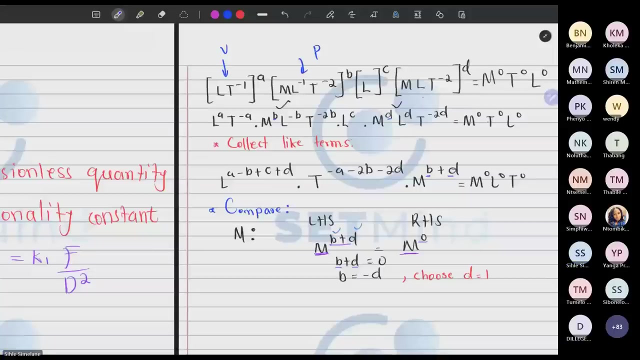 we are trying to compare velocity, and let me see where is that in pressure. so, which means what we should try to do, if you look carefully, if we really wanna be smart about things, this is velocity here and this is present here, so what we should try to do alternatively. so that was one. 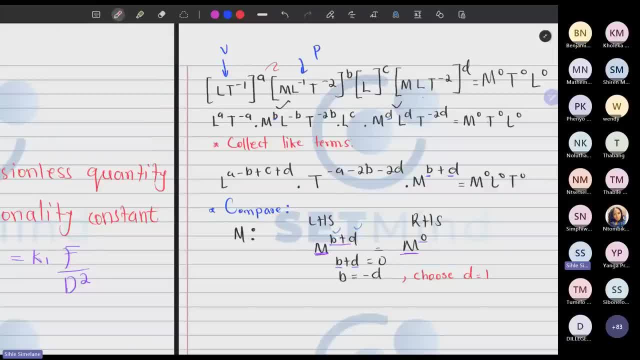 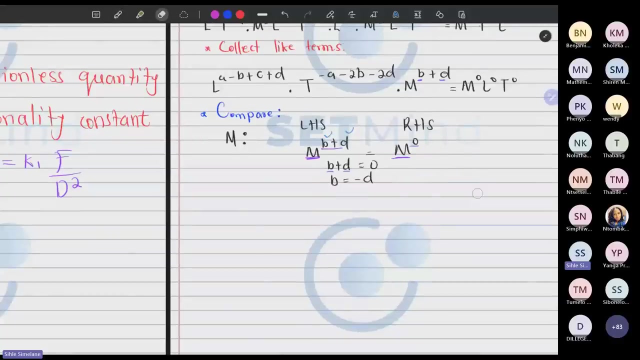 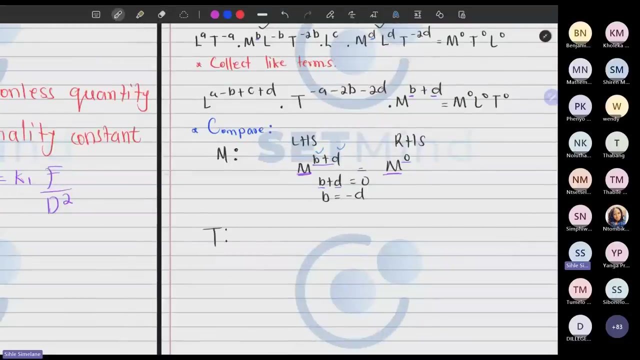 group, we should try to make sure that our a is not zero and our b is not zero. so let's come. let's come to this one and let me remove the choosing here and see if we can try to achieve that. let me copy these ones here: t- let's quickly sort out the t. so for t on the left hand. 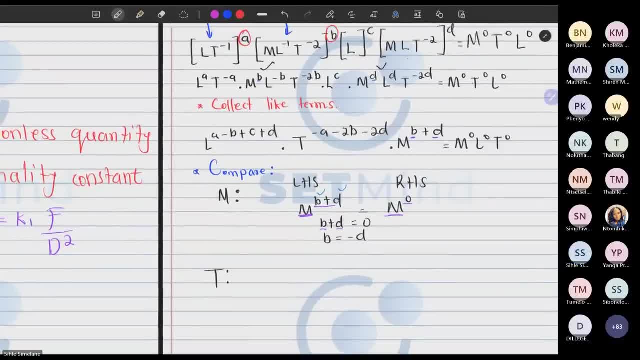 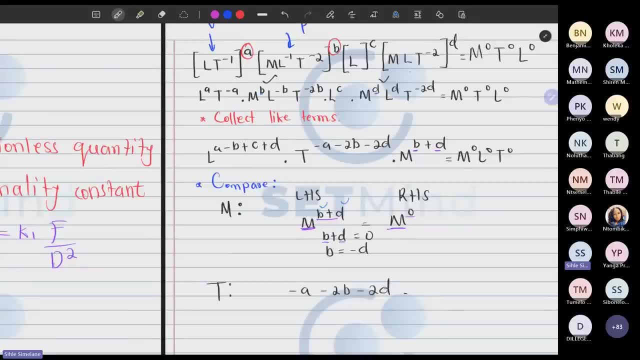 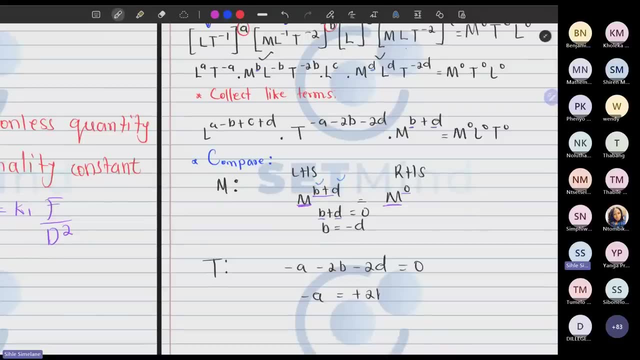 side, what we have is um, where is that? t is minus a, minus two b plus two d is zero, and then, if you look carefully, your a will simply be negative. two will be positive: two b plus two d. so the problem with this one is these will always cancel, so our a is forced. 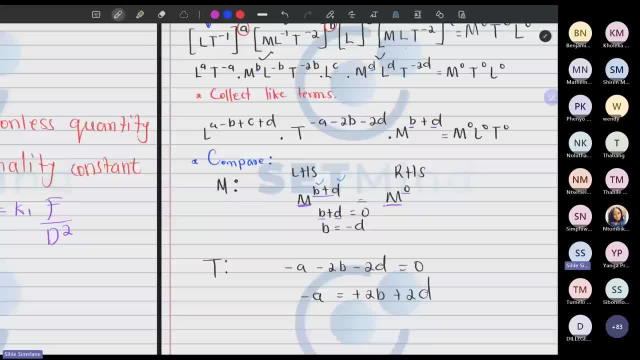 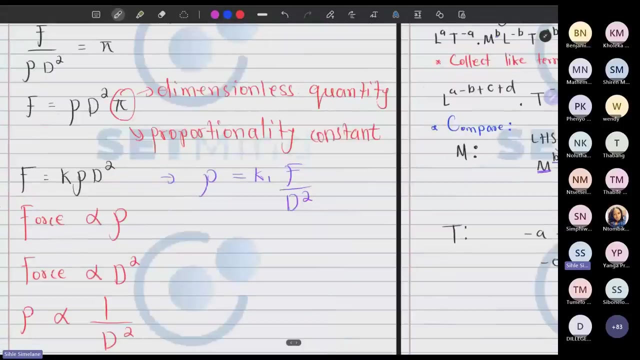 to be, to be zero. you see that, because our b is negative d, so which means finding a direct relationship between velocity and pressure is not there, actually it is not. so it's a question they would not, they would not phrase. so I thought of relating pressure and velocity, but what we can actually relate is the force, the pressure and the diameter. 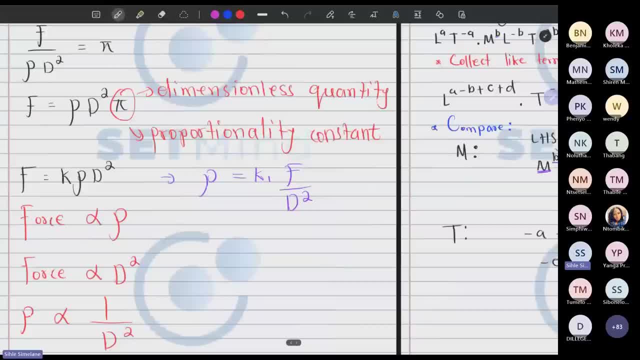 so, regardless of our smart choice here, we would eventually fall to the solution which we currently have. so I'm I'm creating examples to help you to understand and then when you have a specific case which has applied that- but believe me, you will never be presented with. 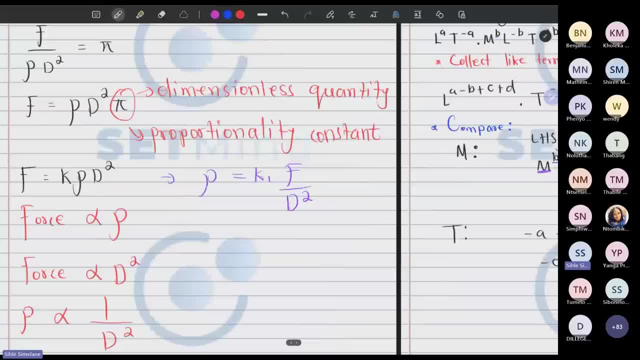 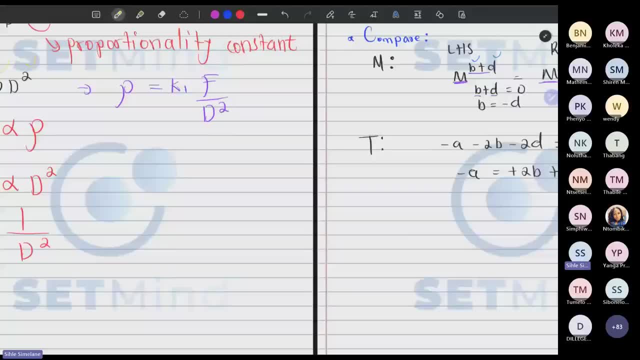 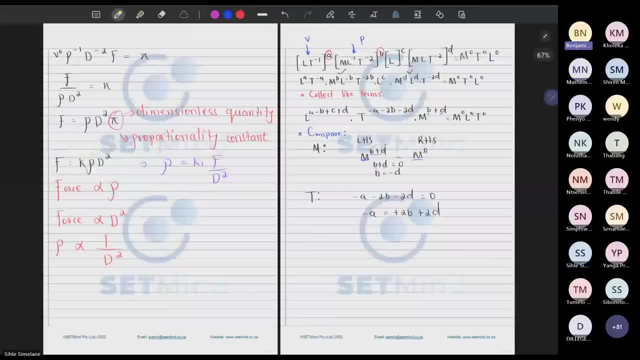 a problem which is way complicated than the what we have looked at. do you see what I'm saying, or is there anyone who sees what I'm saying? okay, so it does make sense. and, um, I have one last question. yes, what was the significance of us like 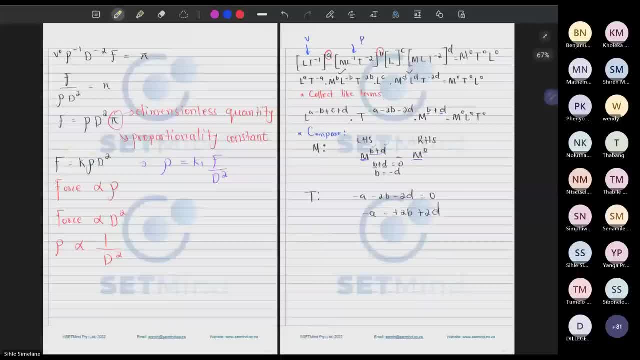 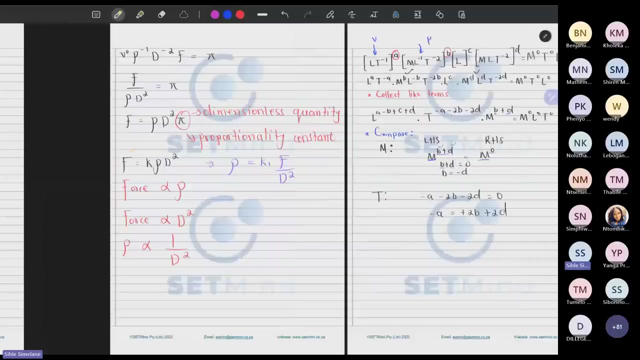 finding the number of groups. you can carry on. sorry, okay, what was your question? please ask it again. oh, I said what was the significance of us finding the number of groups? it is it is. it is because, you see, for example, it is because you can have different combinations which arise depending on your choices of values. so, if you have 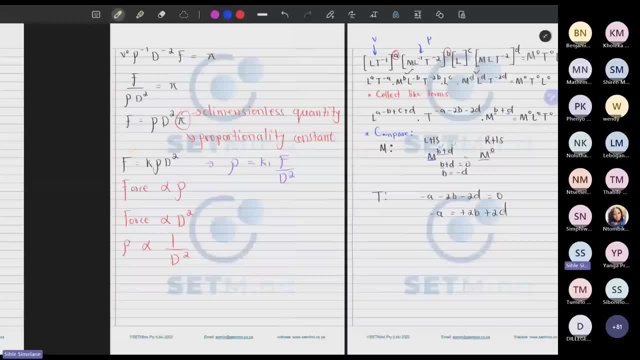 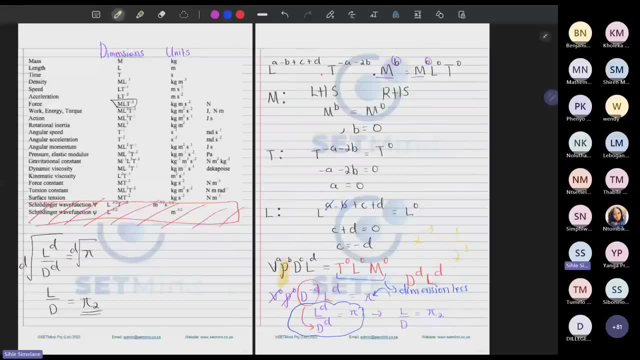 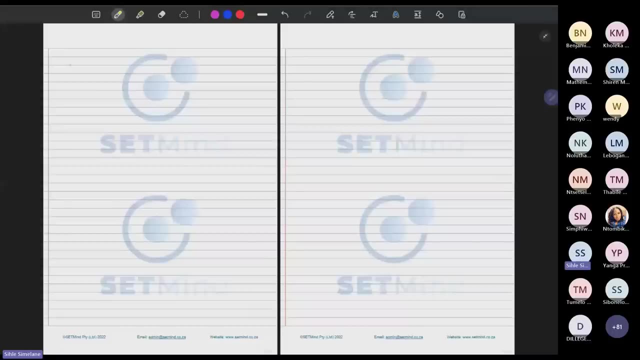 things like your many parameters falling on the same class of dimensions. you will need to have different groups. so, for example, um, you see the problem which we we had. so let's say you have four variables- I cannot think of an example- and then you have two dimensions. what this means is you: 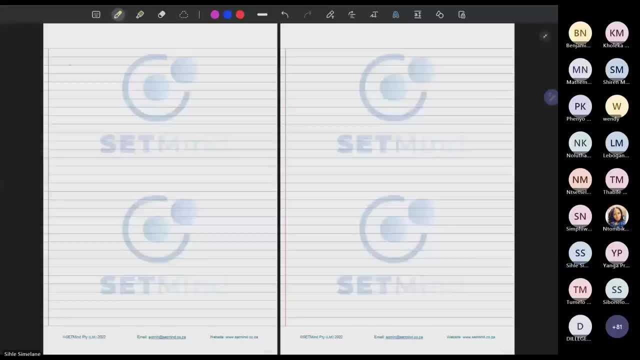 will have four minus two, which will be two groups, um, so, which means the four variables which fall under the same category, let's say dimension, geometric. so, for example, in geometric, if we look at Geometry, if we are speaking of, let's say, for example, length of something, or we are speaking of radius, this would fall under geometric. 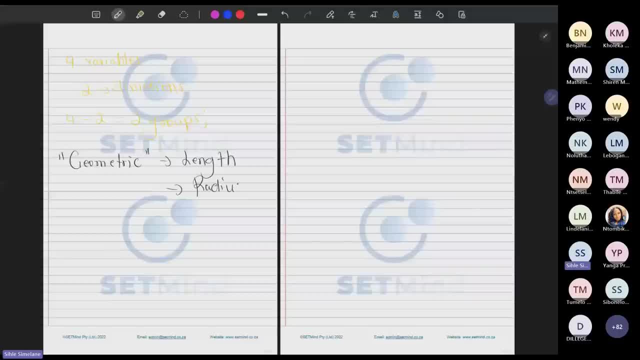 so since we only need two groups, it means one of the group will have length, other one will have. we try not to combine them because these ones they fall on the same group. since we have four variables, it means maybe we are gonna have variable one, then variable two and then the. 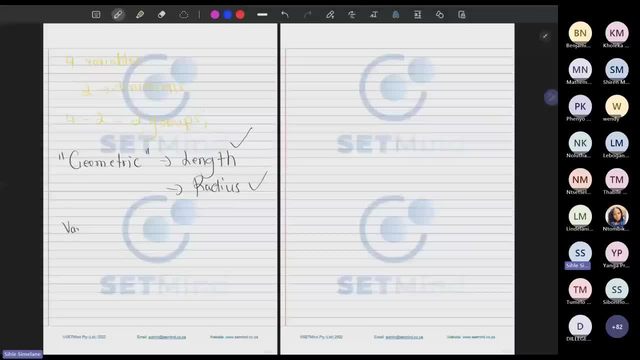 other variable which would make the third would be len, and then we would do c, would do b, then we do a, then we'd have m0, and then t0 and l0, and then the other group, because we need two of them. the geometric property or the geometric dimension is repeating itself, meaning. 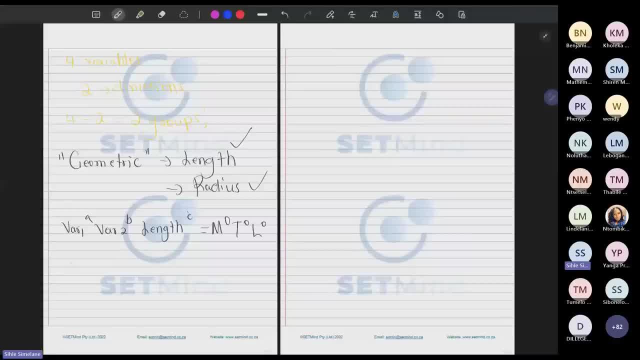 the other group would have var1, var2, and then it would have radius, and then we would have your c here, which would need to solve for your b, then for your a, and it have m0, t0 and l0. so you'd have two solutions because of the two groups, because one property was appearing. 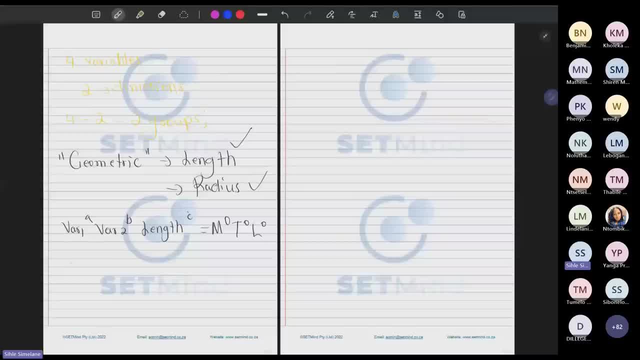 twice on the group. so geometric properties. it is length, radius, so i cannot cluster them on one. that's where you get presented with the problem. so clustering them will eliminate all the other, all the other variables, leaving them dividing one another to form a dimensionless property. does it make sense? 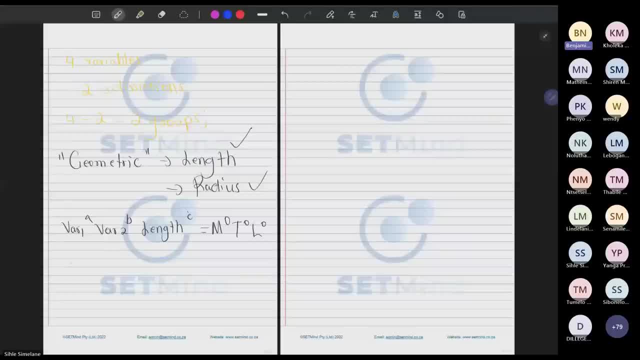 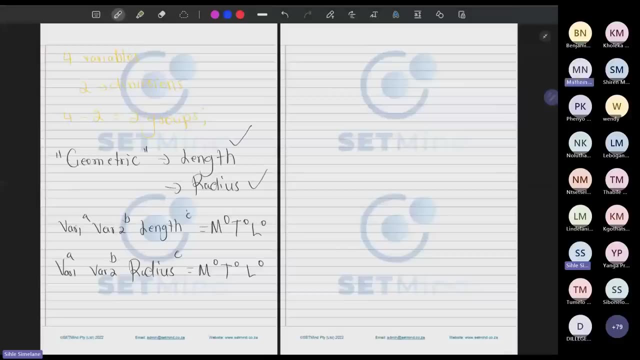 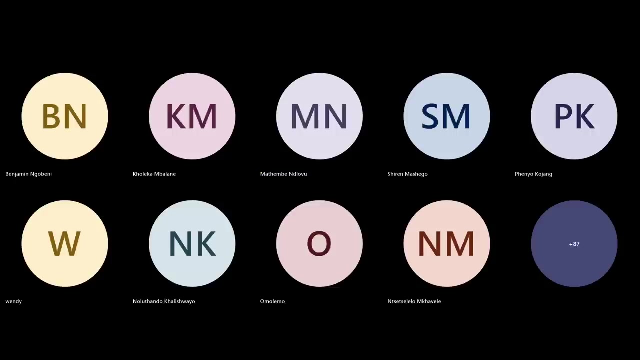 not, not really. is it possible to to make an example for the one of two groups? because currently it doesn't make sense. yeah, so let me quickly stop sharing my screen examples. they always at the point, of course. let me stop here and quickly try to draw and look at last year's tutorial. give me a second. 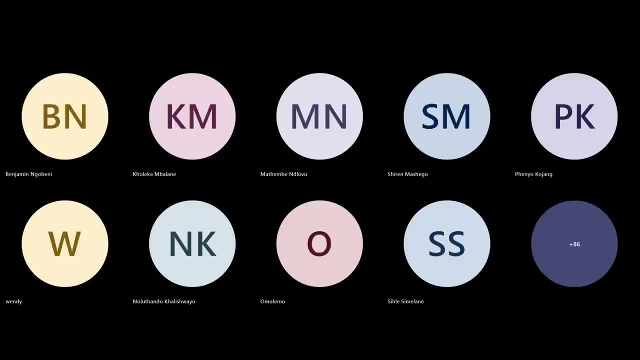 and then i'll talk a little bit more about the general thing in the next part. so if you have any questions, you can always contact me at the end of the video. if you have any questions, please feel free to email me at carter hall. at carter hall. 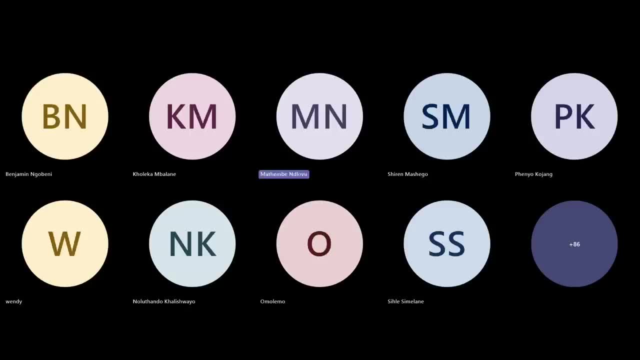 at carter hall. the link is in the description of the video and i'll see you soon. so thank you for watching and i hope you enjoyed today's video. if you enjoyed it, please hit that like button and subscribe to the channel, and if you have any questions, you can leave them in the 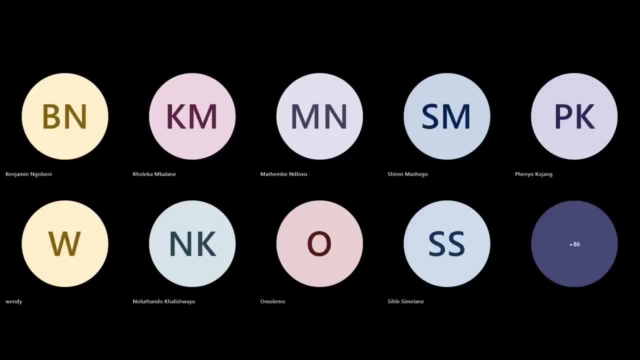 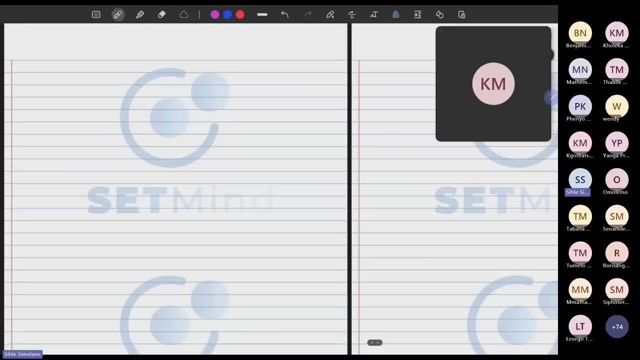 comments section below. you, you, you, hey, i'm back. can you hear me give me a thumb up, if you can? okay, great, i was thinking in 5k, so here's what i'm gonna do. um, this will probably be the first example which you, you do. it will be the first tutorial, so let's consider, let's consider a. 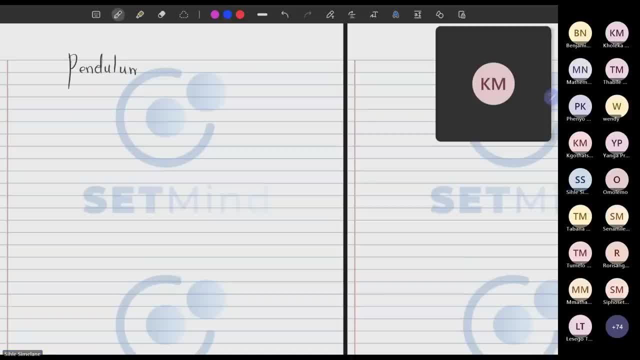 pendulum. so i'll draw a pendulum here, because this will be the very first problem which you are presented with. so when you look at a pendulum, i'll draw a line like this and there's your pendulum. so what i want to get from you, 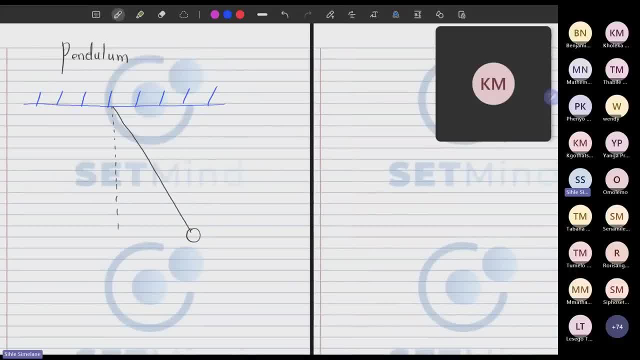 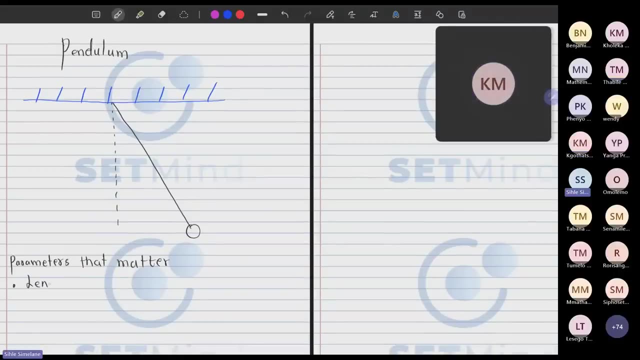 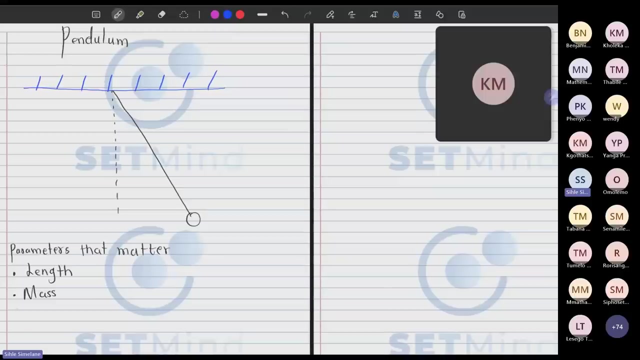 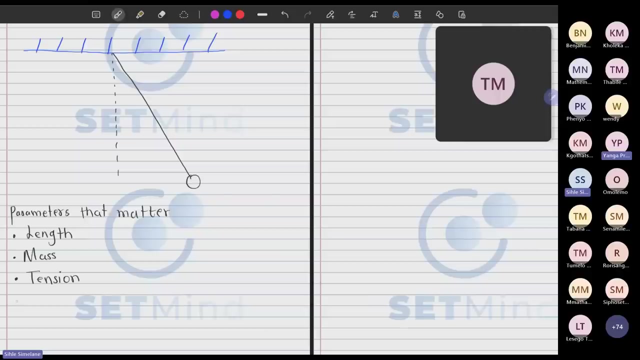 is the. I want the parameters which matter. when we think of a pendulum, Then mass Tension, Then let's go to mass. And then what else? Velocity, Force, tension- Okay, let's take tension. And what else matters? 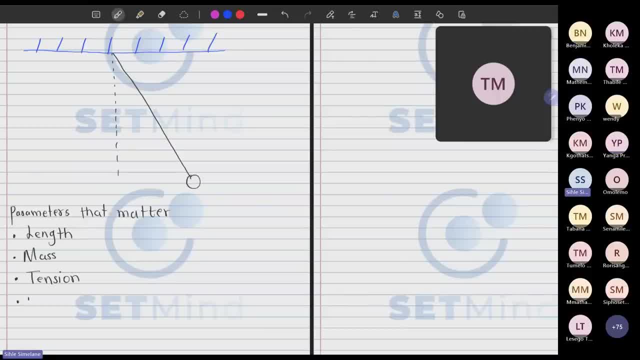 Period. Okay, thank you, It is the period. And what else does matter here? The angle, The energy, Thank you. Okay, so let's say these are the forces which really matter when we look at your, what you call it, your pendulum. 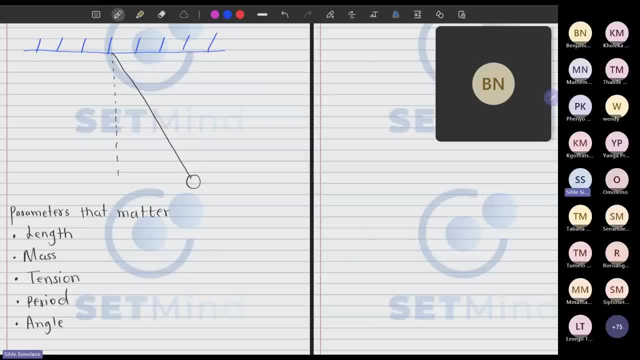 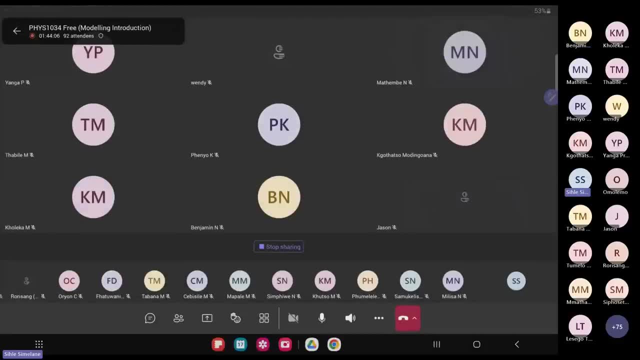 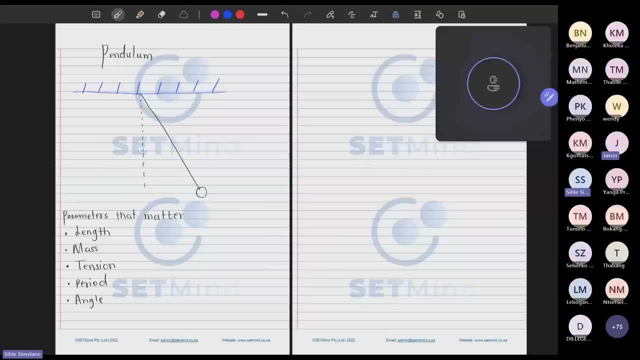 So let me see length: mass tension period. Sorry, sir, Please can you share your screen? Oh, I'm not sharing my screen, My apologies. Can you all not see my screen? Mark, we can see it now. 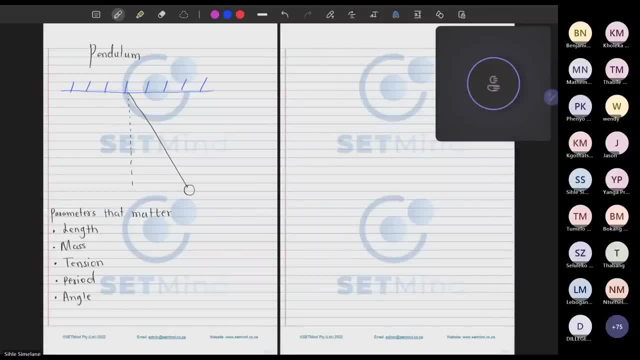 Can you see it now? Yes, Okay, great, Thank you. So we are saying these are the parameters which matter: Length, mass, tension period and angle. Do we have anything else? Yes, Anything else? Yes. What about the force of gravity? 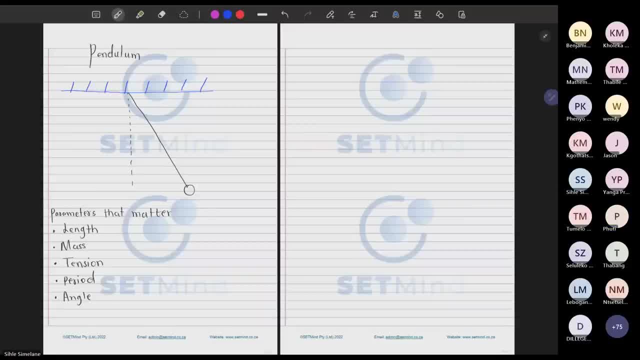 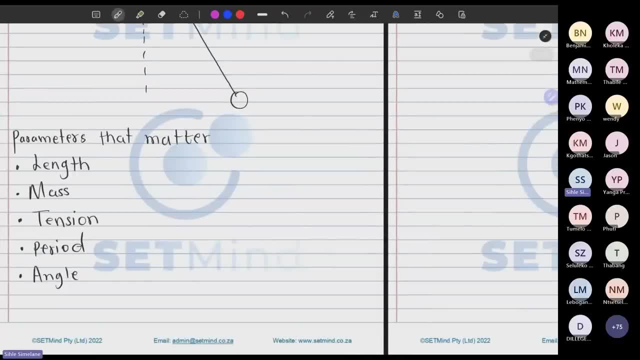 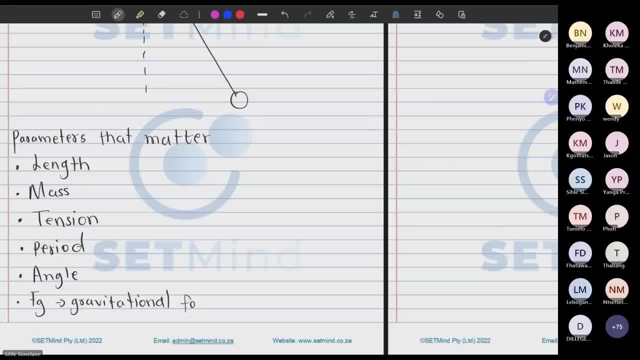 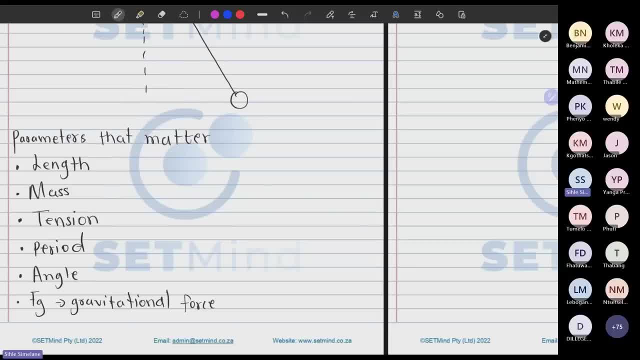 Okay, So let's write the dimensions for these. So the dimension for length is Length. So for length, we are looking at l, For mass, we are looking at m. Then for tension, what is it? Tension is force. 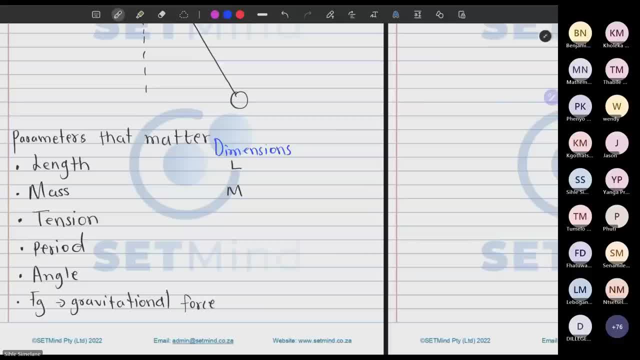 Anyone, Anyone, Anyone, Anyone. are the dimensions for tension, which is first MLT to the power negative 2. MLT to the minus 2. And then for period, what are the dimensions? T, And then the anal. what are the dimensions? 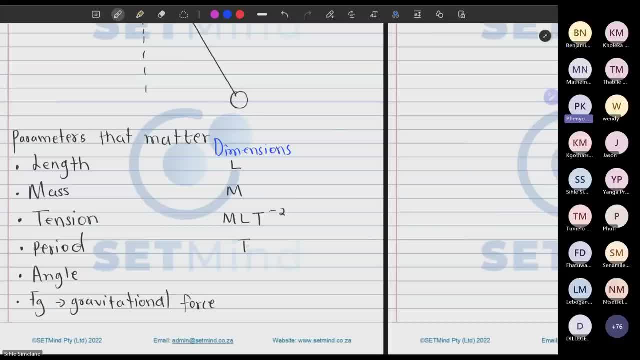 for the anal. I think it's dimensionless. Yep, So the anal is not seconds, it is not anything. So the dimension is N0, T0, L0.. Okay, Then gravitational force will obviously be ML, T minus 2.. 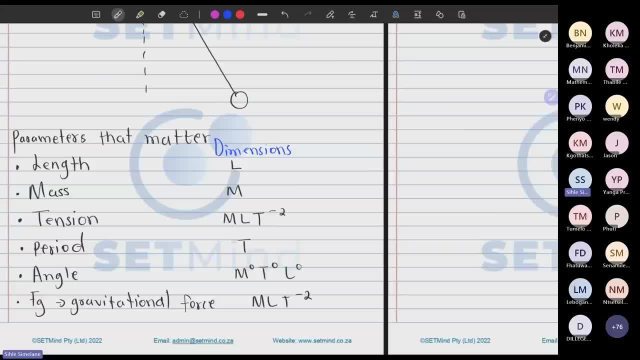 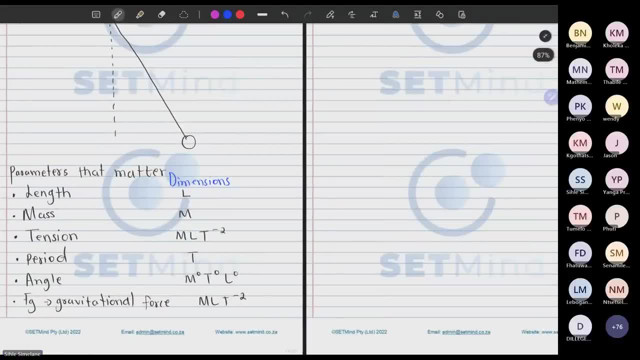 Okay, So now, when we look at what is going on here, we have how many parameters? 1, 2,, 3,, 4, 5.. 1, 2, 3, 4,. 1, 2,, 3, 4,. 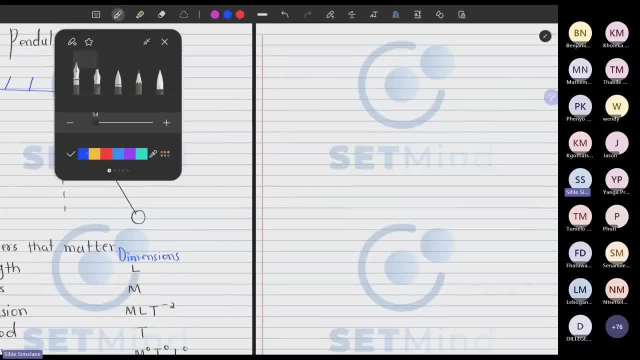 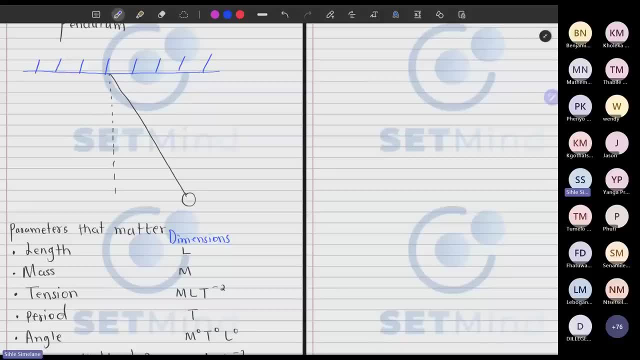 5, 6. Problem. So we have six parameters here, But if you remember a simple pendulum, my question to you was: was the tension force playing a role? So we have six parameters. Let's carry on and see what we. 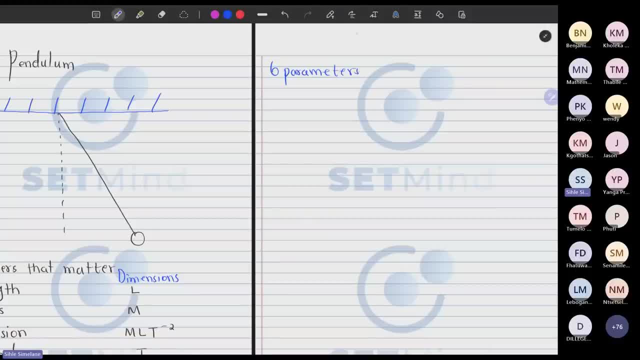 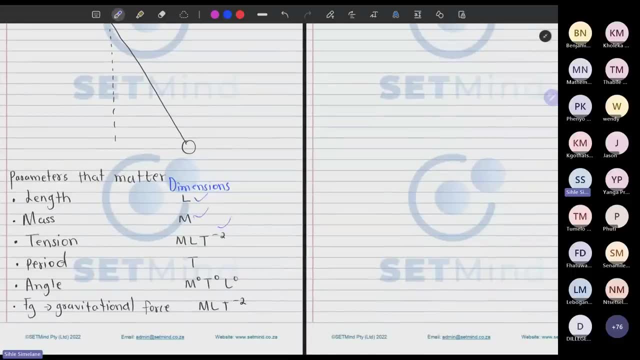 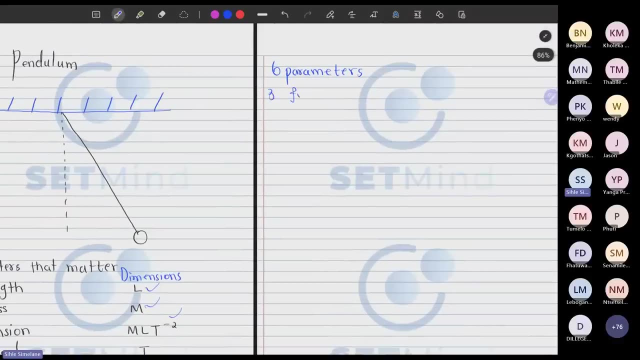 obtain. And then we have four. we have three fundamental dimensions, So the L is there, the M is there, the T is there, So we have four. no, it's not four, it's three, sorry. Three fundamental dimensions present. 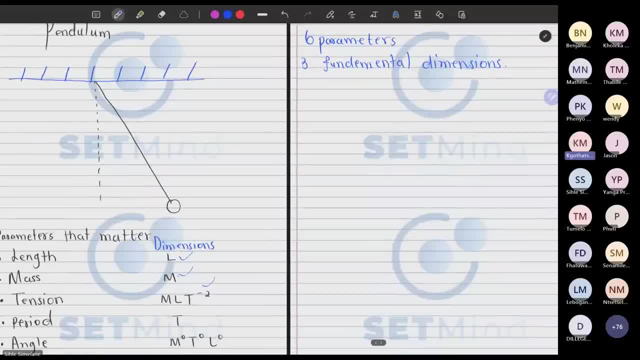 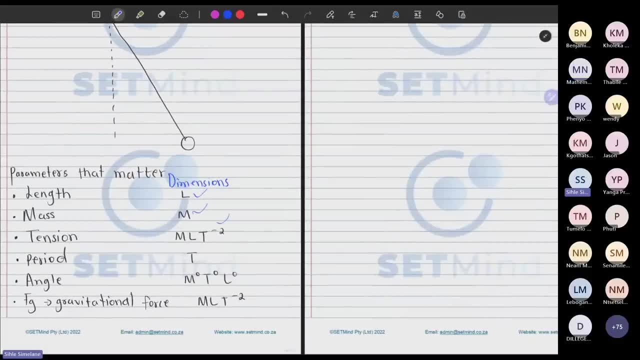 I'm say Yes, Um, why? why do we count the angles? So this dimension is, It's because it does play an effect And it comes. Oh, okay, Thank you, Which is six for the workings of a pendulum. 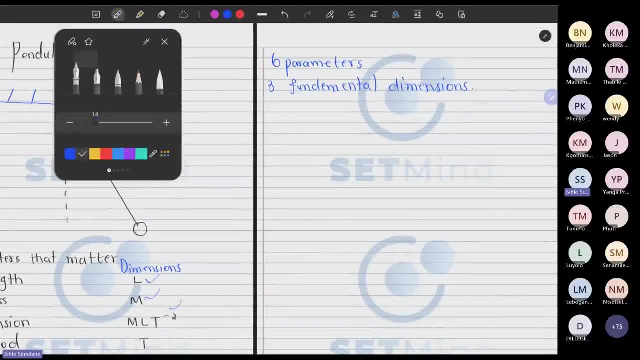 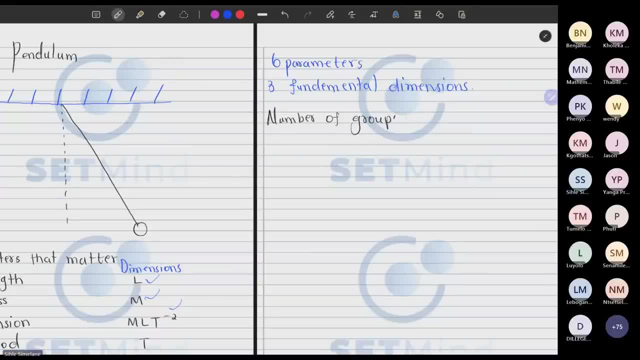 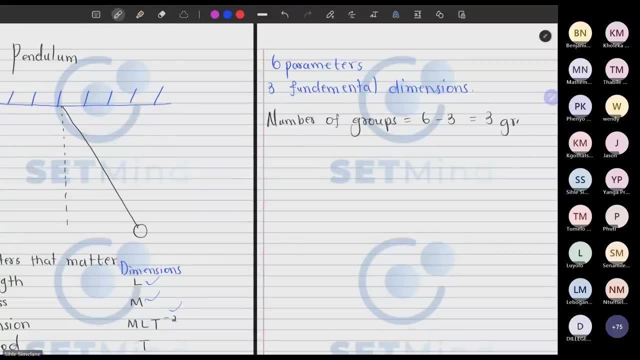 Okay, So we have this and then, if you look carefully, the number of groups, Of groups We are going to have here, it is six minus three, which is three groups. Hello, sir, You can shoot. Yes, sir. 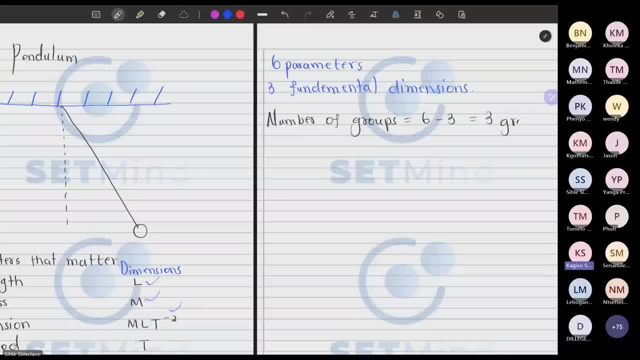 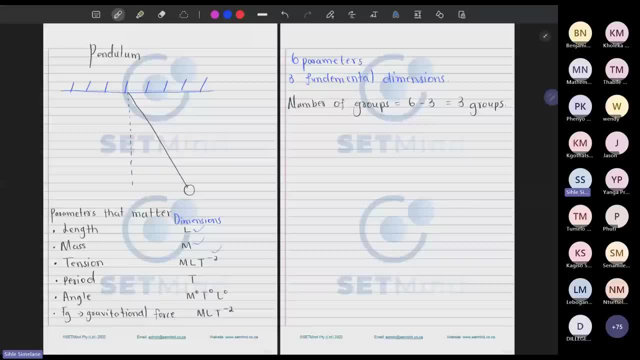 Oh, can I please ask, Is it also necessary to include the Amplitude of the string? Uh, what the amplitude? Yes, sir. Um, what do you mean by amplitude? I mean the, the. okay, it will be the maximum angle that the, the, the pendulum, will make with the equilibrium right. 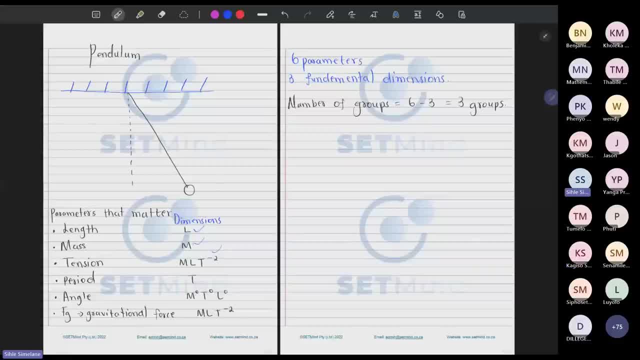 but is? is that not accounted on by just saying beta? see, i'm saying, is that not accounted by peter? yeah, i think yeah, because it will be the maximum angle that it will make with the equilibrium position. yeah, so, so at the end of the day, it's. 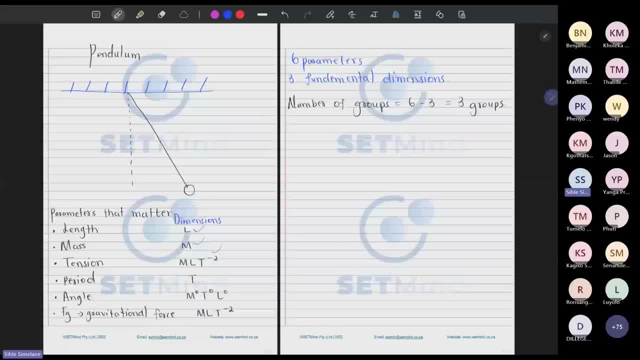 thank you. so we have three groups here. we need to decide on something, which is: how do we then relate these variables such that we do not get presented with problems? so any suggestion from anyone? so the first thing i'm gonna write is: please give me the formula for the period of a pendulum. 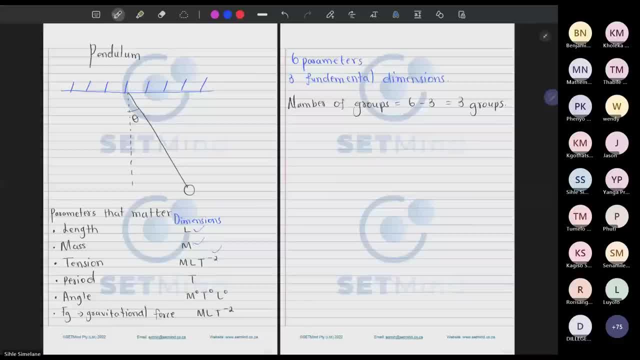 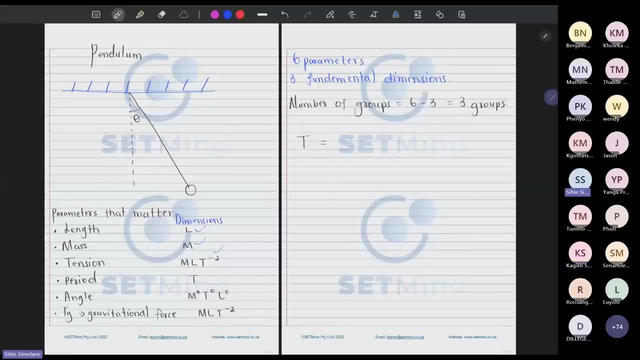 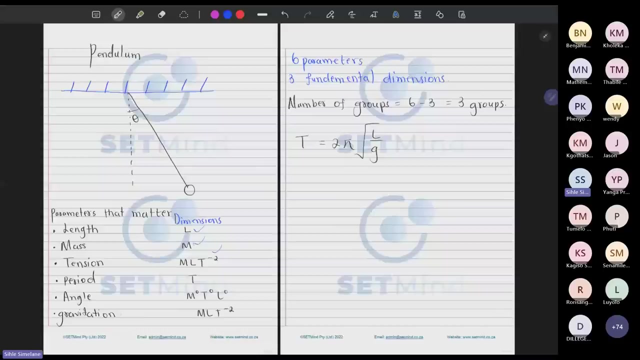 it was what? what was the formula for the period of the pendulum? anyone t is equals to two pi square root of l over g, two pi square root of l over g, and to the entonces. so the z square pneu is the force of gravitational force. 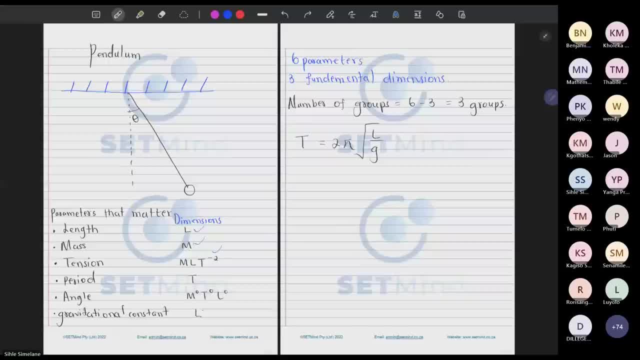 so, in fact, here's my suggestion: let's remove this gravitational force, because we already know we have mass here. instead, let's just put the gravitational constant, tational, understand alors? and gravitational constant and constitutional constant. so what we need to do is to try and come up with combination of variables which will not give us a 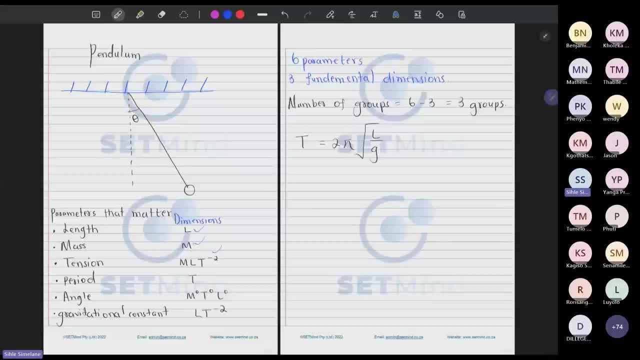 problem here. so anyone who has an idea of how they should think we should choose the different groups, because we should have three groups here, anyone? so i want to ask a question. i'm trying to separate this, this equation for the period, into: so each variable one is separated into different groups. 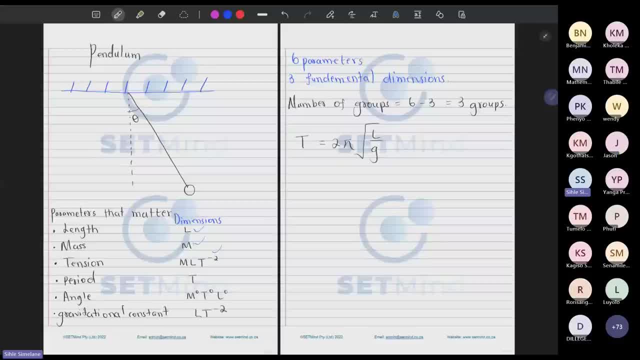 yes, so many. for every group, there should be a new variable which makes that group to be a new group, which means you need to have a variation three times. that's how you're gonna achieve three groups, meaning there's variables which are gonna remain constant. then there's the three. 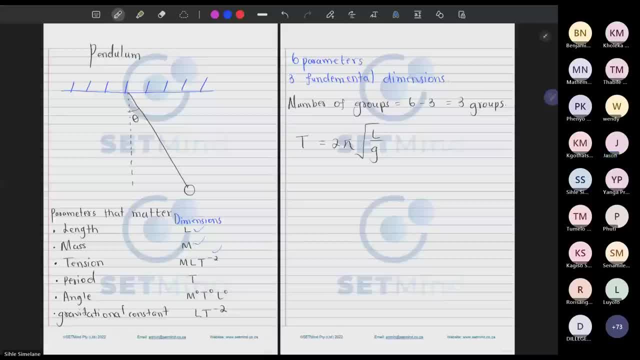 variables which will be changing. so can we say to any type of variable, like, if we were to say like, for example, like l to a and then g equal to b and then maybe t equal to some other variable, um, what do you mean? so, if, if we're trying to set the um, if you're trying to set two pi of square, 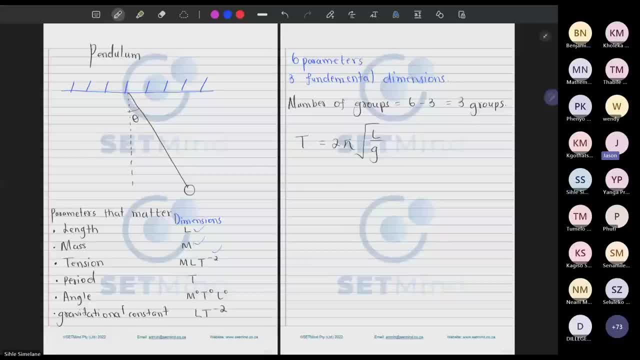 root l over g to have three different variables. so i thought, so i'm thinking of, do we assign it to another type of variable? so, as i said, if we assign the l, which is the which is the length, to a variable a and then g to a variable b, if that's, that's crazy. i'm not sure. 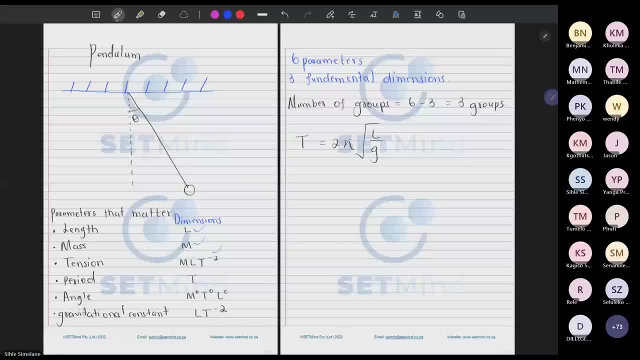 so here's what we need to do: when we choose our groups, we need the variables which will remain constants, which means they will be in all groups. variables that will remain constant, so we'll be in all groups. group now, let me just tell you that, the keyboard meaning yes, although we're 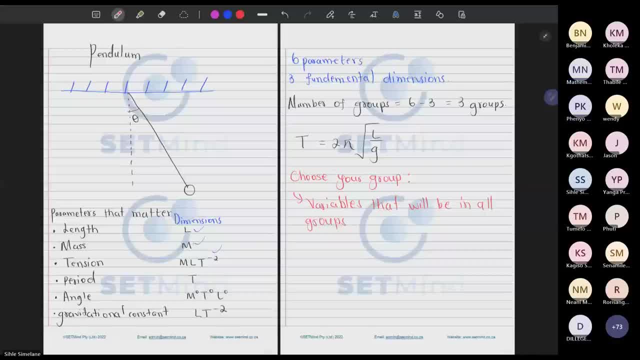 going to it just as you, if that form of the language is involved. that's what we are. i'll call this script so sorry. i'll just call it problem, to be fine. all right, i did. if i had at least one single problem in the algorithm, that would work. i don't know how many problems. 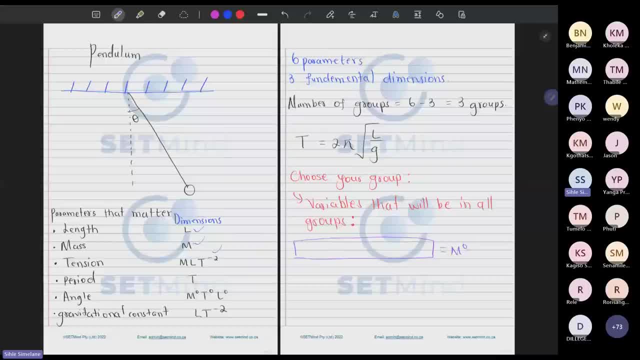 you may have, but maybe by now are you going to figure out. twouy, it would be many problems. all right now look at this here. this is which i am just going to call it, arguments. so what i will callケ, and this is my own figures, excuse me, i'm 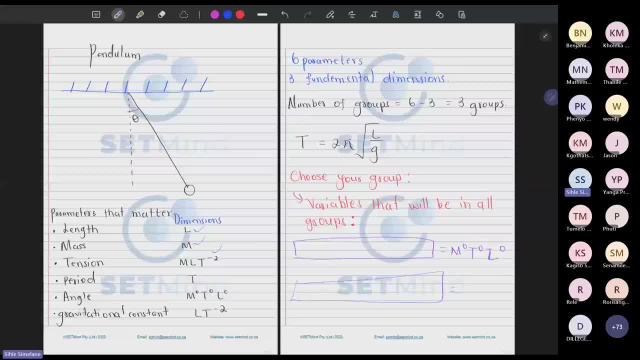 related to others, so we can form three groups here to relate variables to one another. you can go ahead. so, um, i want to ask what is the main question? as we have aligned, we listed all the parameters and the dimensions. what is the question? are we looking for the period as we've written? 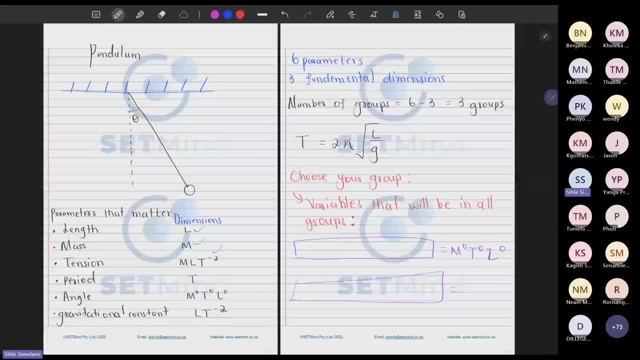 down the period or what? yes, so one of the groups will give us a solution which describes the period. that's one of the solutions which we are gonna get. so, if you look at, do we have anyone with the question for for last year i was looking for. 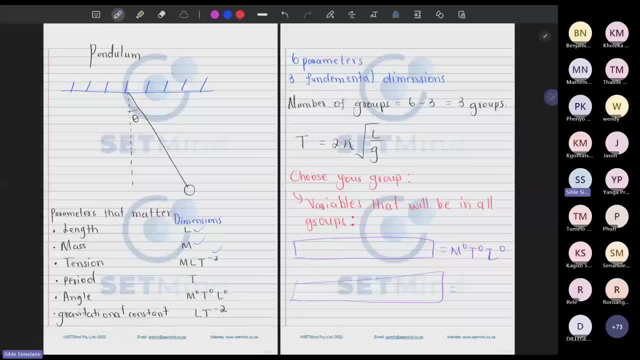 the question. i just cannot get it, i just cannot find it so that you can see what they really want. so they can say: find the three dimensionless groups which will result from this pendulum, and then you need to find that and one of the solutions will show you that actually the period is proportional. 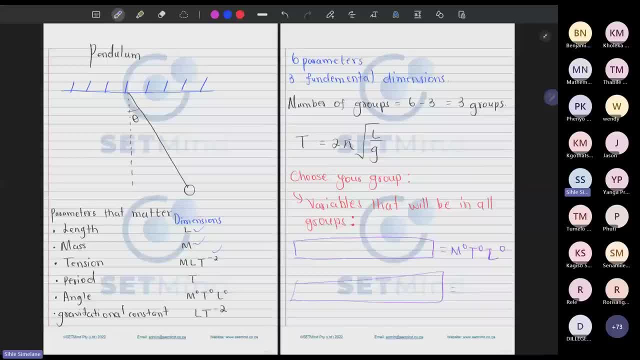 to the square root of the length over the gravitational constant. any question? we have another question, so, um, i still don't get a clear answer to my question, because i can. for the last one, we had a question asking um, what is the relationship between pressure and um area length? if i remember? 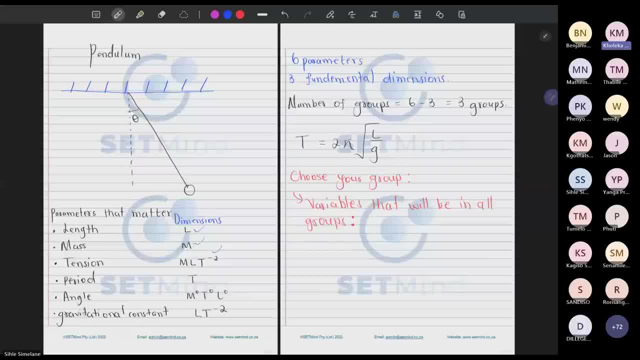 correctly. so in this case, what are we looking for? which relationship are you trying to get to look? so this is no, that's just a question. so how are you trying to get to this? what's the question i'm trying to get to? so i'm just trying to say: is there anything that you can? 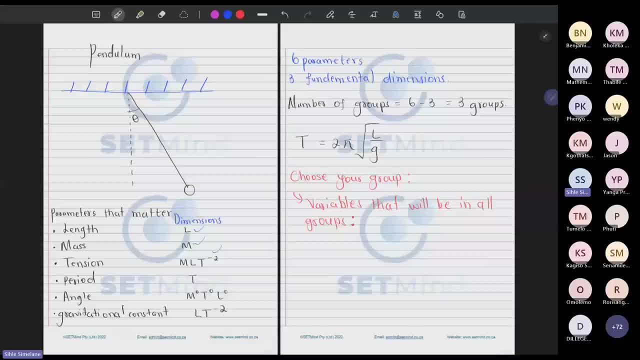 say: what is the relationship between period, the length and the gravitational constant? let's phrase it that way so that it reduces the complexity and we don't need to look for groups which we do not need. so let's say: the question says: what is the relationship between? 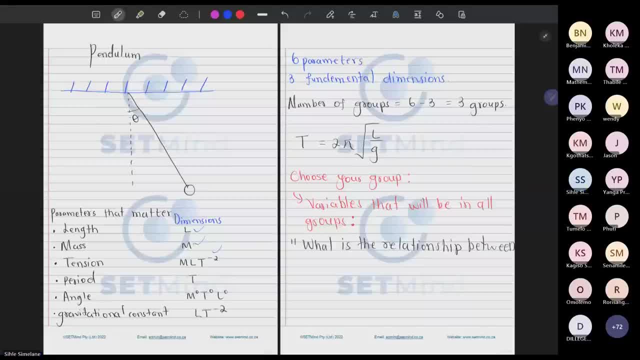 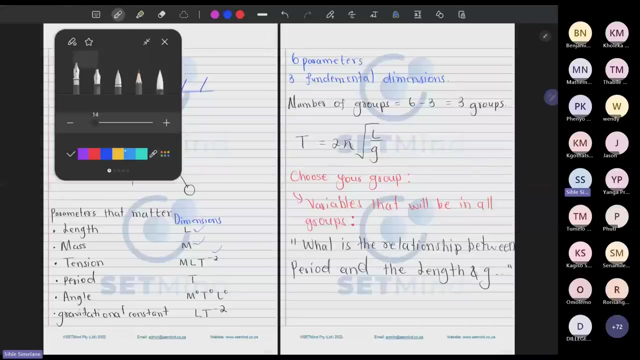 period and the length, and g, which is our gravitational constant. so let's narrow the question to to that. so it means in our group we obviously need to have t, we need to have l, we need to have g. so that's three, four, because they are saying they want the relationship between t, l and g. so it means in our group we will. 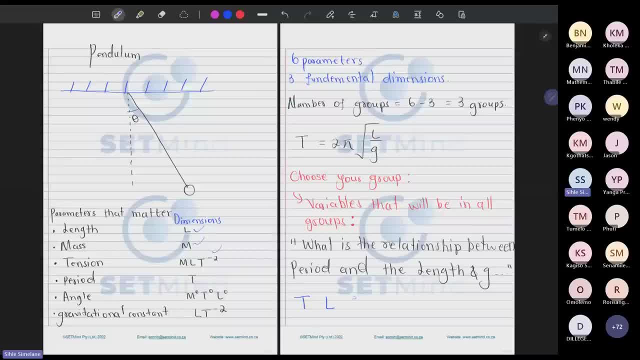 need to have our t, we'll need to have our l, we'll need to have our g. but then the question is: what are the other parameters? so let's put a here, b here and c here. what are the other parameters which we need here? complete our work. 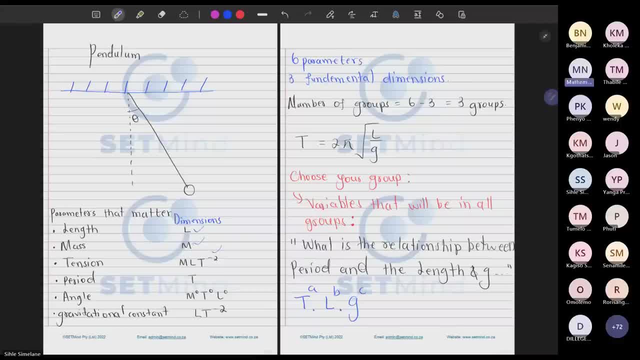 anywhere. okay, if we have to look for parameters that are going to help us complete our work, like to select those parameters. what do we look at? so we look at. so we narrowed this question down. i was going to speak us. what is the force of queria's exercise? we look at the force of something in the body. so these are the bodies that common participants in our interdisciplinary 사람이. 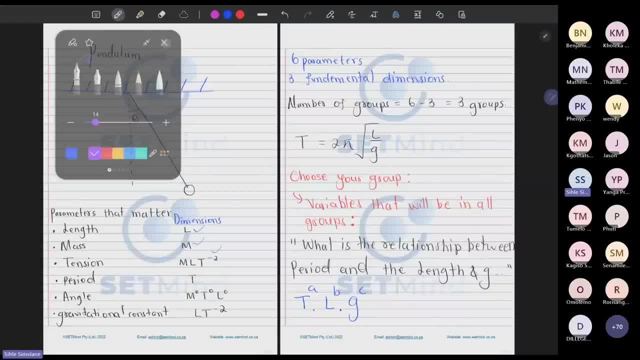 about geometric, because when you choose your parameters you should have geometric parameters, you should have flow parameters and then you should have fluid. So fluid is not here. But if they narrow down the equation to this, then it becomes easy, because you know that in my question or my group, 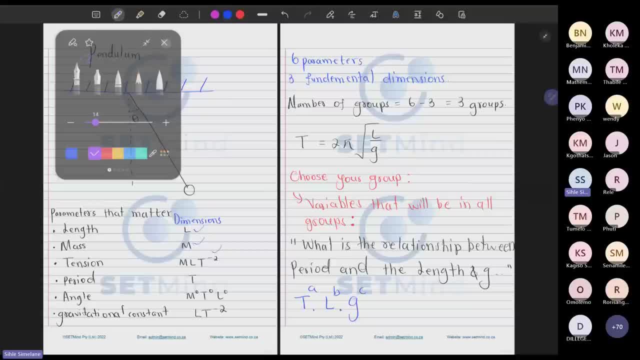 I need to have time, I need to have length and then I need to have g. Now the other thing which we need to stress about is: what is the other variable which we need here? So time, length and g should always be there. 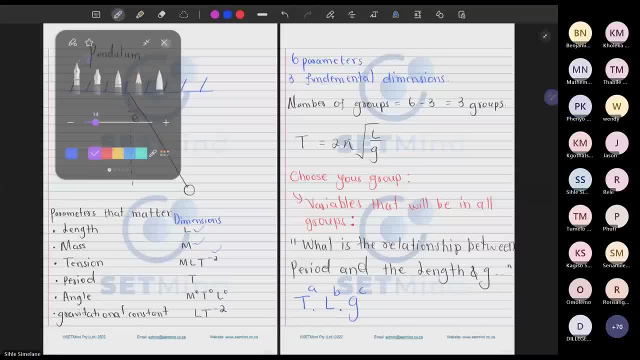 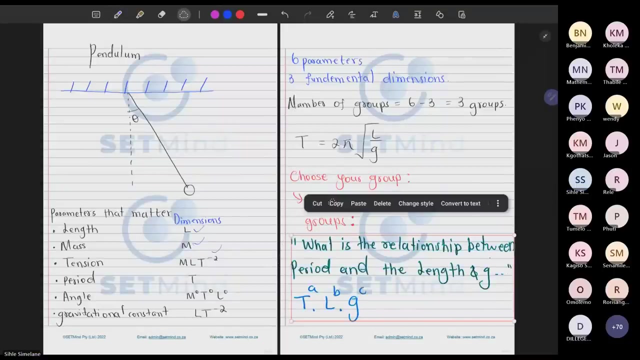 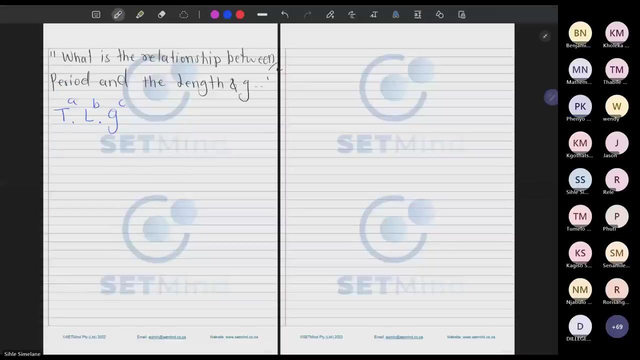 But then what other variable is missing? Do you all understand the question? No, Okay, Let's copy this to the next page, Maybe. like Dima, I'm starting first by probably explaining these three clusters that you mentioned: geometric- I forgot the second one that you mentioned- and the fluid. 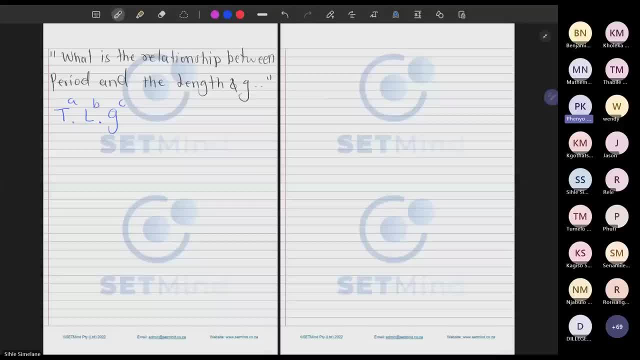 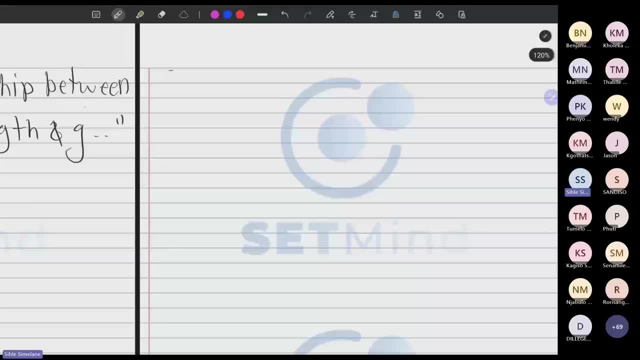 Maybe, if we understand what they imply, we can be able to maybe utilize them to answer the question. No problem, Let's look at what they refer to as the three properties. So you have a property which you refer to as geometric, Geometric. it is just exactly what the terms say. 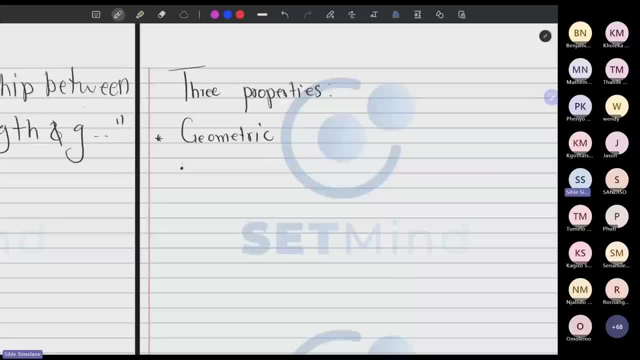 When you look at the geometry of something, what are you most likely to think about? So, when we look at geometry, it's when you're speaking of length, That is part of geometry. when you're looking at width, That would form geometry. 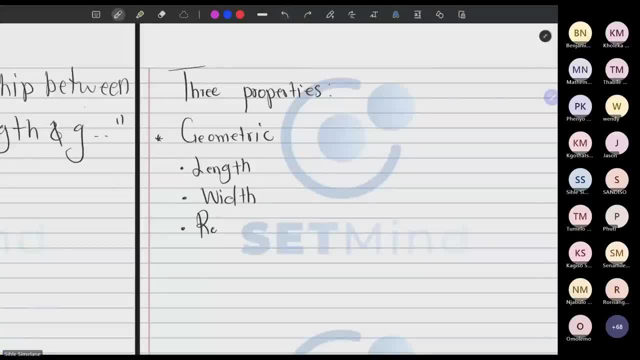 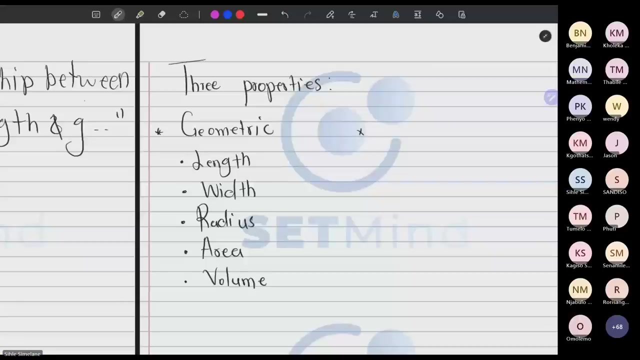 When you're looking at radius, that would form geometry. Then when you're looking at area- something like area- that would form geometry. and then when you're looking at volume, that would form geometry. Then there's a property which we refer to as flow. 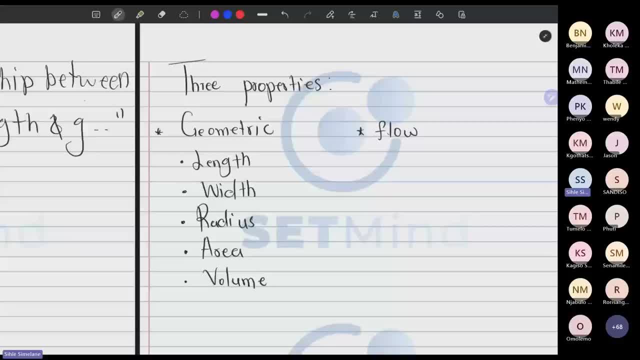 Then when we speak of flow, if you think carefully, you are thinking of movement to some extent. So when you're looking at flow, well, you need to speak of velocity, You need to speak of acceleration. Acceleration describes flow, whether it is gravitational acceleration. 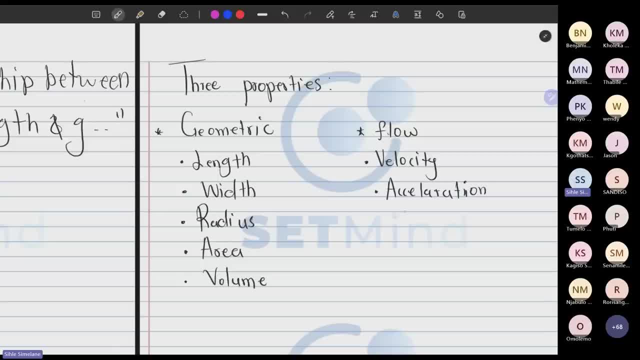 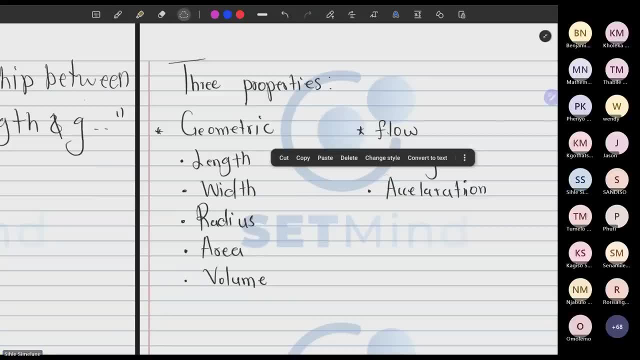 whatever it is, but it's acceleration. it describes flow. Which other quantity can you think of Which describes flow? anyone, Which other quantity describes flow? Could you say momentum? Momentum, Let's think carefully. Momentum is mass times, velocity. 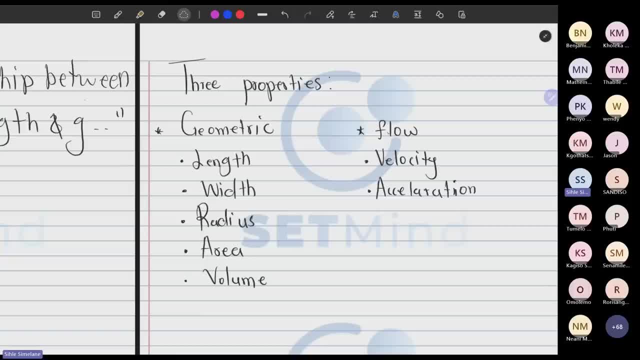 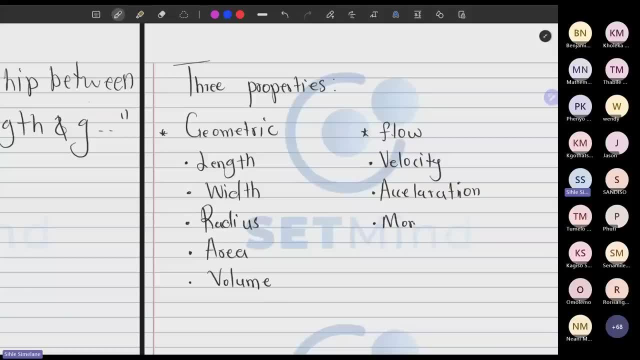 So in a sense it does describe flow. Let's look at it, Let's put it under that You can try and say flow. Let me take it. Anyone else who thinks is thinking of something which describes flow. Could you also say displacement? 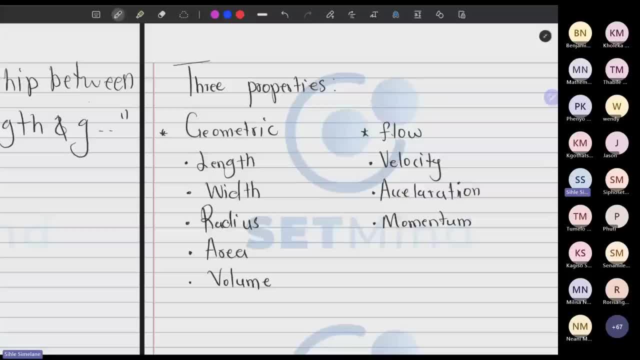 Displacement. You see, displacement is described in flow. Displacement does not describe flow. Displacement does not describe flow. It describes flow or movement. in a sense, It describes the change in position. I would not call it flow, I would not say. 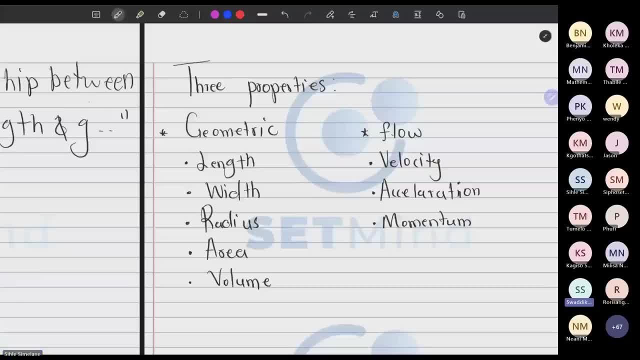 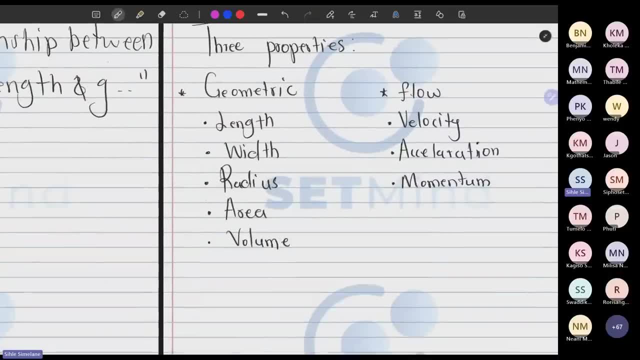 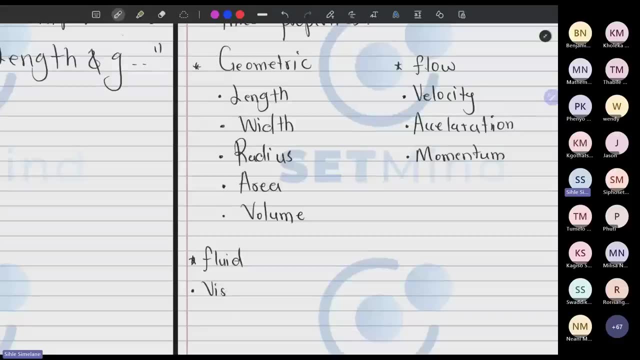 How about viscosity, sir? Viscosity, would you not agree that that falls under? there's a category we call fluid. Okay, So viscosity would easily go. Viscosity would go under fluid. Does it make sense? Yes, sir. 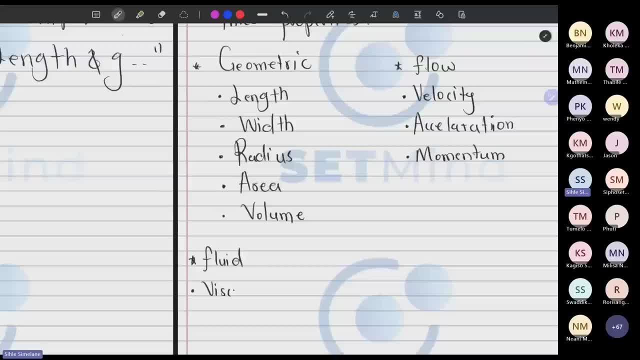 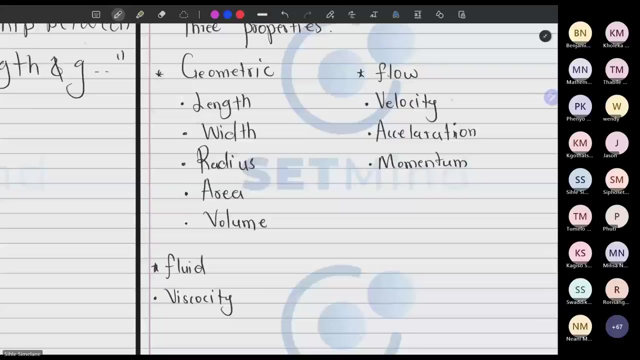 Viscosity, which describes fluid. Anything else which anyone else is thinking should be ended at a, should be added under these properties. Speed Speed would fall under the speed to velocity. that would go under flow Speed would go there. So let's think of of what. where would time fall here and where would mass fall? 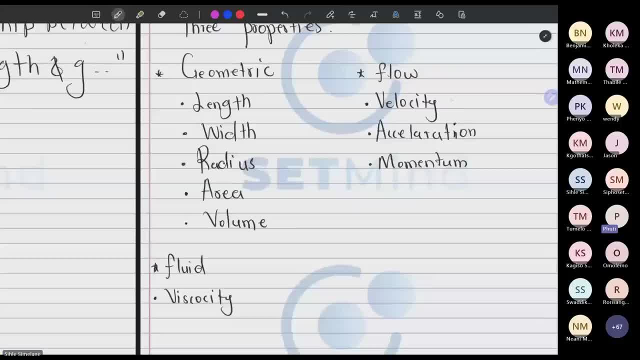 Sorry, sir, am I right if I say all the geometric ones are extensive and the flow is intensive? Yep, Yep, you are. You are right. Okay on point. Good insight. So let's look at flow. What else can we add there? 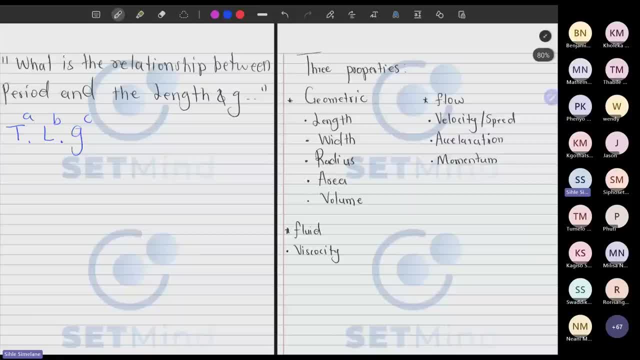 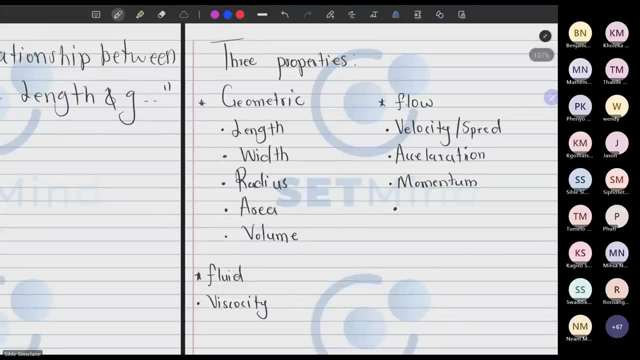 I'm more interested in time. Where do we think time falls Under flow? I think Flow. And where? where is pressure? Where should we put pressure? Where should we put pressure Under flow? Is it fluid, sir? So when you, when, when, when, when you, when you compress a gas or in whatever container you are. 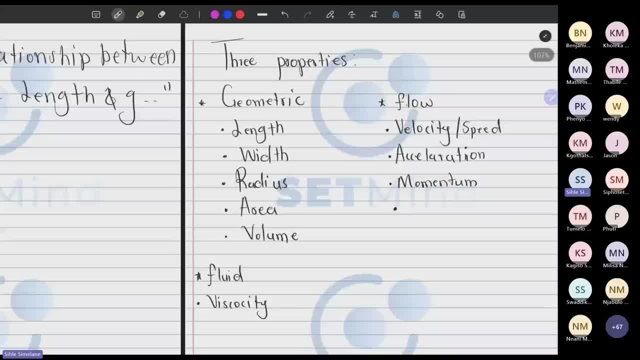 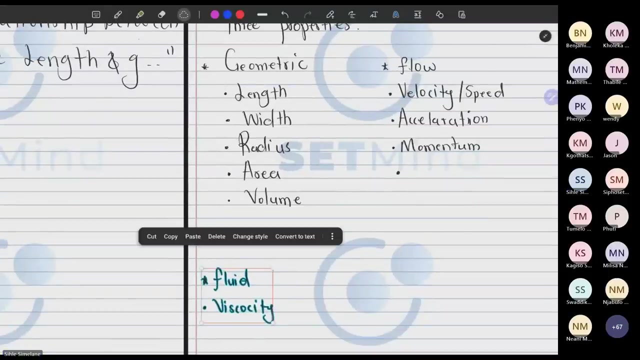 but increasing the pressure, would you consider that is falling under flow, Under fluid, sorry So, let's think carefully. Where do we put pressure here? Geometric, Why? Why are you thinking of geometric? We pull it down. Anyone else? 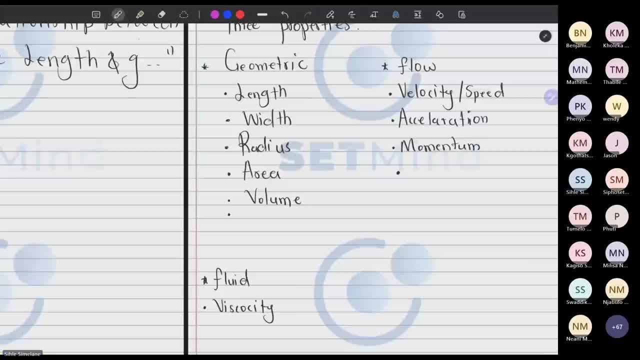 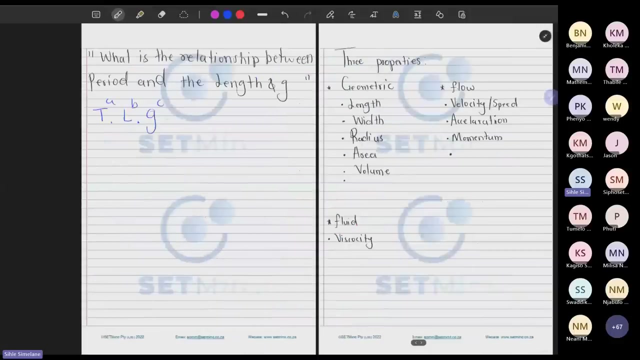 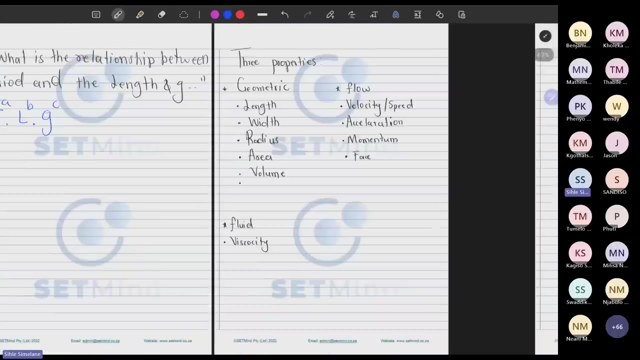 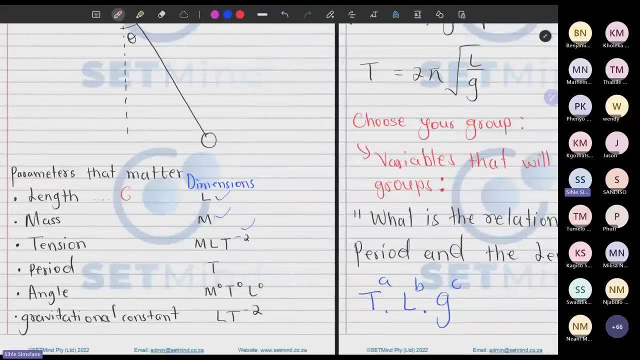 Why do you think it falls under geometry? Hey, let me put this to a pause for now. Let's quickly take the variables which we can classify from here And let me put in force here. Okay, so if you look at the variables which we can we have here, length is a geometric 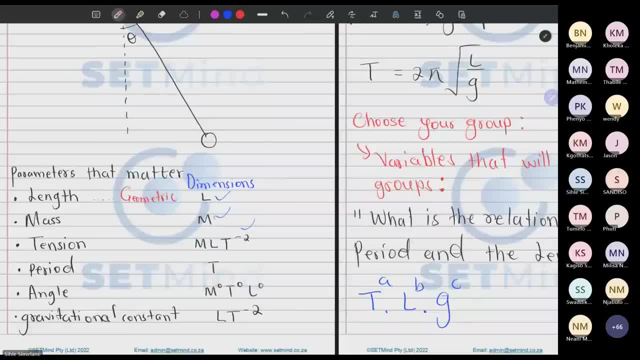 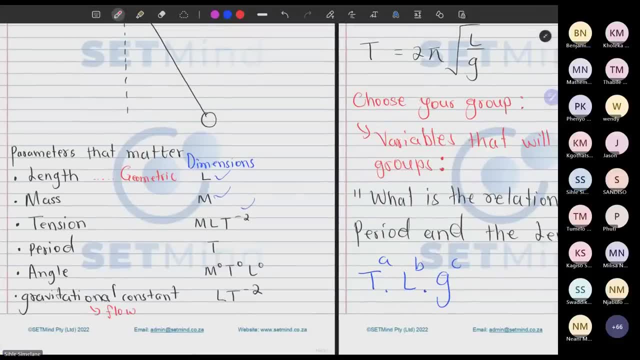 property. And then this gravitational constant. this is a flow, it's acceleration And then tension, this goes under flow. And then here, when I think carefully, I do not see any fluid. There's no viscosity, there's no nothing. 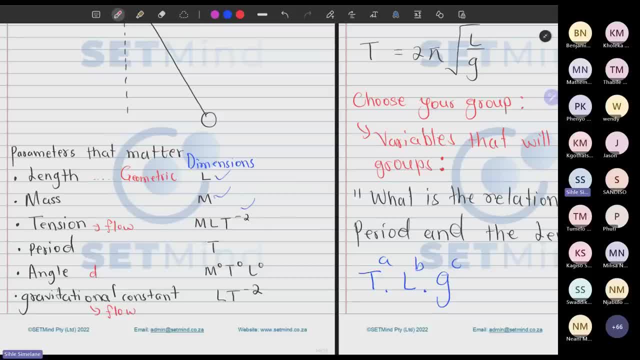 So where do we classify this? as dimensionless? So it's going to be out. So how do we then classify the two which are left? Anyone, Anyone, One, I think. the mass is geometric. I think so. Yeah, I think, because geometric is an extensive property. 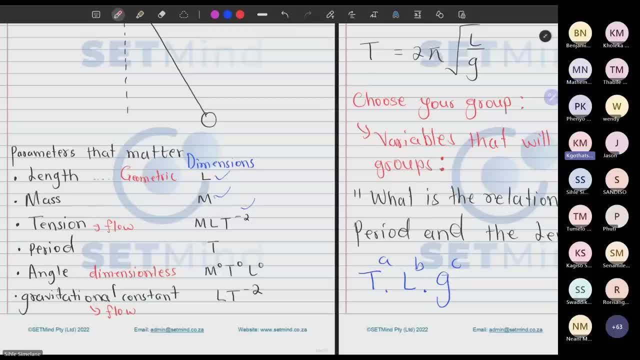 And mass depends on the mass of the substance. Let me think about it carefully. Okay, Geometric property. Okay, let me say geometric. in quotes, I'm still thinking about it, The ones which we are sure of. we'll write them. 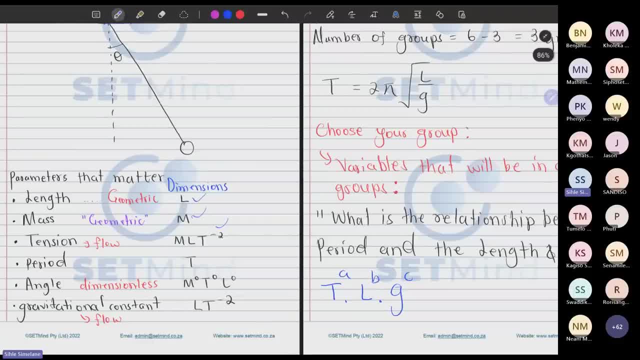 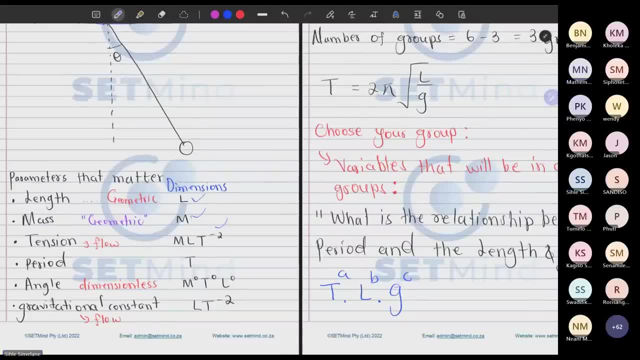 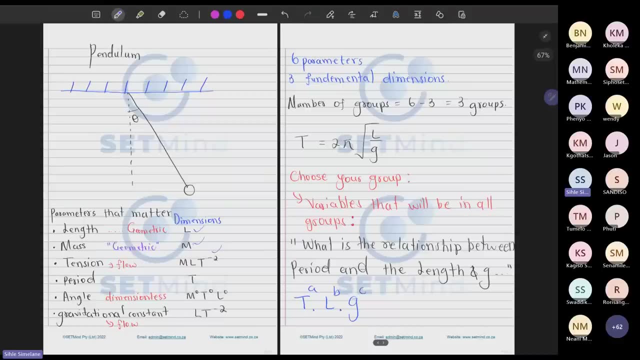 The ones which we are sure of. we'll write them In red. And then here's what we should do afterwards: After you've classified your dimensions, the group which will have the dimensions which do not change. okay, variable. choose your group such that there are variables that will. 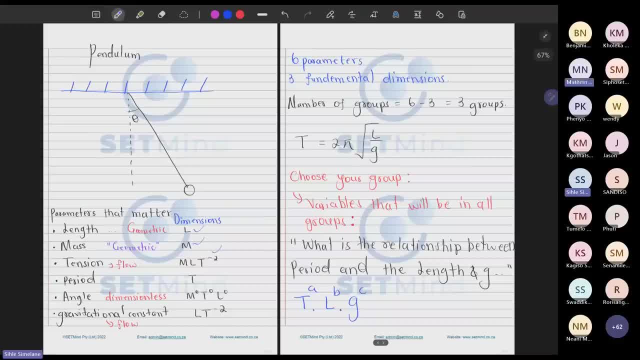 be in all groups. So meaning there are those variables which are not supposed to change, and we will take the ones which we have identified As geometric, as flow and then as fluid. So here we don't have fluid, So we'll take the geometric property, which is length. 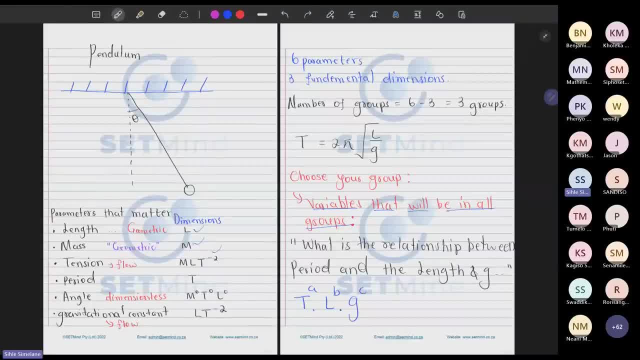 It will be there because we can see, length is a geometric property, Sorry, Length is a geometric property. And then we have the gravitational constant, which should be there, which is the g which describes length. It should be there. And then the ones which we can flip. 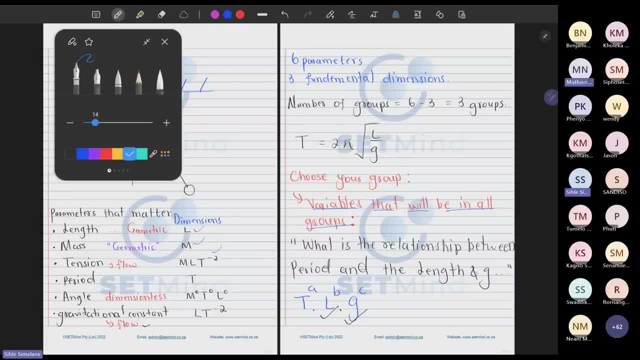 Because we have three groups. it means there's three variables which should vary. So we can choose mass to be one of the variables which will vary, And then we can also choose the period to be one of them. The angle is dimensionless. 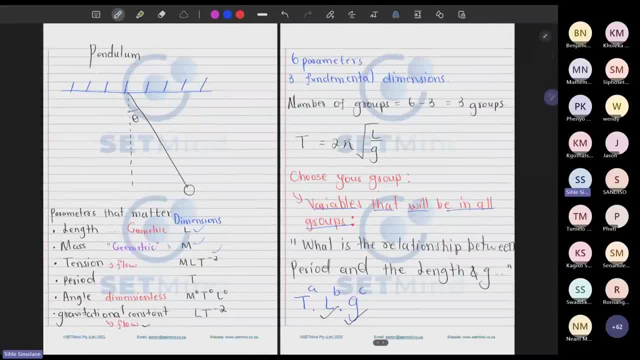 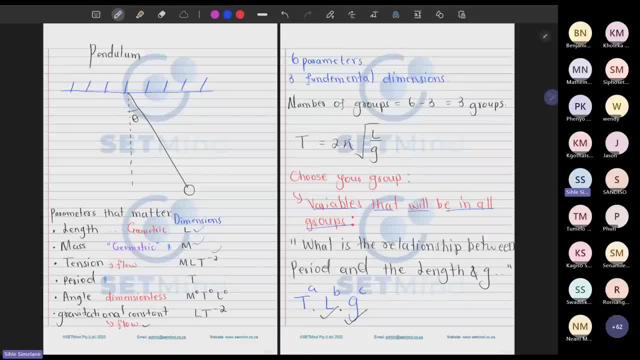 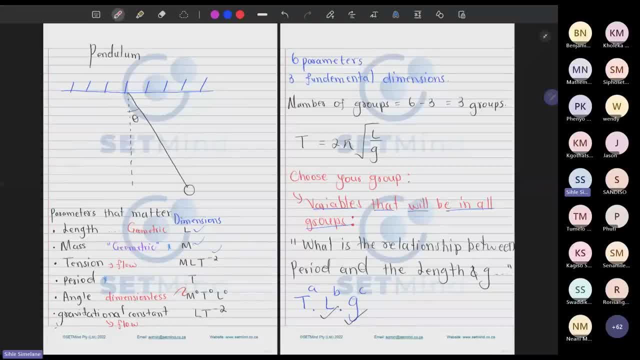 Time Time Time Time, Time, Time Time here and put a d, we need three of them which will vary. so this one can vary, because we are not sure where it belongs mass. i'm not so sure if it belongs under or if it is a geometric property. 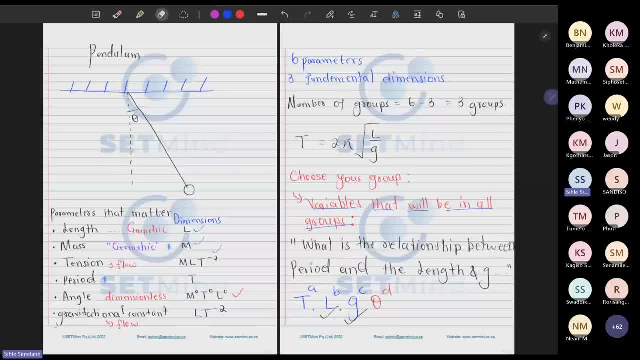 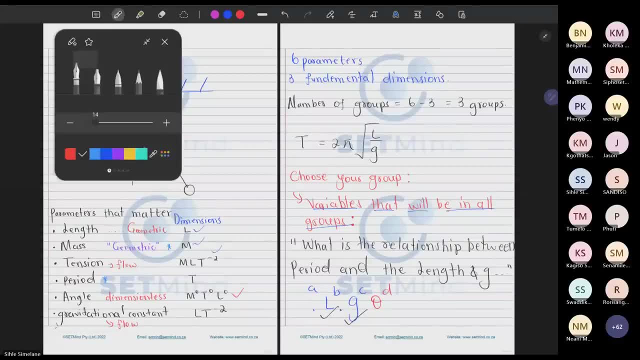 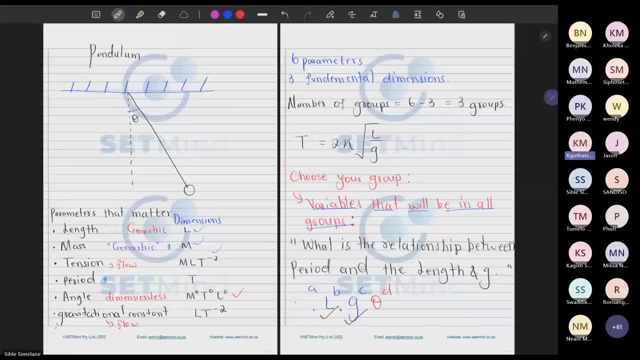 i think you are right. let's put master, the geometric property, because you said it is extensive. so let's put the m here, the mass, i'm say for the period. i think isn't it, it's in flu, it's a flow, since it's an intensive property. it doesn't, it doesn't depend on the amount of 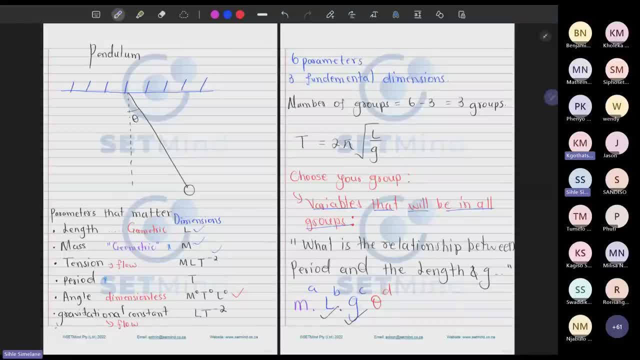 substance, it is a flow present. on that one point, look, is there another way to determine which, what these properties represent, like whether it's geometric flow or or fluid, without using intensive and extensive? i cannot think of another way. you just need to think carefully. what would describe flow? or the rate of movement? what would describe fluid? when you speak of fluid, you must 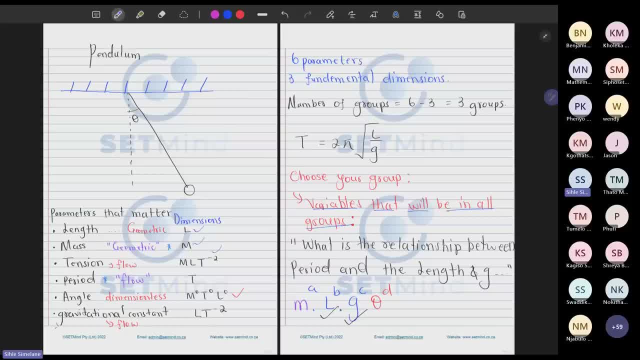 speak of viscosity and other things. so i think it's more of knowing properties of materials rather than having a certain methodology or way of thinking. i think if you know the properties of materials in general, it is easy to classify them okay. so what we need to do from here is that we need to choose. 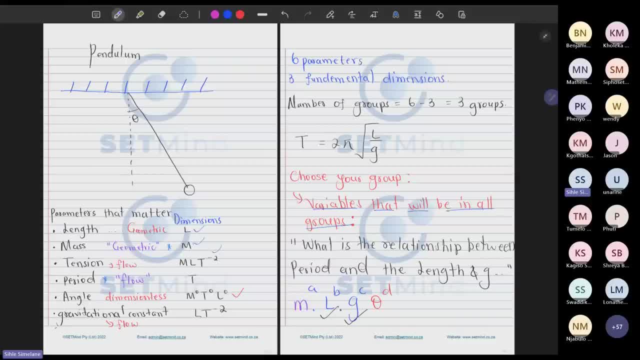 dimensions which will? they will be geometric, and then there will be flow, and then there will be fluid, and then the other ones are the ones that are not the ones which we are going to build. so, for example, one parameter we can vary is this one- i don't know where it belongs- and then another one which we can, because 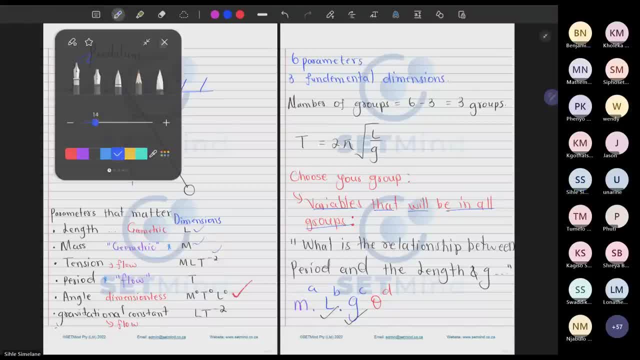 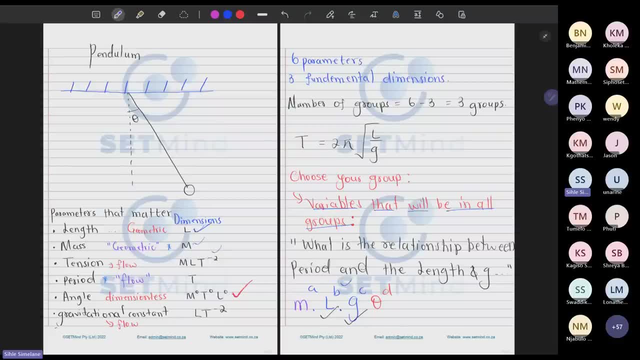 they were saying we need to look for length. it means length must be one of the parameters which is there because we are trying to relay period with your gravitational constant. so length is going to be one of the geometric properties i have. t is going to be one of the. 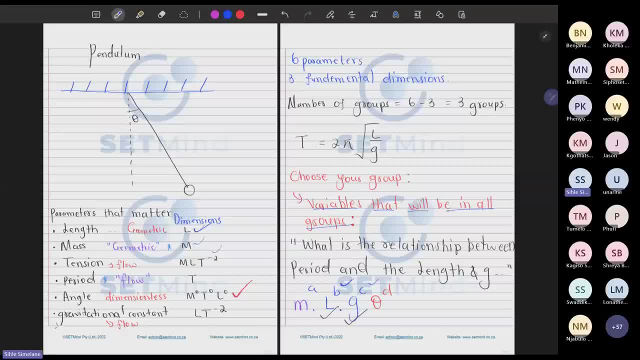 properties i have. and then i need the period, which is one of the mass is geometric flow. so because here there are many variables which are repeating one another, you can repeat them. so i need one last variable. because i want to relate this, i'll put the t here and then this should be: m zero, l zero and then t zero. 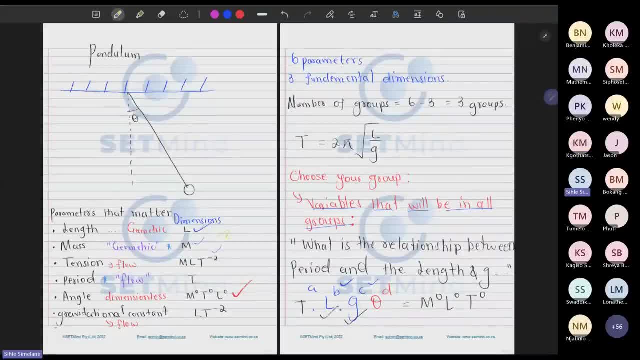 so let me think carefully. if i have one, two, three properties, i can make one, two, three groups. yes, this is okay. do we have anyone who has a question? why do we have four variables multiplying one another day? and why these ones? anyone in? in, in your constant group? what you are trying to achieve, you are trying to have. 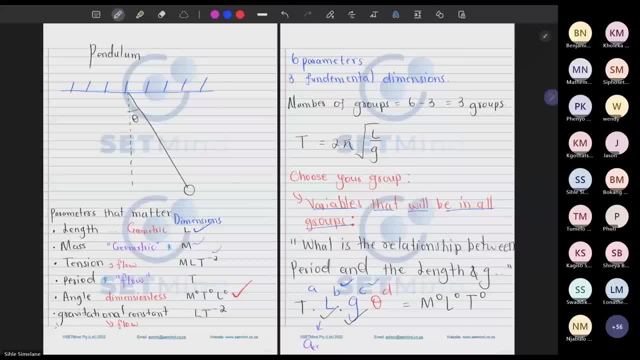 geometric, and then you are trying to have flow, and then the other variable is what will change, so meaning these ones will remain constant: geometric and flow. there's no viscosity here. the other variables are what we will change, so meaning all groups will have length, they will have the period. you'll have the period and then they will also have g. the only thing when i雨ilth have point should beada remains constant and then these vectors will continue, tied with the least. this is what could change. this will be small. all the g will havereiiettes. 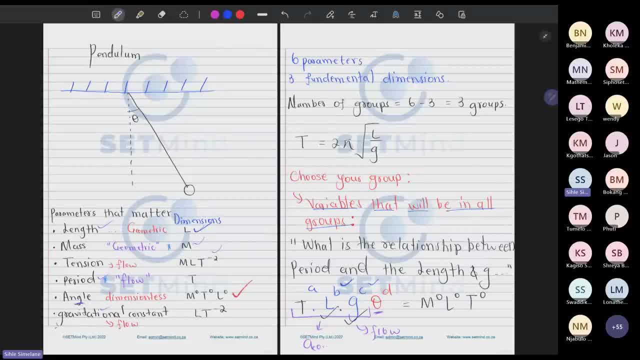 do group two instead of putting theta, the NL, I'm going to put change in, And so on. when I do the other groups, Are we all on the same page? Can I ask something? You can go ahead, So why theta is changing in other? 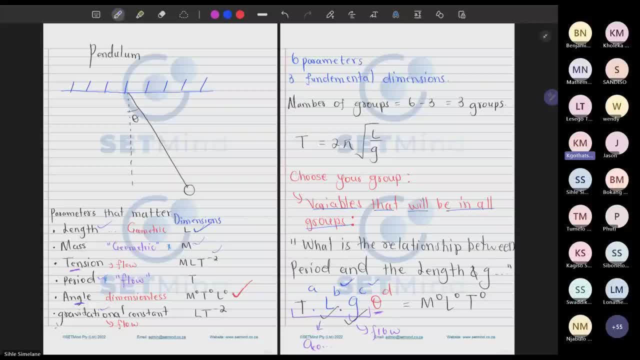 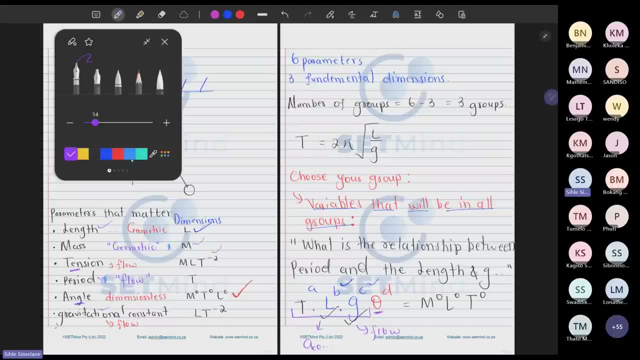 groups and T, L and G. it's constant. Is it because that's why you're trying to find out the relationship between them? Yes, So I have determined the variables. I want to keep constant, but I have to try and include flow and geometric. 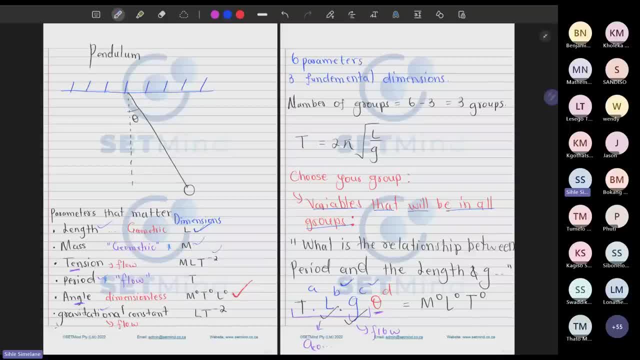 properties. The reason why I chose the flow and geometric properties is because they were looking for this relationship, The other variable. I can choose it to be something else. It's what I'm going to be changing constantly as we go. Does it make sense? 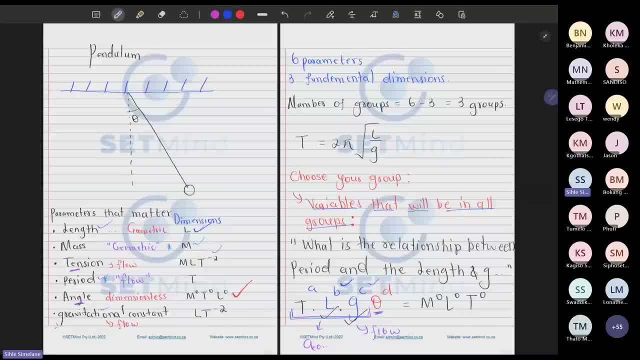 Yes, sir, Thank you. So this would be group one. I just need you to think of this carefully. It's really not complicated. So look at the variables which we chose to keep constant. Let me highlight them. So length is going to be in every group. 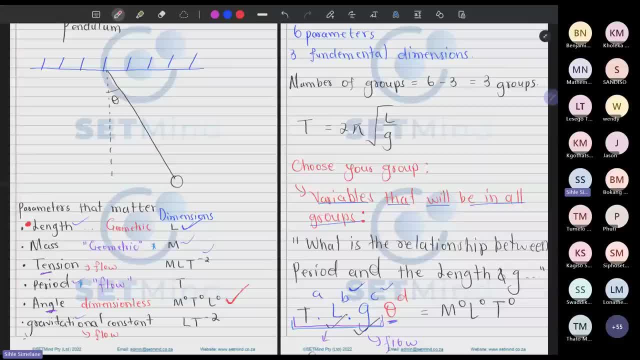 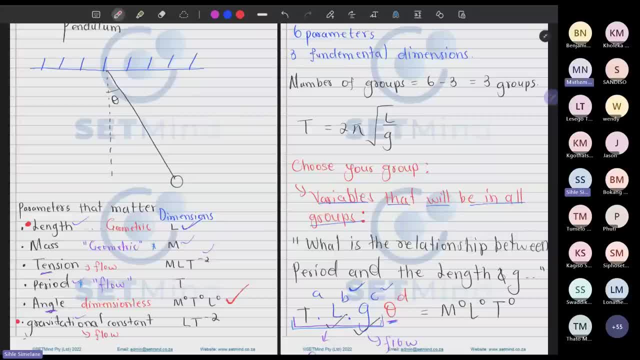 We don't have to do that. We don't have to do that. We don't have a fluid property, We would be forced to include it. Since we don't, it means there's going to be a reputation of some of them, So I chose the length. 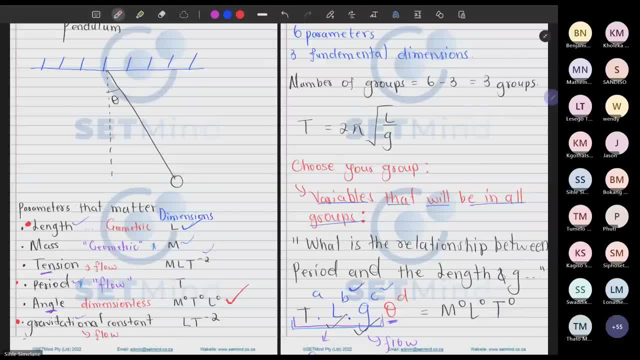 and the period, because they said we are looking for the relationship between the length and the gravitational constant. The other groups will then form the remaining groups, meaning group one will be formed by a combination of the three. with this one, That would be group one. 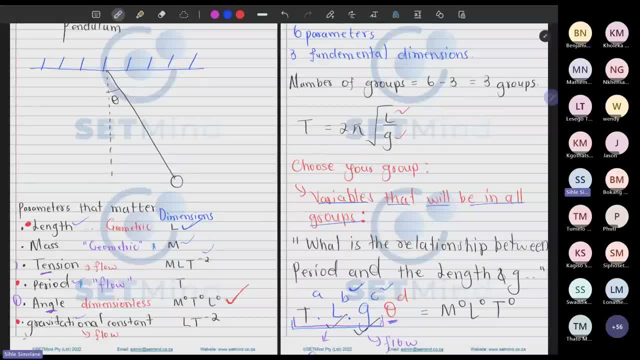 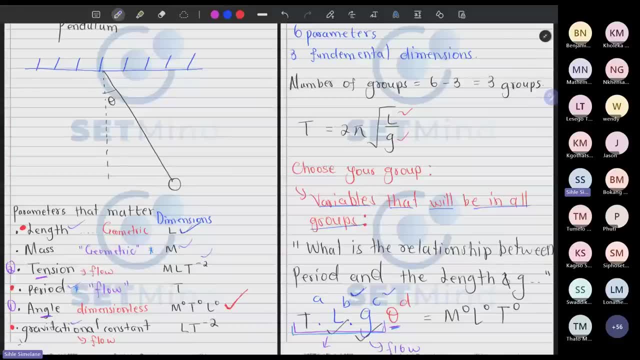 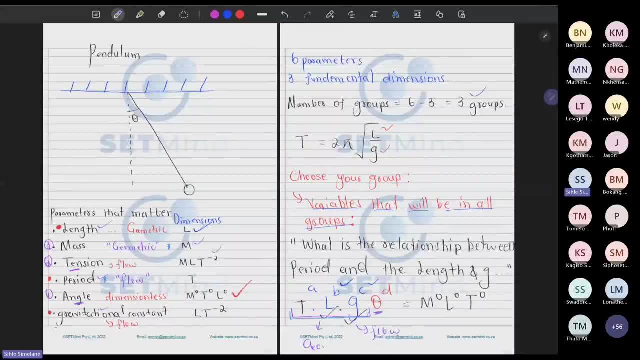 Group two will be formed by a combination of the red ones and the tension where there's theta. Group three will be formed by a combination of the red ones and the mass. That's why that's how we are going to get our three fundamental groups. 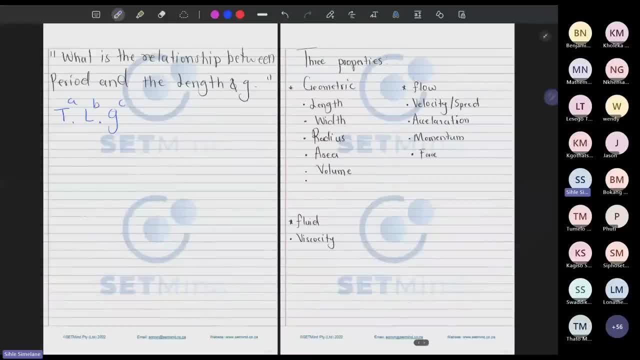 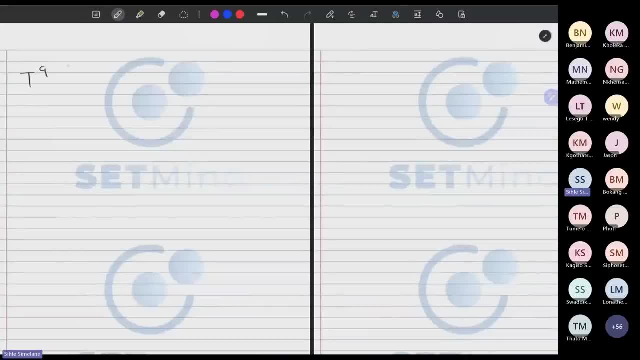 So let's focus on the one which we have here and quickly wrap it up. So what we have there is T to the A, L to the B, G to the C, theta to the D, M, zero, T, zero, L, zero. So our T. 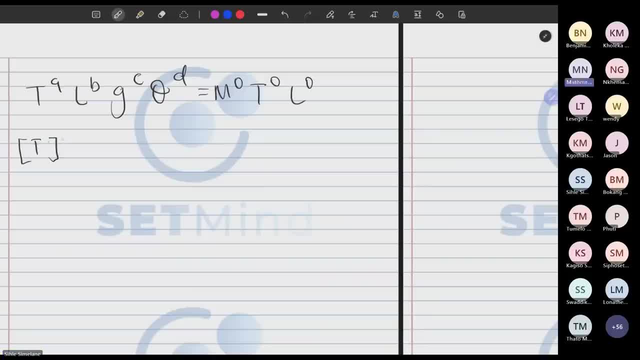 which is the period. it is just T to the A. Our L is just L to the B. Our G, which is acceleration, will be L, T minus two to the C, Our theta. remember that theta is dimensionally, it's dimensionless. So 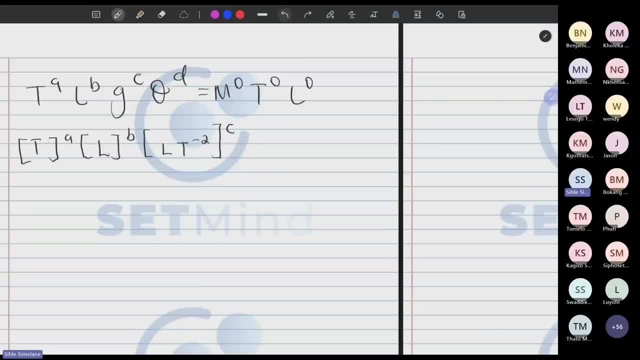 theta is just an angle, it's dimensionless. So I will just leave it as theta, just like that, Because it is dimensionless. It is not going to influence the M's and the L's. Remember that this is dimensionless. 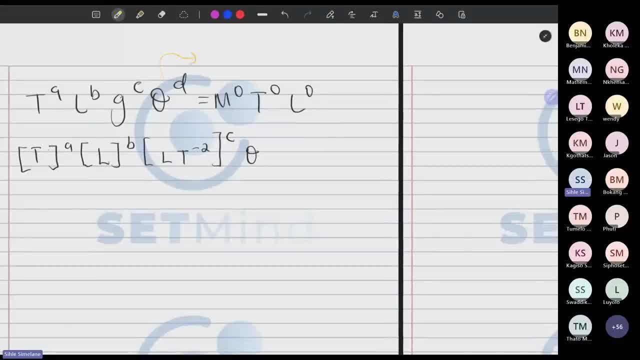 Theta is no length, it is no time and it has no mass Dimensionless, So I can leave it as such. when I'm looking at the dimensions: M zero, T zero, L zero, So let's quickly combine the T's here. So if you look carefully, 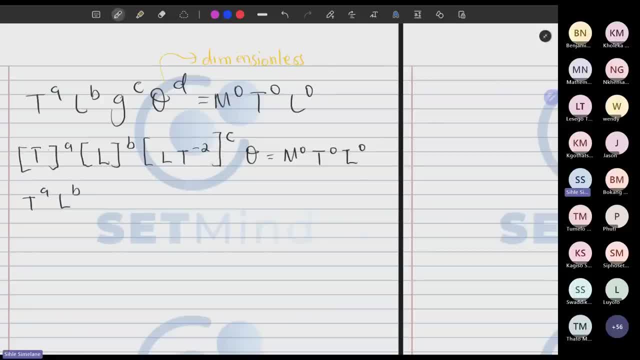 you have T to the A, L to the B, and then L to the C, and then T to the minus two C, And then I'll put this here, But when I'm looking at dimensions it really does not matter, So I'll put M: zero, T, zero. 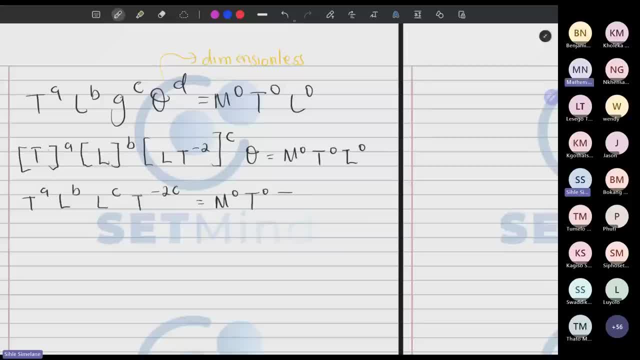 and L zero. So let's combine the T's. So when you look at the T's, it's going to be A minus two C. Then when you look at the L's, it's going to be L B plus C. Okay, there's no M here. 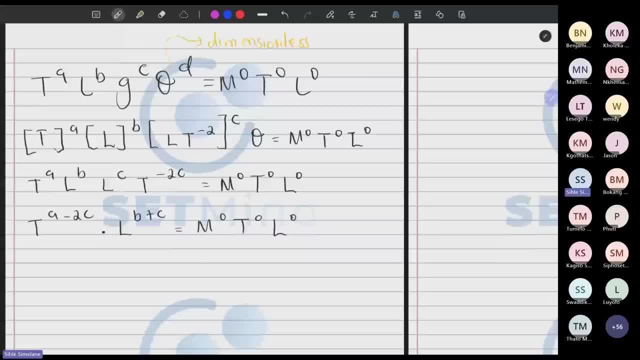 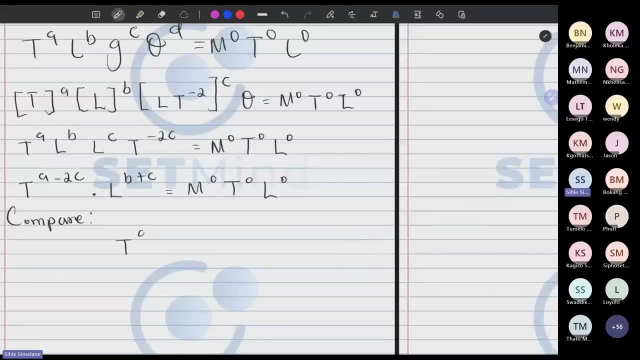 This would be M to the zero, T to the zero, L to the zero. So when we now compare, you can see that we have T to the A minus two C equals T to the zero. on the right hand side, Same phase, We equate the: 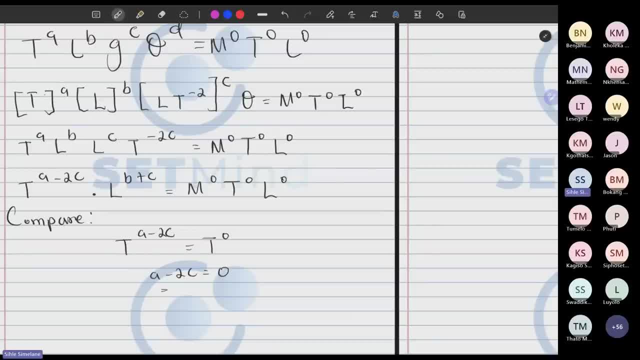 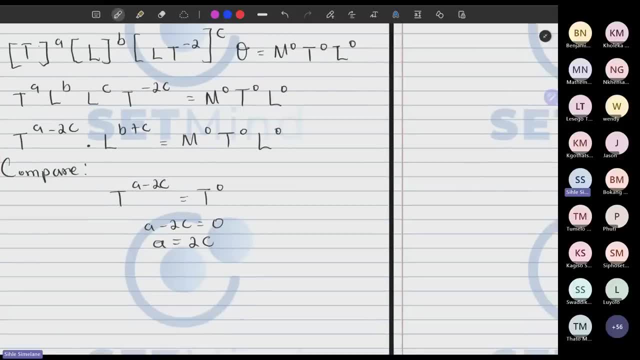 components. So my A minus two C equals zero. So my A becomes two C And the easiest thing you can do is to choose one. So, IE, we can choose C to be one And then, when we choose C to be one, 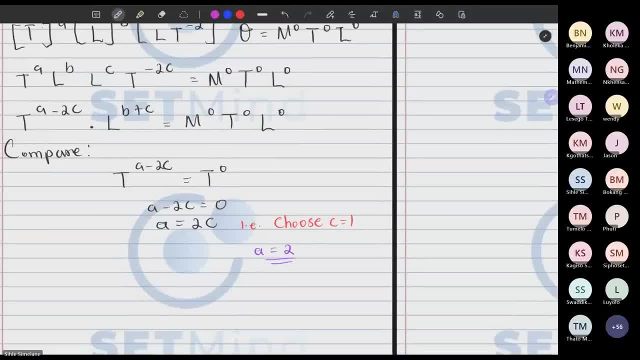 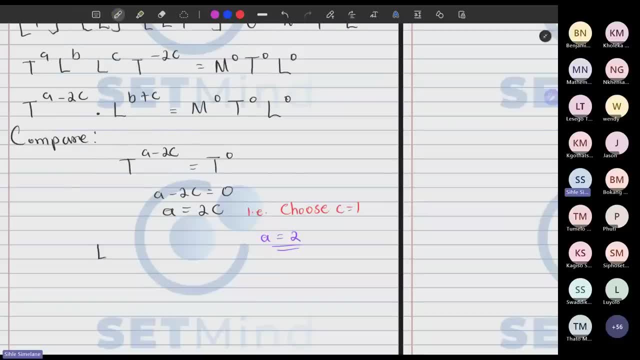 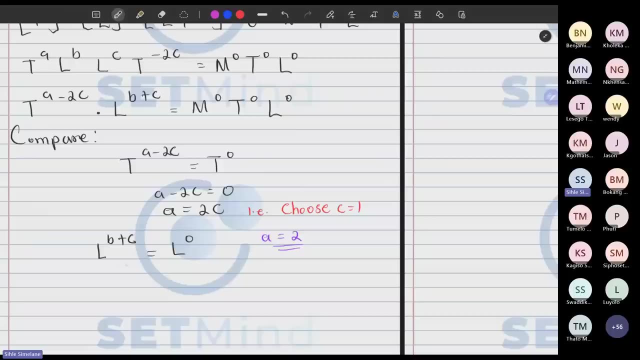 our A becomes two. Okay, let's go to the L's now. So if you look at the L, the left hand side, it is to the power of B plus C. The L on the right hand side is zero. So, same phase. we equate the exponents. 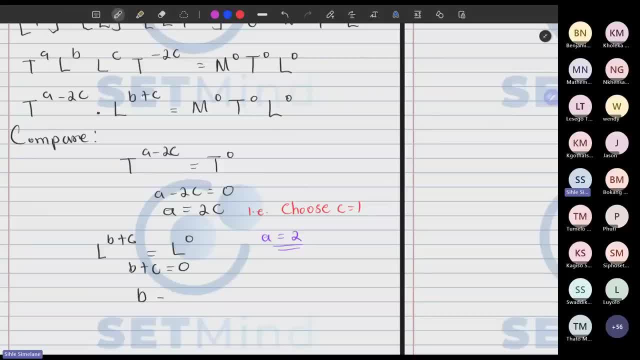 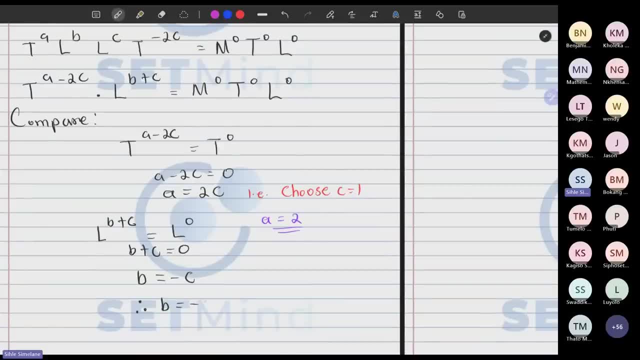 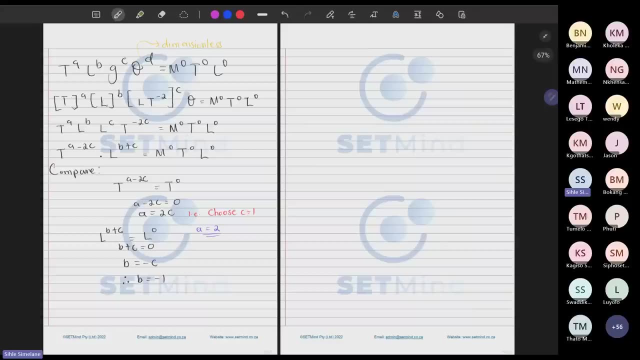 You have B plus C equals zero. You have B is minus C, But C we have chosen as one. so therefore our B is minus one. Okay, and now we can go and plot back there and say: our A we have found as two, So which means I have T. 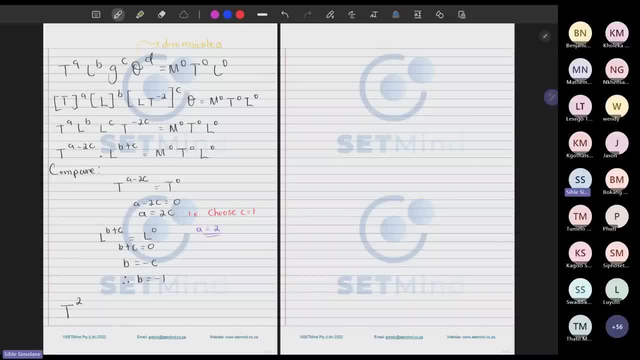 squared. And then L two, which is the length, L to the B. Our B we just obtained is negative one here. Our G, which is to the power of C, C is one, so we have G to the one. So, because our theta 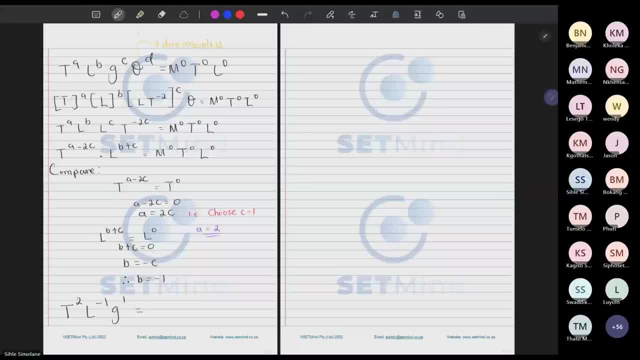 is dimensionless. when you, let's say, divide by the other side, we still obtain a dimensionless quantity. So let's call it pi one, which is just the dimensionless quantity, Pi one, where this is dimensionless. Okay. 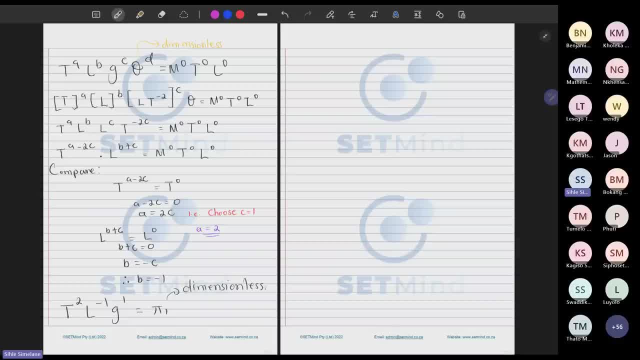 And then what happens here is that, if you look carefully, we have T squared over that, So we find ourselves with T squared times G over L, And this is just equal to some dimensionless constant, And we are trying to relate the period to these things, So we 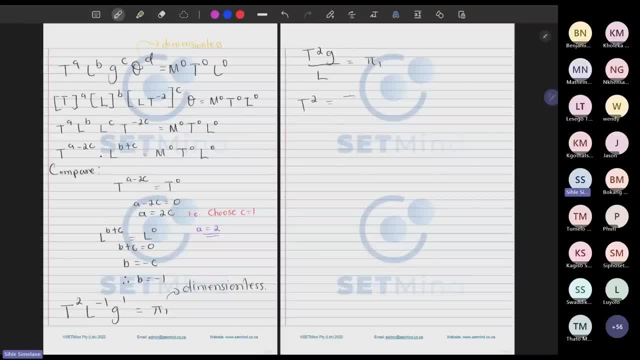 can multiply on the other side and have T squared is equal to pi one L over G. Since we are trying to look for the direct relationship, we can take the square root on both sides. We have pi one L over G and then the square root of that. 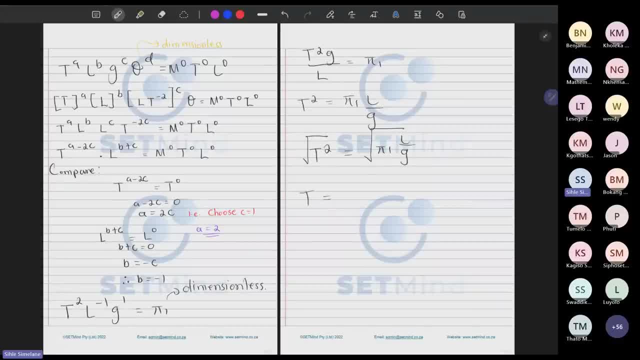 will be T is will have a dimensionless constant. When you square root a dimensionless constant, you get another dimensionless constant. Let's call it pi two. Then you have the square root of L over G. So this is how the period of a pendulum relates. 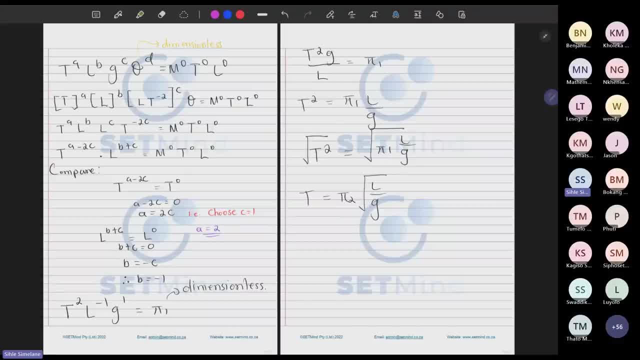 to the length and the gravity. And the question which you might start ascertaining is that: how did they find this constant here, this dimensionless constant? Well, when the scientists were working, they ended up finding that the time is two pi. 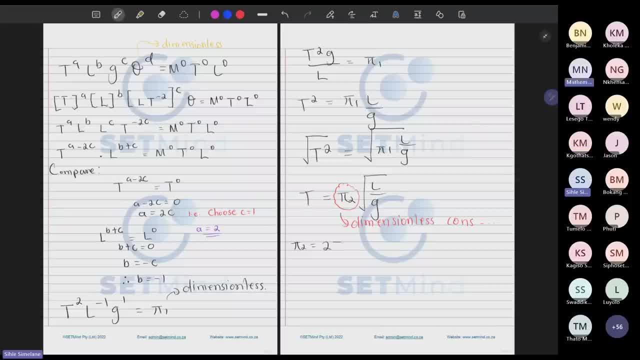 And they found it through experimenting. Yes, you can go ahead. What happened to the theta? So the theta is dimensionless. Okay, What I did was I just plumped it up and said it can be a dimensionless constant When we push it to. 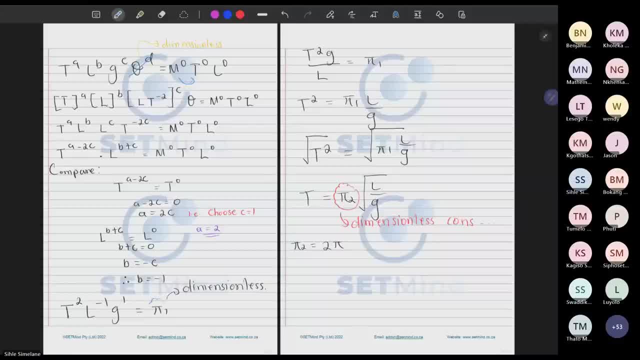 the other side, it lumps up with this. So anything which is dimensionless, you can equate it to whatever you want. I prefer calling them theta pi one or pi two to denote a dimensionless constant. So what we can do, if you really 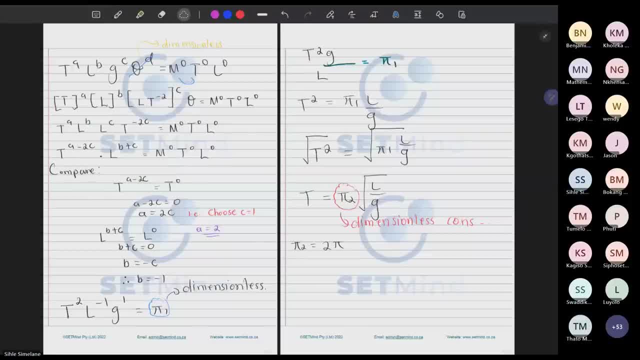 want the theta to stay, we can put it in here, But remember that it is really dimensionless. It doesn't make that much of a difference. We can put the theta here And then afterwards, because we are solving for the t, we'll find. 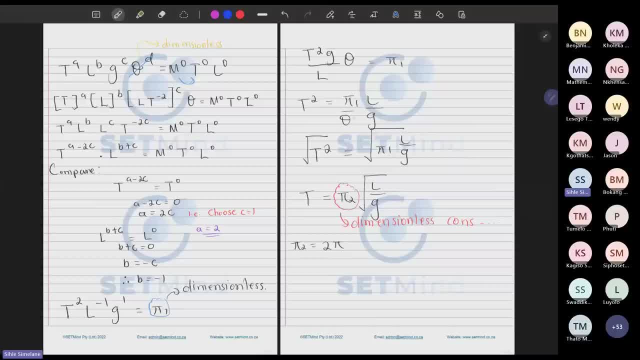 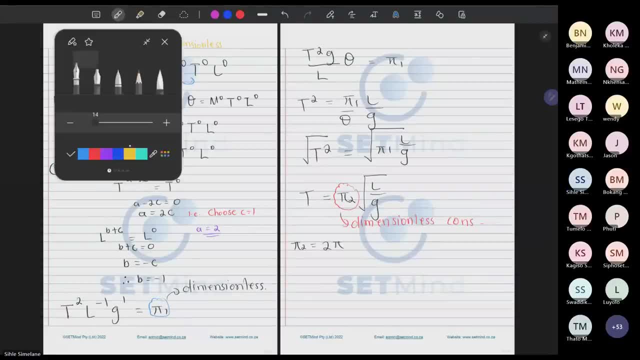 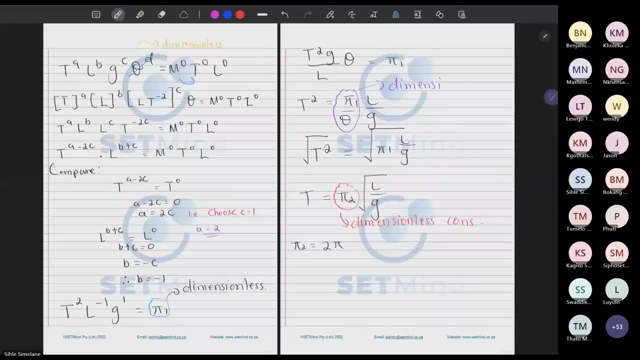 ourselves dividing by the theta. But a dimensionless constant divided by a dimensionless constant gives us another dimensionless constant, Do you agree? Yes, So what we have here is simply a dimensionless constant being divided by another one being divided by a dimensionless constant. 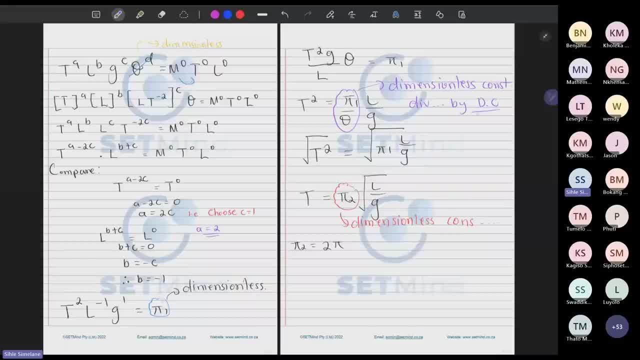 So the answer you get is still a dimensionless constant. There's no ml which is going to emerge, which we need to stress about. Then, when you square root a dimensionless constant, you still get a dimensionless constant because the l is not. 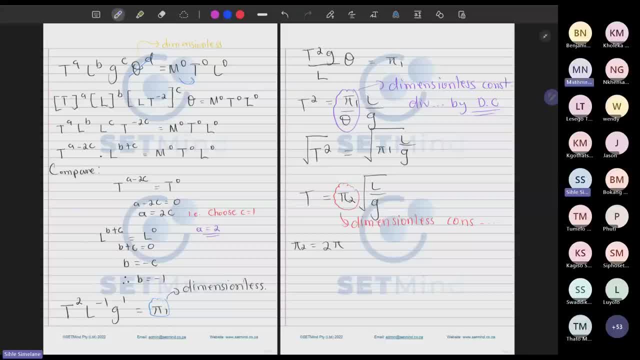 going to emerge out of nowhere. Does it make sense? Yes, So this is the equation which, using dimensional analysis, we find, which relates the period, the length of the pendulum and the gravitational constant, And in that dimensionless constant they found: 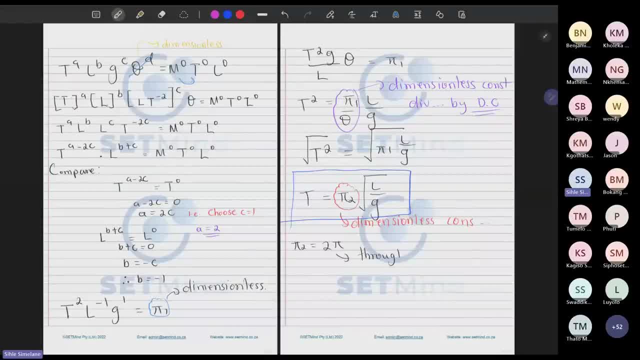 to be 2 pi, and this is through performing experiments. That's how they found that dimensionless constant has a dimensionless constant, That 2 pi. actually, when we put it there, that's the constant which will make us to be able to obtain the period. 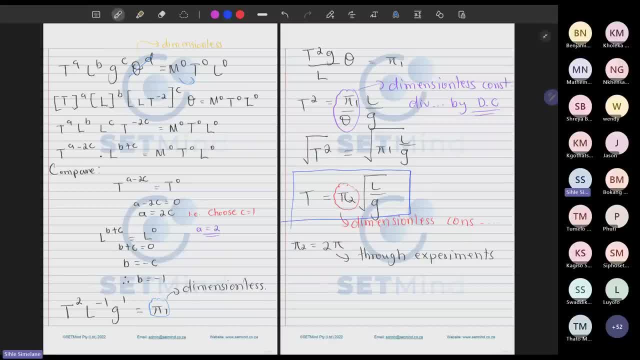 So this is how you would go about dealing with this problem. Do we have any questions, Sir? Since you said like, when we're calculating the number of groups, we found out that we have three groups right, And meaning that I don't know, we have to. 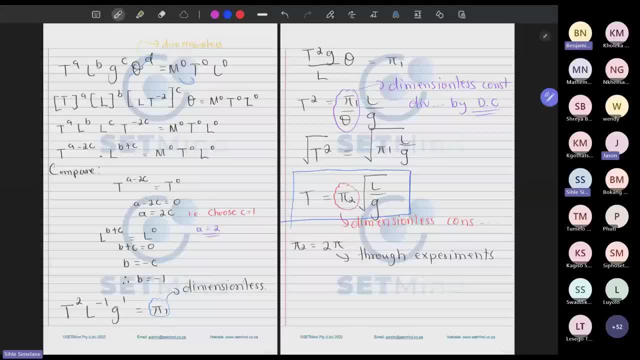 sort of like a three, can I say three equations, Three solutions. For this one, if the questioner was saying we should find the relationship between the period and the length and the gravitational constant, this would be the solution. The other solution would be: let me. 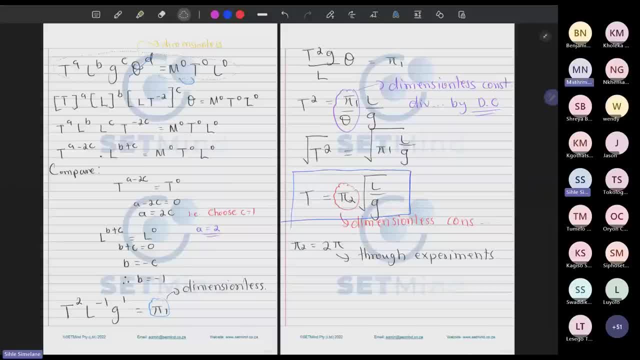 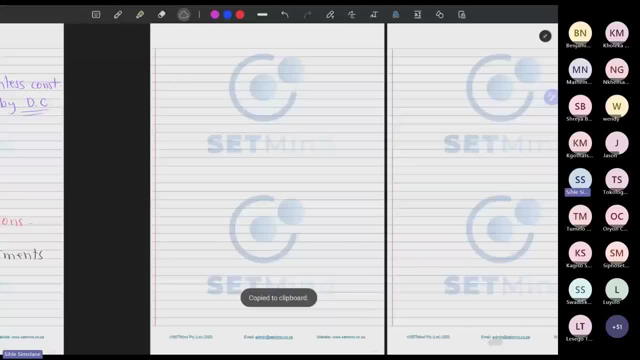 copy that, because three groups means you need three solutions: Copy and paste. So let's go to that. So the two will not change, These three will not change, One will need to change. So look at what we did here. We have utilized: 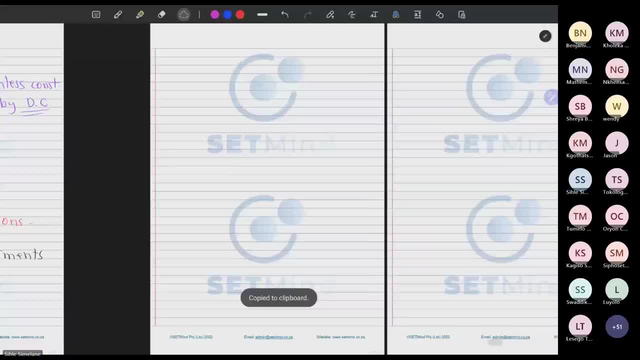 the NL as group one, Group two, we need to utilize one of the things which was not there. We can take tension, but we will get the same answer with these variables. I can see that ahead. So, for example, let's take mass. 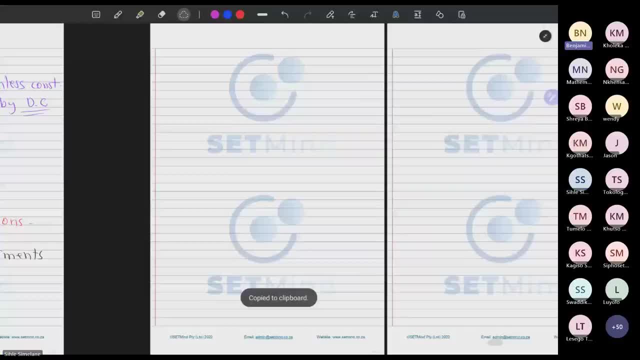 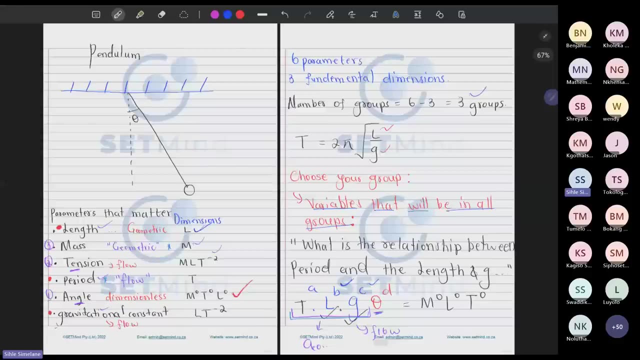 Let's put in mass here: M0 and then T0 and then L0.. So when you break this apart, let me copy the work we have done already. No, this should not be here. Let's copy it and come Here. 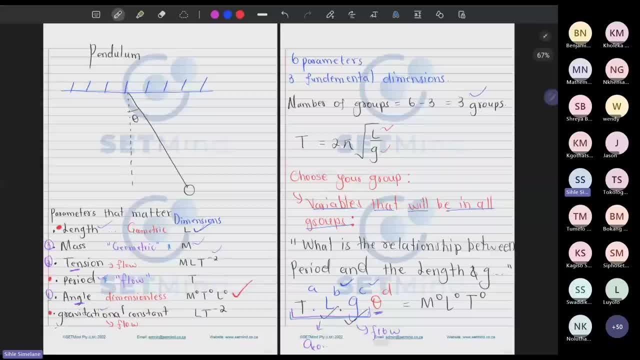 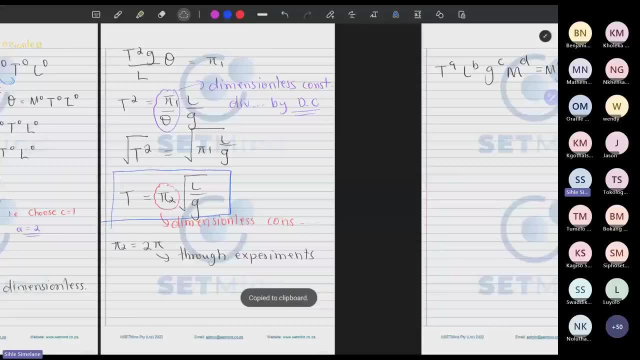 So I need to put MD here. So let me copy where we are breaking them down, which is here: Copy and paste, Okay. And then the only difference here will come and put M to the D To the D. Do you see that? 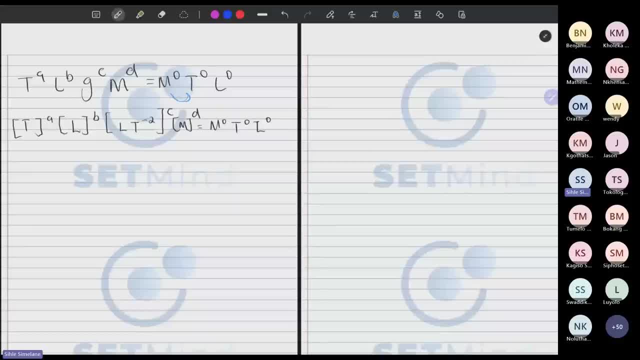 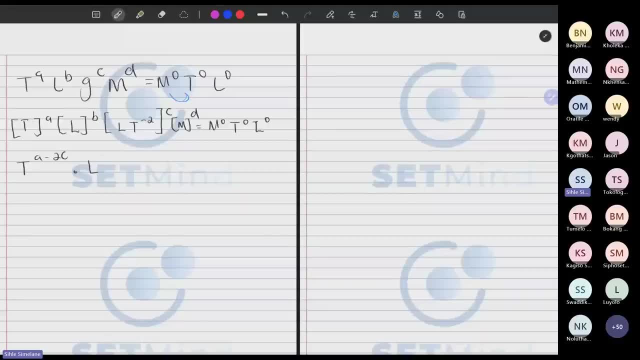 And then, when we collect the T's, we'll obtain nearly the same answer. So A minus 2C, That's the T's, and then the L's, It's the B plus the C. B plus C, yes, And then the M. 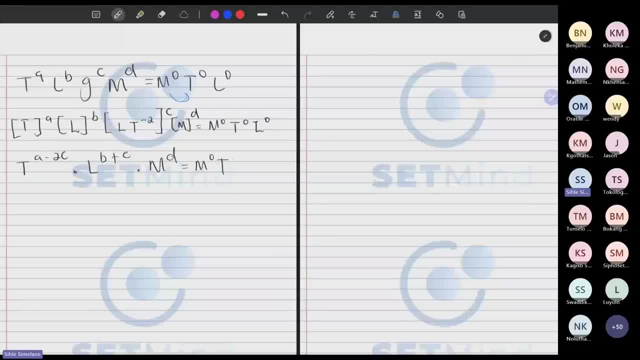 is M to the D, And then we have M0, T0 and then L0.. So when you compare, if you look carefully, when you compare the M's, you'll have M to the D equals M to the 0, which 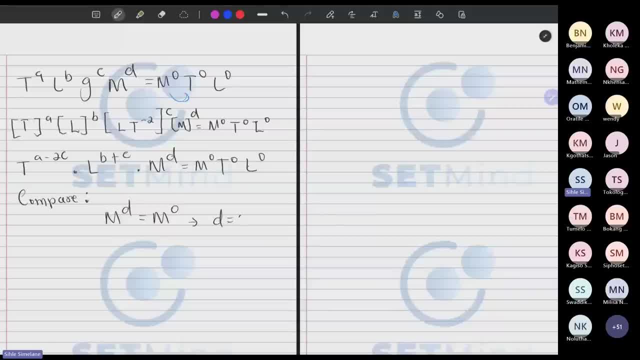 means just D is equal to 0. And then all the other solutions. they will turn out just like the other one. So when we do T, we'll have A minus 2C equals T to the 0. You'll have: A is equal to 2C. 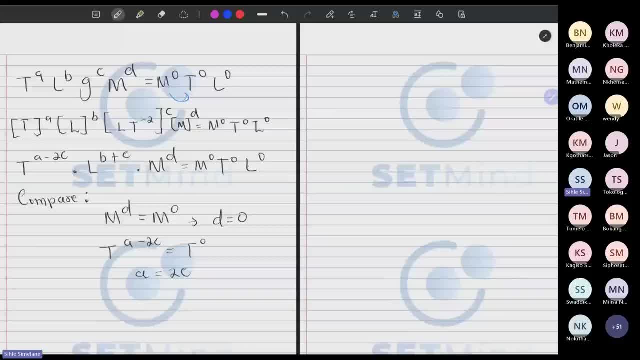 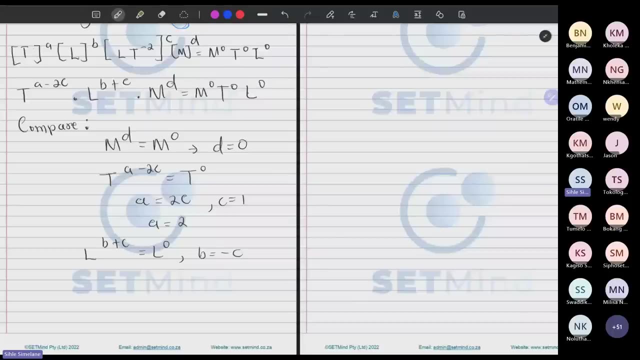 You can make exactly the same assumptions where you say C is 1, which makes A to be 2. And then, when we look at L, you have B plus C equals L to the 0. And you have B equals negative C, which. 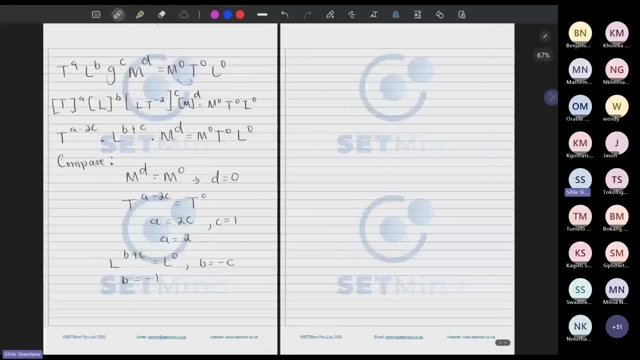 means B will be minus 1.. So when you substitute back, you can see that the D is 0,, meaning how the period, the length and the gravitational constant are related is independent of mass, And that should have been an experiment which you did in physics. that 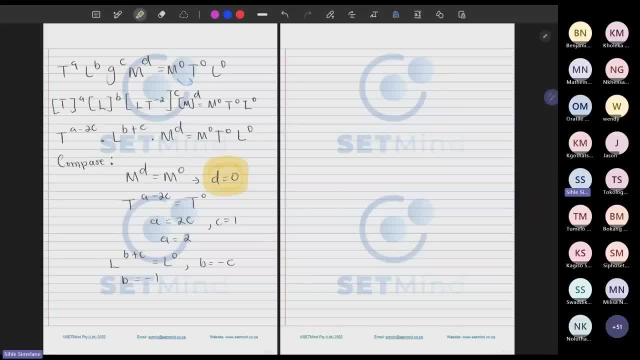 the mass does not affect the period or how the period, the length and the gravitational constant are related, Because you see that D is now 0, which means when we go up there we'll say that T to the power of A, the A. 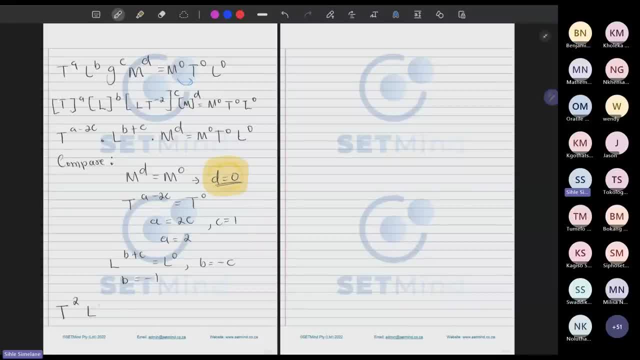 we obtained as 2, the B, we obtained as negative 1, the G, the C, we obtained as 1, and then our M is to the power of 0, and this will be equal to a dimensionless quantity. So which means: 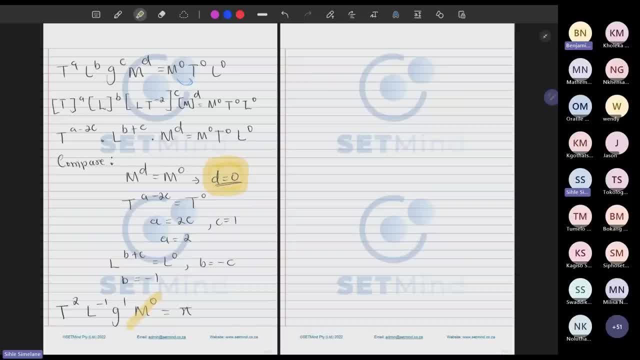 actually how the length and the gravitational constant are related is independent of mass. That's what this would mean. This solution would be telling us that the relationship between the period, the length and the gravitational constant is independent of mass, Meaning whether what you are hanging there is heavier. 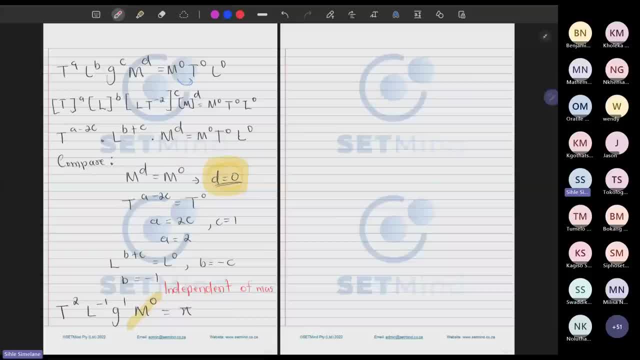 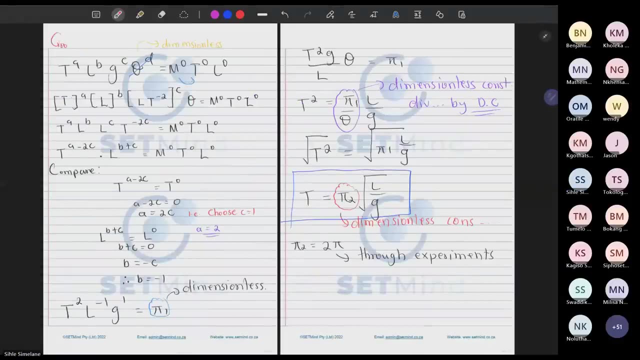 the relationship between period length and gravity will always be the same. Whether you make the mass to be smaller, it doesn't change the period. This would be group 2.. What we were dealing with was group 1.. In group 1, what it's saying essentially. 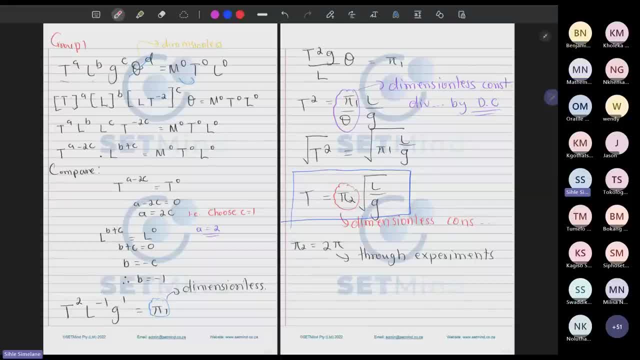 is that the relationship between the period, the length and the gravitational constant is really not much affected by the initial angle, Whether your friend makes the angle to be bigger. what they need to know is what is the length and what is the gravitational constant here. 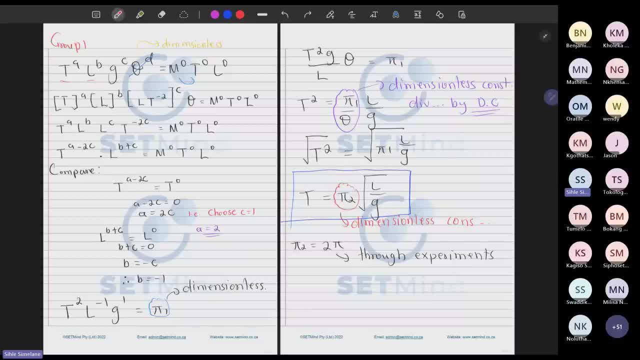 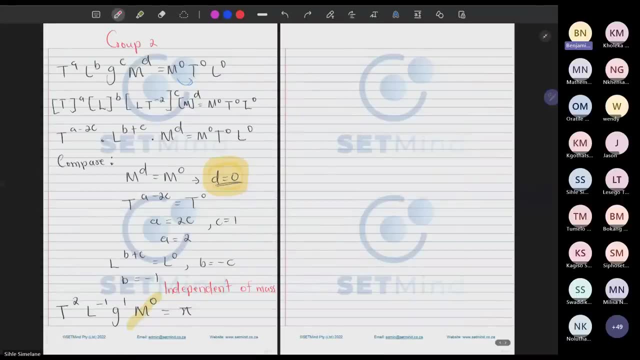 in this lab here, WSS, Then they will be able to tell you the period. Whether someone pulls the angle to be bigger, it doesn't make the period to be bigger. Does that make sense? Yeah, it makes sense. So, since we get, 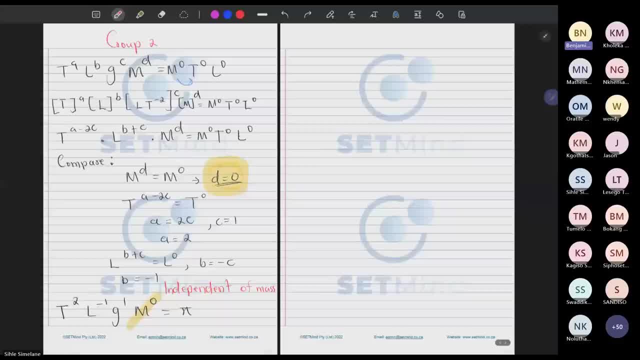 the same answer. but is it necessary for me to write all these three solutions, or I can just write one when I'm in the test? For example, they were just saying to, let's say, just find the relationship between the period and the length and the 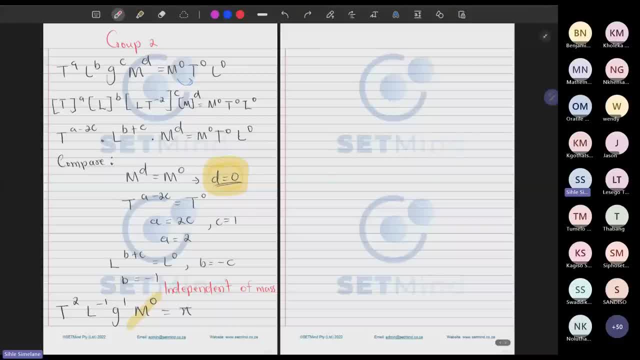 gravitational constant. You would just do one solution and you are done. But then you see to the mass. you would do the other solution and show them that really there's no relationship to the mass because these parameters are independent of the mass. It depends on the question, but my 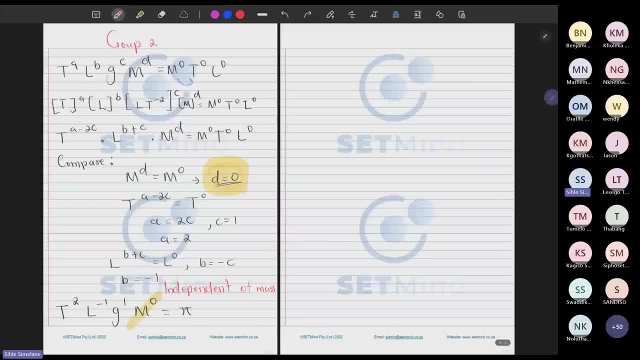 advice to you is: you'd rather do more work than do less work, Because one mass is what differentiates a 49-4 to a 50, and it also differentiates a 74 from a 75. So you'd rather do more work if the 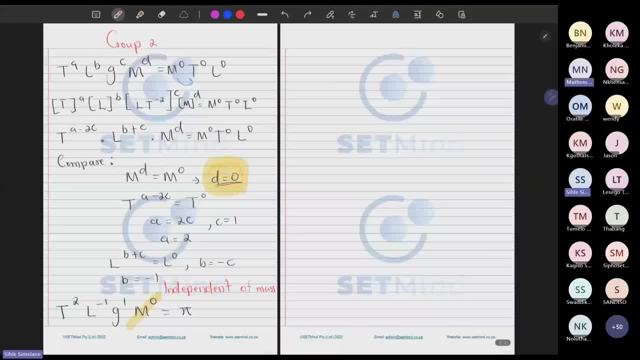 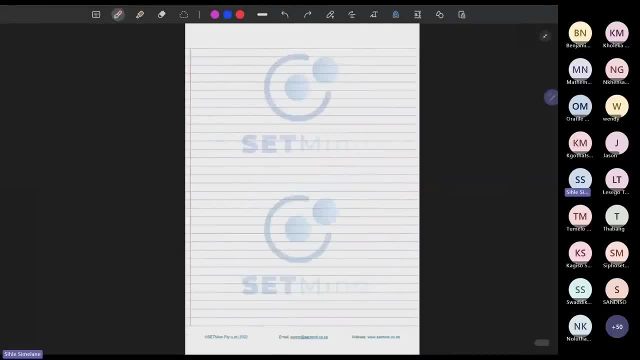 question is not clear, but normalize asking in the test or exam setting. Raise your question and say: look, I've spotted here that I need more than one group. What should I do? Are you expecting me to do all groups, or I should focus on the question where? 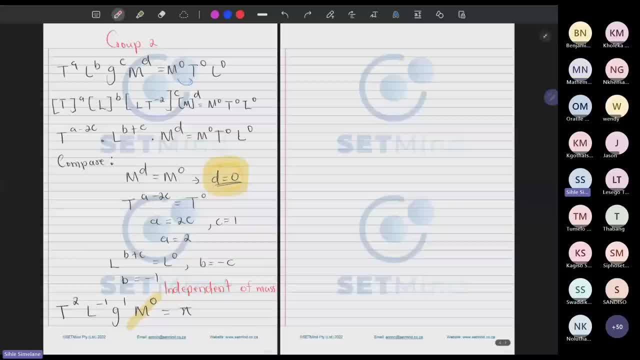 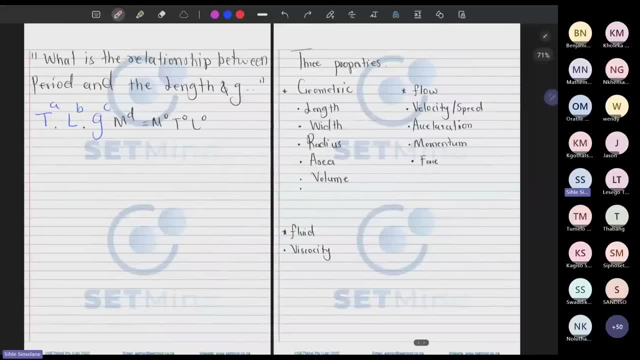 they are saying: just find how this is related to this. You construct that group and then you have what is done. So this will be the first, I think. when you look at your study guide, the pendulum is the first problem which they present there. 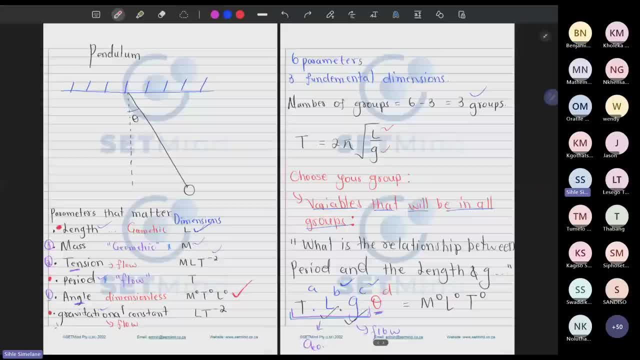 You should have a look at it And the pendulum. obviously you can always introduce many things because there's different pendulums. There's pendulums which are 10, so they will introduce another fourth here. But do we have any questions from? 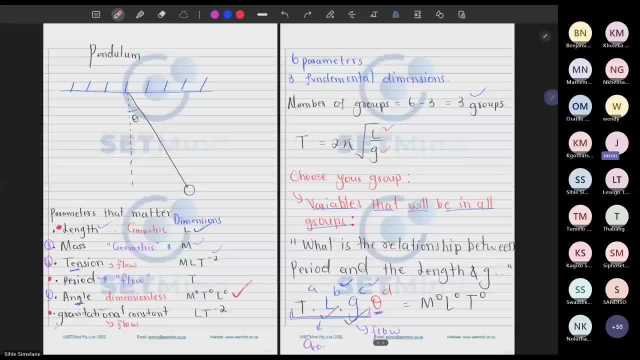 anyone. Yeah, I've got a question, sir. I wanted to ask, when you're selecting, which variables you're going to keep constant changing. so you chose to change mass period and the angle. So my question is: how does 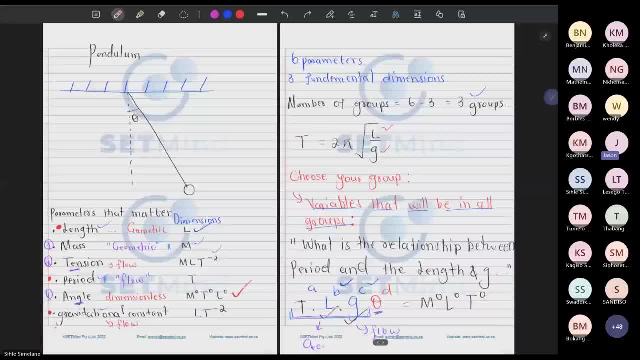 mass tension and the angle. So my question is: how did you get tension to be a changing variable? Okay, so here's what I mean when I change variables. So you need to decide on three variables which you are going to keep constant. 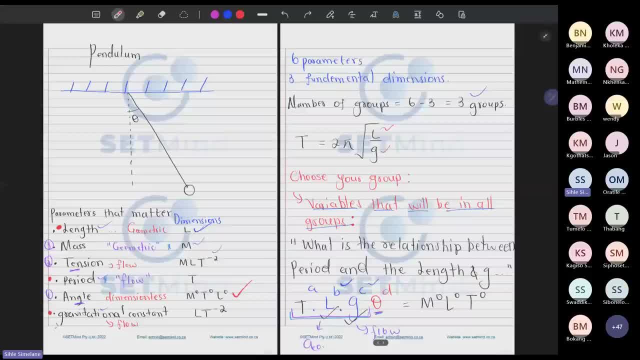 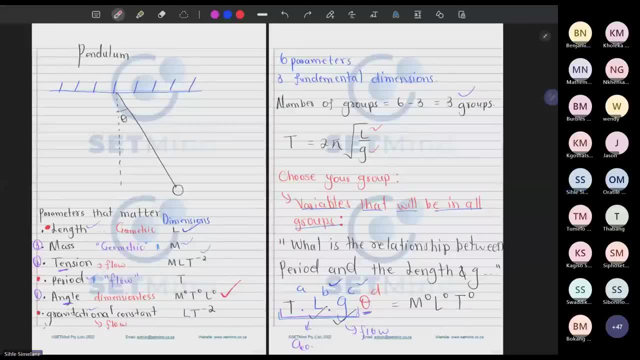 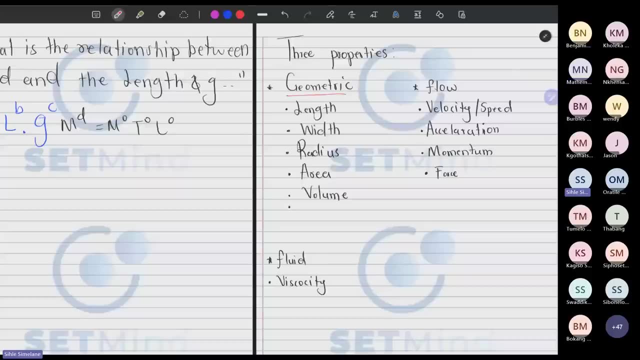 And then you will vary the others. So the three variables which you want to keep constant- ideally they should be in those variables which you want to keep constant- There should be at least one geometric and then there should be at least one flow, at least. 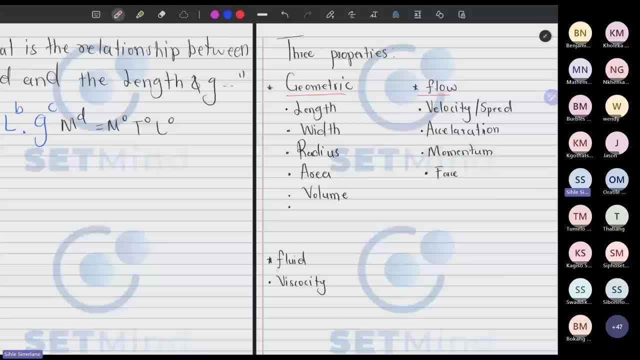 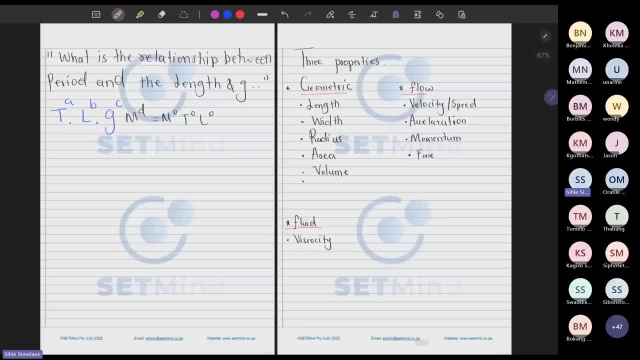 one fluid. But if there's no fluid, it means in the variables, which you will keep constant, you can't put fluid because it is not there. So when you look at our problem, they were trying to make us to find how is the period. 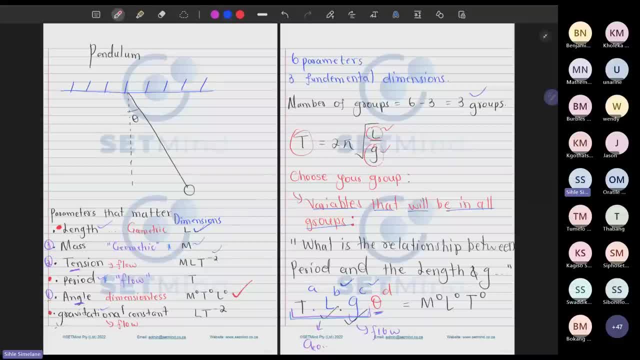 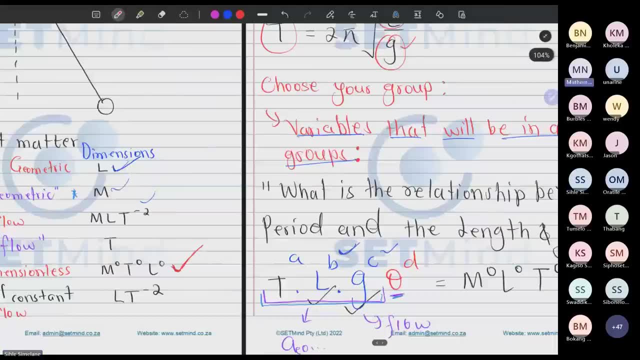 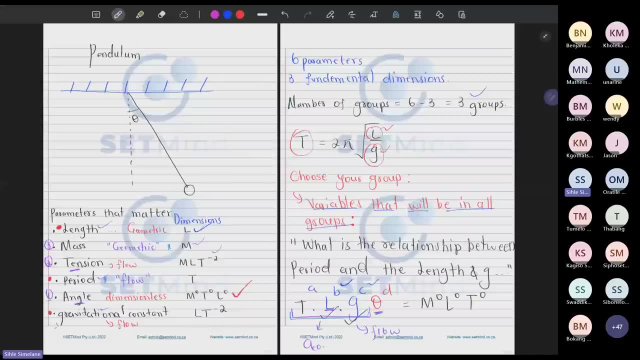 related to the length and g the gravitational constant. So when I looked at my problem I was like: okay, cool, It means I need to have length in my group, because that's what I'm looking to relate And length is a geometric property, That's. 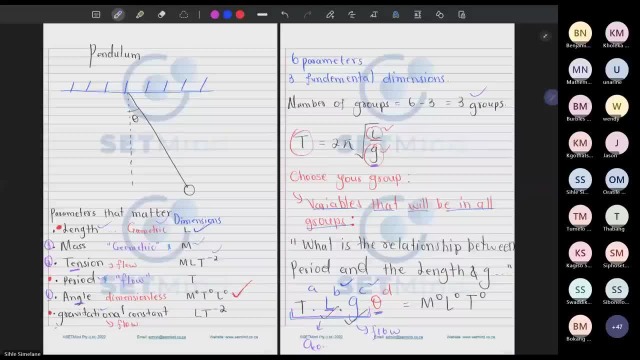 okay, It means I need to have g, which I have, and g is a flow property. Do I have any property which describes viscosity? And the answer is no. There's no property which describes fluid, And viscosity would be the property which describes. 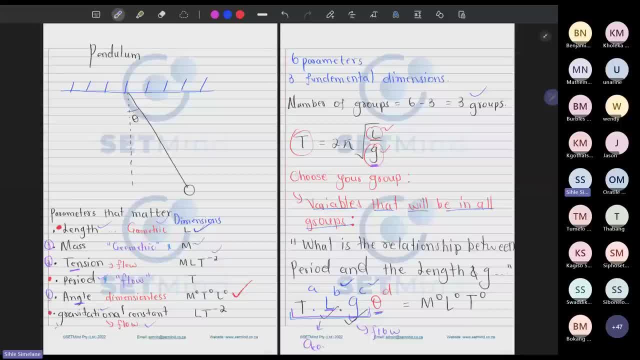 fluid, but we don't have viscosity here, So, which means I'm forced to take another variable here, whether it's geometric or it is flow. I can repeat one of them, But when I look at my problem, I need time. Time is a. 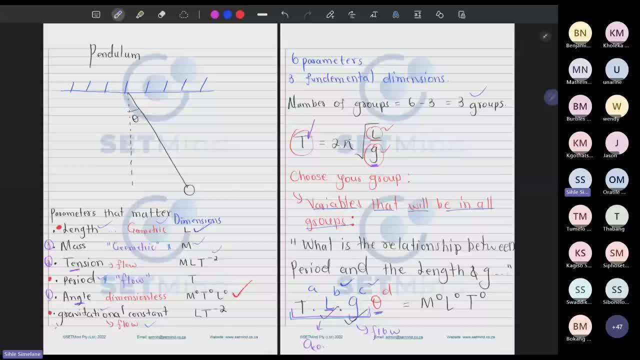 flow period, flow property. So I'm just going to put the time here. Now that I have these three, it means I'm done choosing those three variables. Now I need to vary the groups and put in the ones which are left, So meaning one of the groups. 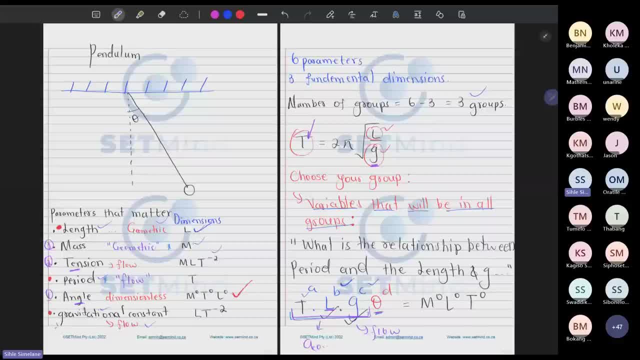 will have one of the variables which I didn't choose, which is angle. That's why it's here. The other group will be the same with the t, l and g. The only difference is I'll put in mass and put in a, d on top of mass. 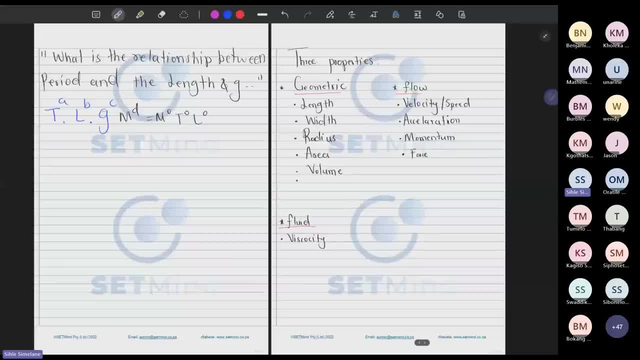 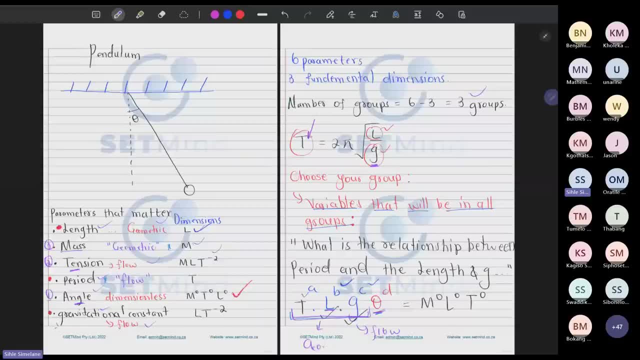 which is what I did with this problem, the group two problem. The group three will be: I didn't do anything with tension, so I need to include tension. I'll put tension to the power of d. That's how I formulate my groups. 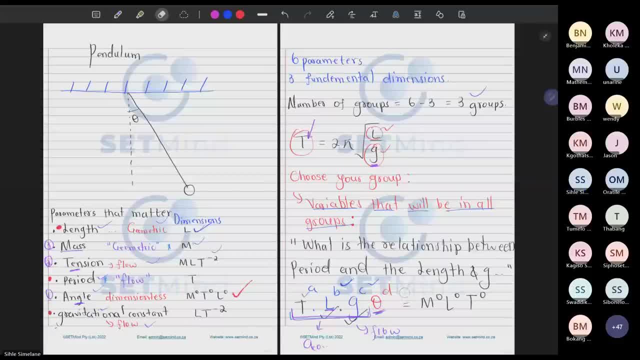 Does this answer your question? Yes, yes. So then also going back to the flow one. So you said that you chose time Because it was the only available option that was related to the geometric. No, So I chose length, which was geometric. 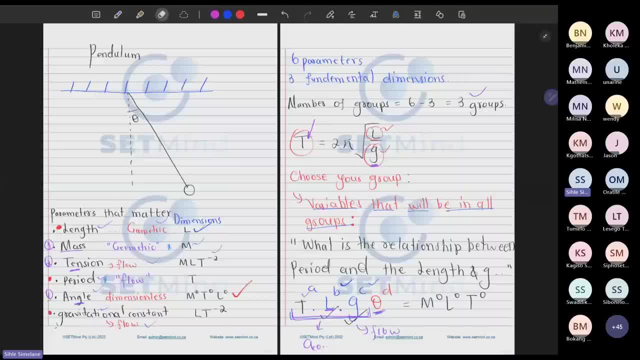 Agreed. And then there was mass. Look at how I chose it. It's because already the question was: how is period related to length and mass? Okay, So length is a geometric property. It occurred for me to put it in as one of the 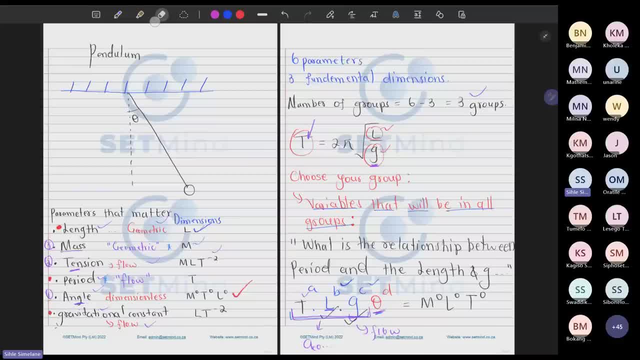 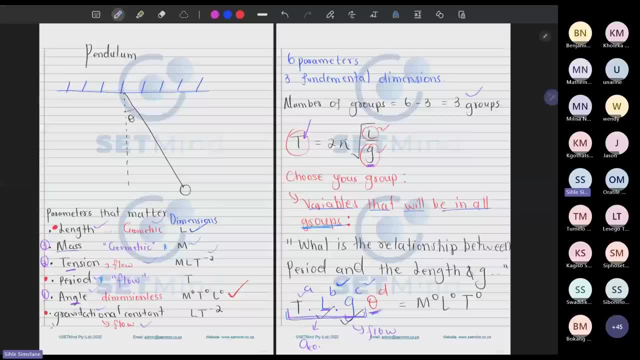 variables which will not change. That's why I said here there will be variables that will be in all groups. So length is a geometric property, So I'm going to put it in. I need to now look for a flow property, But 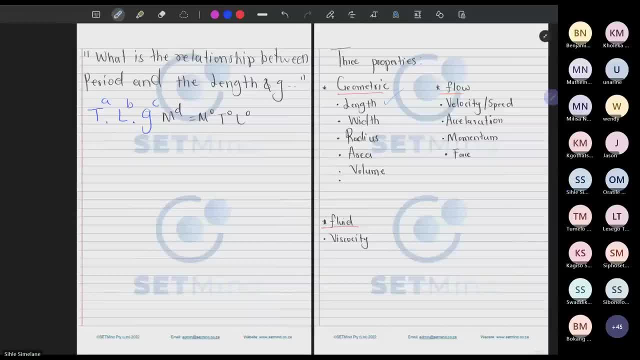 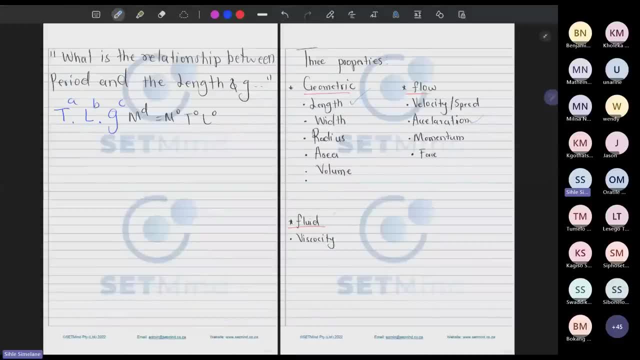 already. I know that g is a flow property, so I'm going to put g, And there's my g, which is acceleration. Then now the question I need to ask myself is: do I have a fluid property? Well, the problem doesn't have viscosity. 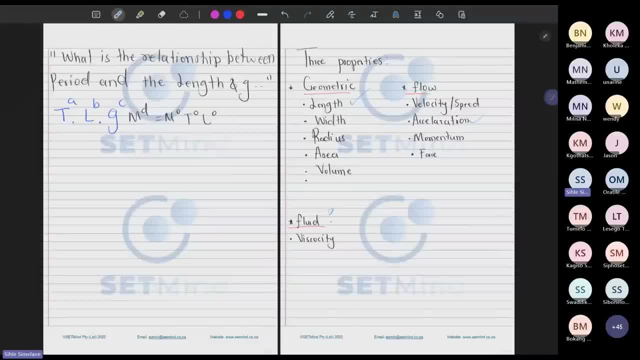 so no. So, since I don't have a fluid property, it means I can repeat either a flow or a geometric property, because I need three properties which will be there, which do not change in my group always. So, since I don't have, 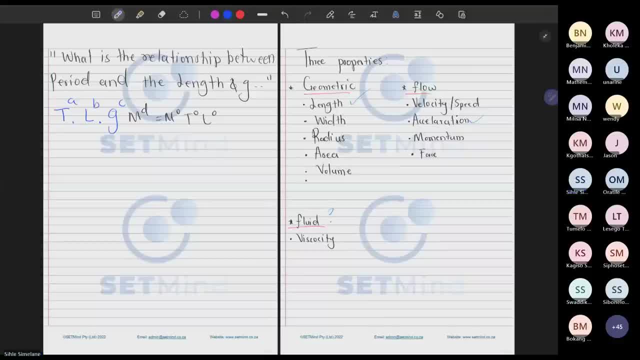 a fluid property, I'm going to repeat a geometric or a flow property and then change all the other variables which are left, Putting this one for this group, putting the other one which I didn't put for the next group, but the three variables. 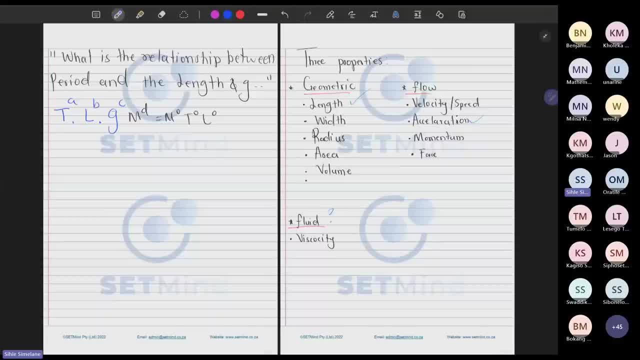 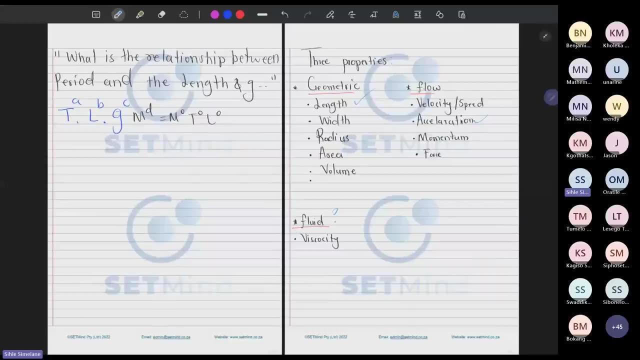 which I choose here, should remain constant. So length has been chosen, acceleration or gravitational acceleration has been chosen. Since I don't have fluid, it means I need to repeat either geometric or flow, because I need three variables which will not change. So when I go to my question, I'm like: 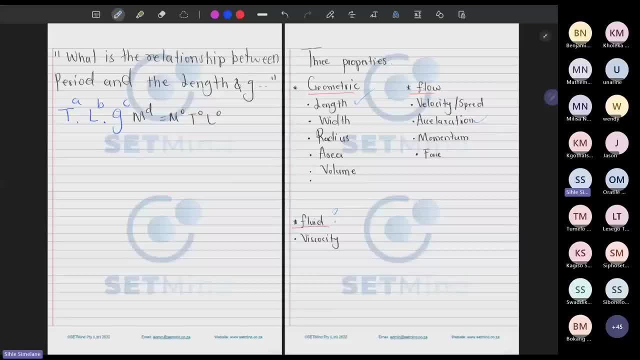 okay, so l and g are accounted for. but then there's t, But t is still under falls, under flow, so I can just put in t, because I'm forced to repeat either flow or geometric, because fluid is not there. 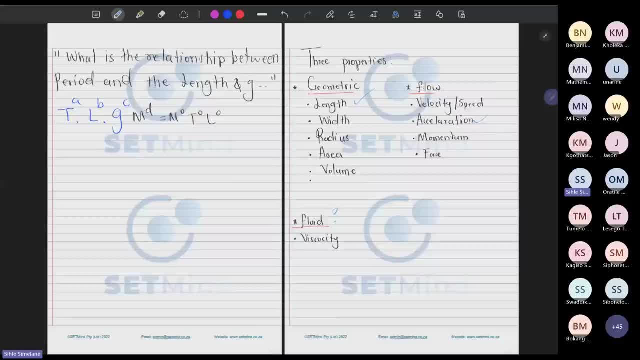 So that's why I have the t here. So these three variables will always be in every group. The only thing now I'm varying is that one. That's the one I'm changing. Now I have theta. The next one, I'm going to go to my variable. 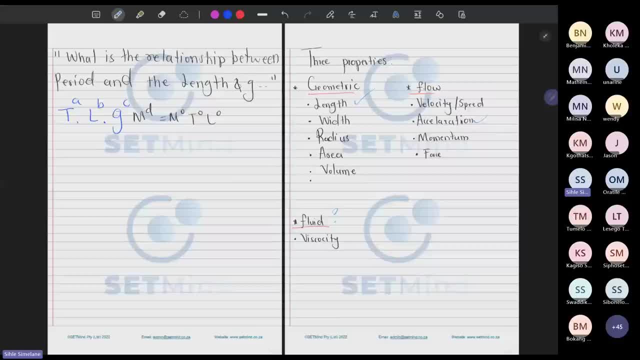 and say I didn't put mass anyway, Let's put mass. That would be group two. Group three, the last one, I'd say I didn't put tension. Let's go and put tension to the power of d there. That's how you change them. 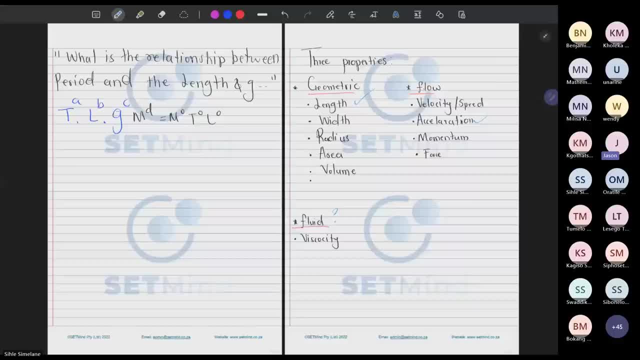 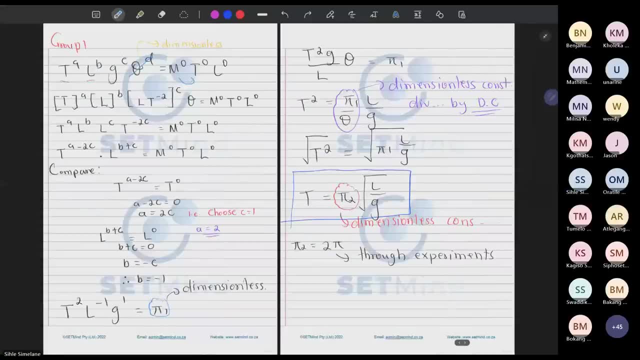 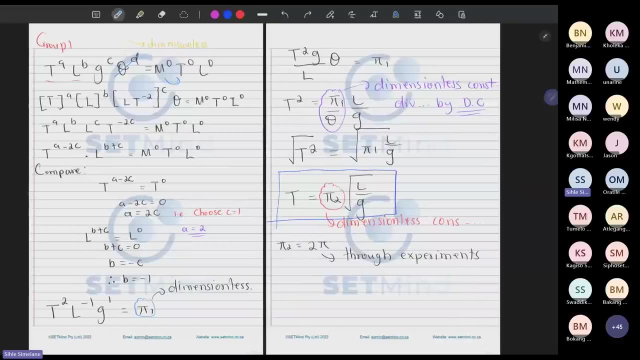 You understand? Yes, it makes sense. Okay, no problem. Any other questions from anyone, Please shoot. The ground is open and things will not start making sense after the session. So instead of saying what was he saying, or asking what he's saying, 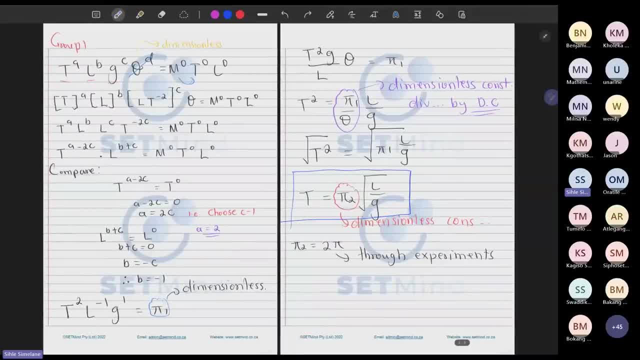 it was really not going to be useful after the session to say what was he really saying here. Sorry, sir, I have a question. Yes, Sir, can you hear me? I can hear you. Okay, Let's say now I'm in an exam. 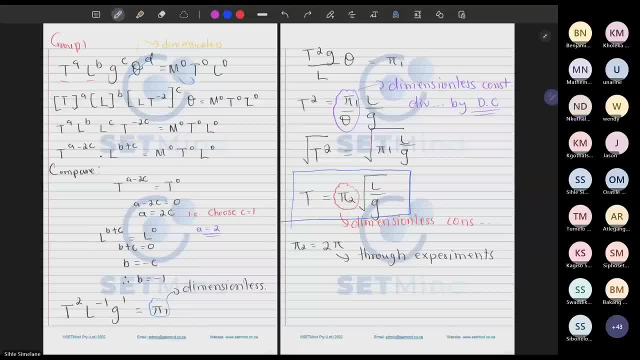 and I want to choose these variables or parameters that will be constant and the one that will be changed. Let me say I forgot the process that you just explained. Am I wrong when I say the parameters that are in the question will be constant? 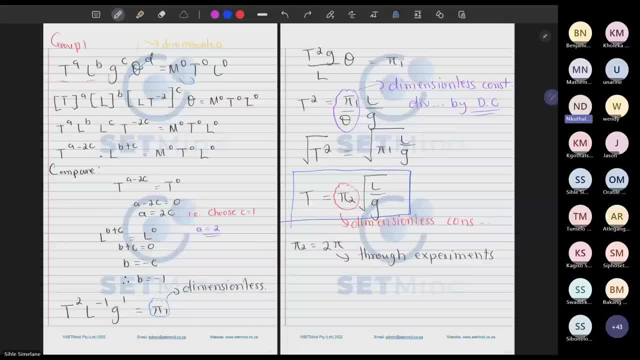 then the others that are left out, I'll interchange them to find the critical groups. Okay, so you're saying the parameters which are in the question, which are the ones they want you to relate, you will keep them constant and then you interchange the other ones. 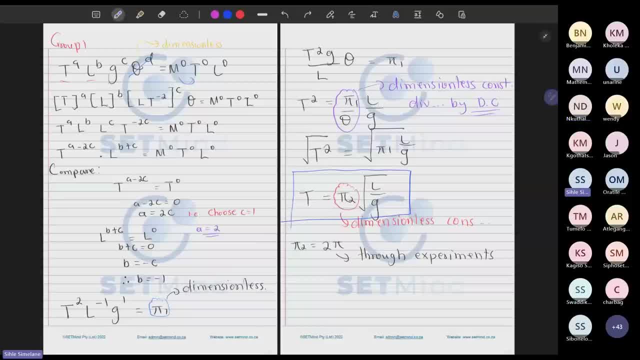 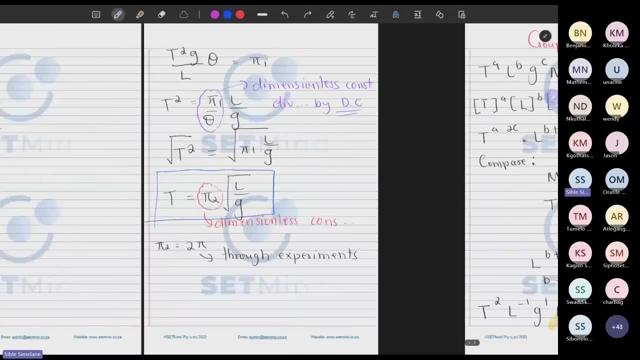 Yes, Am I wrong? or Sounds smart. I think it can work, I believe it will work, So it's one smart way to go about. My suggestion is: you can do that, but really remembering these is not hard. Just think you're like geometry. 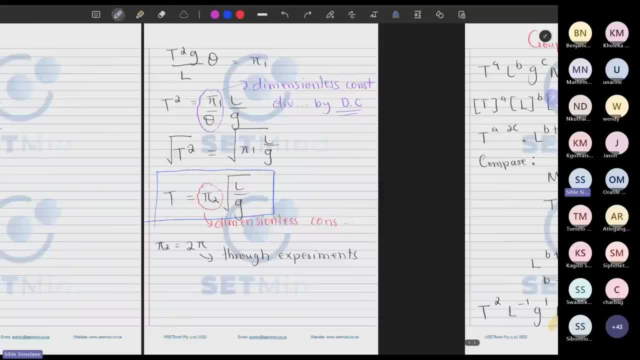 when they speak of geometry, obviously the same volume, area, width, whatever Things which you can easily measure with the tape and work around. then you classify those under dimensions, Under geometric. sorry, But what we are saying would work, I think. 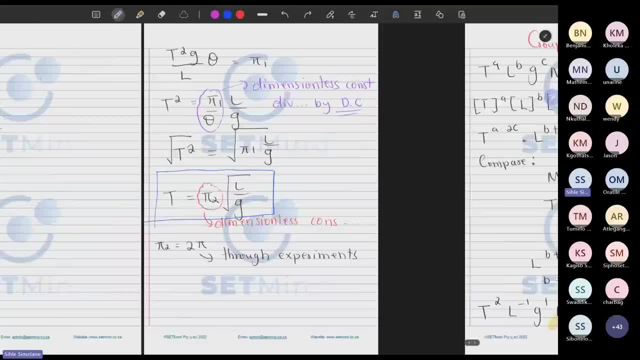 But you still have what Five, six weeks to be able to internalize geometric properties, flow properties and fluids. So you have plenty of time to wrap your head around and say, okay, let me see what is geometric here, Label them. 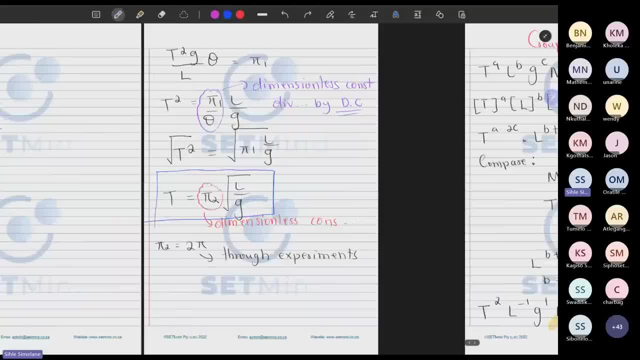 What is flow? Label them. Okay, these ones, I'm not sure I'm going to leave up hanging. And then you make a group, and then you make the variations. So believe me, you can master anything. I have faith in all of you. 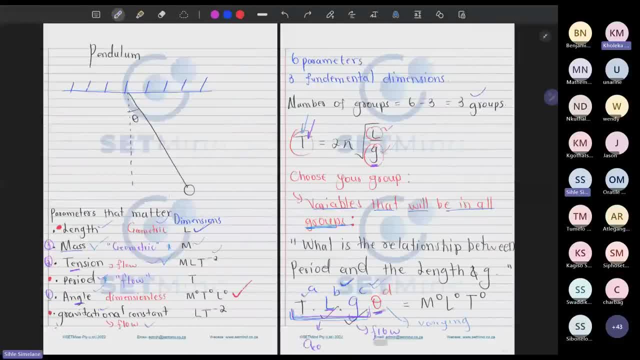 Please go ahead and I can believe. May you please explain again the groups part? Yes, You mean on the example. Yes, Okay, So the group part. I said to you we need to choose. So here's what. let me go to this page. 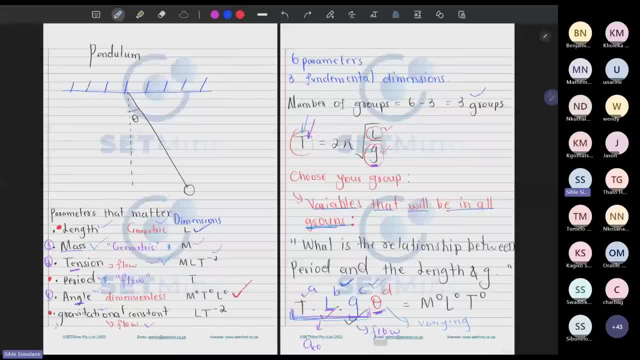 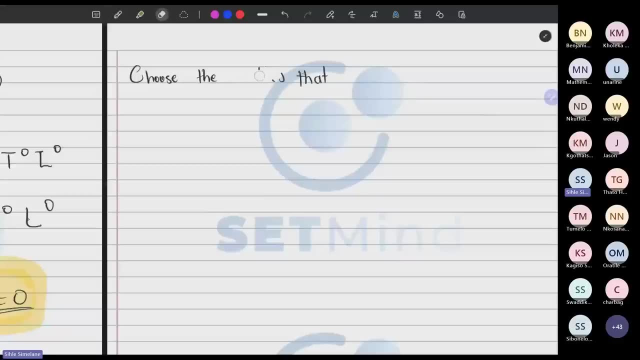 When we look at groups, you need to choose a group that will remain constant. You need to choose the variables that, or let me call them parameters. You need to choose the parameters that will appear in every group, Appear in every group. 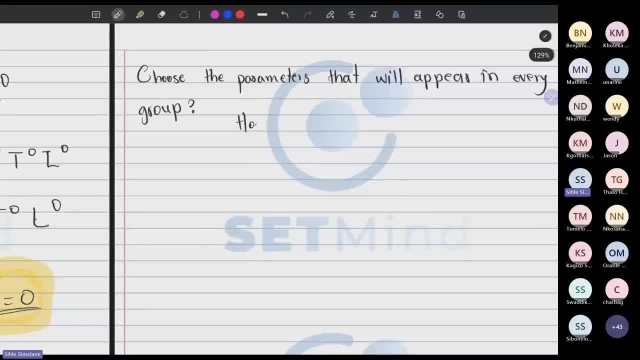 And the question which you should ascertain is how. And here's the how. So you need to choose A, You need to choose A geometric parameter, You need to choose a flow parameter And then you need to choose a fluid parameter. So they should always be three. 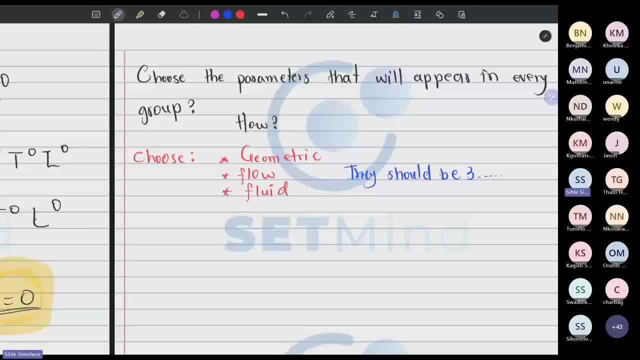 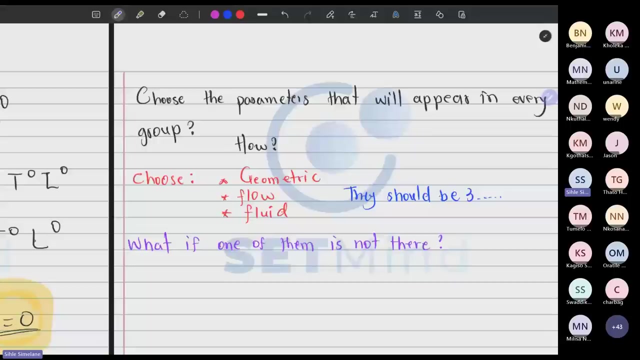 But then the question which you need to ascertain is: what if one of them- Sir, I can't hear you. Okay, Can you all still hear me? I think I was out for a minute. Can you hear me? Yes, sir, Yes. 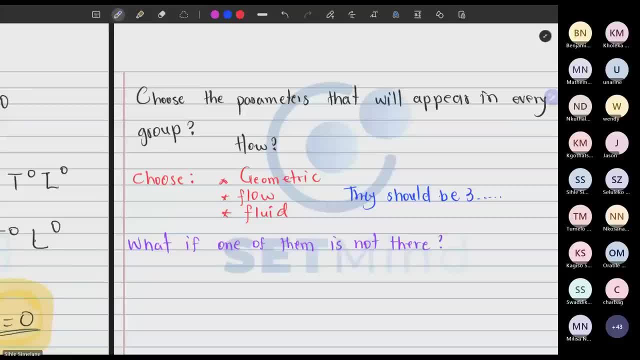 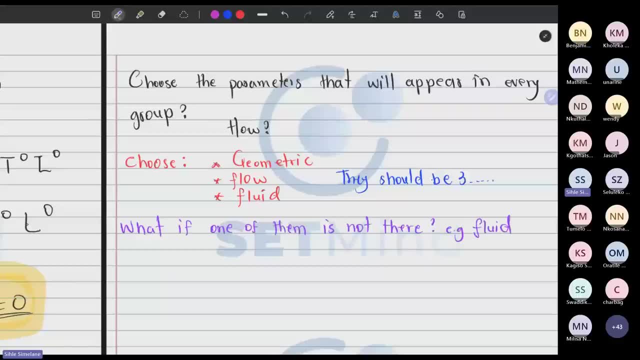 So I'm saying, what if one of them is not there- Example: you can't see any fluid property- Then what you do is you can repeat one of the parameters. Okay. You can repeat A geometric or flow flow parameter, Okay. 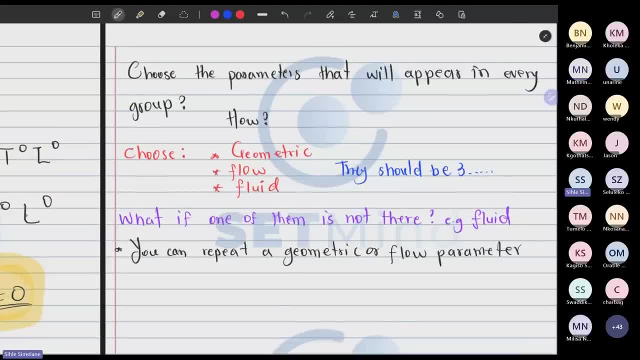 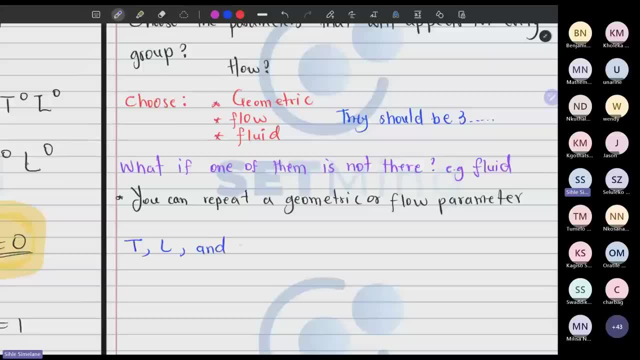 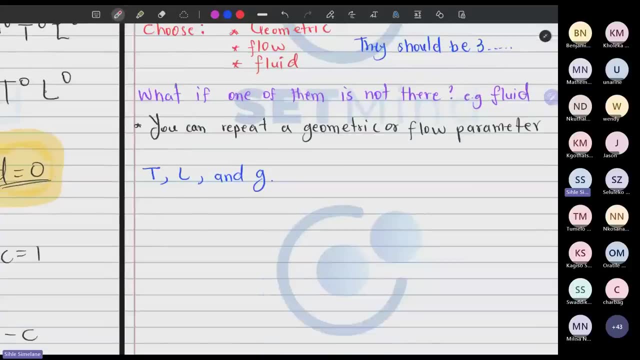 That's what you can do. You can repeat one of them. So, if you look at my problem, we were looking for the relationship between T, L and G. Okay, And in my long list of variables I had to look up which. 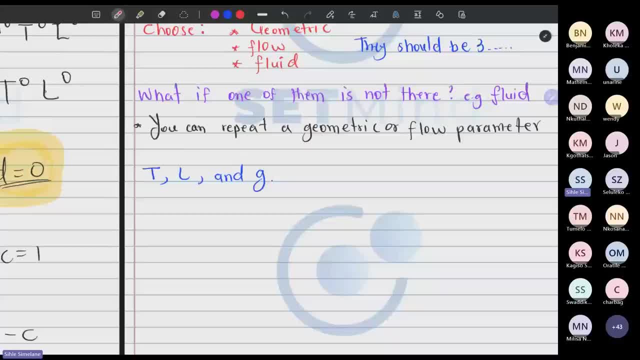 variables are geometric, which one are parameters are flow and which one are fluid. So when you look at my list, the previous list, I have no flow property, No fluid, sorry, No fluid. let's say parameter. There was no fluid parameter. 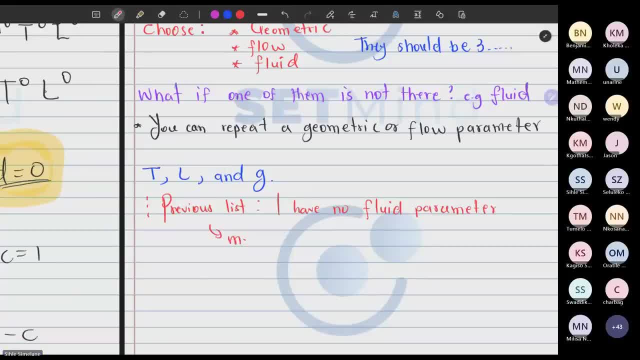 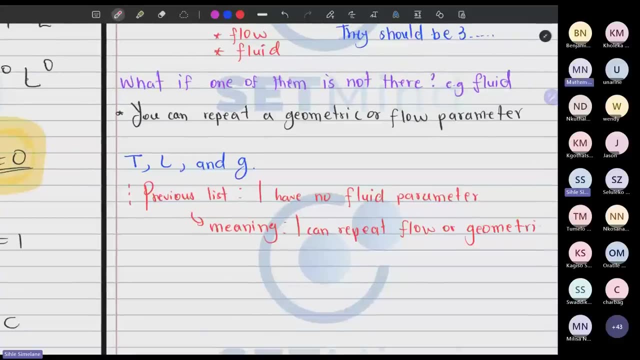 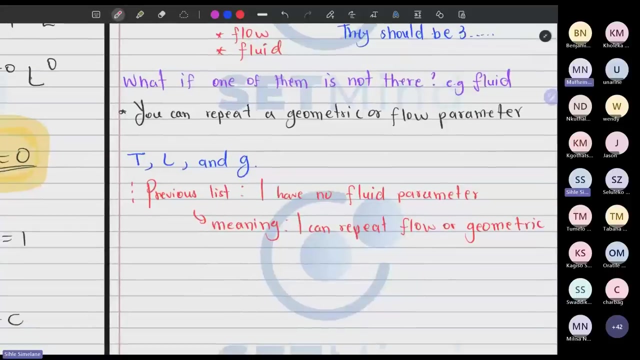 which means then I can repeat flow or geometric, because the other one was supposed to be fluid. They need to be three of them, So since the third one is not there, I can repeat the other one. So what I did in my previous problem- because I'm 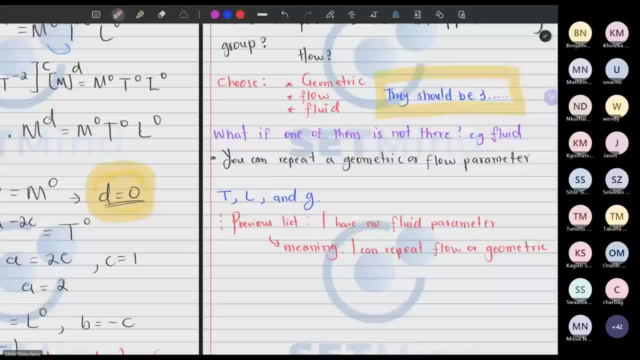 looking for this relationship. I then said: let's take length. Length is a geometric property, So I'm sorted already with geometric ones. And then gravity, which is acceleration. gravitational constant is a flow property. No, And then, since I couldn't find any fluid, 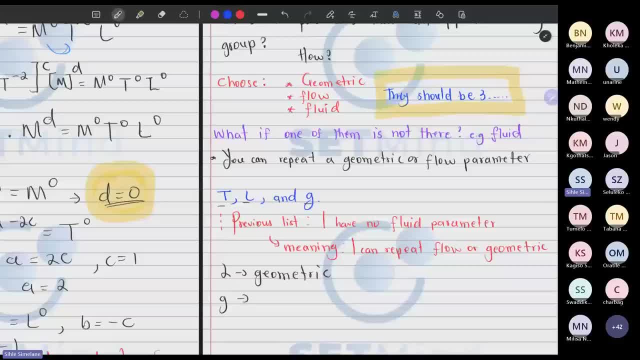 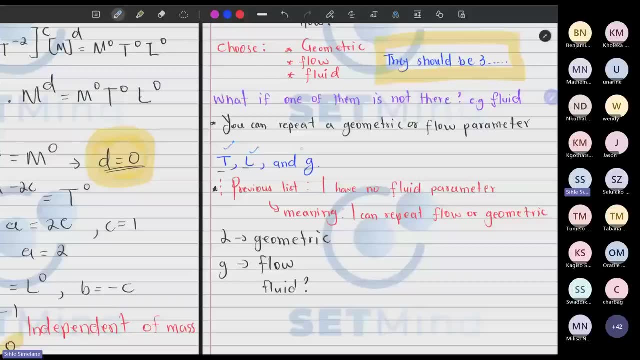 I opted for this, which means you can repeat either a geometric or a flow property. So, since I was looking for the relationship between time, length and g, it means t was the one which I could repeat, which is flow. So now we can. 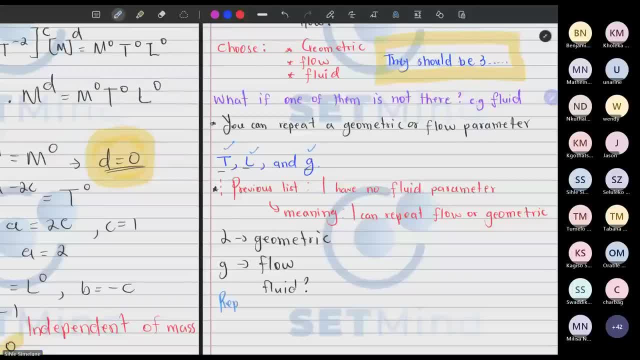 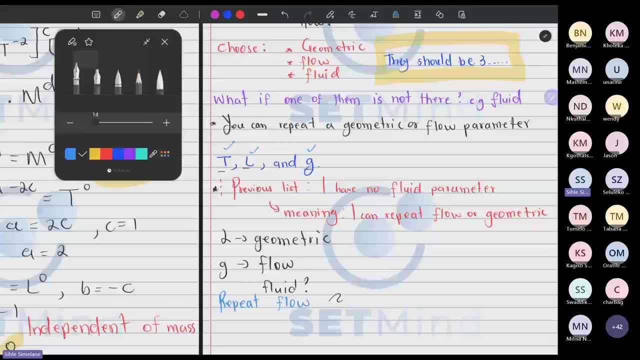 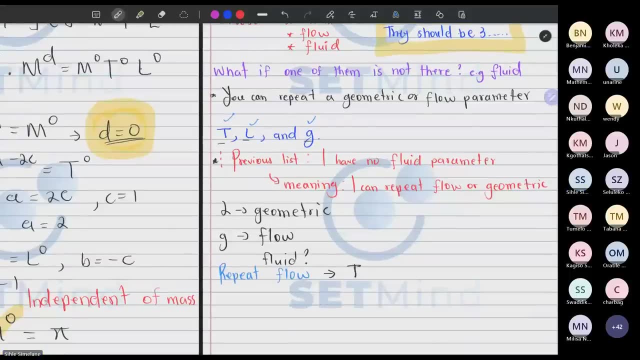 repeat flow which is t, which is t. So which means my constant group group will be the t to the a, the l to the b, the g to the c. That's my constant group. They should be three. And then now. 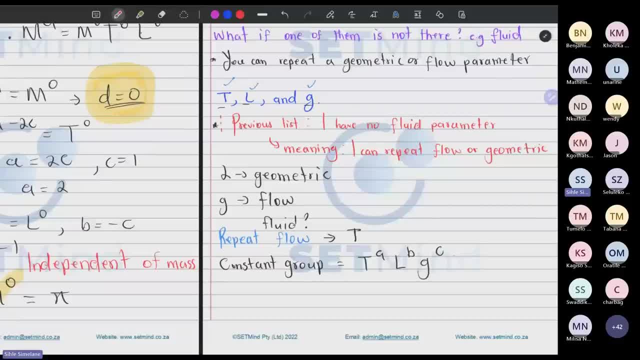 we need to put in the group which will change. So let me say, changing t, The p is for parameters- to the d, The change in parameters will be what is left. And what is left, if you remember, is the annel. 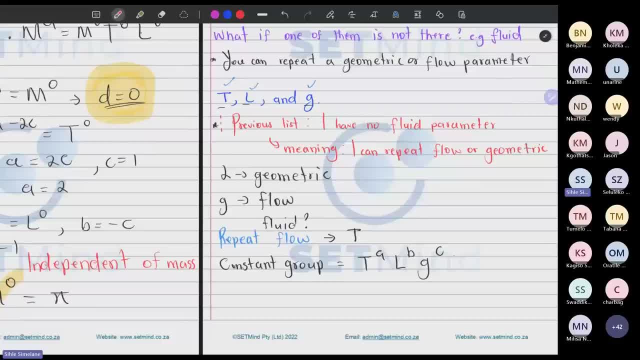 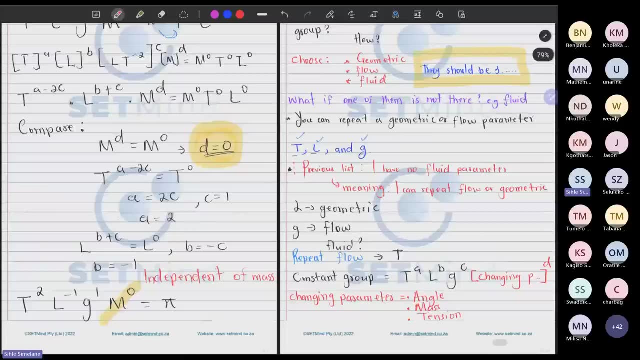 And what else is left is the mass. What else is left? it is the tension, Okay, Which means group one, my group one, is going to have the mass there. Group two is going to have the mass there and the change in parameters. 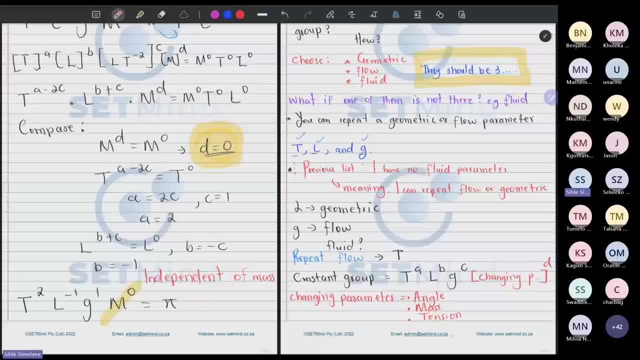 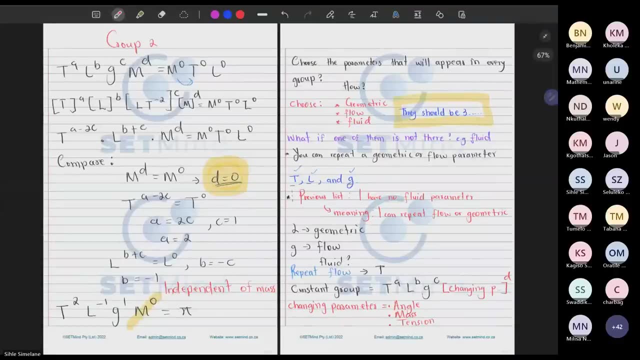 Group three is going to have the tension there, And then what we do is the same. We equate to m zero, t zero, l zero and try to find the a, b, c and d. Does this help The person who posed the question? 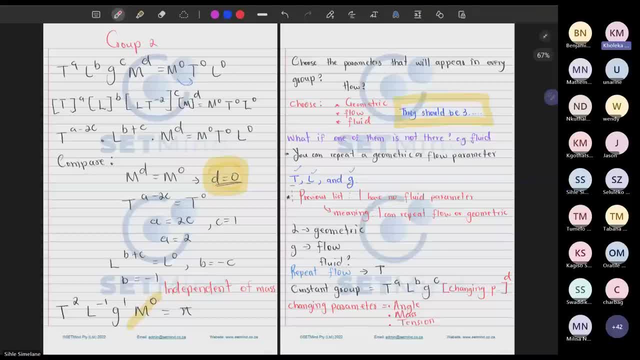 do you follow? Yes, I'm following, No problem. Someone else was asking a question. Please go ahead. Okay, And then maybe let's say we have any other general questions. So when you do these things in class tomorrow, they should make sense. 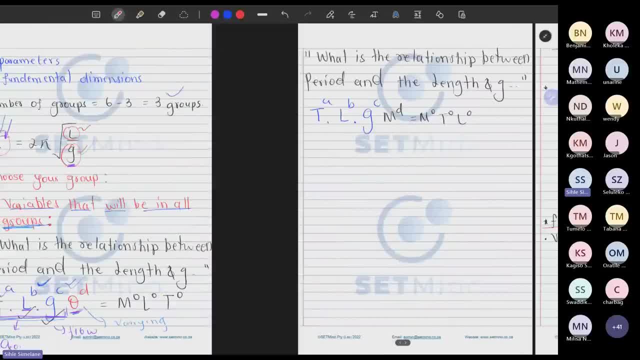 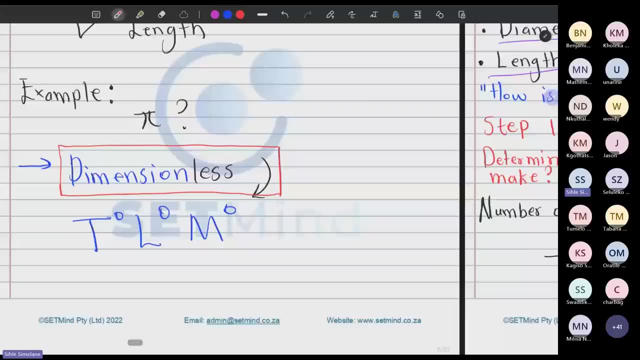 You should be able to see and say okay. so the first thing which Sir needs to do is to tell us about the dimensions. He needs to Then, after the dimensions, he needs to tell us what they mean when they say dimensions. Dimensions means t to the zero. 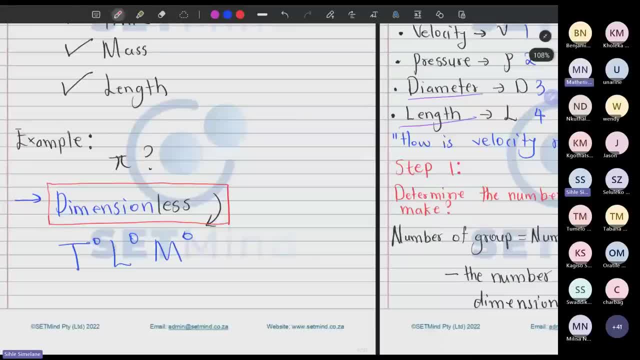 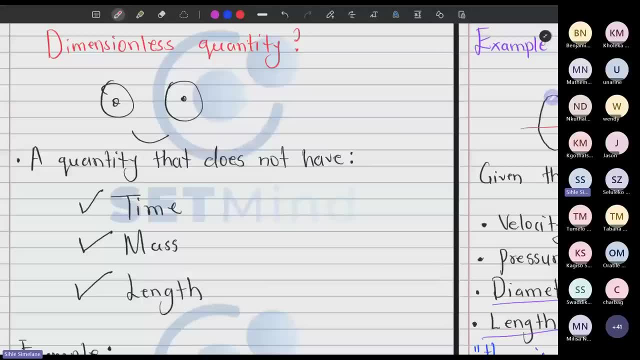 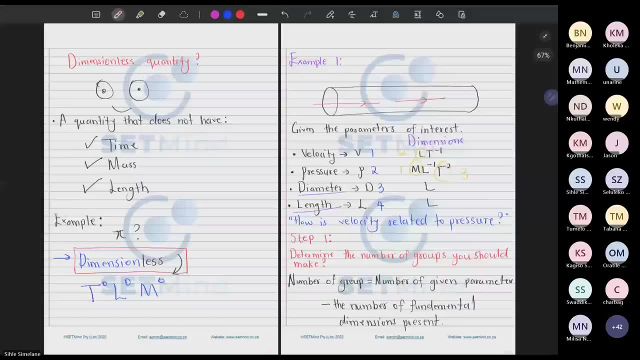 l to the zero and n to the zero. That's what they mean when they say dimensions. He needs to tell us about the fundamental quantities- not quantities, sorry- the fundamental dimensions, which are the t and the fundamental units. you know them. 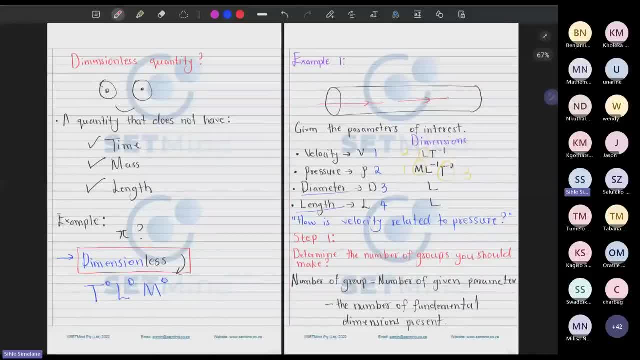 So I hope tomorrow doesn't become as hectic as it would be if you were going there with no tools, because the problem is class is 45 minutes and there's a lot of dynamics. You're moving from one class to another, so it's very hard to understand. 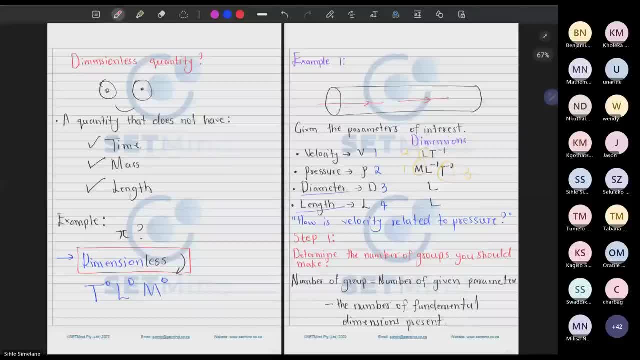 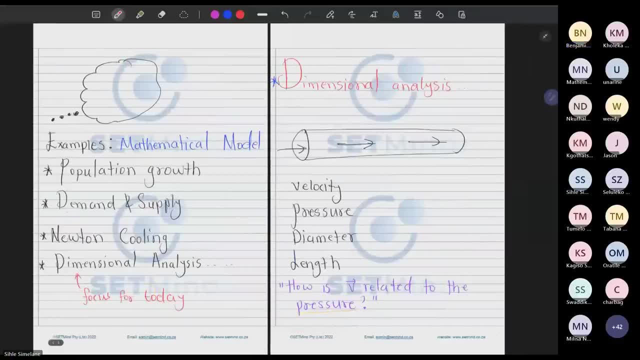 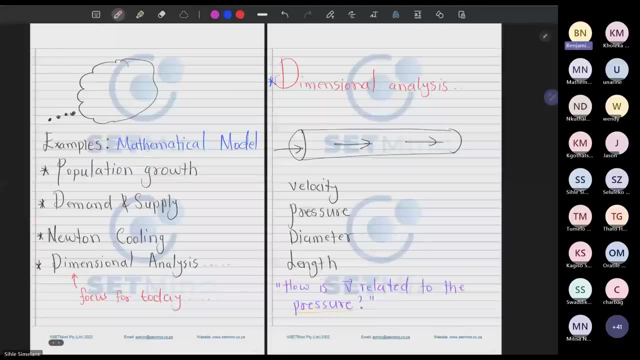 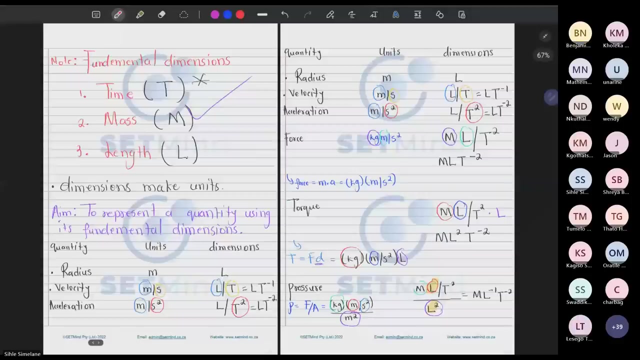 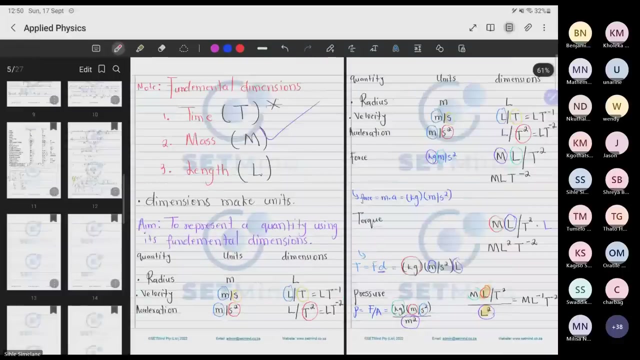 things which, believe me, are really important. So before we wrap up, I'd like to ask a few questions from anyone. Suppose we are having five parameters, and on those five parameters we do have geometric fluid and flow, And then now we have three of them. 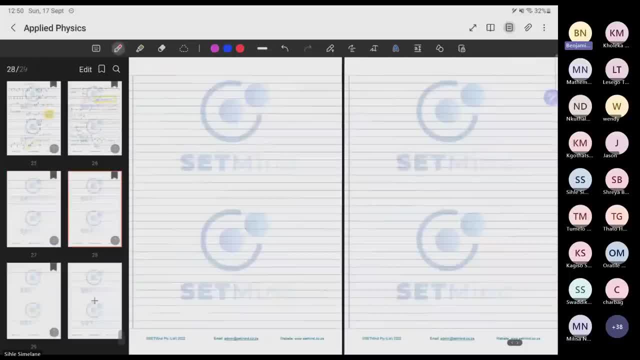 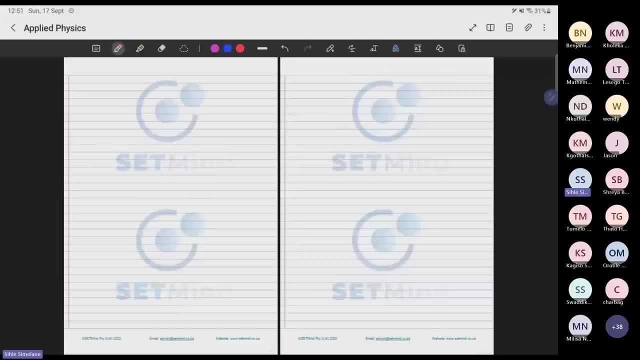 and that the remaining two parameters- geometric is repeating and fluid is repeating, right? So they ask us to find a relationship between two parameters and then only to find out that those two parameters- one is geometric and then the other, it is um. 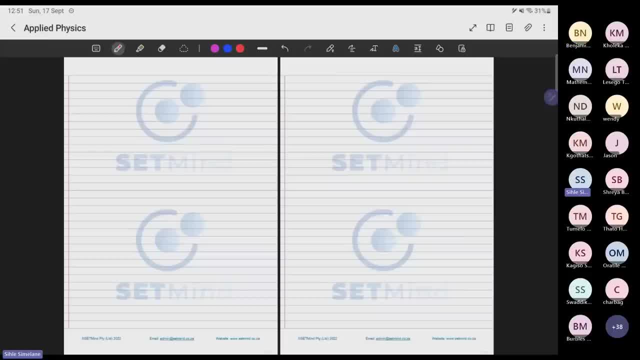 is this thing. it's fluid, So but then because we have sort of like two geometric and then the other is fluid, on the two geometric, which one I sort of like choose. So if you think carefully, let me write that down for those. 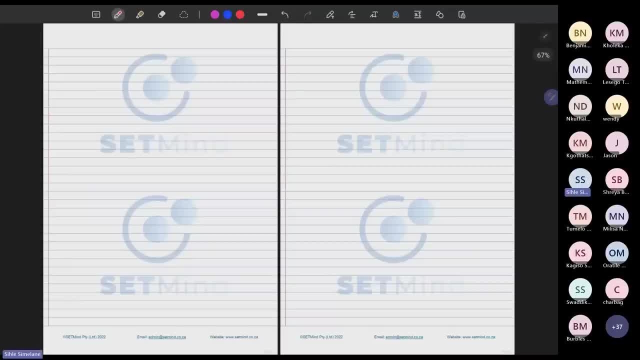 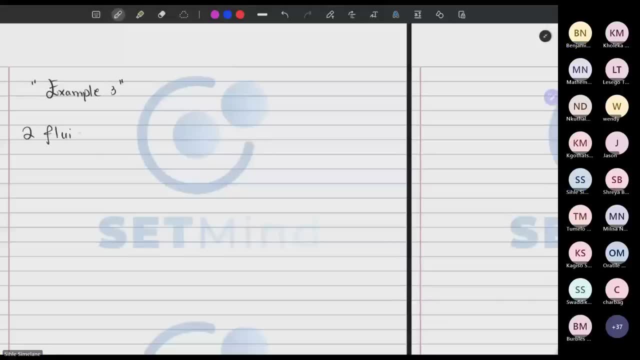 who might have missed it, So let me call it example three. So you are saying we have two fluid parameters, And then we have two geometric parameters, Mm-hmm- Three parameters. And then, for the sake of completing this thing, let's just say: 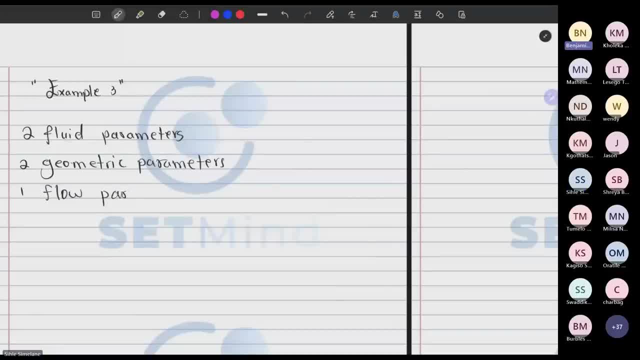 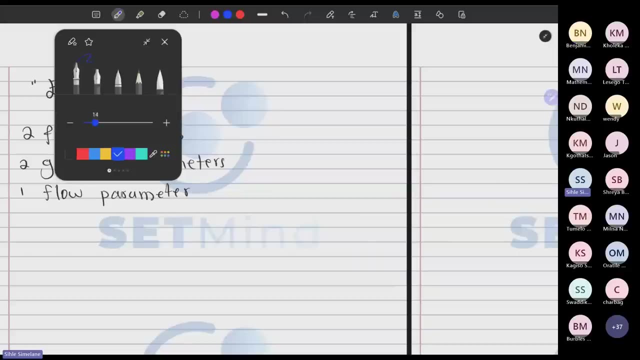 we have one flow parameter. So, if you remember, we said you need to make sure that when we, the first thing you can do obviously is to find the number of groups. So here, obviously, the group number on group will be. we have 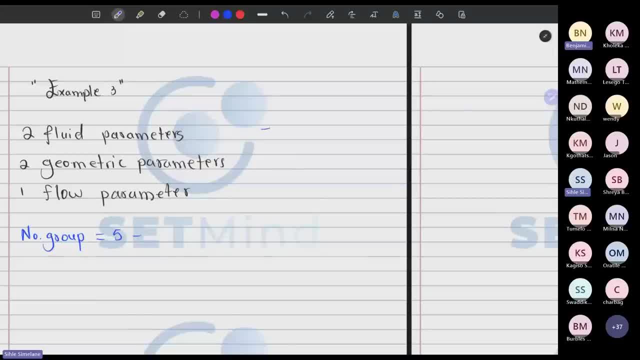 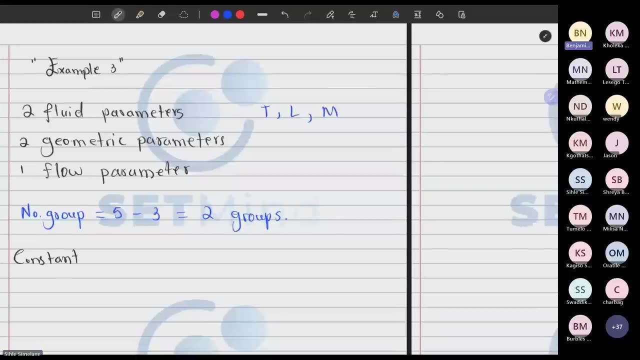 five minus here. assuming in these variables we'll have t, we'll have l and have m will minus three, which gives us two groups, So two groups. we need to determine the constant group, Mm-hmm. And remember the constant group must consist of: 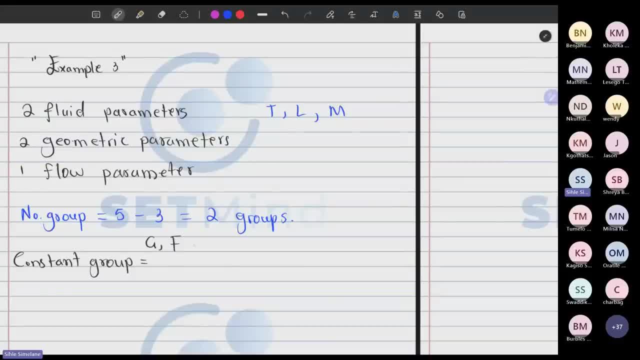 geometric parameters, a flow parameter, a flow parameter and a fluid one, Mm-hmm. So what I'm gonna do here is I'm gonna name these parameters hypothetically, So let's say the relationship. they are saying we should find the relationship. 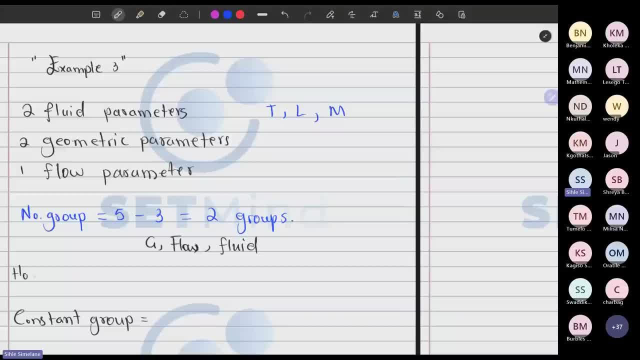 the question says we should find, or they say: how is the is, let's say, geometric? how is their geometric parameter? Because we have two of them: Geometric parameter, Mm-hmm, How is it related to, let me say, fluid parameter two? 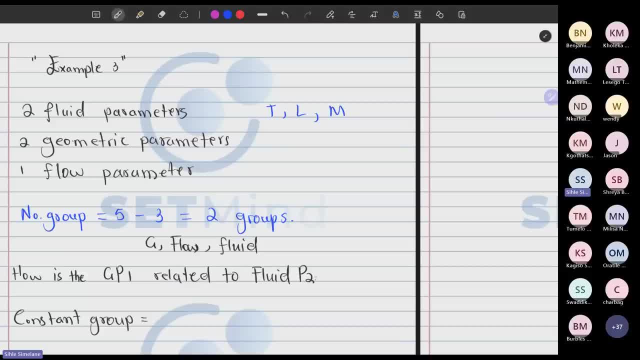 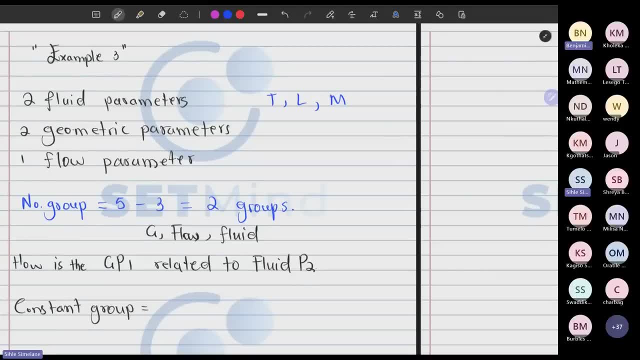 Whatever those would be given, it would give you that the fluid parameter is viscosity, the other one is this: But let's say the equation says this. So what I would do is: I know I need a geometric flow parameter, So flow parameter is: 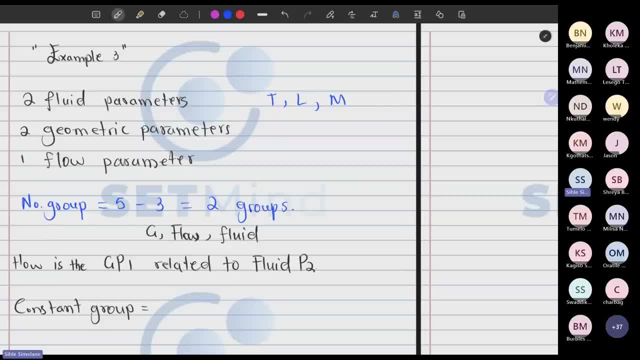 one, obviously. So there's one of them, I'm forced to put it here. So, flow parameter, that's gonna be there, and then I'm gonna put the a, Whatever it is, if it's velocity, if it's acceleration, you put it there. 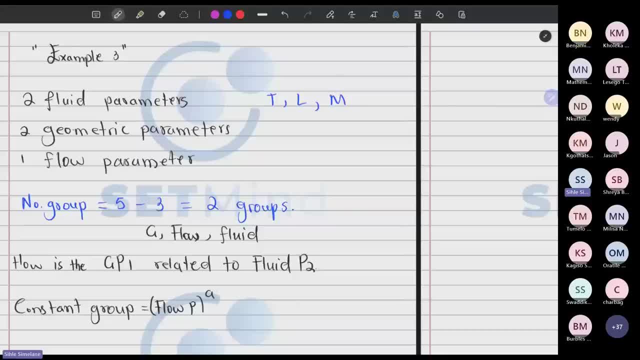 Mm-hmm, And then the geometric parameter. I can choose any of them. Let's take geometric parameter one Which is geometric parameter one to the b, And then I can also choose the fluid parameter. Either I choose the first one or the second one. 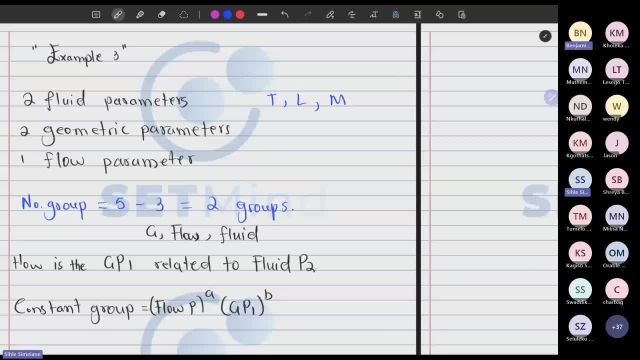 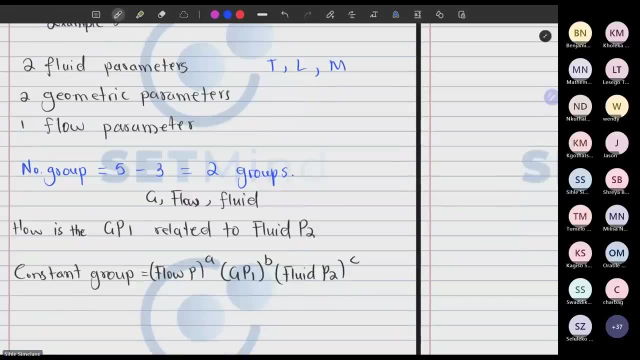 It doesn't matter. So let me choose the fluid one, Let me choose the one they want, which is fluid parameter two, And then I put the c. This would be the group which would remain constant. Okay, And then group one. So 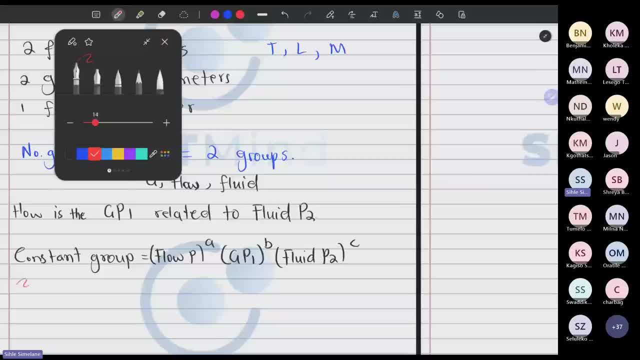 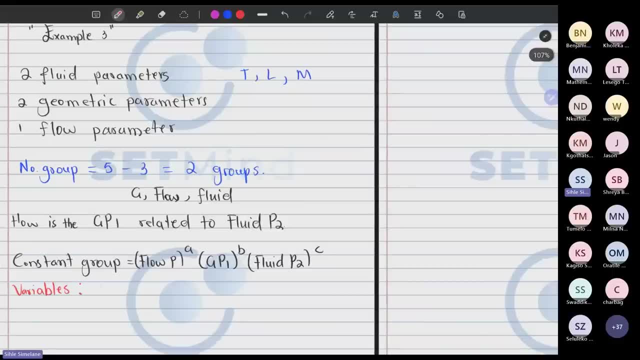 now, what I did not vary is the variable. the variables are, Be careful. So since I have, it means I have the flow. the flow parameter is taken, geometric parameter one is taken. So what is flexible is geometric parameter two and the flow parameter one. 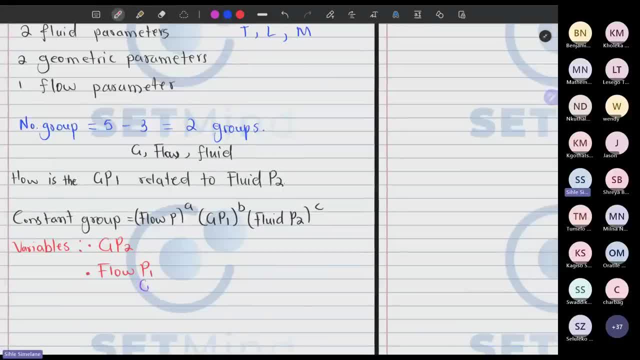 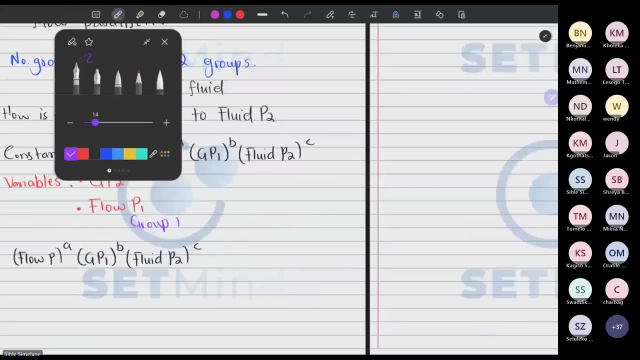 So it means group one. I would do something like group one. I would go and copy this here And then paste it here, And then I could choose to put in that geometric parameter two to the d And then equate it to m: zero, t, zero. 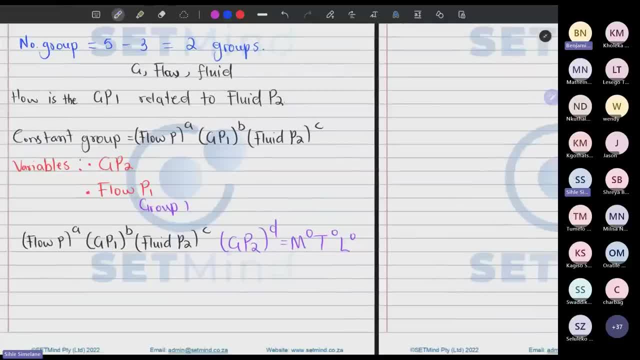 l zero. And then group two: we copy exactly the same thing, We just change: we put in the other variable, which is variable which was not there, We paste here. And then I come and say: the variable now I need is flow p one. 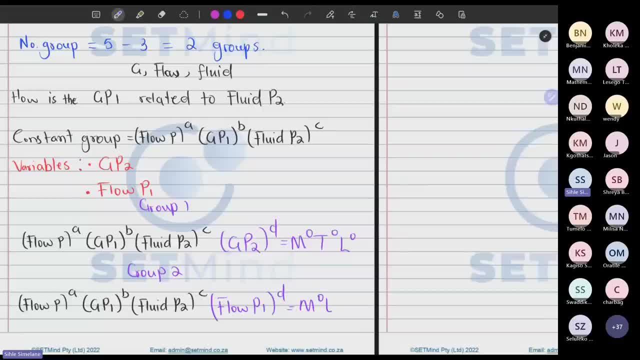 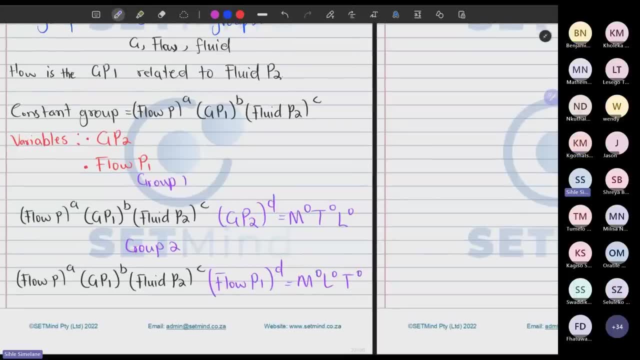 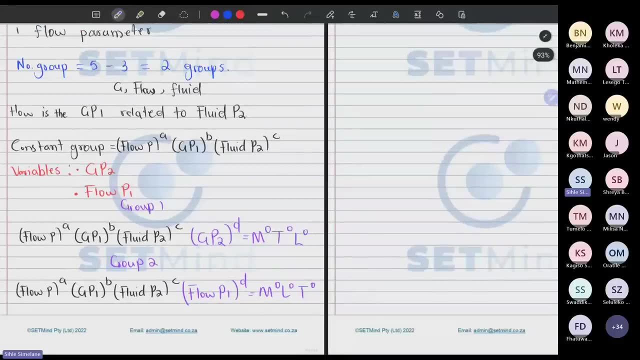 And then to the d, And then this should be m, zero And zero, And now I can relate and do the d and the t And then I can put in the relationship however way they want. Are they looking for the flow? How it related to fluid property? 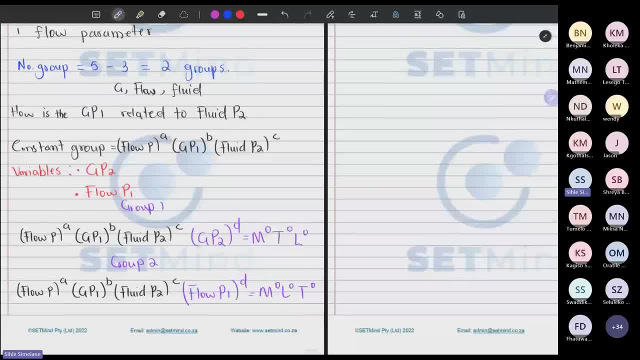 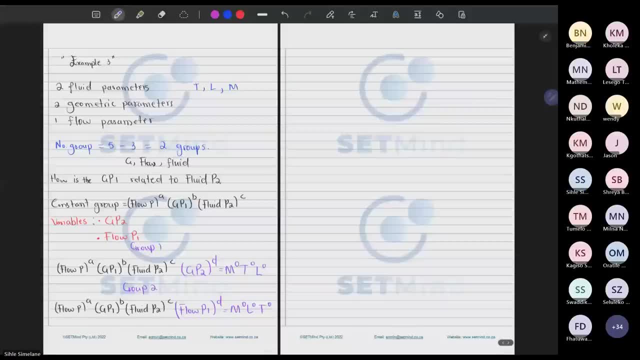 two, or fluid one, Or how it related to geometric property. one or two. Does it make sense? So, On the variables there, it's supposed to be fluid one, Fluid parameter one, Because we have one flow parameter. Okay, Let me flow one. 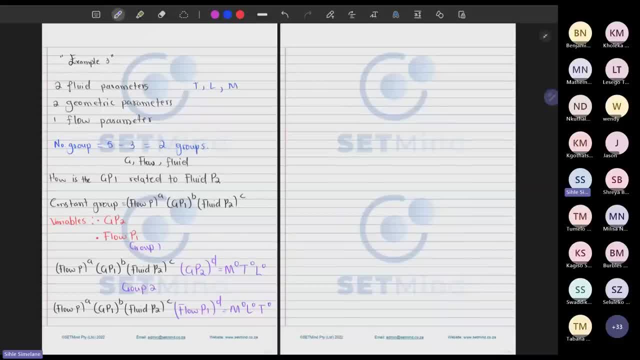 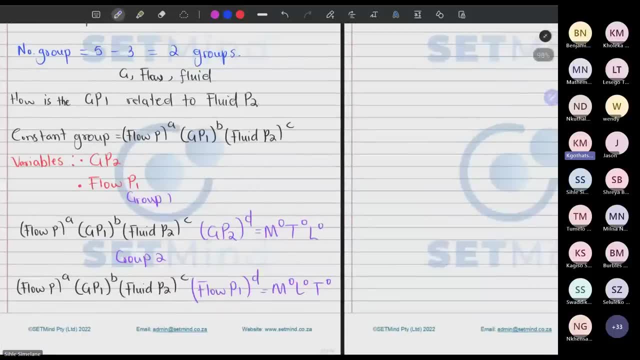 Please point it out for me. Which one are you referring to On the variables there? you said geometric parameter two and flow parameter one. It's supposed to be fluid parameter one, since we have one flow parameter. Oh, So that's supposed to be g. 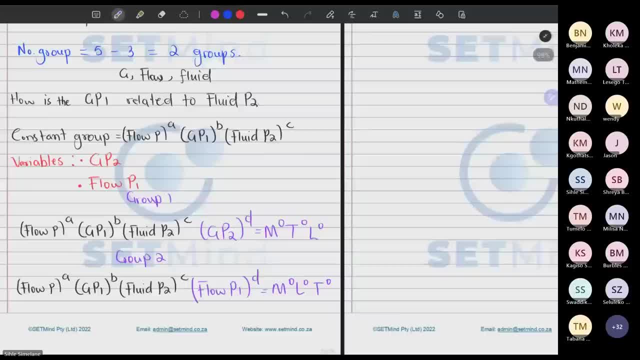 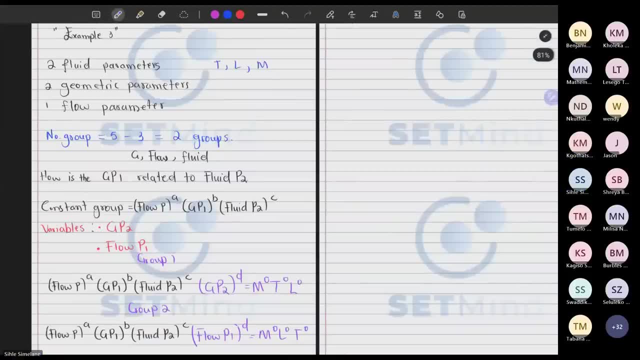 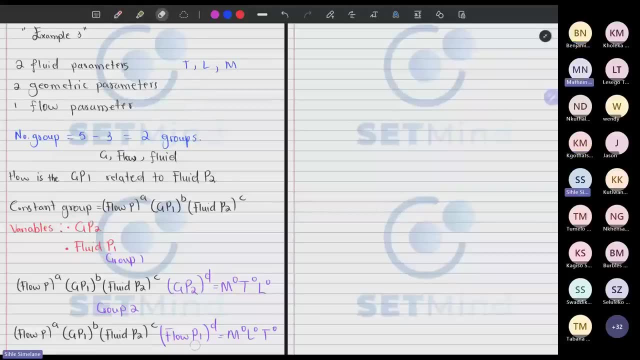 fluid two. Is that what we are saying? Flow parameter is one, So this is supposed to be fluid Fluid parameter two. Oh, one, Not two. one, Yes, Fluid that, So that was fluid. Silly mistake. But if the person 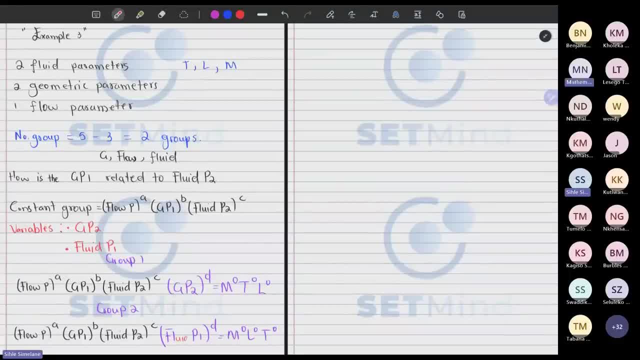 who's marking is not happy. you would easily lose many marks. So thank you for raising it up, Because we only have one geometric parameter, So pg, But we have one flow parameter, Yes. Yes, So, sir, Does that mean that? 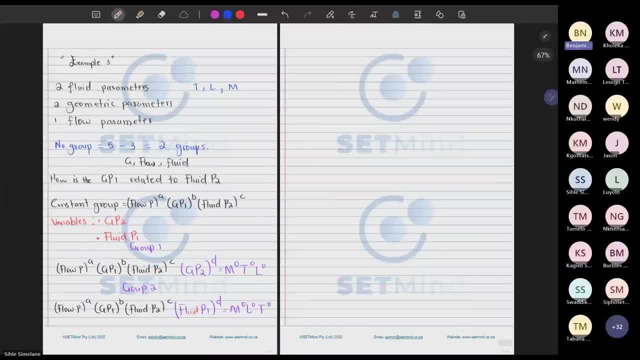 even though they wanted us to find a relationship between a geometric and a fluid. we must include the flow as a constant to satisfy you. know those theorems? Yes, So you can't just exclude a parameter which was given because you are hoping to relate this one. 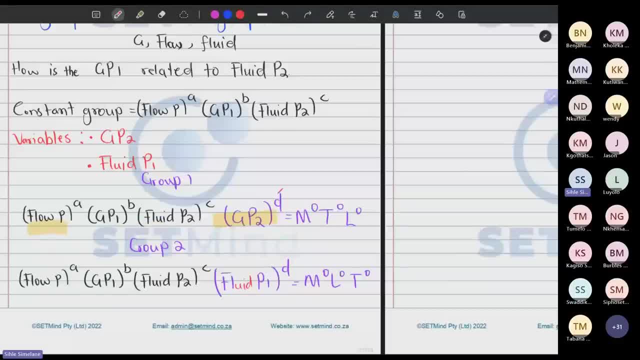 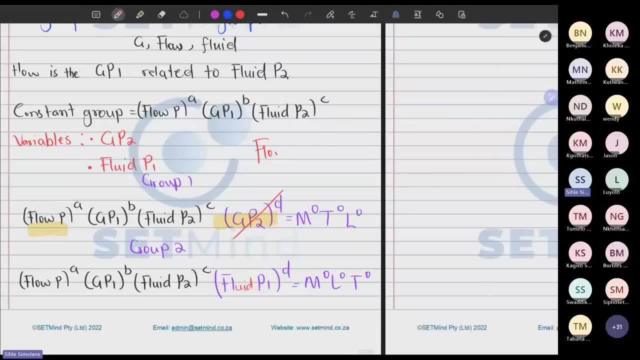 in this one. This one will come redundant. When you now relate them, maybe you will say: flow p is maybe directly proportional to one over the fluid parameter p2.. Because that's where your focus would be: Just comment and say, look. 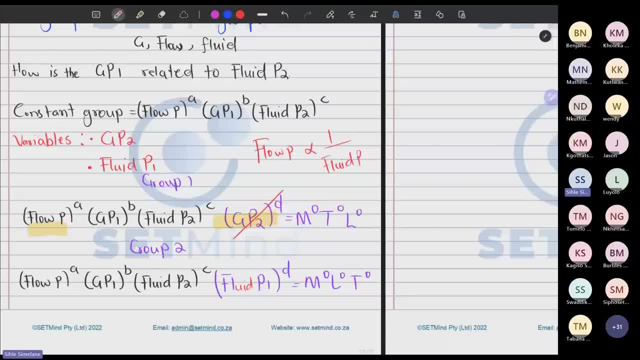 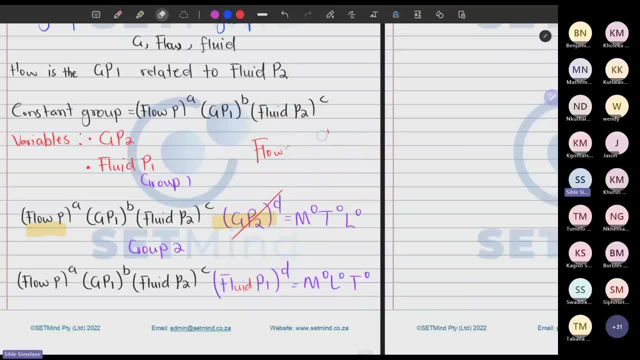 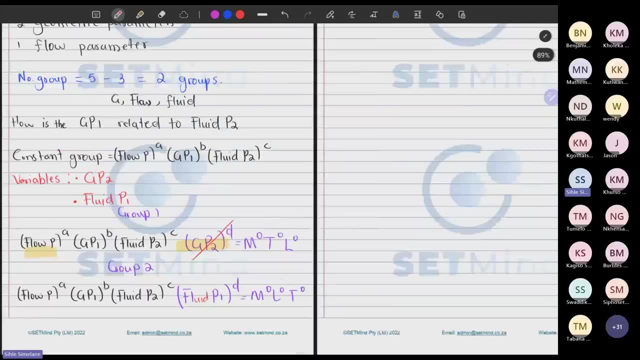 the flow parameter is inversely proportional to maybe the square of the fluid parameter, That specific one. But you do not exclude it. You do not only, in the problem, put in what you want. All variables should be accounted for. And then, when you now conclude, 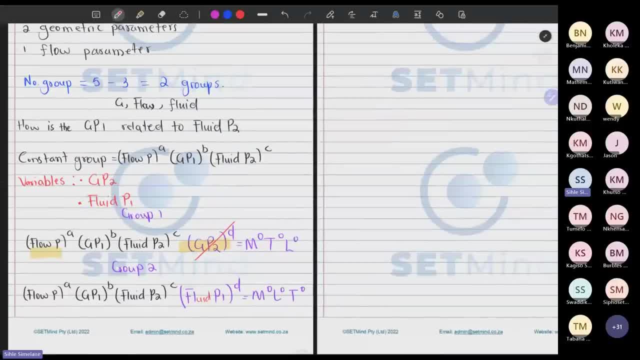 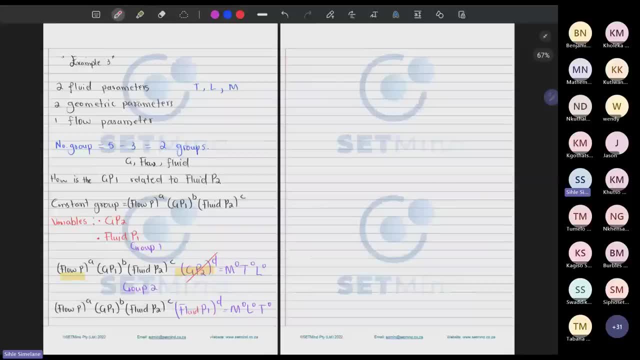 you focus on the variables of interest, But when you do the groups, no variable should be left. You have to find, because you do not see in the question, how it's going to relate to then the other ones. Okay, Any more questions? 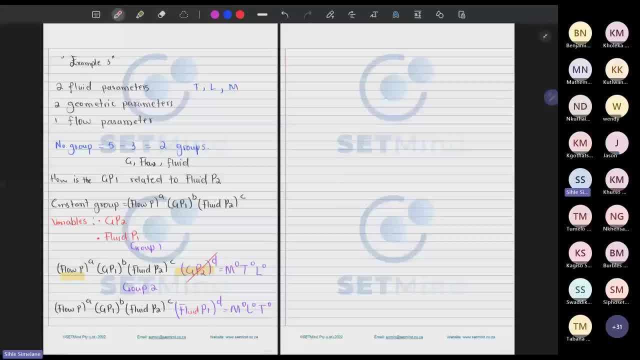 I am happy when questions come in because there's someone. I've got a question with the responses that we So after we've determined the relationship. when going back to the example that you made with the, with pi one is equal to two pi And. 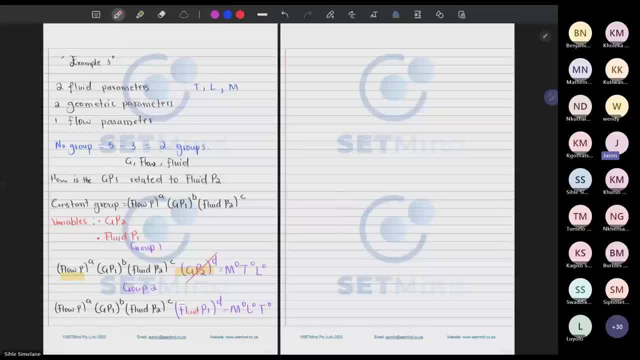 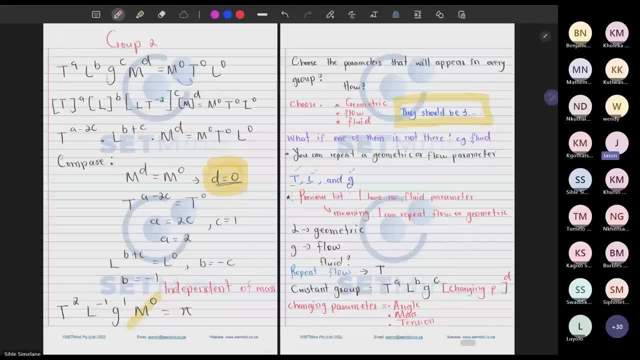 then you commented saying that that two pi was experimentally obtained. So how do we end up commenting, or knowing how to comment based on the relationships? like that, For the proportionality constant, you do not need to know. Okay, So when you deal with the problem, there's always going to be. 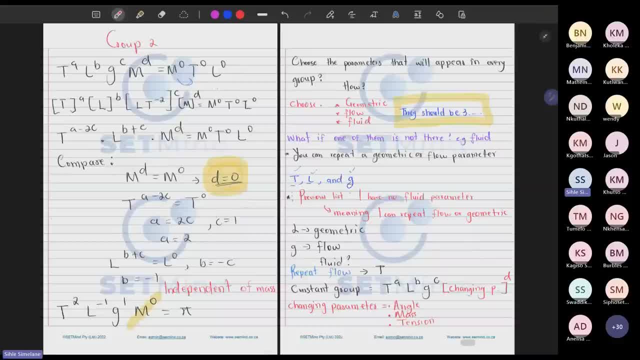 the pi, which is on the right hand side from here, will always be there. You don't need to know its value, You can just say it's just the proportionality constant. You are done So for this one. we just happen to know that it's going to be. 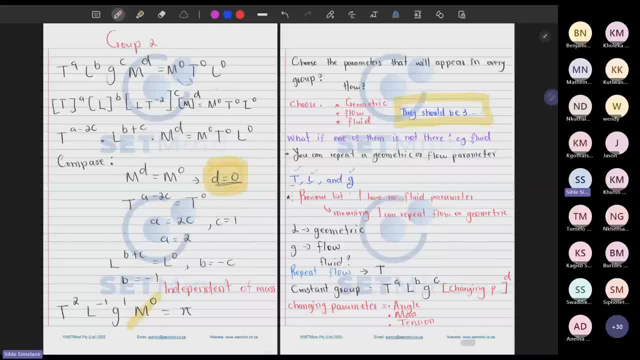 two pi because it has been experimentally proven. But for other questions the proportionality constant will remain as it is. You just leave it as pi one or you can just choose to assign a k, But it should be clear that it's a. 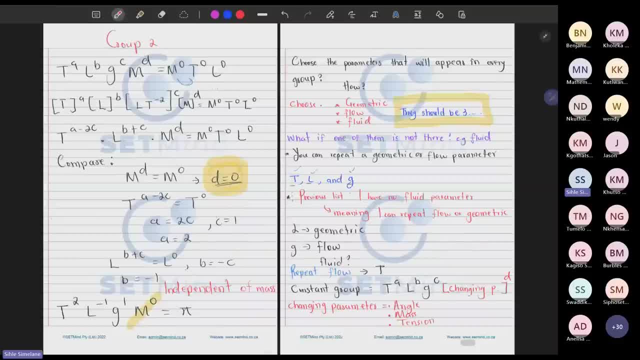 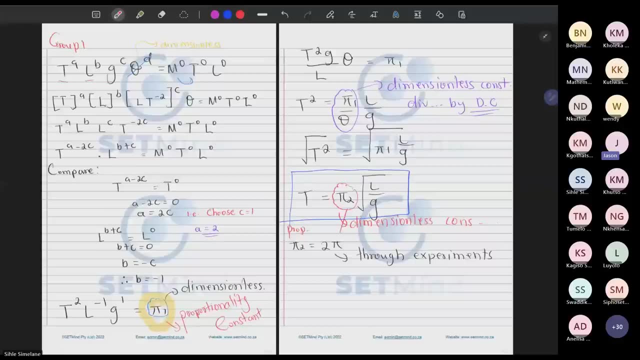 proportionality constant. Dimensionless slash prop. proportionality constant. Does this answer your question? So after we solve this, like how you solve it now with t, two is equal to pi l over g And then that final answer we get, we can. 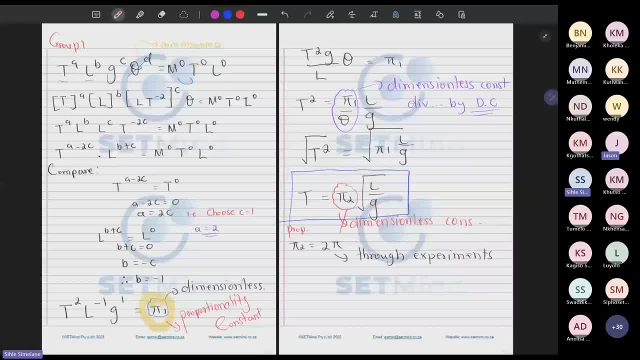 just leave our answer there and don't mark it. So this would be my final answer. So here we just happen to be lucky that we know what this constant is, But in other questions you won't know what the proportionality constant is. 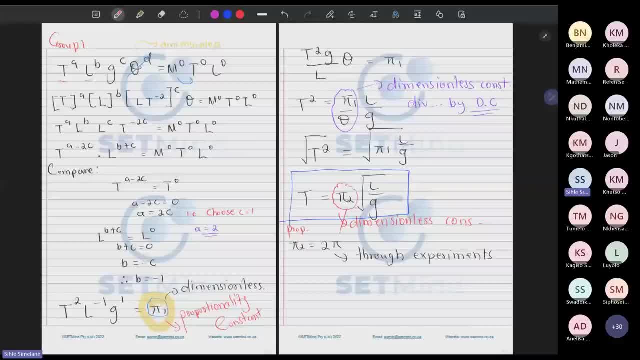 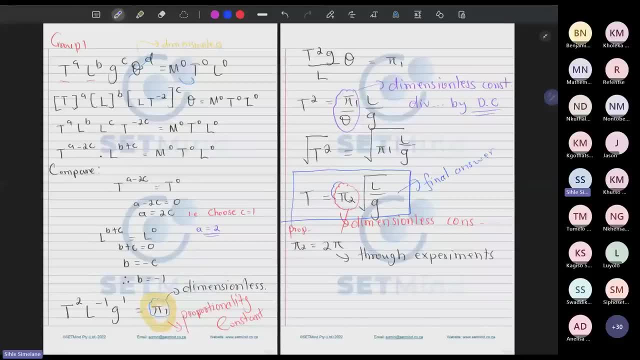 So your answer. leave it as it is. There is no need to comment. You can comment on the relationship. They ask you: how is t related to g? You can see here that it is. t is inversely proportional to the square root of g. 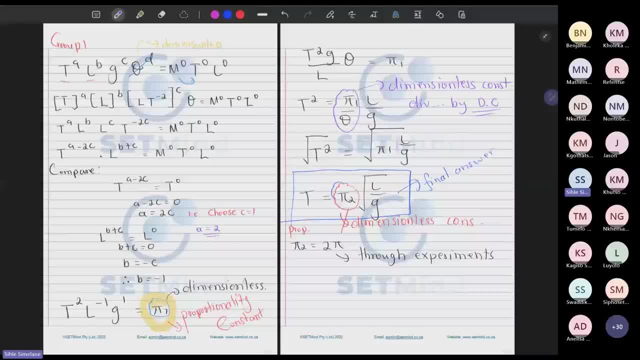 That's what you would say, That's your comment And that's done, Okay, Okay, More questions. There's more questions. Please go ahead. If you see your mate typing on the chat section, please ask on their behalf. It is not useful to. 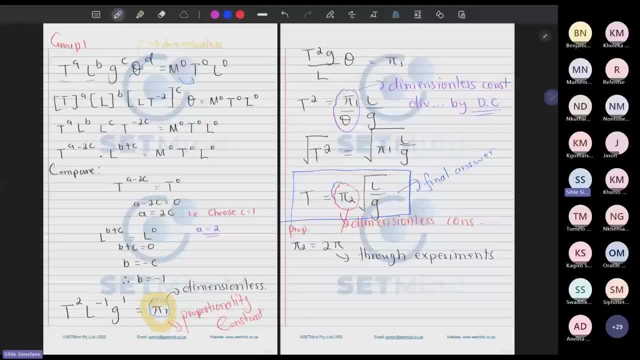 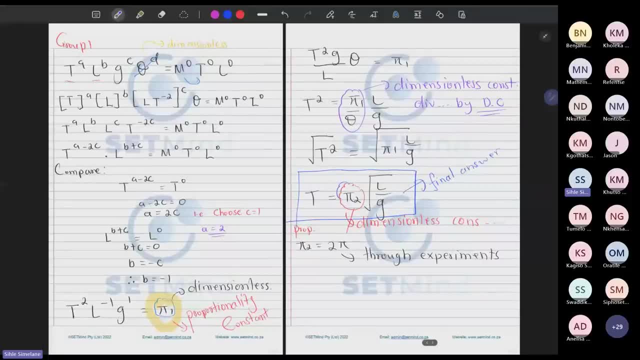 figure out what I was saying after the session When I'm here, when I can answer that question in two minutes instead of you spending 30 minutes trying to understand why did he do this? it is a waste of time. Make time to be useful. Answer me. 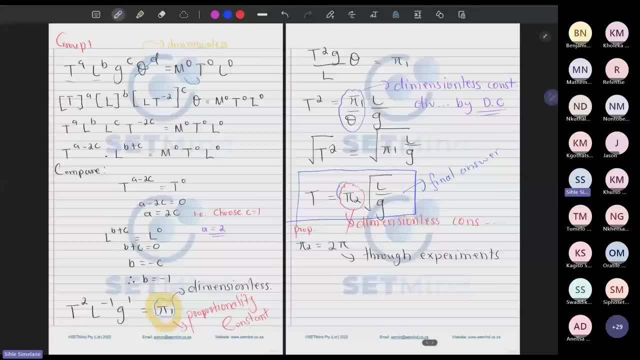 Believe me, it will take shorter than you going to figure it out yourself what I was saying, Or asking your friend what they think I was saying. when you can ask me what I'm saying, Please go ahead. Okay, We are counting down. 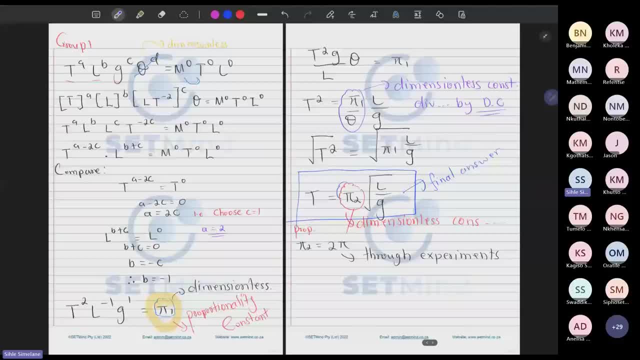 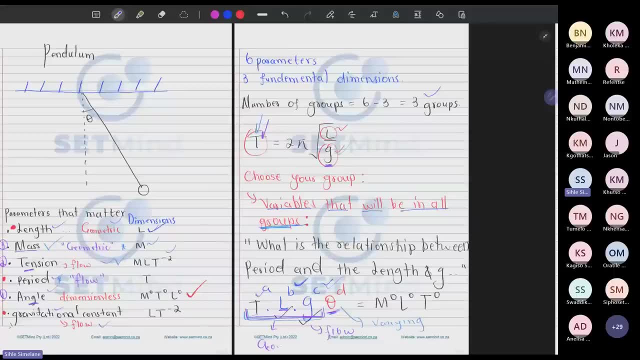 Please go ahead if you have a question and ask. It can be about dimensional analysis in general, But the aim of the session was to at least show you that it's not really as scary as it appears, Because over the years it has been scary. 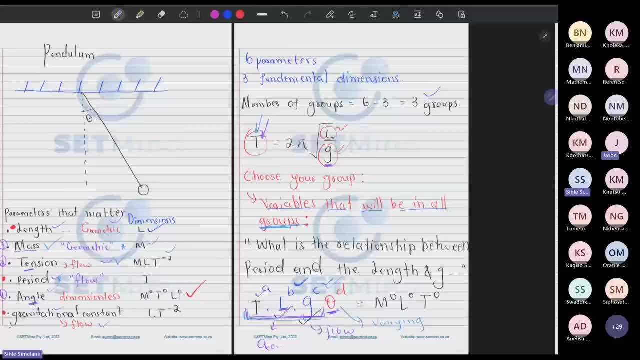 to students. So if you have a question relating to this, But I think it's a bit After we've learnt this information or this first part of dimensional analysis, then how would you advise that we- Because I think also on the groups- 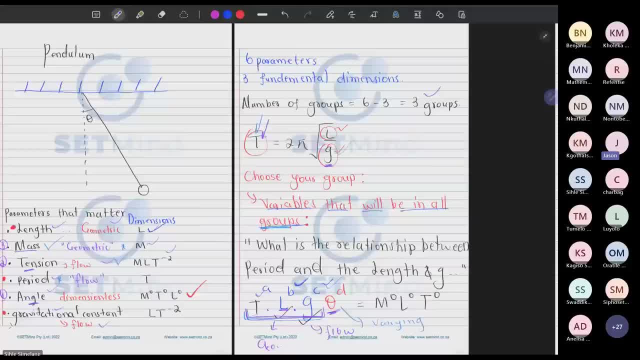 you did say that you also give advice of how we should also prepare or go over these concepts within the remaining five weeks that we have left before we write our exams. So here's my advice to all. If there's one thing which you should do, 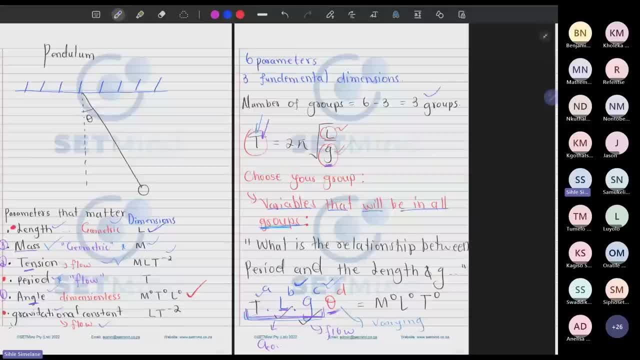 but this is always what I say to people in general. So this is not hard, It's reasonably doable. The only problem which means it's not easy for people to pass is the combination number of variables. So number one dimensional analysis is not complex. 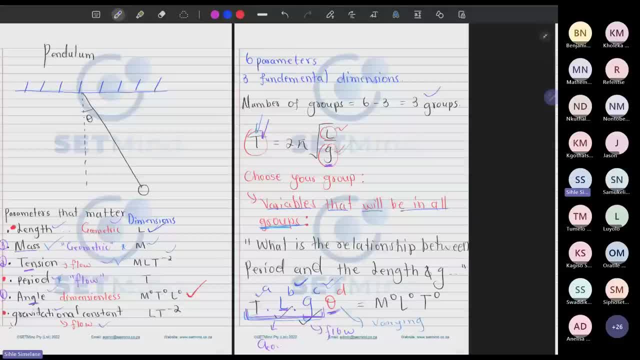 But it is going to be complex Because it's complexity number one is not hard, but complexity combined with the work overload which you are faced with And plus the short time which you have, is what will make understanding some of these concepts to be hard. 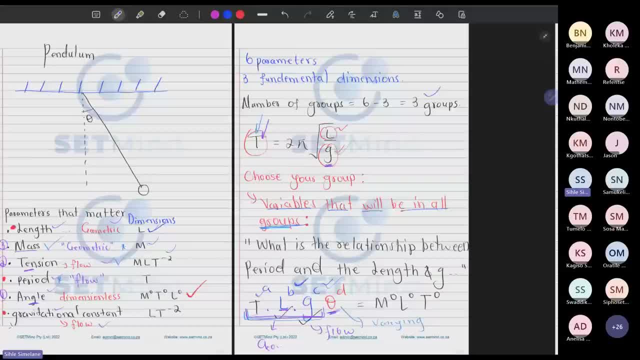 So my suggestion to all is: when you are in class, because you can't buy time, make sure you make use of that time, Because that hour which has lapsed, unfortunately, time is one thing which we can't buy. You can't buy it back And 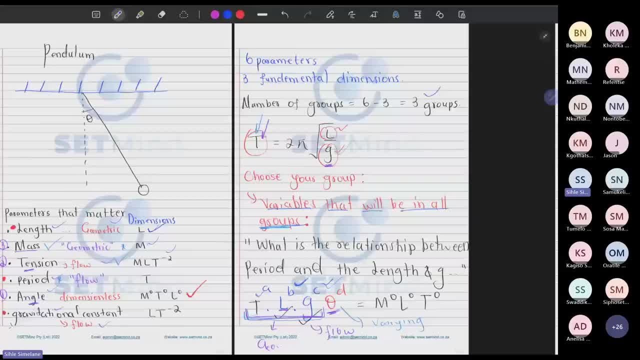 also the benefit of working in advance, as we are now, is that when the lecturer is introducing the concept, instead of wrapping your head around and trying to figure out the introduction and what they are saying, you are understanding more. So that's the benefit of. 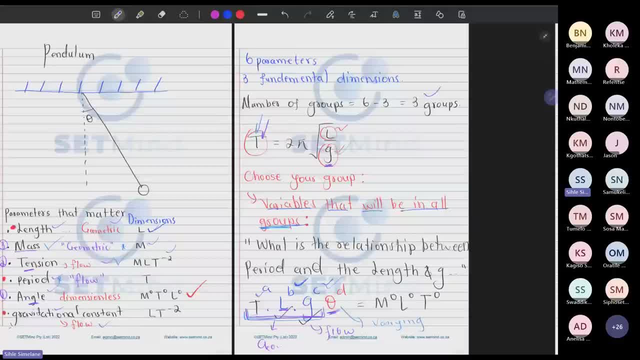 working in advance. So work by your own in advance so that when you go in class, instead of trying to understand in real time because the pace at which they go with is not the same, Some of them they go faster and by the time you make a note, 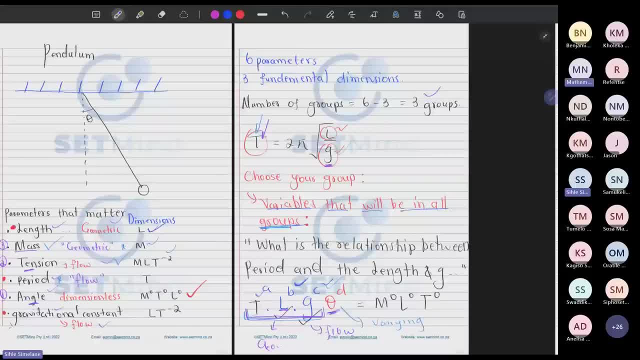 it slides away, It's a problem, But what you can afford yourself is learning in advance. Then, when you go to the lecture room, you are understanding, instead of trying to capture things and process them in real time. So imagine this week, the starting week you are going to be. 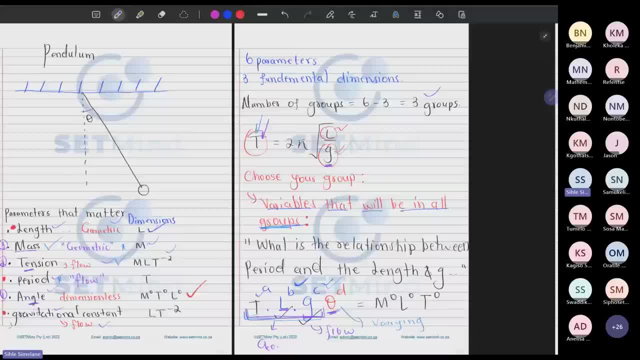 doing an introduction to modeling, but more focused in dimensional analysis. If you know what you know now, what you need to make sure is that next week, by the time you advance the concepts and you go to things like difference equations and other concepts, you build up to population. 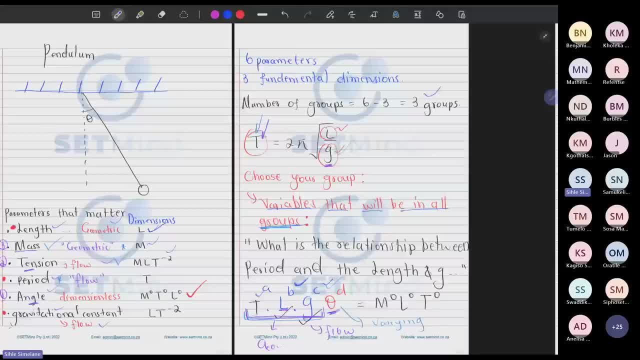 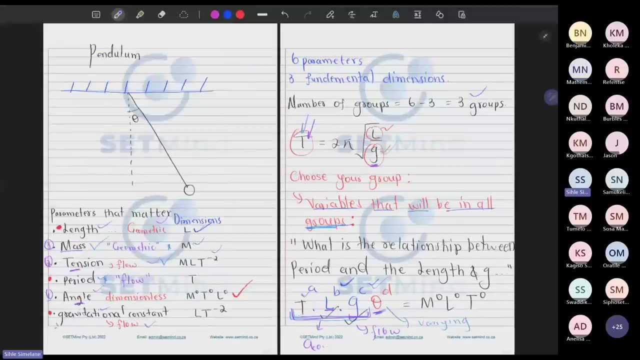 growth. by the time you get there, you must make sure that you have already done the work in advance, because at least now you have two steps advantage to dimensional analysis. But if you drag your feet by the time you finish dimensional analysis and you go to the other, 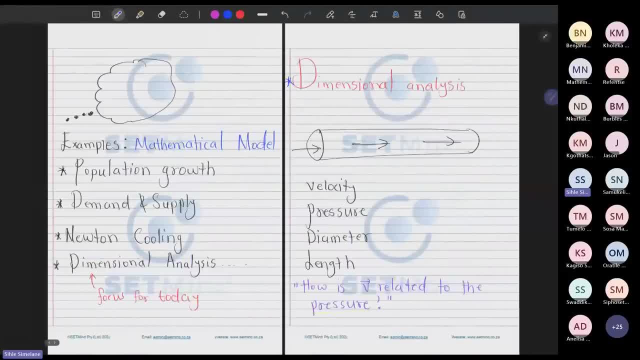 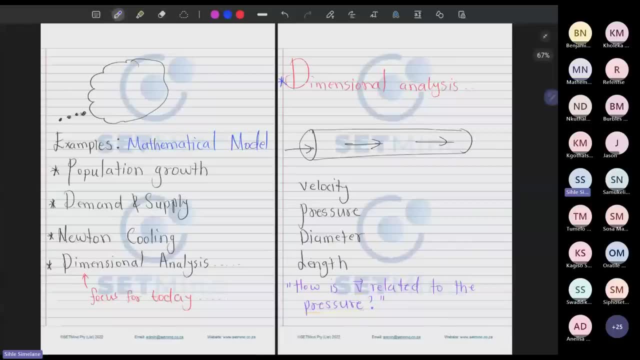 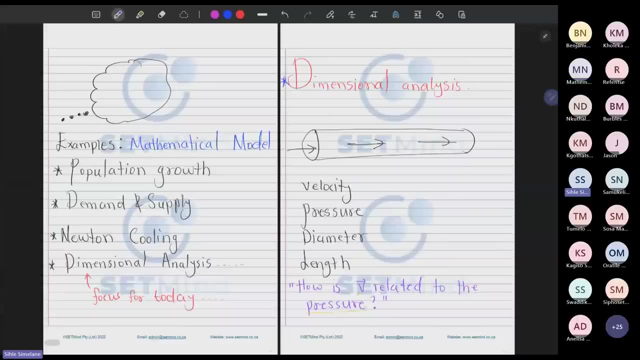 parts which are on my page one. you will be equally struggling as everyone, So make sure you try to listen in class and then also review the work which we did. go over the PDF, Try to make sense of what we were doing and then try to conceptualize. 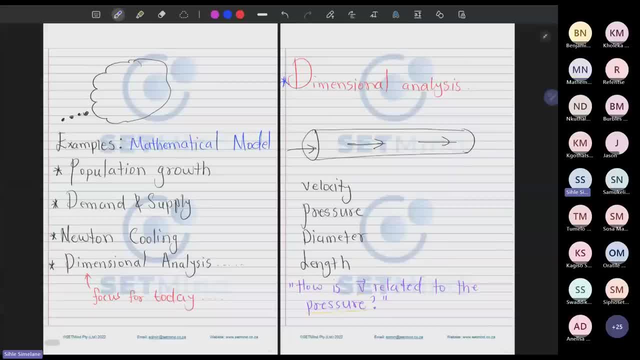 it. Watch the video again and then make sure that you try to attend the questions as the lecturer presents them. It will save you a lot of time. That's how you can buy time within advance, because combined with the pressure and the less time you are given. that's why 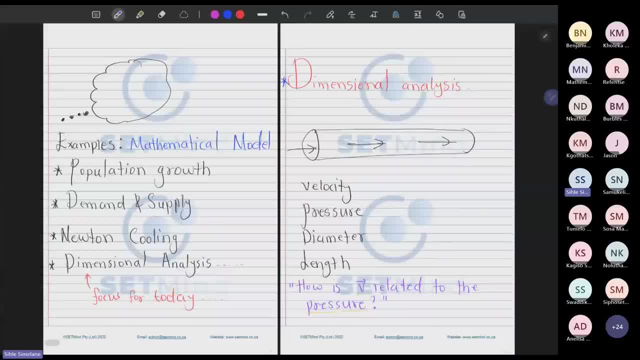 people fail Because dimensional analysis is only a part of the course. After dimensional analysis, you need to jump to population growth. Then, after population growth, you need to jump to demand and supply. After demand and supply, you conclude with newton cooling. So there is work which still needs to be. 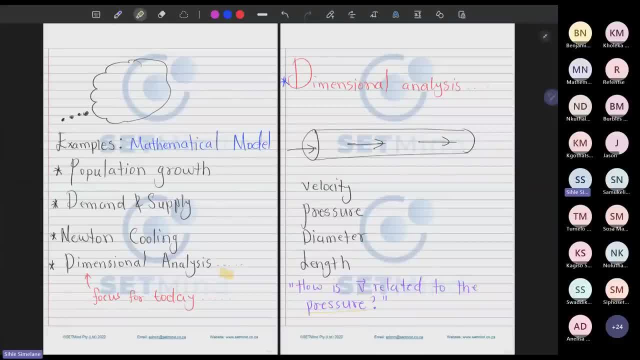 done, but at least you have checked out the first part. So when they introduce it, it is not going to be as harsh as it would be if you went into class with no idea of what is going on. So please go ahead and jump in. 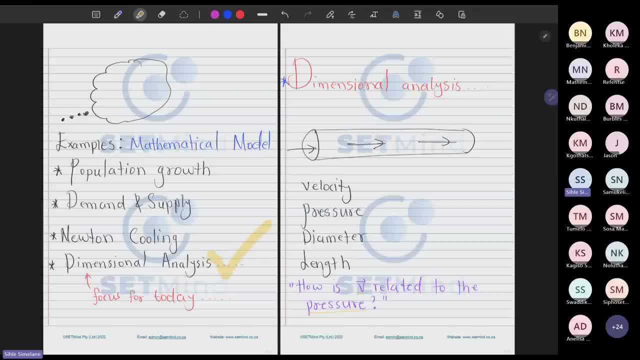 Is there more which you would like me to say or is there a question that you have? No, that's fine. thank you, No problem, Anyone else? Anyone else with a question about dimensional analysis Or a question in general? It is about, say, passing second semester. 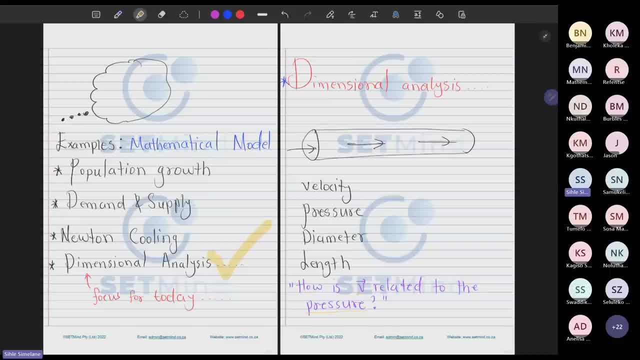 or passing subjects in general, or coping, studying. Whatever question you have, please feel free to drop the question and then I can comment. the best way I know how, And if there is one thing I need you to process is we are about to conclude, is that 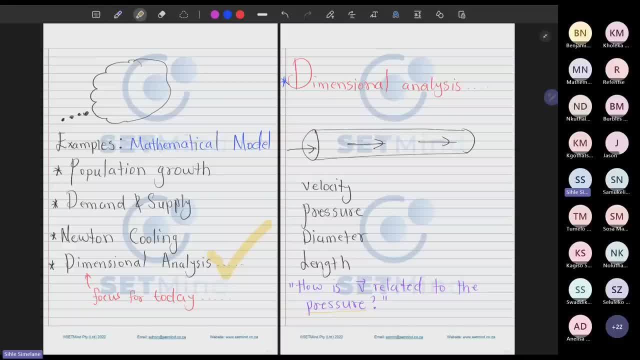 if there is another human being who can make sense of the concept in their head, then it means it is not impossible. It is either. number one: the way you are working is not effective, and that is why you need to reach out to people who are doing. 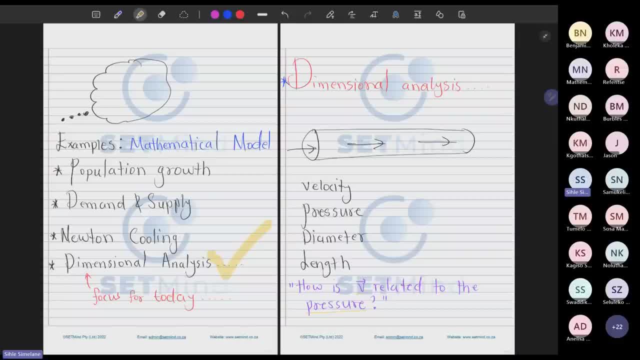 reasonably well so that they can assist you to reach their standard. If there is someone who understands what you are struggling with and would say the problem you are getting frustrated by is easy, then it means actually it is not really difficult. So my advice to you, as you are about, 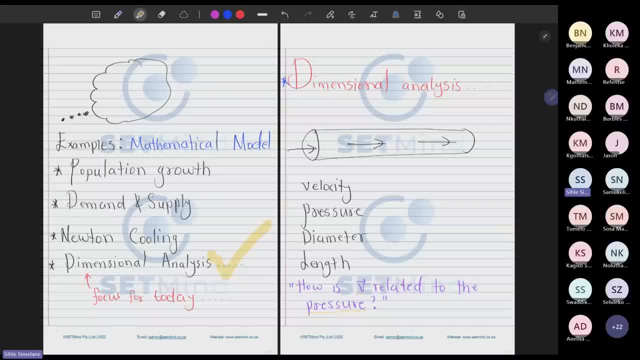 to start the block is number one. make sure that the people you hang around with are in the direction which you plan to go to. If last semester you were not happy, you got 57, 56- which person is really great, but you are hoping to get. 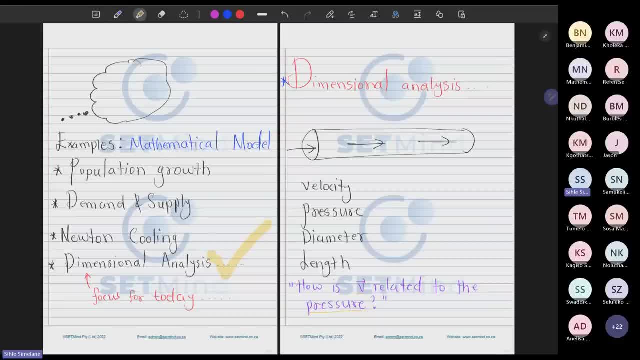 70,. try to look for that person in class which you see that they are in that direction and talk with them. maybe sit with them, practice with them when they do their practice session. you will learn something from them And the problem with people approaching others. 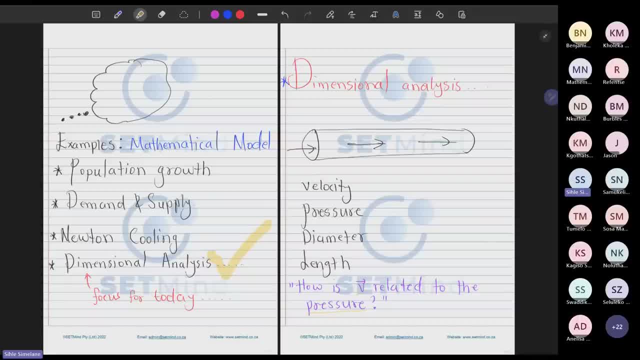 to help them to study, because this inherent nature in many people who want to compete, even where they are not supposed to compete. So some people you meet them to compete with, they are just supposed to help you to pass and then you move on. that is the end. 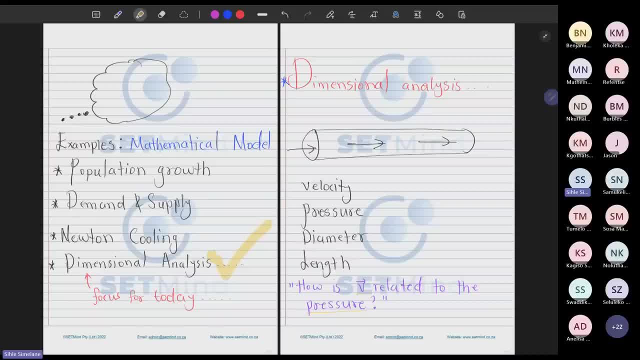 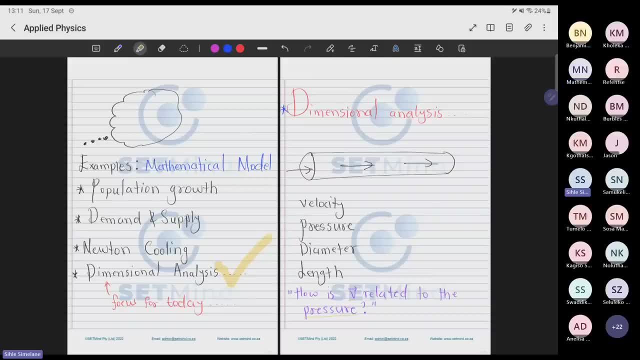 So if you can start not looking at things in the eyes of competition but rather say there are people who are genuinely there to assist you to pass, and then that is the end, there is no need for me to say I am trying to compete with them, because I am also. 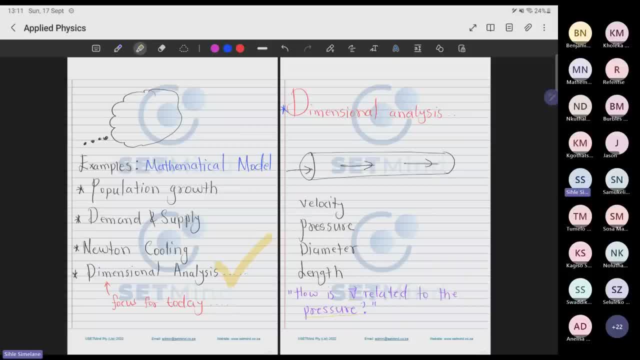 trying to survive with them. There is always going to be someone who does more than you do, and that is the reality. So please, as you are about to start this semester, get in study groups and send questions. You know the notion of people sending many questions the day before a test. 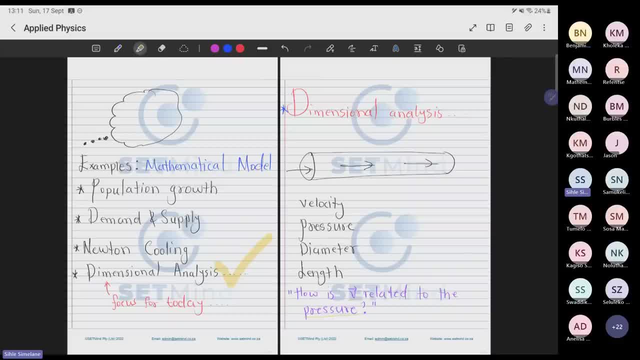 or the day before an exam. it really does not make sense, It doesn't help. It doesn't help. So you don't want to discover two days or one day before an exam that actually dimensional analysis is easy, That actually differential equations are easy. 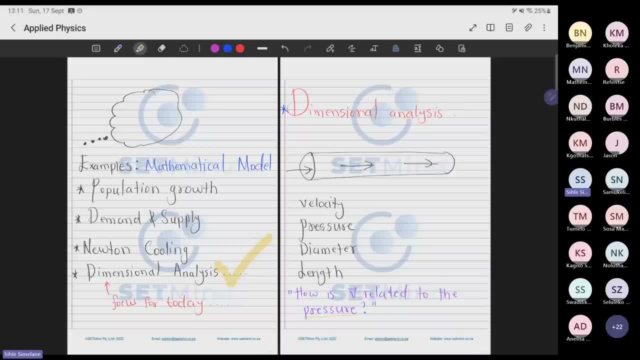 That actually complex numbers are easy, That equations of planes are easy, That all the topics you are doing in all the courses are easy. You don't want to discover that two days before the exam because it is really emotionally draining to see that. So as you go to 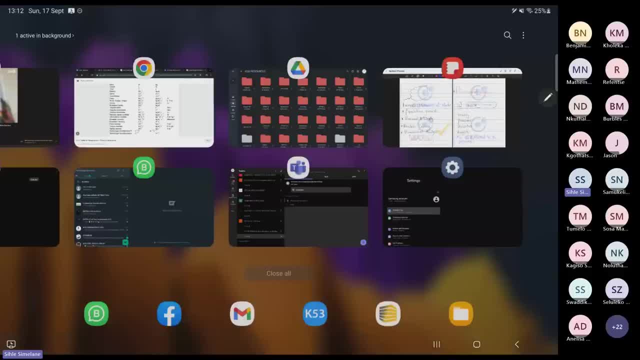 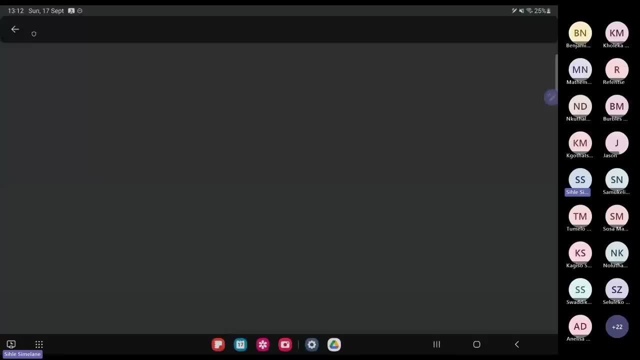 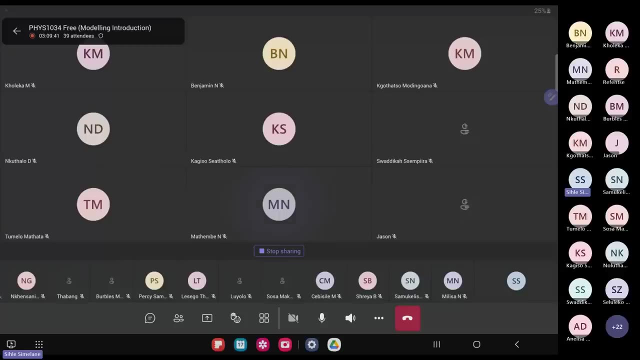 work. please make sure that you normalize working way in advance. so study groups collect a number of friends. meet with them there by WSS and home study groups. believe me you will read the that come at the end of the semester. Reach out for help and consult. 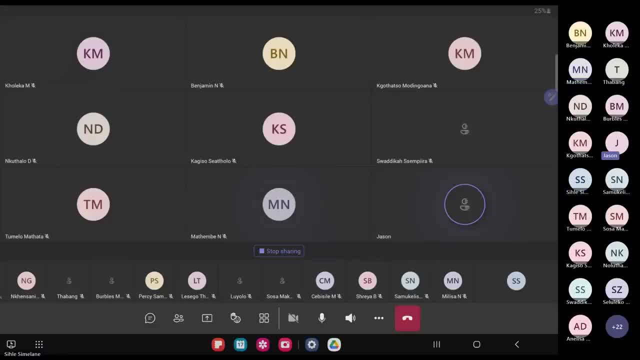 Do you have any questions? Yes, will there be any other? I always want to sign up for the state mind and when the next videos, like these online lectures, will be. So the plan is we will have. we will have three sessions there and there, but there will be. 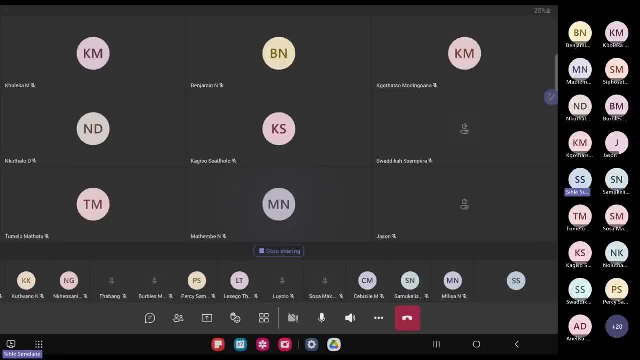 sessions where there is subscriptions, where we are hosting them on a weekly basis, where there is consistency. So, for example, next week we are going to be taking the sessions online and then doing them, because this week was just to expose you to the concept and some of the questions were: 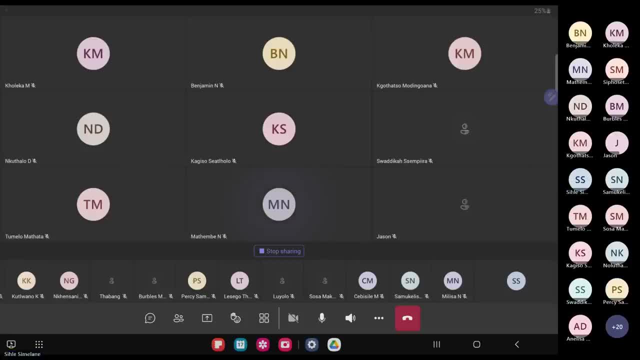 well, not structured, because I was just thinking them on top of my mind and the sessions are obviously going to be online, and the reason why we make sessions to be online it is not that we can't be there in person, but if a session is online when you prepare for your exam. 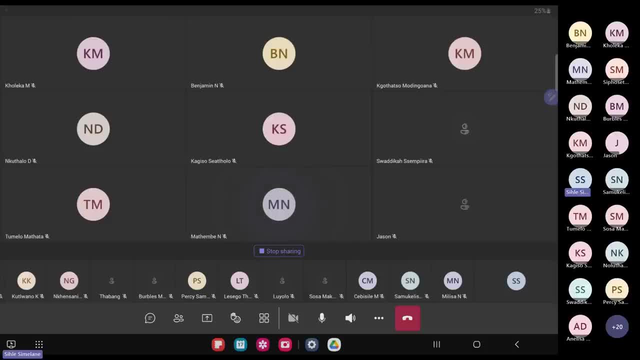 I forgot how to do dimensional analysis. the recording will be sent to you, so you just go to your email, go to your drive and then watch the video, access the PDF I was writing on and review what we covered, and then you will understand. but if we do it in person, 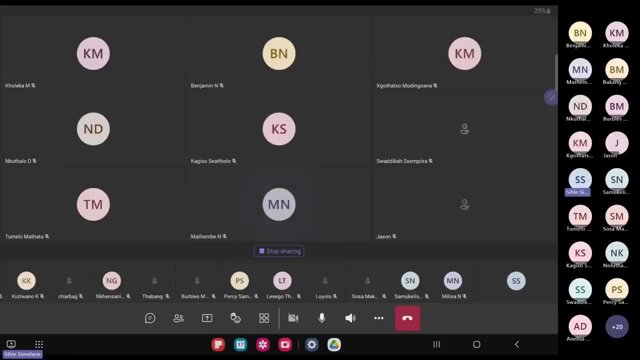 it's either you hear what I said or you don't. Come revision time, you need to battle by yourself. so that's why we are in favor of online sessions, but there is obviously we are going to carry on in person session, one on one. but as far as groups are concerned, 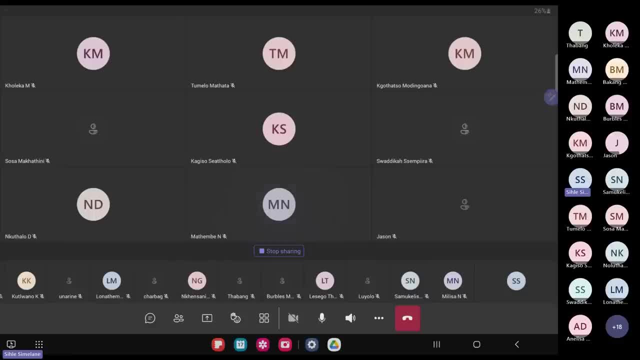 we are going to carry on working online because in a group there is someone who will ask a question which is useful and it will help the others. and the sessions we will make them to be weekly sessions. a month you will pay. if I remember it should be 400 lends.